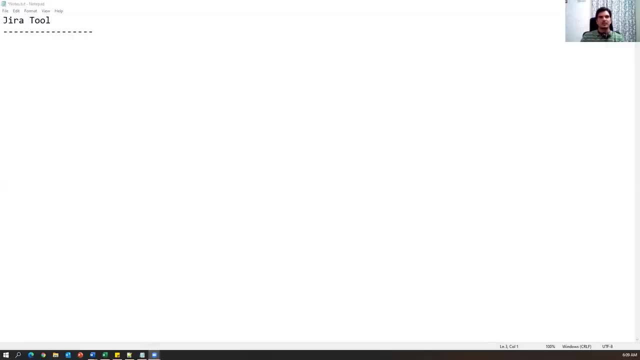 automation tools, performance testing tools, security testing tools. So there are a number of tools are there in the market especially for testing. Okay, And these are different, different type of testings. we have a different type of tools And again we can divide these tools into two different parts. One is management tools and the other one is automation tools. So what is a management tools means? What is the process we are following And what are the documents we are preparing Or what are the activities. 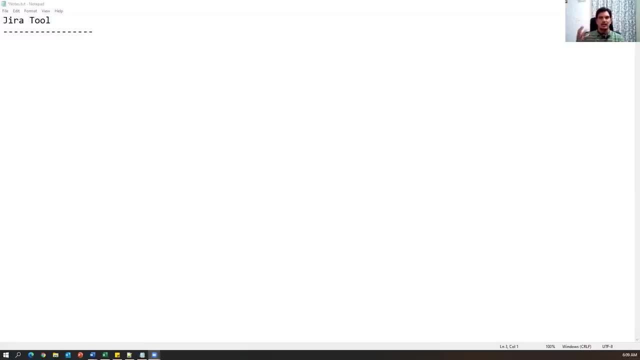 we are doing throughout the testing cycle. we can track all these activities in a tool, instead of using the templates or instead of using Word or Excel templates. we can track all these activities in a tool, So they are basically comes under test management tools. So, whatever activities we are doing throughout the testing process or throughout the testing lifecycle, we are organizing the tasks or managing the tasks or tracking the tasks in a tool. those tools are comes under test management tools. 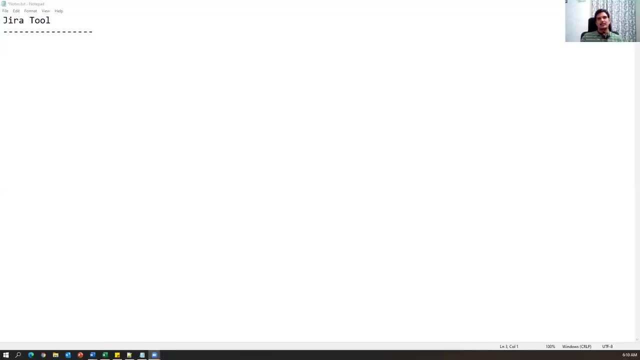 so what we can do in the test management tools: we can define the requirements, we can write the test scenarios, test cases, and we can update the test case execution status and we can report the bugs. okay, and finally we can close the requirement. so all these things are testing activities, stlc. 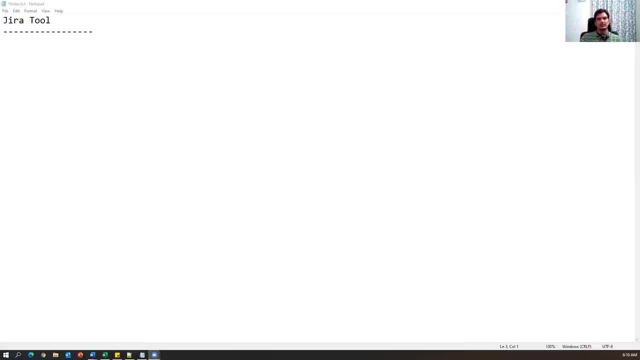 so these activities we can do in the tool itself instead of using the templates. so that is there. some tools support these activities, so those tools are comes under test management tools. there are some other tools called bug tracking tools or defect tracking tools, and those tools will be used only for defect tracking, so whenever you find a bug, you can report the bug through that. 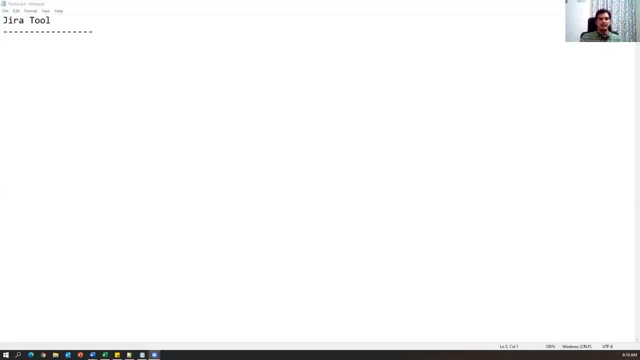 particular tool instead of using templates, so you can just write the defective description, priority, severity steps. you can attach the screenshot. i can send it for developer and developer will take care of the defect. so they are all comes under the defective tracking tools or bug tracking tools. that is another type of 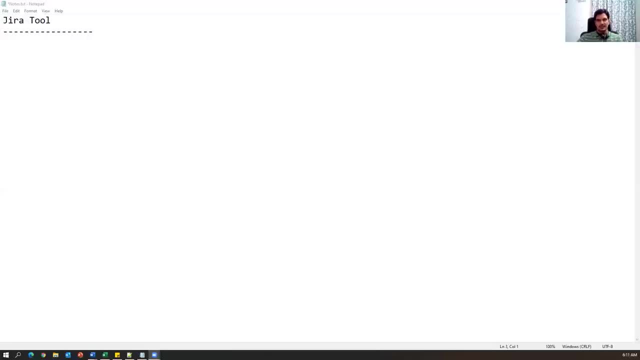 tools we have. okay, and let me just write here: understand the difference, which is very, very important as a beginner guys, okay, people may expect something in an interview, so do you know the differences between these tools or not? so, the test management tools: test management tools: okay, so each and every activity we can track in the test management tools, like from the beginning. 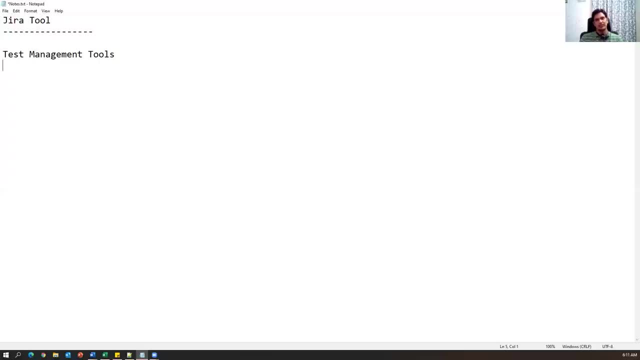 test cases, writing test cases, execution, bug reporting- everything we can track in the test management tools, and similarly we also have bug tracking tools, back tracking tools or defect tracking tools, and these tools only for bug tracking or defect reporting tools. or we can say bug reporting and tracking tools, bug reporting and tracking tools, we can say defect. 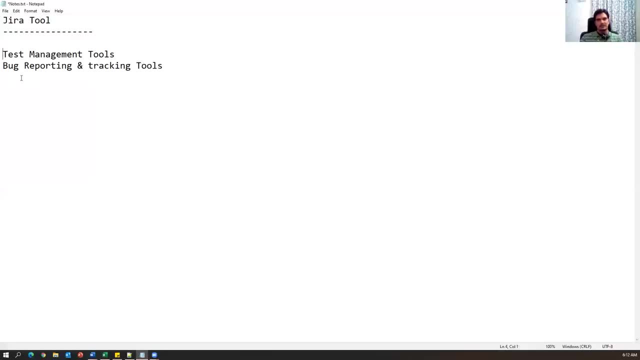 reporting and tracking tools also. everything is fine. so these are the two main- and أvel. so these are the two main tools we have apart from this. okay, we also have automation tools like selenium, qtp. these are all test automation tools. so whatever test cases we have we can. 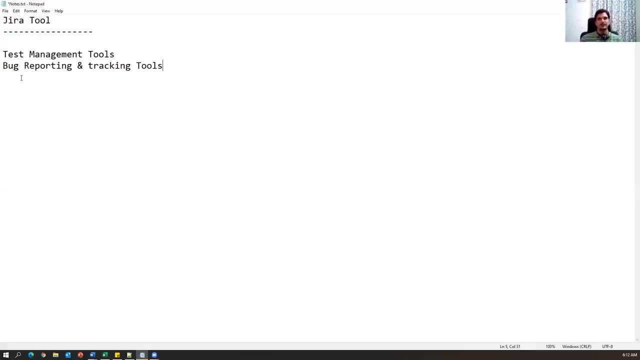 automate those test cases. okay, they are the completely different tools and these are the process related, like what are the activities we do during the testing. we will automate all these process tasks, like we can track how we can maintain the activities in those particular tools. so test management tools and bug reporting and tracking tools again. 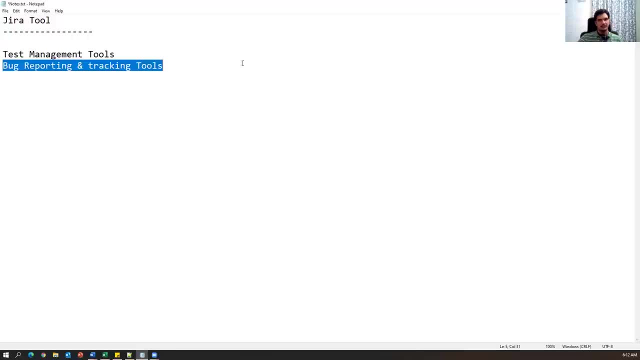 the test management tools also having features of bug reporting. so this is also part of sdlc. so test management tools: when i use test management tools, we can also use it for bug tracking purpose. okay, but apart from these two, there are other other type of tools called agile. 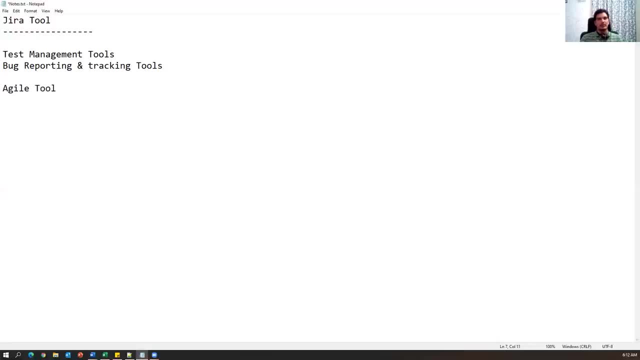 tools- okay, agile tool. so what is agile tools? or agile tools means? basically, these tools, especially these tools, are the tools that we use to track the activities of the test cases so we can design for automating the agile process. okay, especially these tools are designed for tracking. 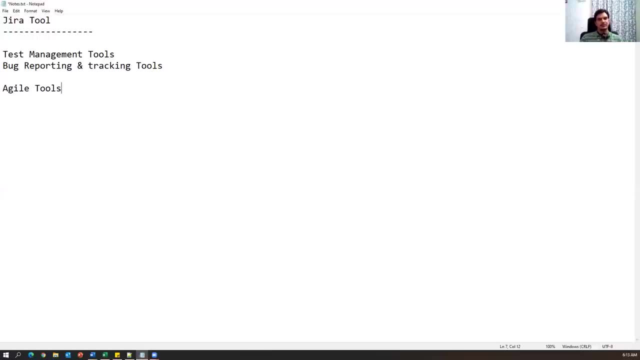 the agile tasks, like in agile process. in the previous session we have discussed about a lot of things like from the epic stories we will define by the product owner and then after that we will have product backlog. then we have a sprint planning meeting. then we will select the some of the stories. 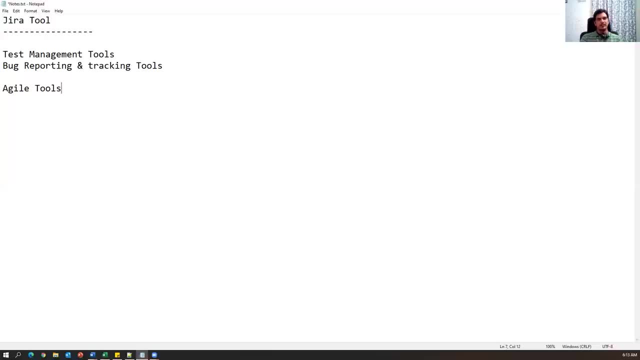 from backlog and we prepare the sprint backlog which contains some of the stories which are committed by the dev and qa. then we will have a sprint and the sprint duration will be two to four weeks of time and once you start a story which will go to different stages, like starting the 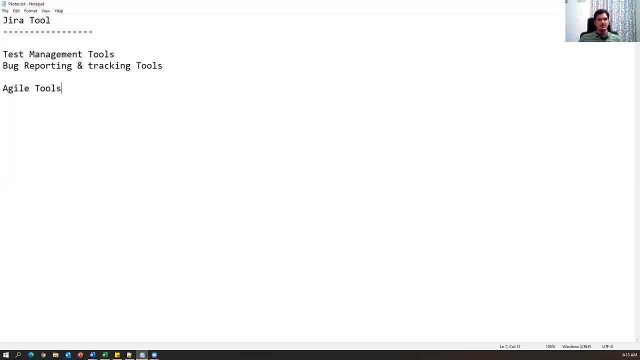 story, development, testing, deployment, so multiple stages, the story will go on and finally we will close all the bugs related to the story and we close the story and we will demo the story to the product owner and finally release to the customer. so in this agile process, whatever activities we 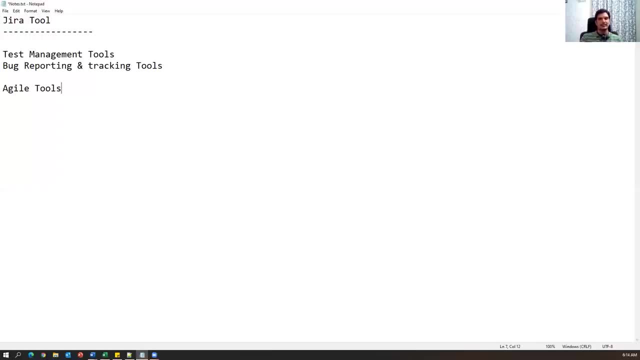 are doing so. to define this agile process, we will have to define the product owner and then we will have to define these activities and tracking these activities. we have a different tools called agile tools, and all the scrum related activities we will perform in the agile tool itself. and 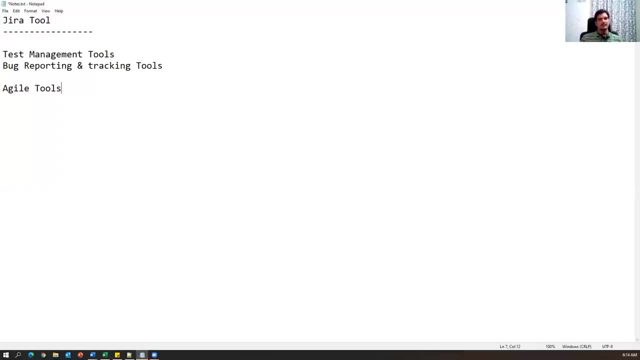 we can also maintain the scrum board or storyboard in the tool itself and we can generate the graphs like burn, burn down chart and velocity chart. so all these things we can automatically generate in the tools and everything we can do, whatever activity, even the small activity, whatever you do. 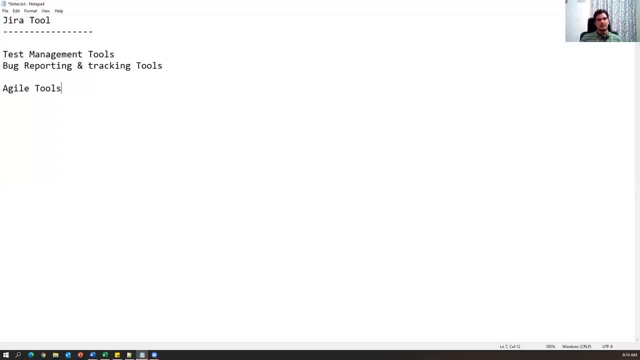 we can track or we can define those activities in the agile tool. okay, so that is all about agile. so what are the tools available in the market? as part of agile? we have most popular tool is jira. okay, and apart from this jira, we also have something called. 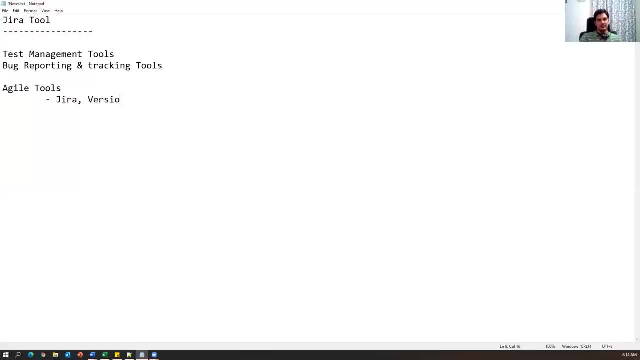 version one. so this is also one of the tool which is available in the market. okay and uh, team city. okay and uh. there are multiple tools are available in the market. some of them are free, some of them are open source. okay, okay, these are all comes under agile. tools means. 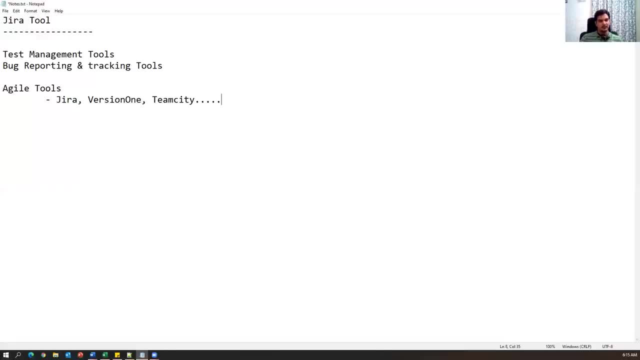 each and every activity in the agile process. agile process contains, again, development activities, testing activities. everything will be part of agile. so these tools will assist you to define each and everything which we follow in the agile process. okay, so these are the tools, which are examples of agile tools. so now we are going to discuss about. 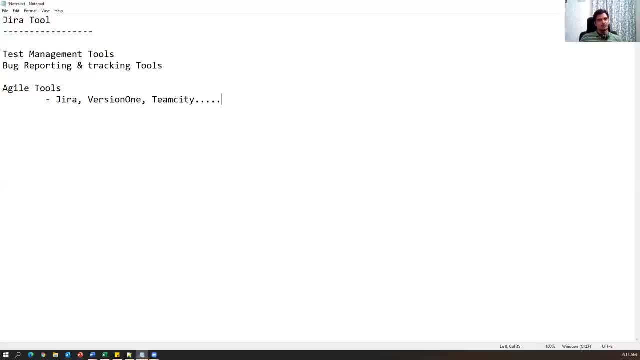 agile management tool. so jira is a purely agile management tool. we can say agile management tool. each and every activity we can define we can track in jira tool itself and this tool can be used by developers, tester, product owner, so over is working on the team in the agile team. they have access on. 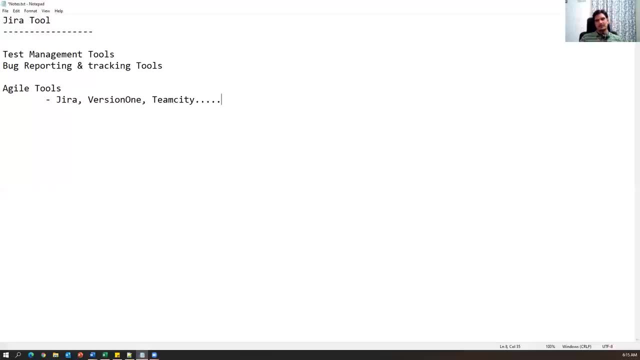 jira tool. okay, so in the jira we will do a lot of activities. so i will just show you what are the activities we do. first i'll list out here and then we will do step by step. okay, so what is jira? so we understood what is jira. so jira is a agile project management tool, or we can 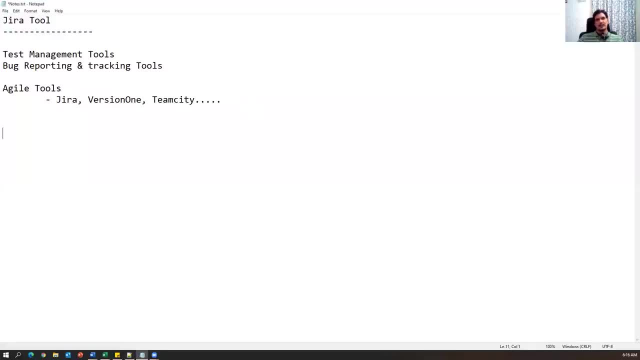 say agile management tool. jira is a agile management tool means which includes the development activities, testing activities, product owner, everybody will track everything in jira itself. we should not go out of jira tool. even in jira we can also do test management activities, but jira itself is not. 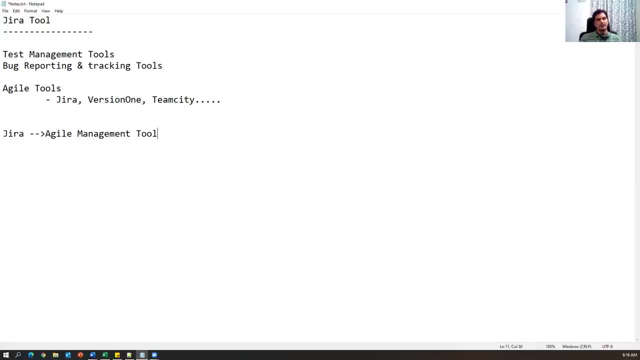 any test management activities by default. so by default jira and jira. we cannot define the test cases, bugs and everything, but we have a special plugin called jeff fire and if i install that particular plugin in within the jira, we can also do test management activities. right, we can also. 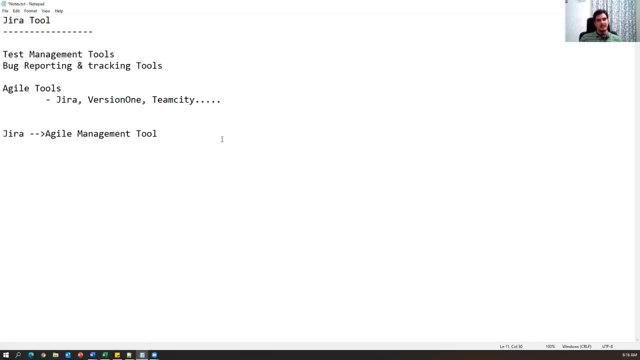 define the test cases, we can write the test cases, we can upgrade the status of the test cases, we can report the bugs- okay, and we can generate the test simple test reports. everything we can do in the jira itself by by using jeff fire plugin along with the jira- okay, apart from the agile management. 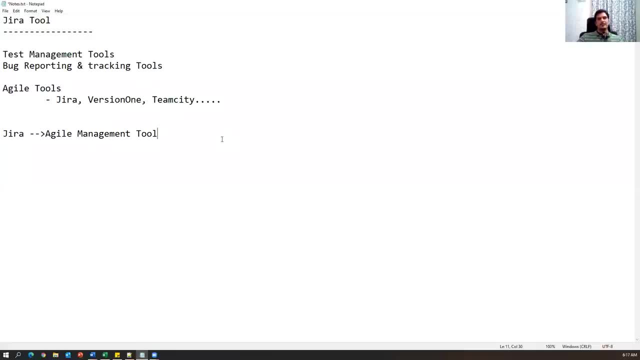 activities. so we will see all of them practically. so first of all, let us start. so first we will see how to install and configure jira tool. okay, and there is some workflow is available, so we need to follow that workflow- jira workflow. so what is the jira workflow? so let me just write here: 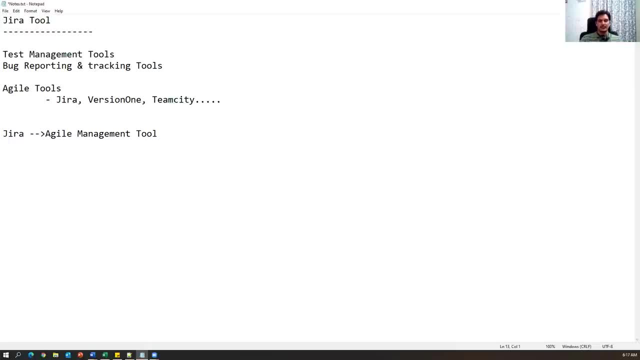 jira can be used in two different angles, guys. okay, the first thing is we will see how we can use jira for tracking the agile related activities. what is mean? what is meant by gel related activities? first we will have creation of project and then we will have a backlog which contains different stories, epics and stories. 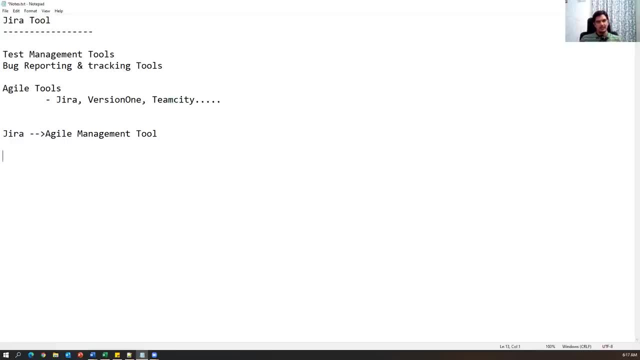 we will define and after that we will create a sprint and we will add stories to the sprint and then we will start our sprint, which will go two to three weeks of time, or four weeks of time, and during the sprint there are multiple tasks we are going to do for that particular story. so for that, 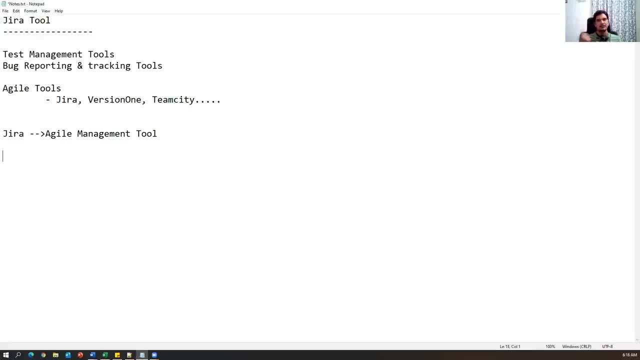 particular story and developer and testers: both will write their tasks for each story and they will cover, they will complete those tasks during that period of time, or sprint time, and finally we will close the story. so this is called as a workflow. okay, once the story is defined by 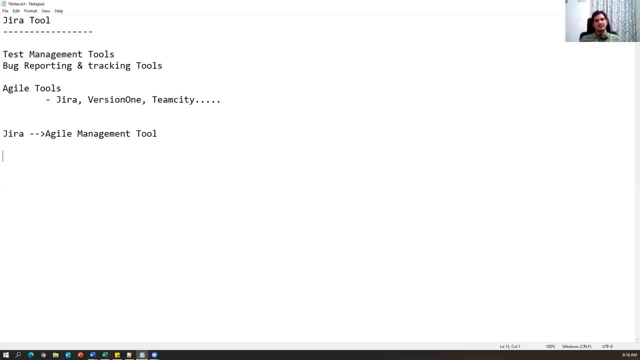 product owner. the story will go to different stages till it is closed. okay, so that is basically called as a workflow. so that is agile process, agile workflow in jira, and apart from this, we also have a test management activities. right, that is a different workflow again. so once you install, 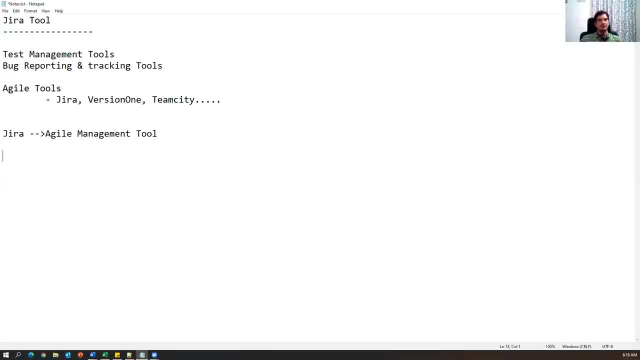 java fire plugin within the jira. we have to follow a different workflow to perform test management activities like: first we need to uh create our test cases or we can import the test cases. suppose in excel you have n number of test cases, so you need to upload all the test case at once in the 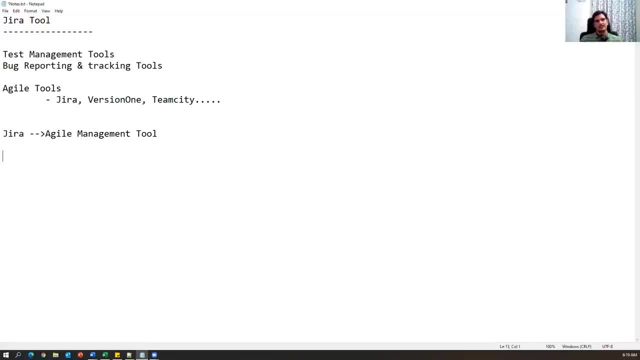 jira. you can also do that. you can import the test cases and then you can import the test cases, and you can import all the test cases once, instead of writing each test case individually takes time. so you can import all the test cases in jira once and then we can create a test cycle. 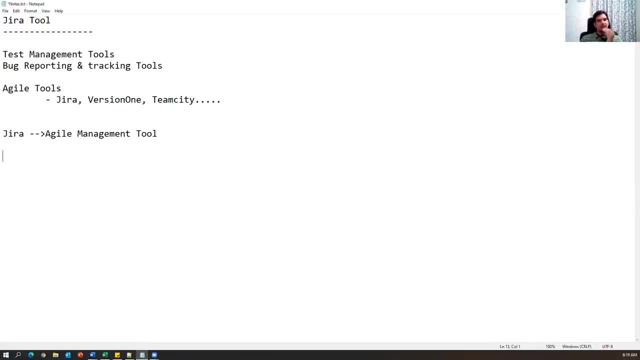 then we'll add the test cases to that particular test cycle, then we can execute the test cases, and if there is any failure we can report the bugs and then we will generate the reports. so these are all test management activities. so these activities also we can do in the agile. 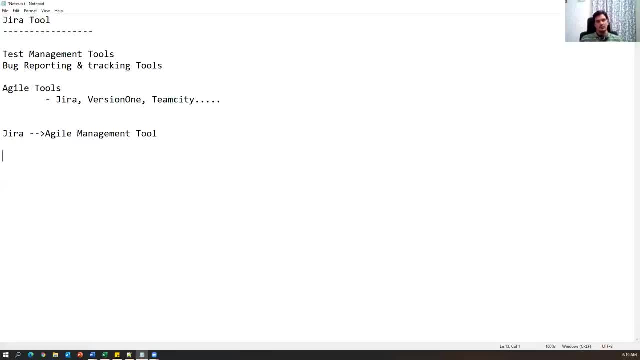 or in the jira tool, and it is also having a different workflow, okay, so first of all, we will see agile part and then we will come to the test management activities- how to write test cases and everything we will see later. okay, so that is all about workflow, jira workflow. so first let us 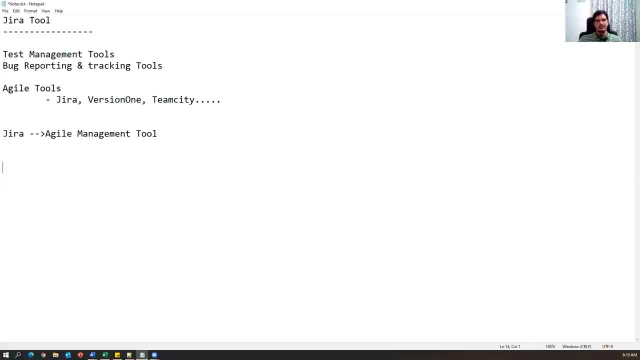 start with, uh, agile related activities, how we can uh do agile related activities in the zira tool. okay, the first and most important thing is i'm going to show you so what are agile or scrum activities. okay, so i'll just show you what are agile or scrum activities. 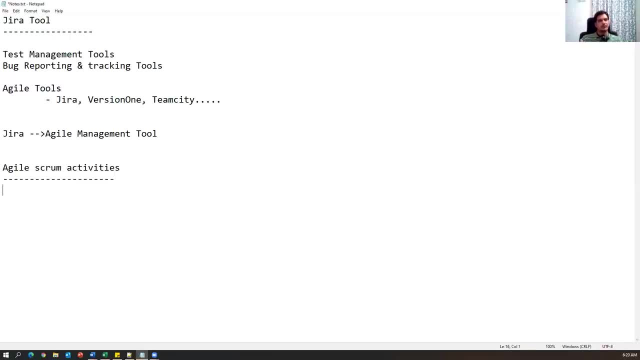 list out here step by step, one by one, and then we will see how we can perform them in jira tool. so before doing that, i'll show you how to install and configure uh jira tool. okay, so first we will see how to install and configure zira tool. so 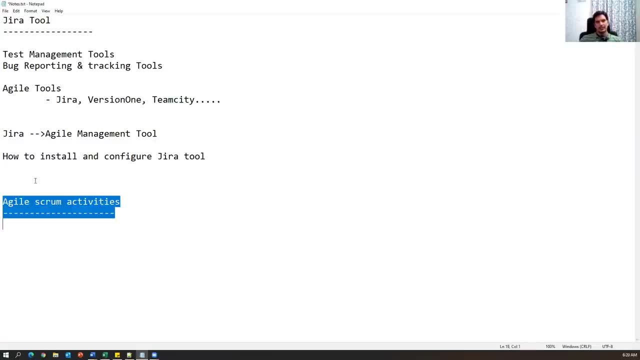 jira is basically uh available. okay, let me discuss this later. so, how to install and configure jira tool, this is the first thing which we need to do. okay, so jira is basically agile management tool. okay, so, which is uh available in two different flavors. so which is available in the two different flavors? and if i just go to jira official website: 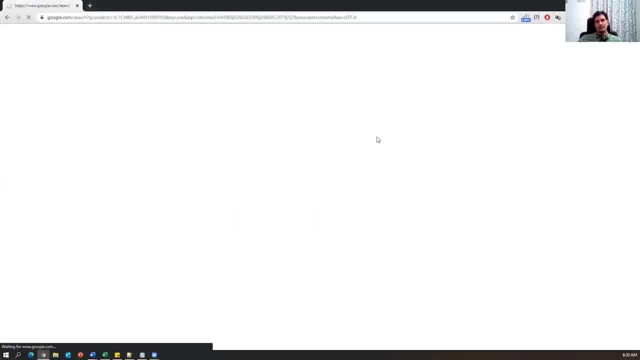 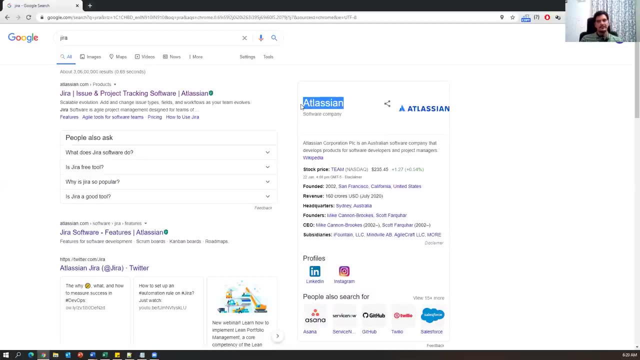 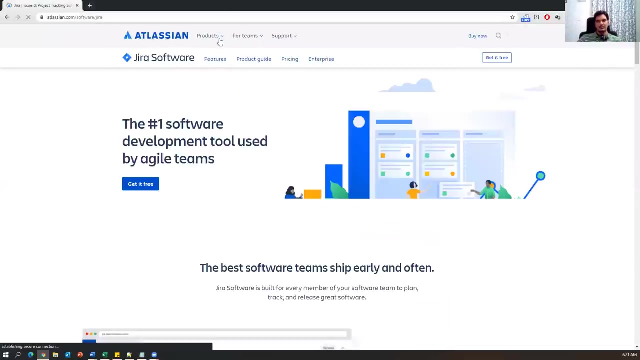 i'm just searching jira tool, okay, and this is from atlassian company. so this is a company and this is a product-based company. they will develop different type of products and jira software is one of the product of atlassian company. okay, so now just click on this atlassiancom software, jira. and if i just look at here, these are the: 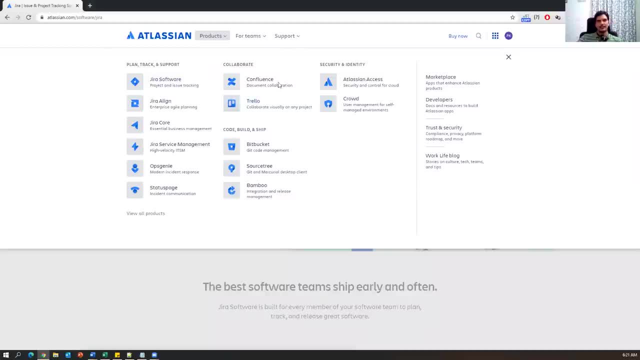 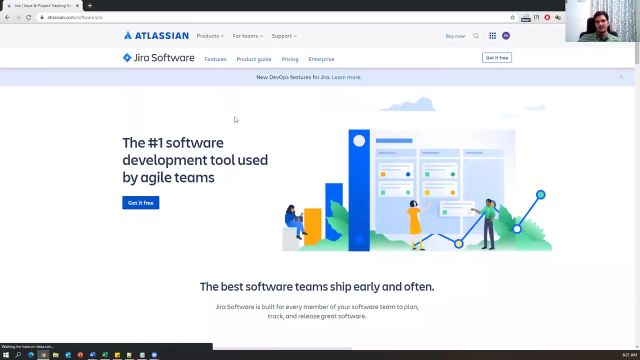 different products they develop from the atlassian company, and jira software is one of the most popular software for agile jira software. okay, now, if i just click on this jira software, you will get some information about the jira tool. so this is a page you will get. 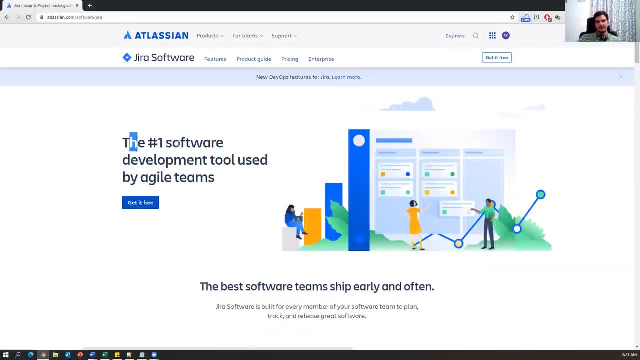 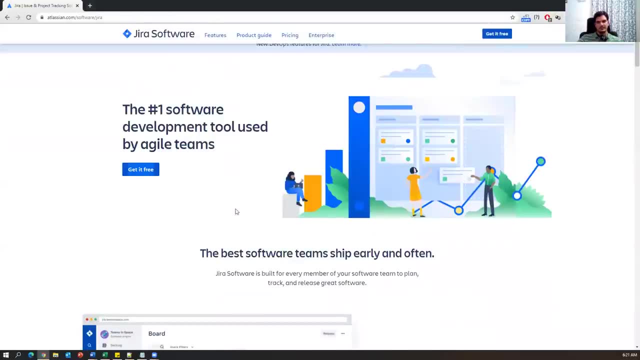 and they said it is a free cc. number one software development tool used for agile teams. so they said it is get it free, but this is free only for 30 days. okay, and this software we no need to download. okay, we can also download install, but it is again a complex process. we. 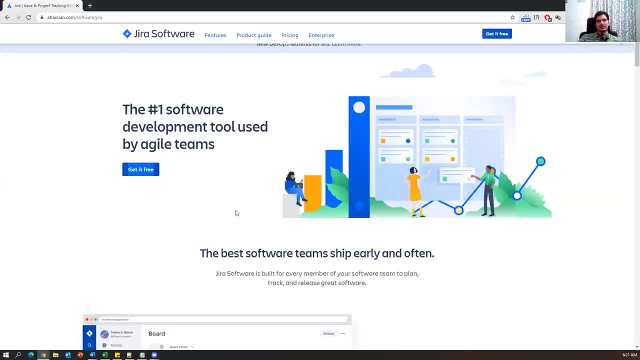 need to set up a server and everything. so instead, what you can do is we can create a jira instance on their cloud. so cloud means what they allocate some space and they will configure jira for us and they will provide the link to us so we can use that link. 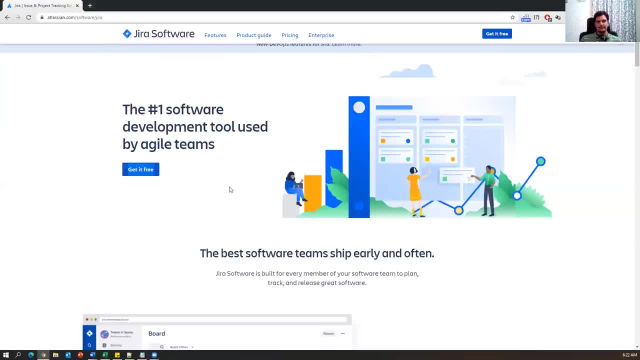 and we can work with the jira tool for 30 days. okay, so the jira is available on the cloud, so they will. we can create our cloud instance for jira software and we can use it for 30 days. okay, if you want to plan any practice anything, so within 30 days we can finish it out. 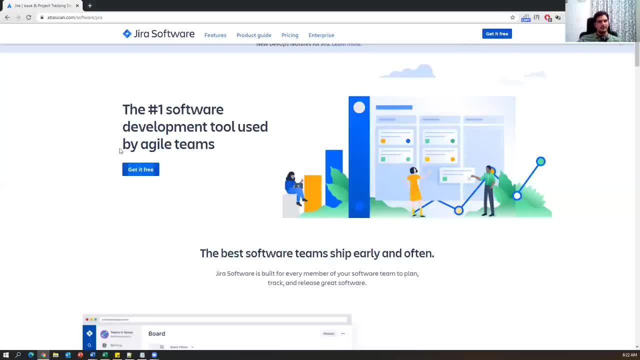 okay, so this is for 30 days, if available, and uh in within the 30 days. within the 30 days or 10 members you can use the software because in the jira there are multiple people are using right product owner, testers, developers, scrum master- so multiple team members will be using. 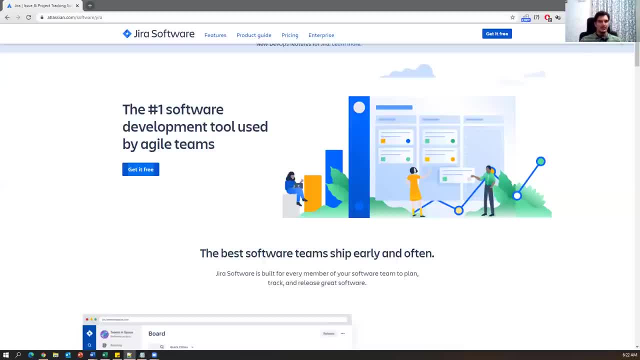 jira tool. right, so all the users should be part of the jira tool. so this particular cloud instance will support maximum 10 users. okay, so within 30 days, dingually, we can add 10 users and you can work with the zira tool. so that is a limitation which we have on. 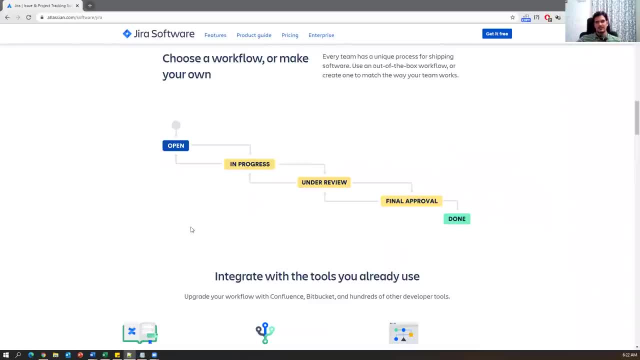 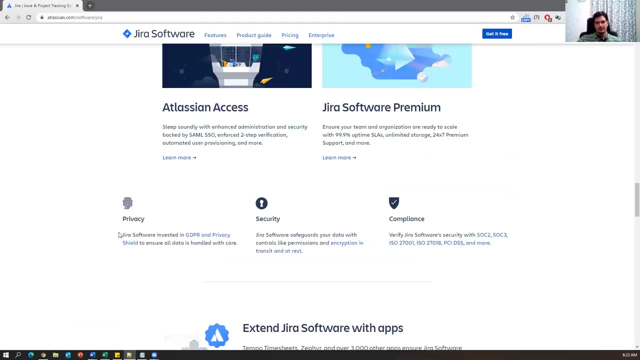 cloud instance. okay, so they have given some information about this jira tool and workflow here. you can just look at here. so open in progress, under review, final approval done. this is a small workflow of agile as per jira tool and some other information also they have provided in this. 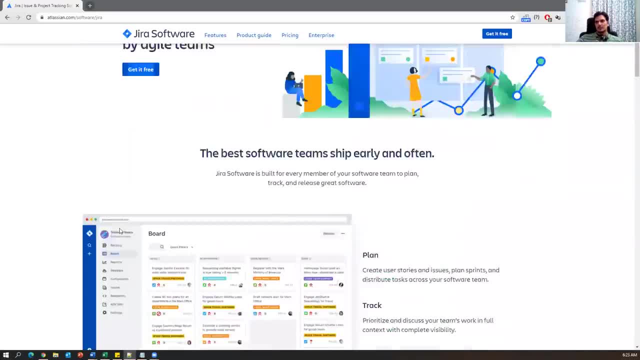 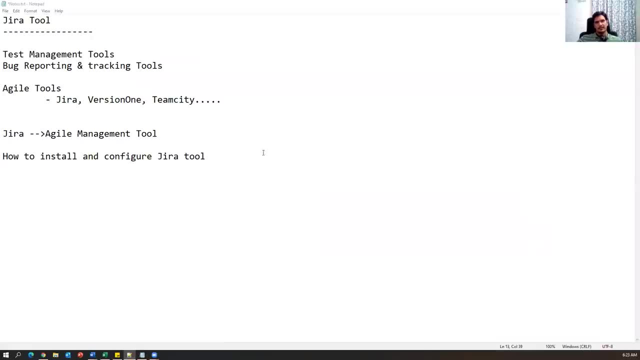 particular website. you can just go through this later. so how we can uh con, how we can install and configure jira tool. so basically, they have provided jira in two flavors. okay, one is uh in the cloud itself. we can have uh two types of instances. one is a free version and 10 users are. 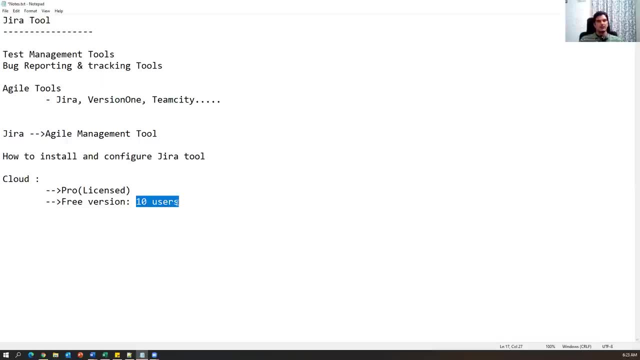 limited. and the other one is: if you want to still continue after 10 days- sorry, after 30 days, 10 users, 30 days, okay, so after you want to continue with the zira after 30 days, or if you want to increase number of users, then you have to go with provisional version. so this is a licensed 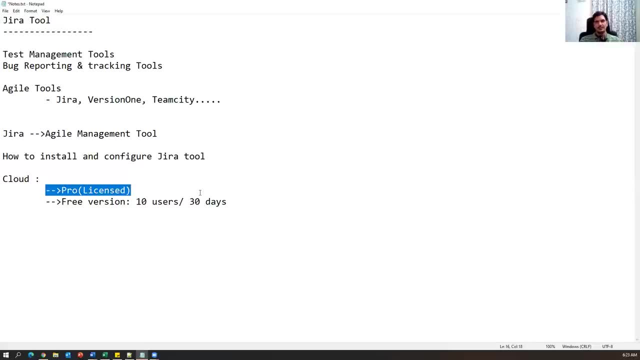 version on the same cloud, the same url. you can still use it, but you need to pay for uh, the jira tool, so we need to buy some license for that, which is professional version which is available for 30 days. 10 users we can access freely on the cloud. okay, so nowadays we 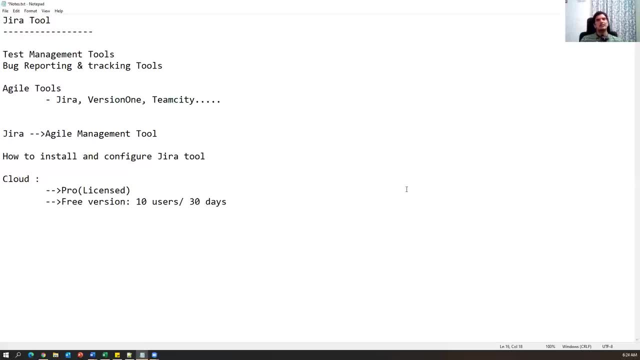 most of the companies are going with the cloud instances, guys. okay, they are not setting up any environment in their locally. they are not ready to setting up any machines to install a complex softwares. so most of the companies are moving to the cloud. so nowadays cloud technologies are becoming very, very popular, so similarly most of the softwares also companies. 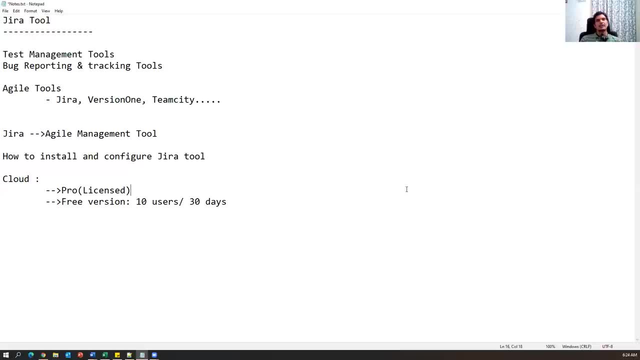 are offering on the cloud environment directly. so we can have an instance on the cloud and we can use it for our company and as many days i want. so after that, after i completed my work, i can close it. okay. so some companies, uh, initially they offer a free of cost and after some duration we need to pay for them to maintain our instances on the. 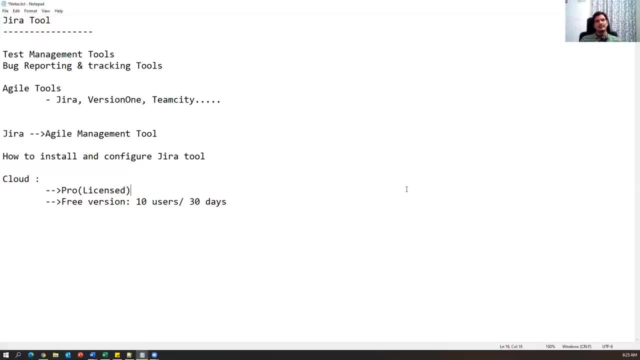 cloud environment. okay, so now jira is available on the cloud and basically they are offering two flavors. one is free version- 30 user- for 30 days we can use and then, if you want to still continue, we can go with provisional version, which is a licensed version. okay, so now let us see how we 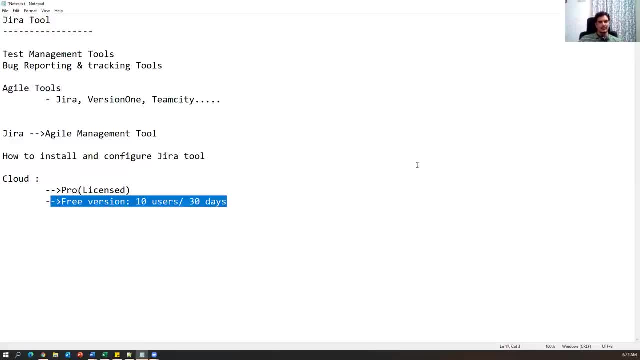 can get the cloud instance to work with the agile. okay, so now i'll show you step by step. so please concentrate on this. so what we need to do is, uh, i'll just provide you one small link which will go to jira download location. okay, this is a link. so if i just go to this link, 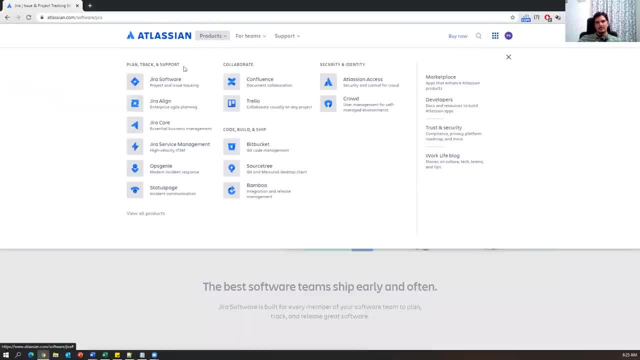 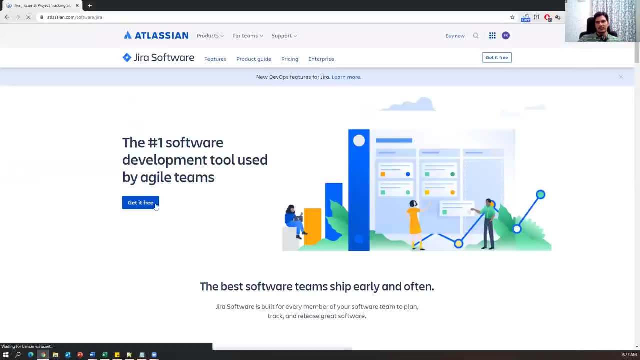 or you can just go here. also, you can just go to jira software. you can go to jira software and you can go to jira download location, and you can. i have provided direct link here. or else you can just go here. get it free, click on. get it free. okay, now you can just look at this website and this page. you can get- and if i just look at, support up to 10 users or three agents and includes the 2gb of storage, offers community support. it always free, no credit, no card needed, but it is only for 30 days. okay, right, so? 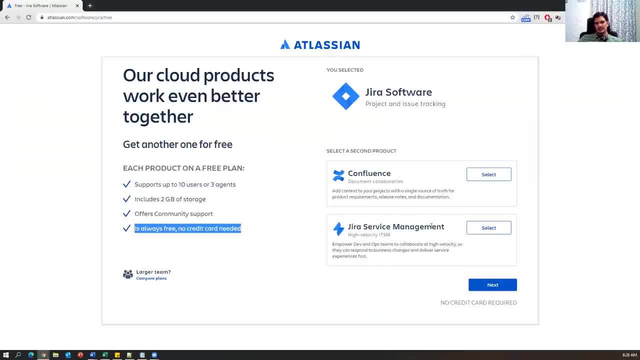 so they have given two things here: confluence and jira service management. so we don't need to go for confluence- it is only for document collaboration tool- and we need to go for jira service management. okay, or else you can just click on the next, no need to select anything. 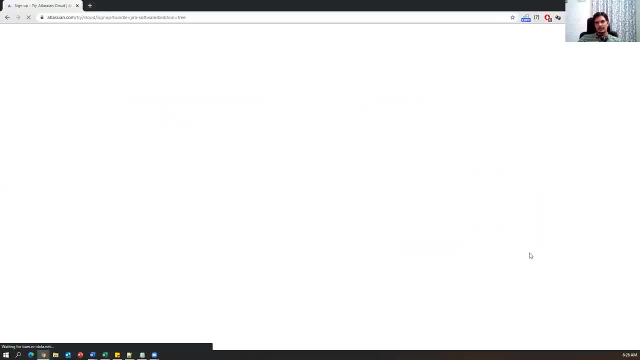 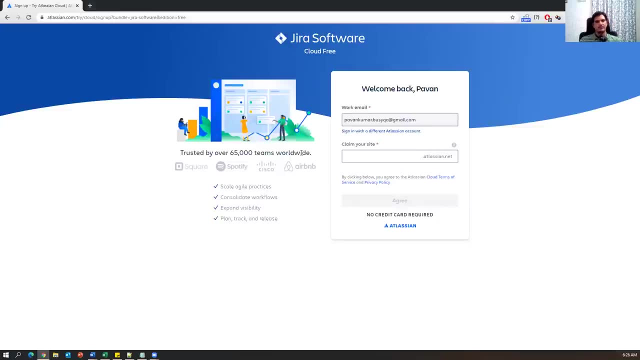 you can just click on the next and here, which will show you a few things. so here it will ask you the login guys. okay, so first of all, before creating the cloud instance of jira, you have to use your gmail account. okay, with that gmail id, which will create a new instance. 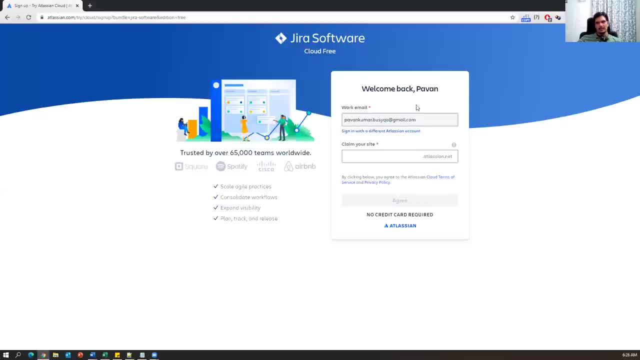 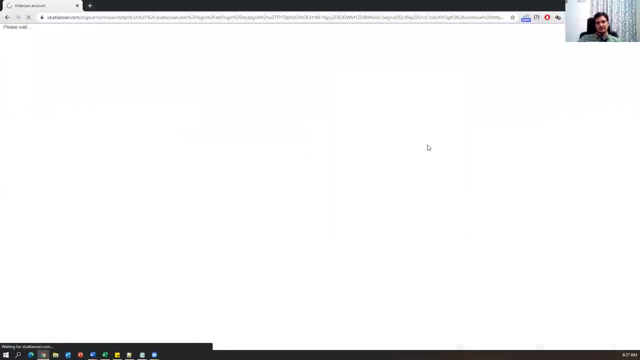 so here you can just provide your gmail account. so what i will do is i'll just provide my email account. so sign in with a different assistant account. i'm just atlasian account. i'm just clicking on this and you can provide your gmail id just a moment. so first time it will ask you. 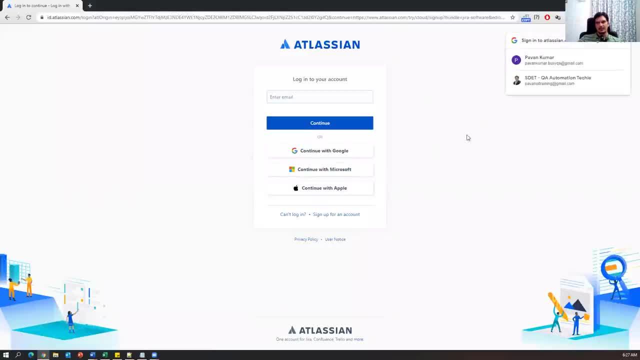 to provide your gmail id, because you need to sign in with your gmail account and you can just click on this sign up with the site. yeah, now you will get this screen, okay, so here, whichever account you have, you can use that account to create an instance. so i'm just choosing the. continue with the google. 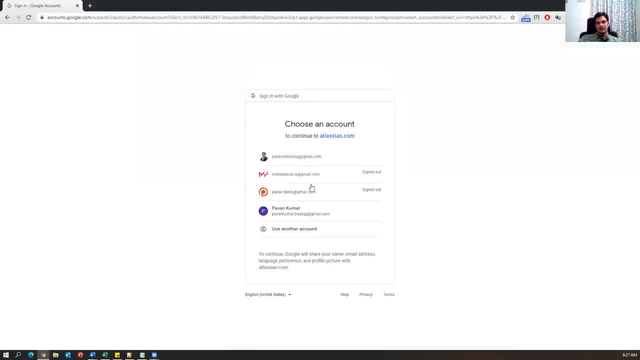 and i want to use my gmail account, so i have multiple accounts. i'm just using one account here- my gmail account, existing account- and you need to just provide the password here and then click on the next, so your gmail account will be used as your jira account. okay then. 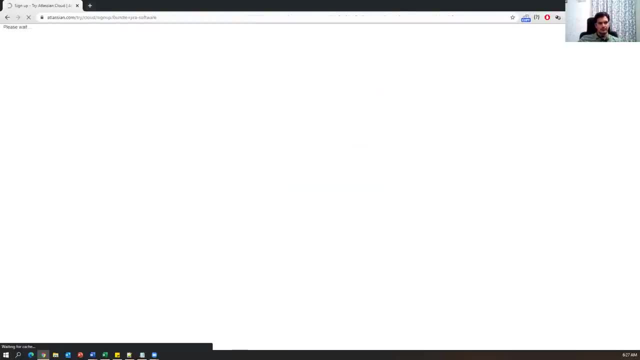 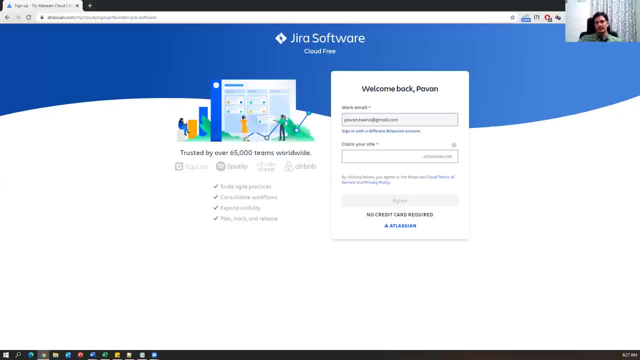 now it will go to another screen. so once you provided your gmail account, okay, now you can just look at here: this is a gmail id currently you are using. okay, to create your jira instance. and then, this is most important step- climb your site. so here we have to provide some uh name. what exactly you are looking in the url? 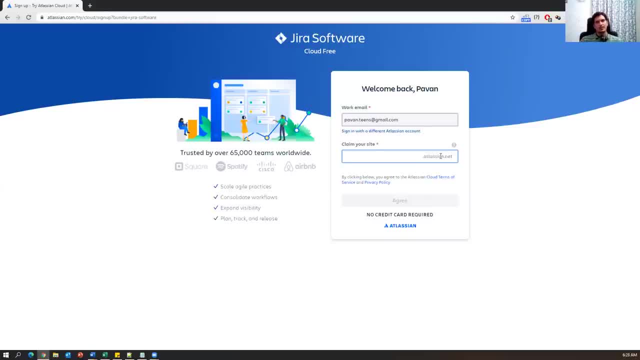 so when i accessing the jira tool, you will have to provide some url. so what should the url contains? okay, that url you have to specify here. okay, so let me just show you what exactly it is. so here, uh, just a second. so let me just give something called zira, demo by power. so when i 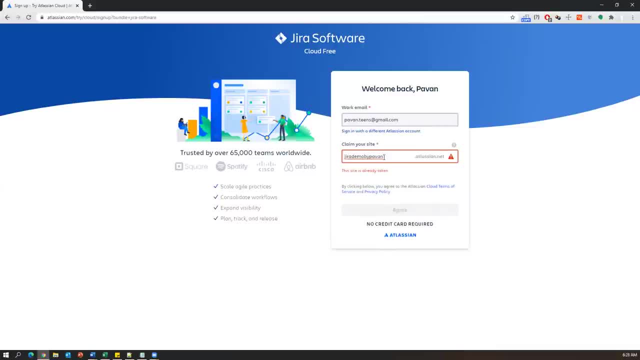 enter something which will check which is already there or not. now we can just look at here: this site is already taken, so we need to give something else. okay, so we need to give something else, so let me just uh. okay, so we need to give something else, so let me just give some other name. let's say: 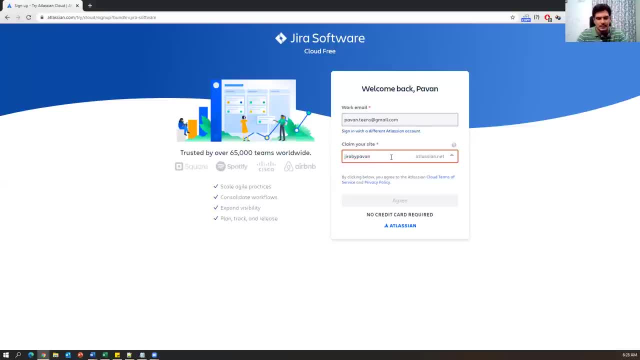 uh, instead of zira demo by power, i say zira training. now let us check whether it is available or not. yes, now we can see which is available. so zira training by power. so this is the name i'm just using in the url and once it is available, you can see the green color tick mark and then say i agree. so this will. 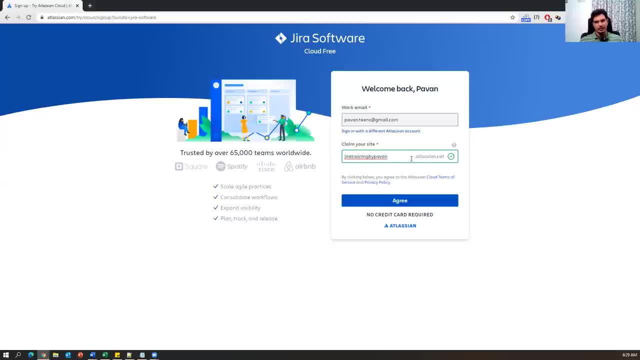 come under url: okay, zira training by power. one dot at last in dot net. so this is a complete url which you have to use later, so i say i agree. so, once you said i agree, so which will go and try to create a zira instance for you. 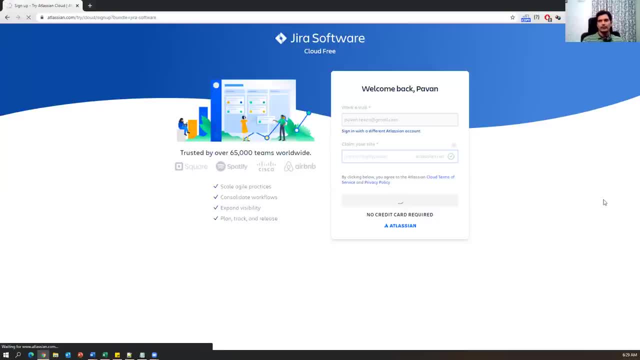 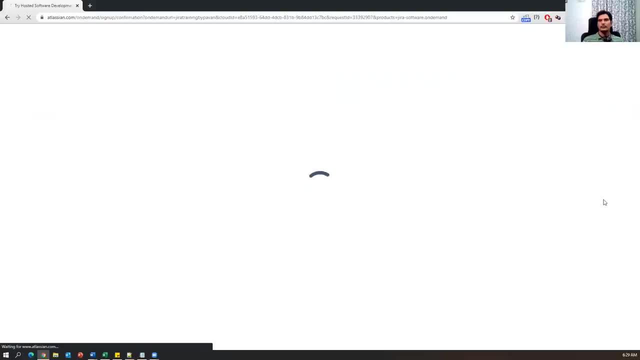 so it is trying to create. so it is right, it is still trying to create. yeah, now we can see this patala scheme. you can just select some of the options if you're required, or else you can skip the question not required and again you can skip it. so basically, they are asking: who are you? you are a founder or your? 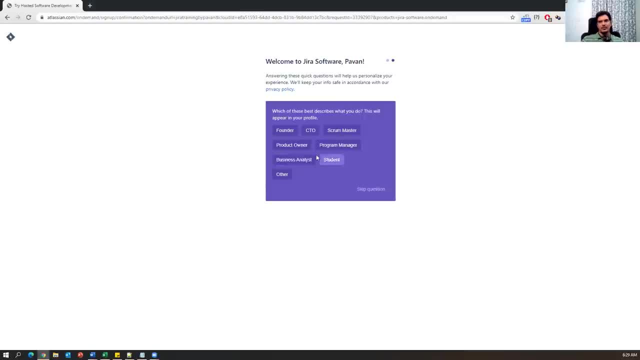 product owner, your student or your business analyst what you are exactly. so they are asking here- and you can also skip this question- not mandatory, so once you have it, it will come under the use of power and zira training. now let's see what is. Once you skip it, then it is going to create. 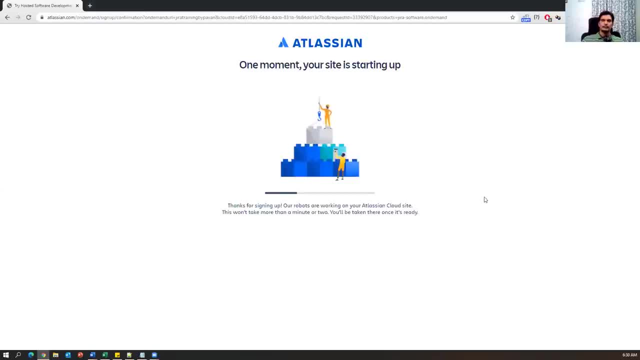 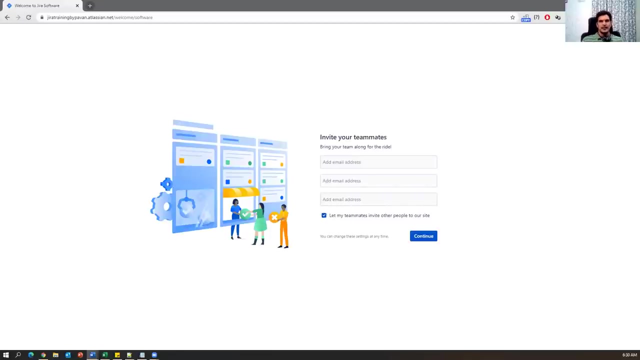 a new Jira instance. So let it complete. Okay, So now it is trying to create our Jira instance. Yeah, so now the next step will start. So when you create a Jira instance right, So multiple people in a team can access the Jira right. 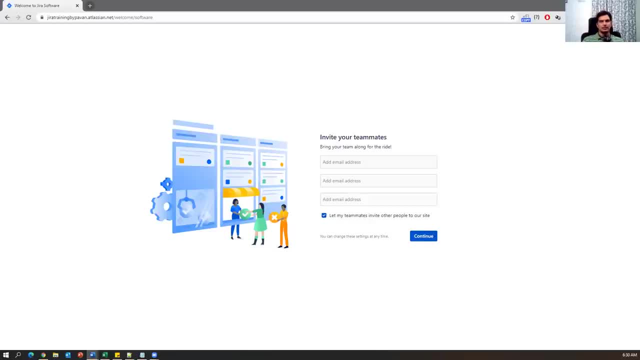 So you need to add different people in your team, like including product owner, like developers, testers, scrum master, And these people will be part of the Jira project, So they should be able to access the Jira tool. So here you can specify those email addresses. 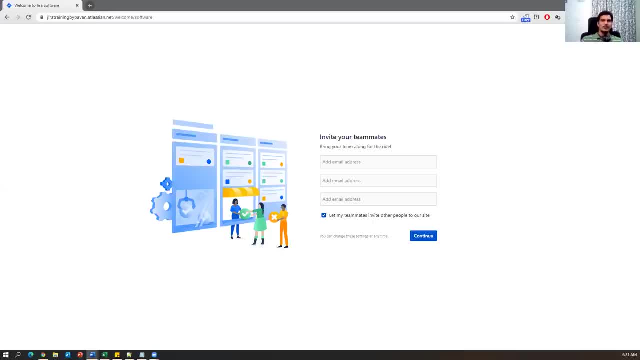 So whoever is working on your Jira, your team in that particular project, you can specify the email addresses of them. Then automatically these people will be added to the Jira project. Okay, so we can do this step later also, So once you created the project. 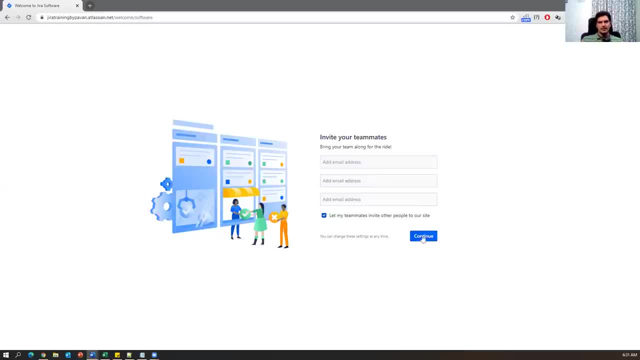 then I will add the people to that project. So for now you can just skip it. I say continue, Okay. so once you continue, it is asking like: help us set up your Jira. So what exactly it is I am, You can select. I am new to Jira or I'm experienced with 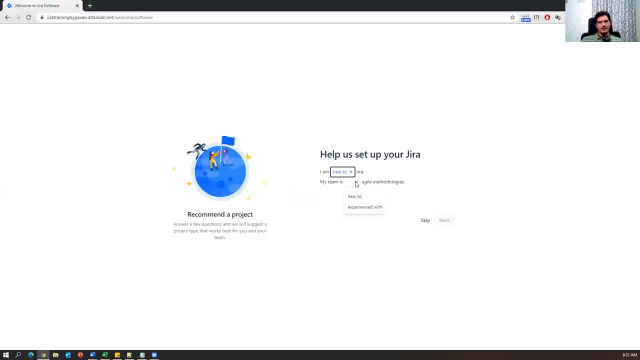 So you can just select. I'm new to Jira and my team is here. You can just select the second box- My team is also new to agile methodologies- or my team is also experienced with agile methodology. You can select one of this option. 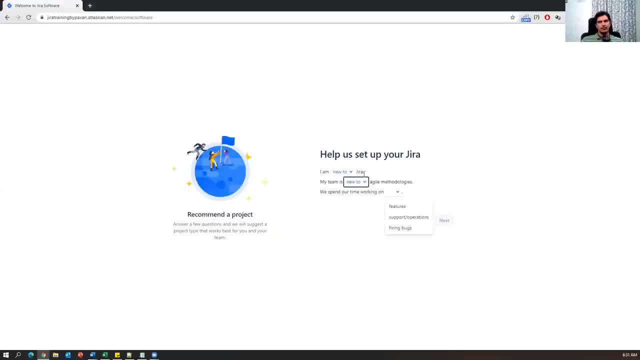 I say new to it is just like a fill in the bank case. Okay, I am new to Jira And my team is also new to agile methodologies And we spent our time working on here in the dropdown box Most of the times on what we are working features. 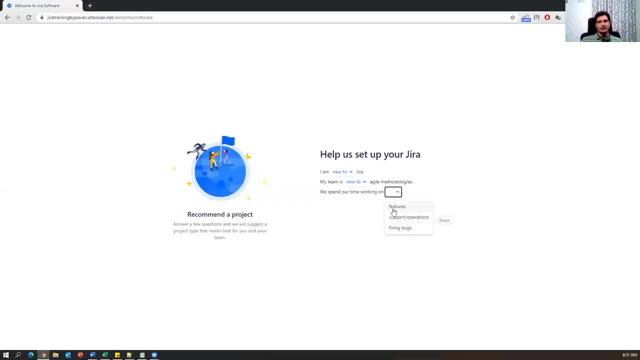 support operations and fixing bugs, anything we can select, And I'm just selecting the features, or these are all. things are optional, guys. Okay, not manually required. I just say, skip it here. Okay, now we will see something called three options. 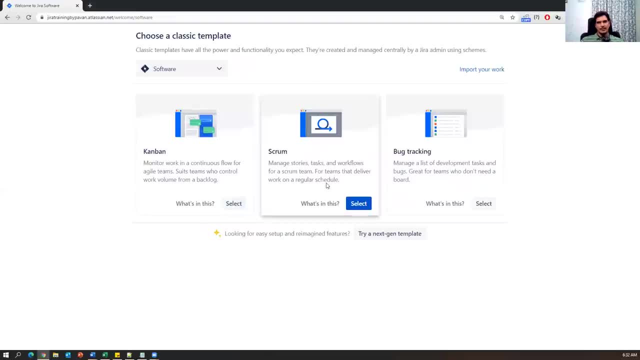 You can just look at here: Okay, this is Kanban project, Scrum project, bug tracking project. So three different paths we have. So we will work on Scrum project. So which will manage the stories, tasks, workflows for Scrum team? 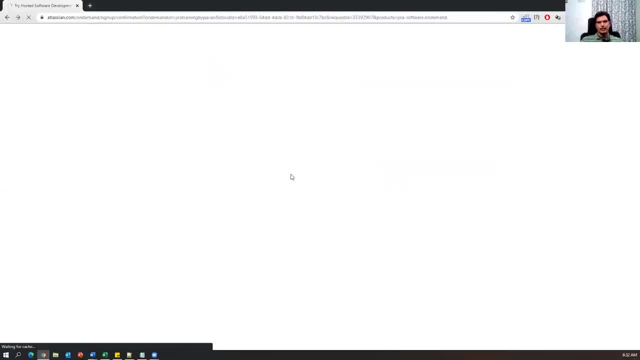 So for teams. sorry, Just go back again. Okay, so we need to select the middle project. So there are three options. it is provided, So we have to select the middle one. So again, I'm skipping it. Okay, so if you have a team, 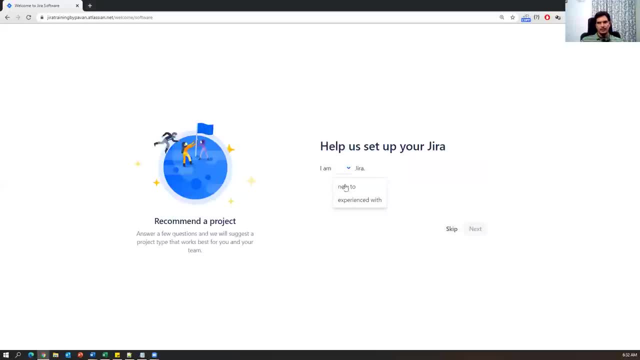 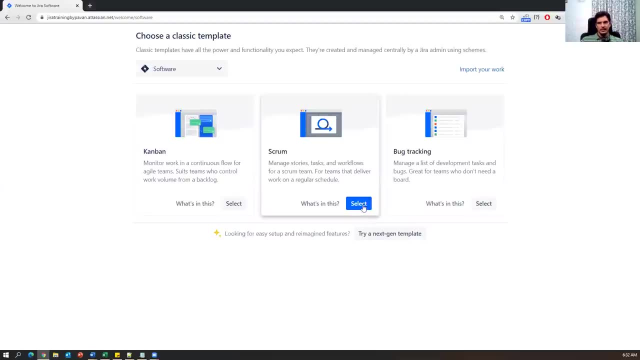 you have to provide the email addresses or else you can just skip it And you don't need to select this option. just skip it Now. this is a project which you have to select the middle one, So click on select Now. here it is asking for project name. 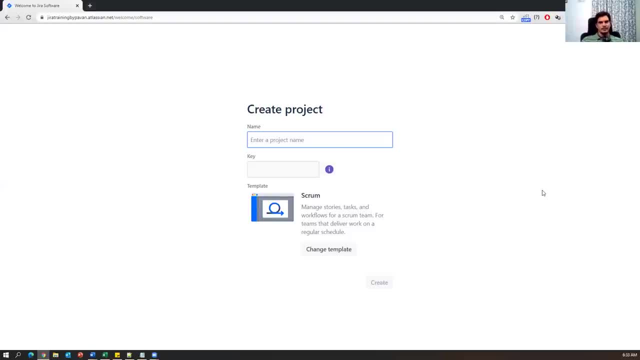 So what project we are going to do? So we have to provide the name of the project. So initially, my project name is, I'll say, open card. This is my project name. And once you specify your project name, it will automatically try to create one key. 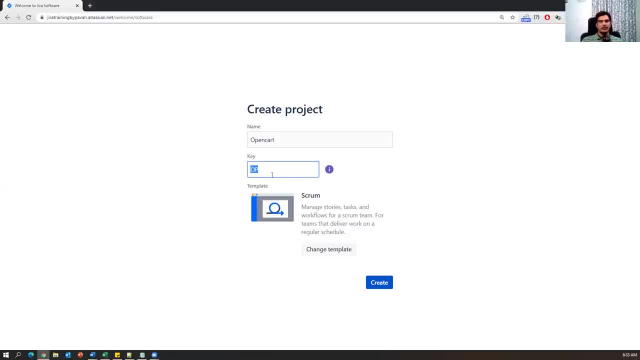 So what is key means So, whenever you create a story, or whenever you create a task, or whenever you create a bug or test case, whatever you do, whatever the object you are creating in the Jira, So you have to provide some name to that. 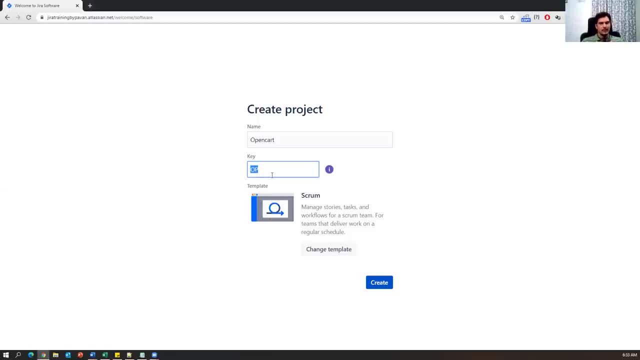 So the name is always followed by the prefix. So that is your key. So, for example, when I create a new story and the story contains some ID- let's say 001, and which will automatically add this key, let's say OP underscore 001.. 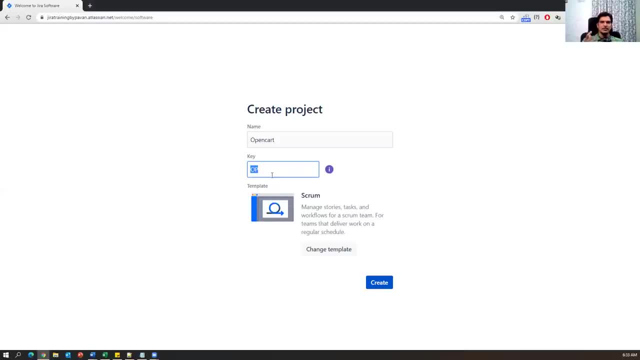 Okay. similarly, if you add some task, so task ID will be there. let's: 002 is my task ID, So the task ID will be created by using this key. Let's say: OP underscore your task ID number. So whatever object we created in the Agile process. 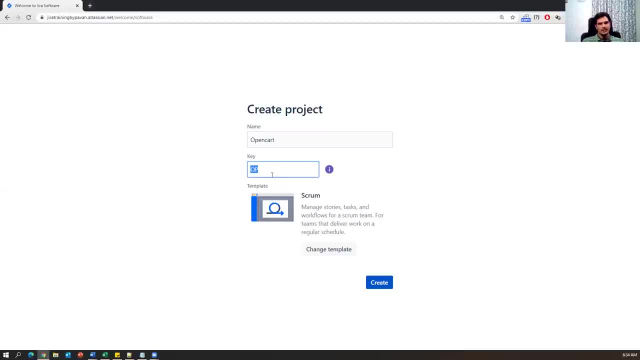 like. it can be story, it can be APIC, or it can be a bug, or it can be task. whatever you created, everything is called as an object in the Jira tool And these objects names will be starting with key. 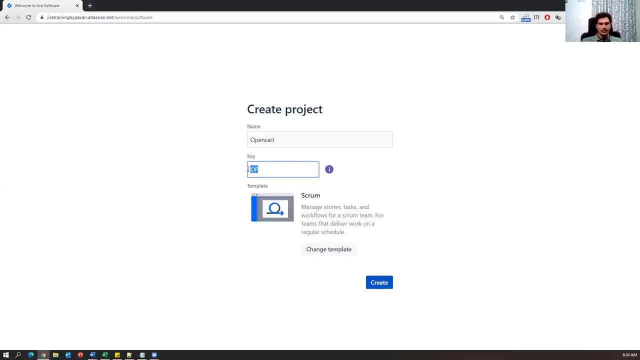 So that key we have to specify here. So by default it will suggest one key here and you can change it. Let's say, as a open card I say OC. I'm just saying OC. You can change it. This is called key and this is the name of my project. 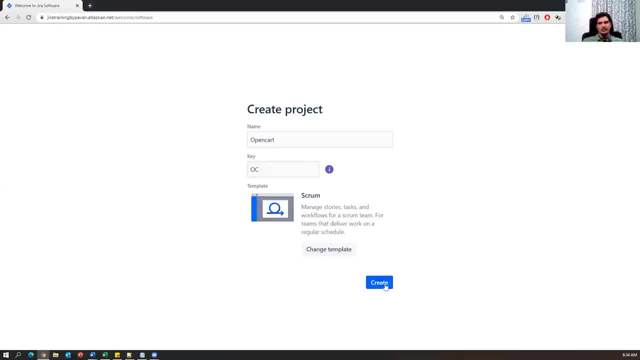 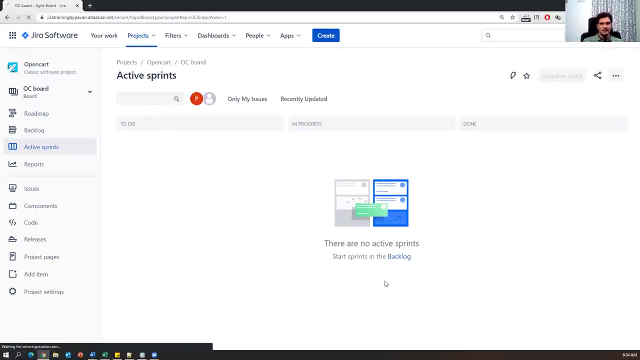 And then I say create directly, can click on the create And once you have done this, which will automatically create a new project in Jira tool. So now we can see this is the homepage of your Jira tool. So now the Jira instance is created for you. 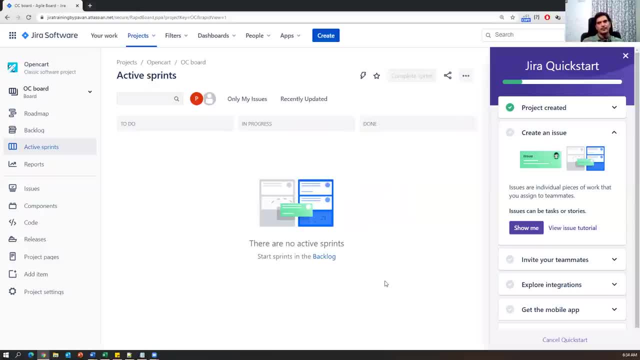 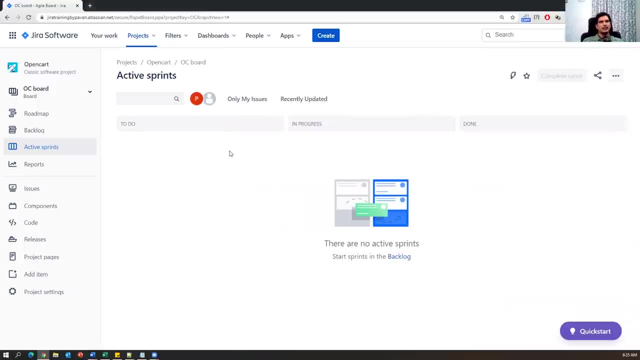 And this instance is managed with your Gmail ID for 30 days and you can add into this particular project. So now we can just click on this Jira quick start and everything. we don't need this. So now this is the first user interface of your Jira tool. 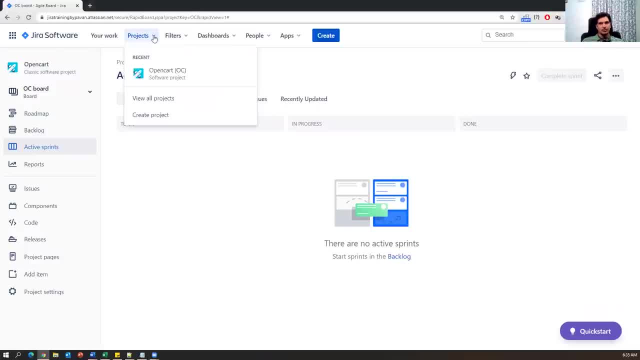 And you can find a lot of things here- your work projects. If I just go to the projects, your project name by default it will show you, And if you have a multiple projects, all the projects will show you in this list. 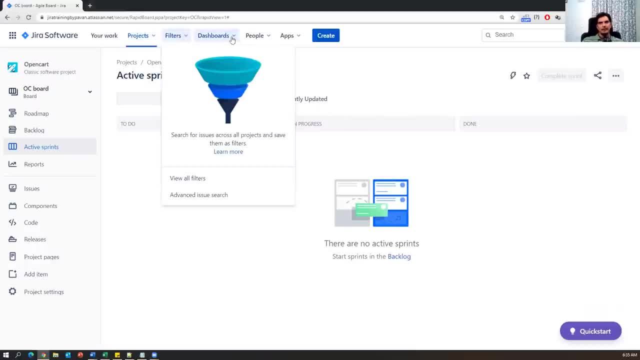 You can select which your project currently are working and filters dashboards. If I just go to the dashboard, I can see this. This is the dashboard which will show you all your activities in the dashboard And people here you can see the. 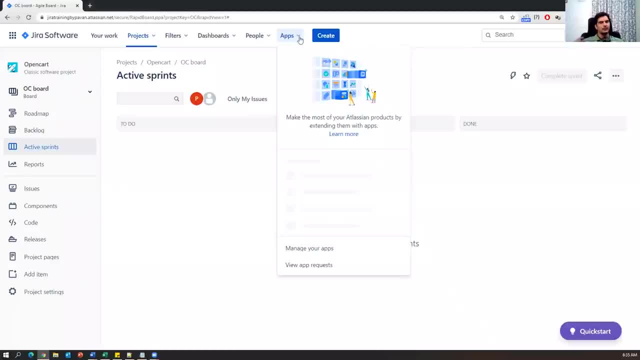 all the team members. information and apps means here. If you want to add any additional plugins into Jira, like a Jafar plugin, you can add it through apps menu. So there are multiple things that are available here And also this side you can see here. 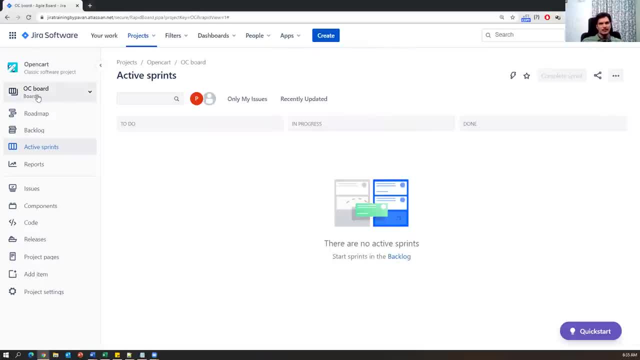 this is my project name and this is a board or a scrum board. we can say A roadmap, backlog, active sprints, reports, issues, components. A lot of things are there We will discuss later. Okay, So this is a UI, the front UI. 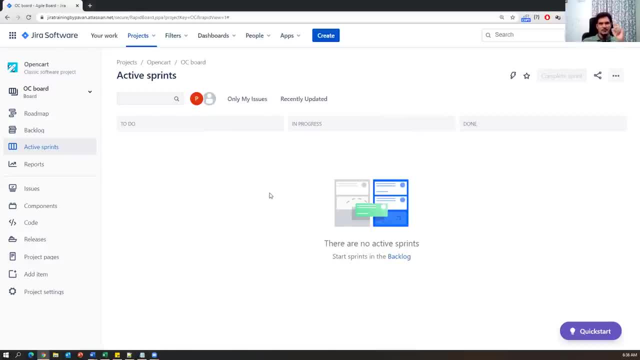 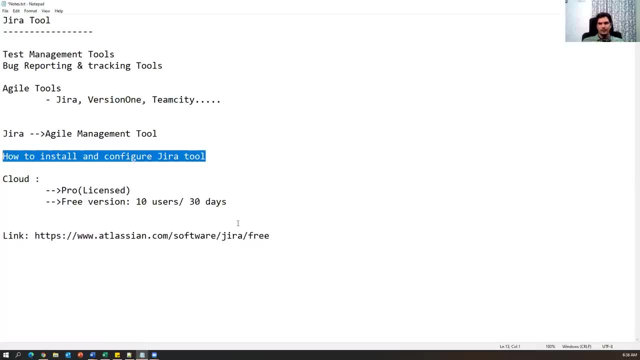 the first UI of your Jira application. Okay, So this is the way we need to configure, install Jira tool. Okay, So I will also provide the screenshot step-by-step. You guys can also follow that, because I already captured the screenshot for this. 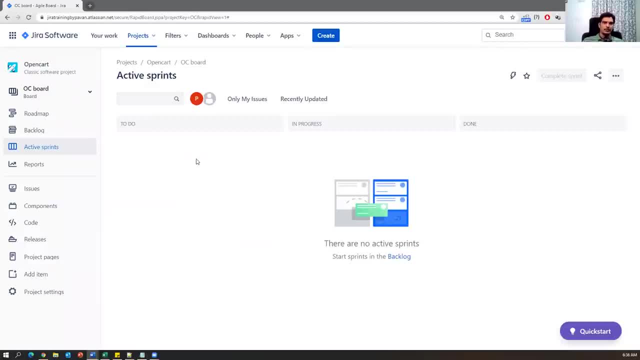 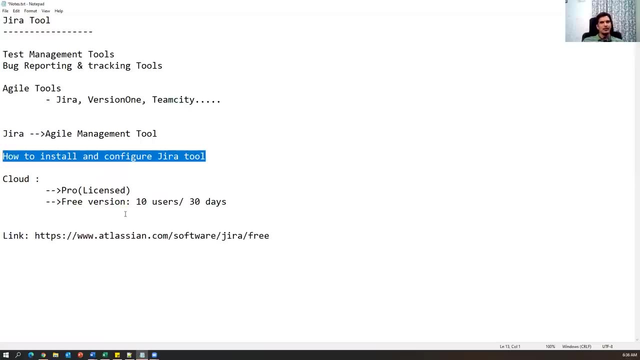 Okay, All right. So now we have successfully configured the cloud instance of Jira tool. We have successfully configured cloud instance of Jira tool. We have not downloaded, we have not installed anything. We have just configured the cloud instance of Jira tool. 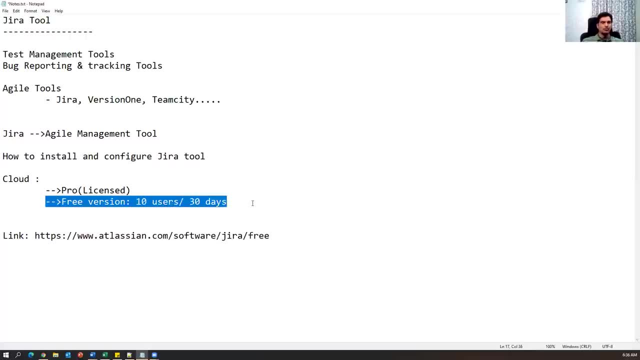 Free version: 10 users, 30 days. Okay, So now we can work with this tool. 30 days You can practice it, So everybody can create their own instances of cloud. Okay, So after that? so we have to know the workflow. 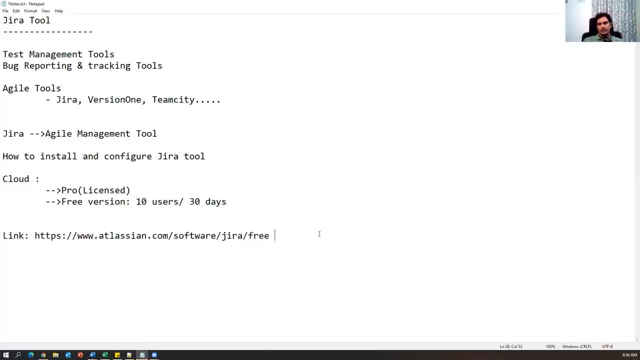 So what exactly we can do in the Jira tool. So we have to know the workflow. So what exactly we can do in the Jira tool. So what exactly we can do in the Jira tool. so in the previous session we have discussed about what are the exactly scrum activities. right, the 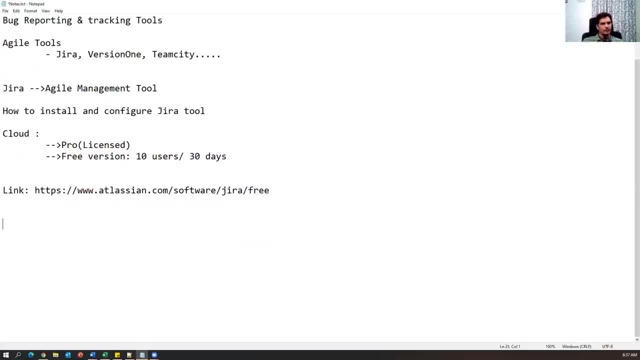 same activities we are going to perform in the jira tool. so what are those activities? so what are the agile or scrum activities we do? so let me just list out here one by one. we will try to do it. so we already installed and configured jira tool. so now we are in the home. 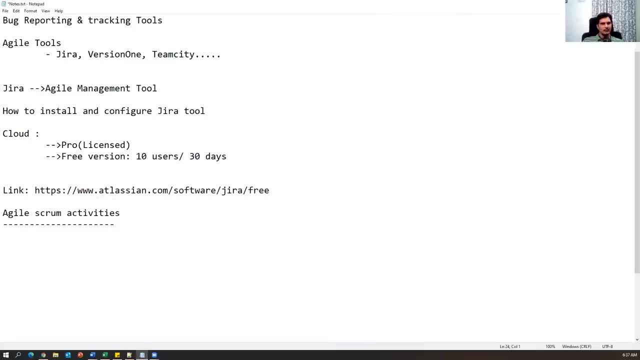 page. we are ready to do all the activities. so the first and most activity is creating the project. okay, so creating the project, how to create a project in jira? so at the time of creating the instance itself, we have provided the project name right. so that's the reason, by default, you. 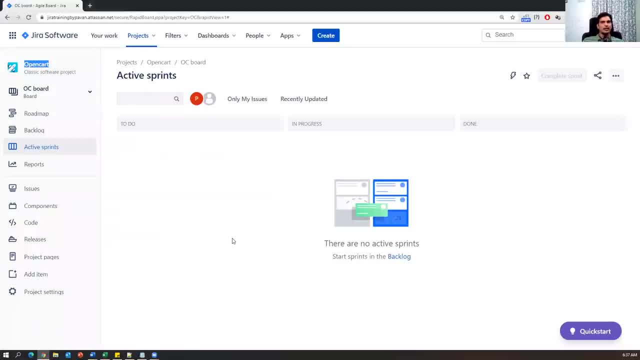 can see your project here. suppose tomorrow, if i want to create a new project in the jira, then you can just go to projects menu and you can select this option. you can just select the create project and again you have to select what type of project you want to select. suppose here: 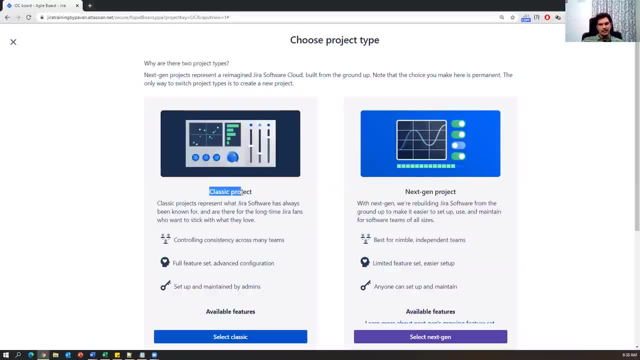 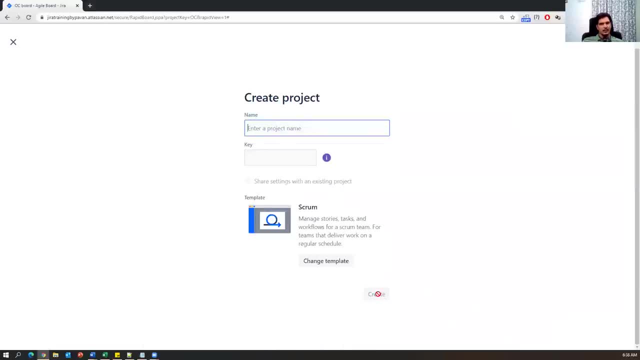 classic project or next generation project and say classic project and then click on select classic. then again it will ask you the project name, it will generate the key and then create. so this particular flow we can use to create a new projects. for now i'm just closing this because 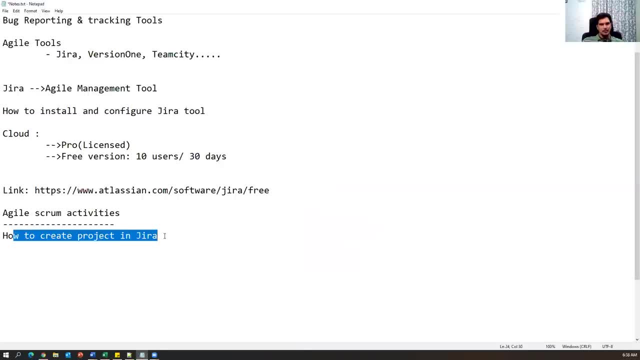 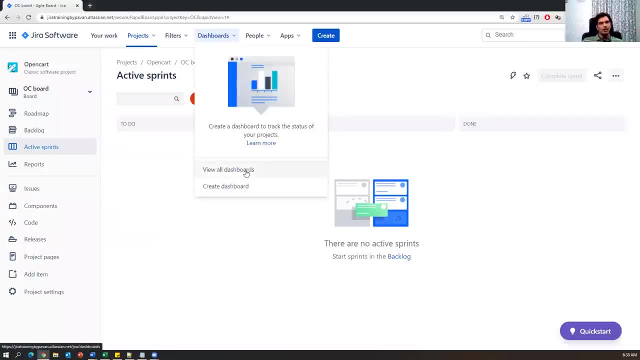 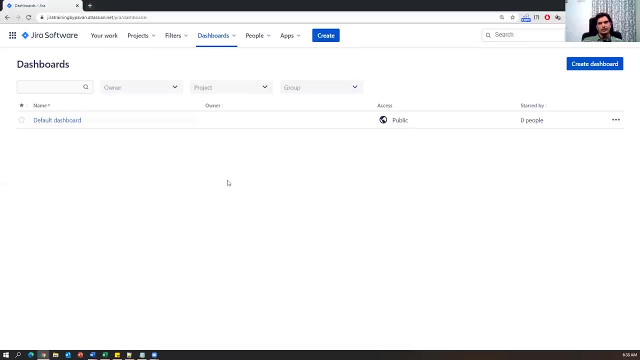 we already have a project that is a project creation- how to create a project in jira- and there is something called dashboard here. if i just go to the dashboards, view all dashboards and then you can see all the different projects we have and who is the owner, access level, how many. 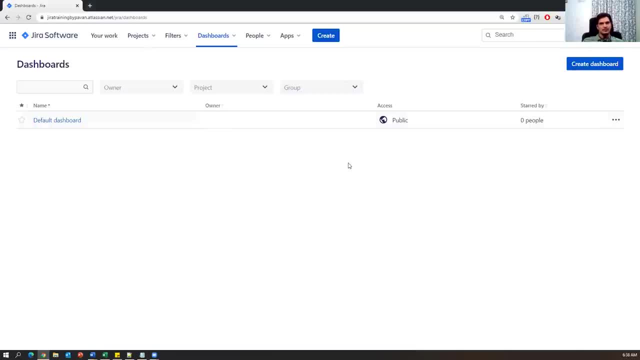 people are working on that project. all the information will be shown in the dashboards. so once we created everything, it will show you here. these are the dashboards. most of the time, management people will look at these particular dashboards to know the status of the projects. 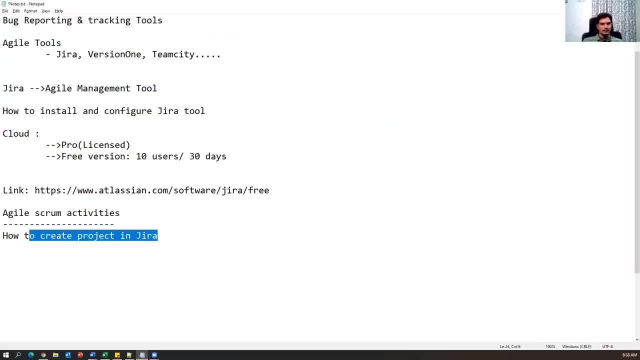 okay, and then how to create a project we have seen. and then the first and main activity is their team works on the jira right. so team means what? scrum master, product owner, developers, tester, so all the team members should be part of this project. so the first and most important, 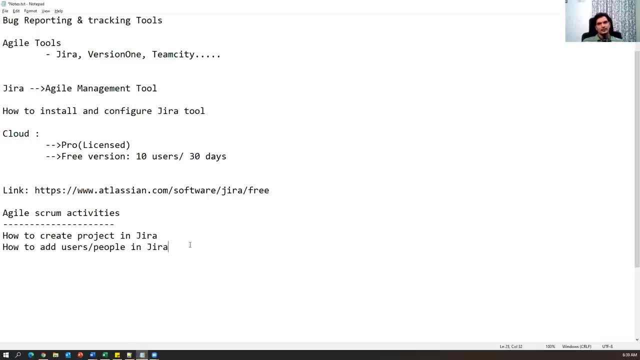 activity is: let us see how we can add users or people to the project, or in jira: okay, there's a next activity. so first we have seen how to create a new project and second thing is we need to add a certain number of people to that particular project. 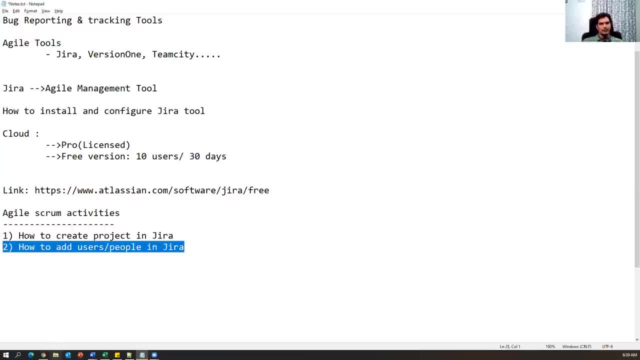 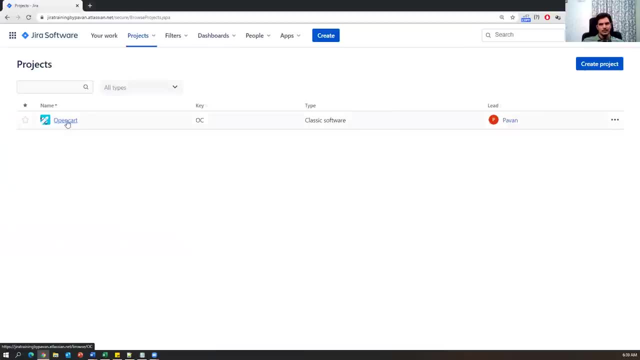 okay, so now i'll show you how we can add users or peoples into jira project. so if i just click on here- again jira software- we will go to home page, or this is my project name, so you can just click on this, which will go to home page. so now we are in the home page of jira software. so how to create? 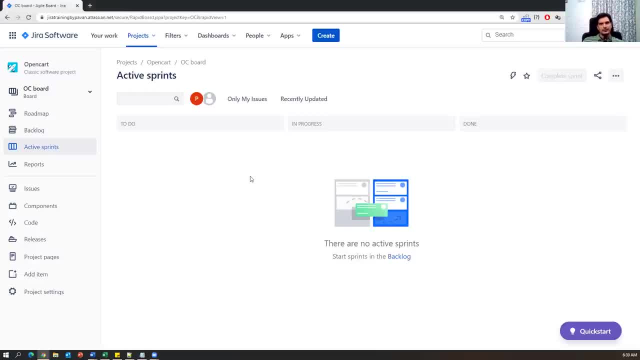 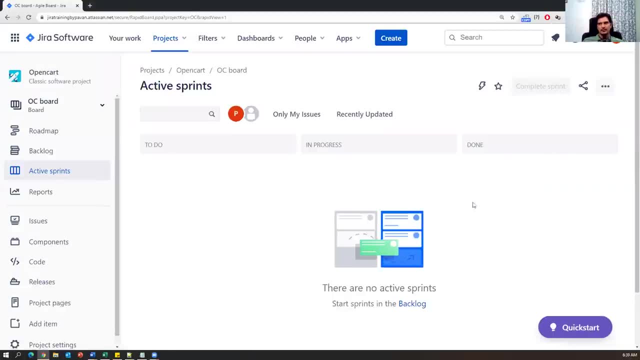 a users or people in jira. so create users for this project. what you can do is we have to go to the settings here. you can just look at here- let me increase the size also. you can just look at a small gear icon: settings menu. so in the settings menu you have to just click on the settings here. 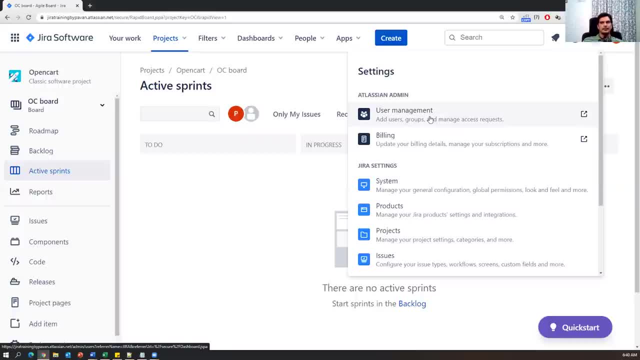 and you can find something called user management. so by using this option, what you can do is you can add users groups and manage access request. so not only adding the people. every people is having, every user is having different role, like one guy is acting as a product manager or product owner. 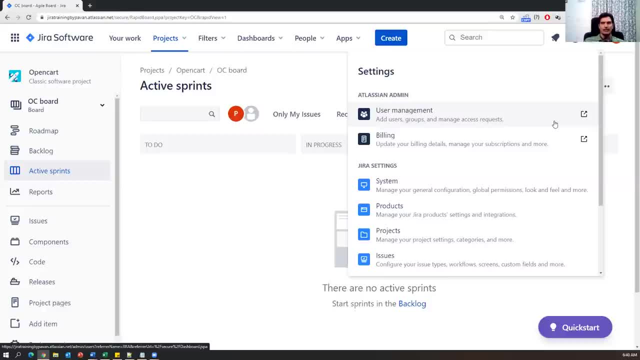 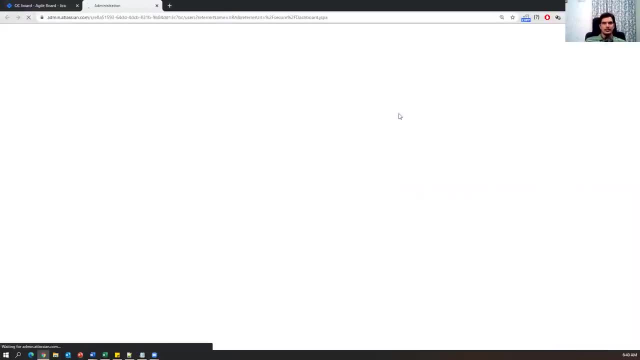 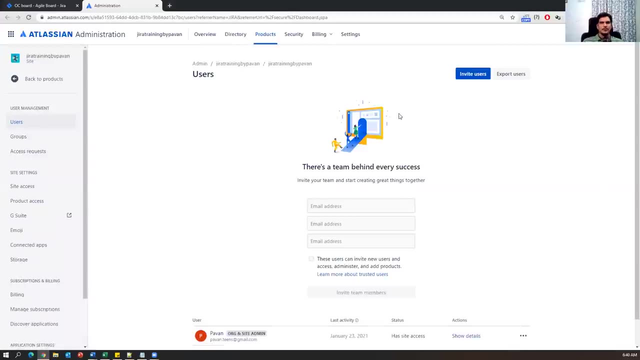 one guy is cum master, other is developers, tester- multiple roles we have. so let's go to user management, click on user management and then it will automatically open another tab, like we are entering into the administration part, and once you go to this particular screen, so here we have to add email addresses of the users. 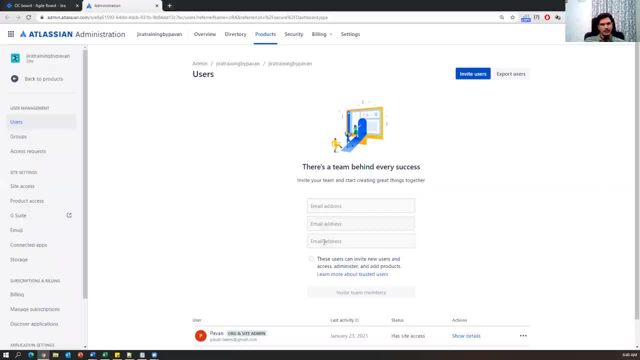 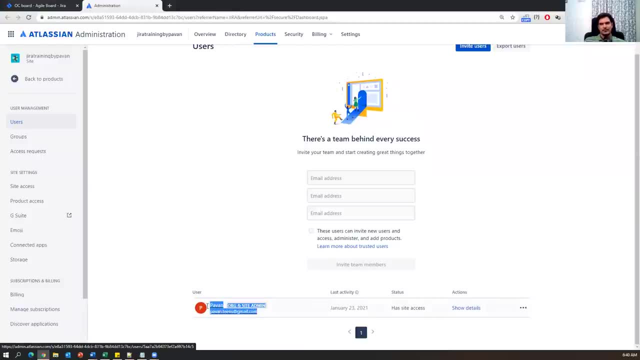 so we're all working on this particular project. we have to provide the email addresses here and currently, if i just look at here, i am only the user for this particular project. all right, so if you want to add multiple users, i can also add those users. let me go back again. 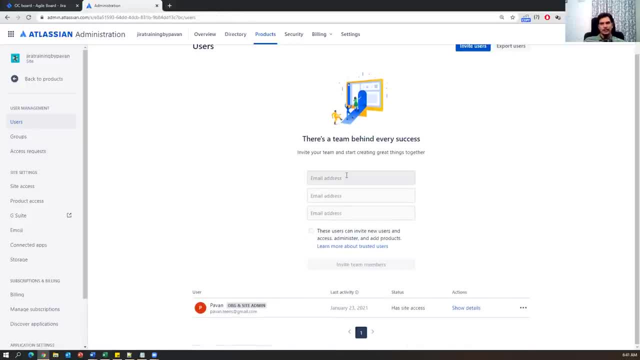 okay, so here we need to provide the email address, so your team members who are working on your team, you can just provide addresses of those email address. let's say i'm just using some dummy. i'll say abc- okay, he's a developer. i'll say dev. abc developer. i say prefix dev. 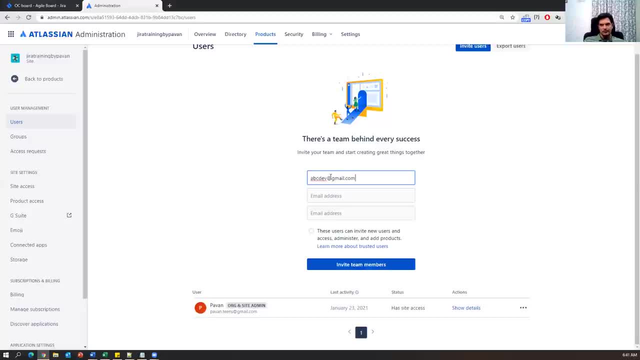 and i say some gmailcom and some. similarly, i say some xyz and he's a qa as a qa at gmailcom, and similarly i say something uh mno, so he's a product owner, i'll say pvo, so there is gmailcom. so like this, 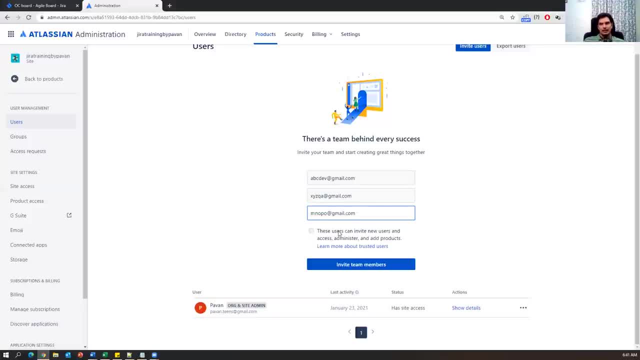 you can create multiple users to this project. okay, and if i select this checkbox, what happens is these users can invite new users and access administrator and add products and these are basically not administrator users. so i just don't want to select this checkbox and say invite team members as soon as i click on. 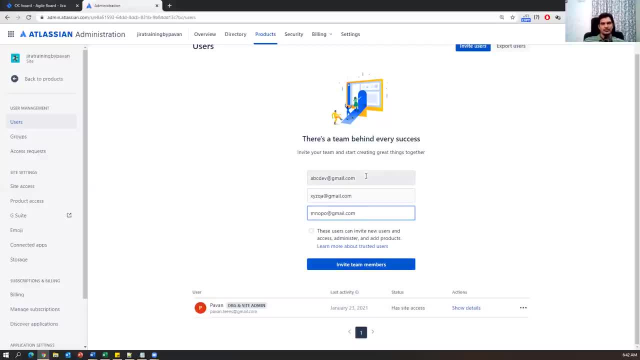 the team members, and here you can use the real gmail ids also. guys, if i add your email ids here, you will automatically invite it to this jira. you guys can use my jira tool from your location if i add your email addresses here. okay, so i can just say: invite team members and once you click, 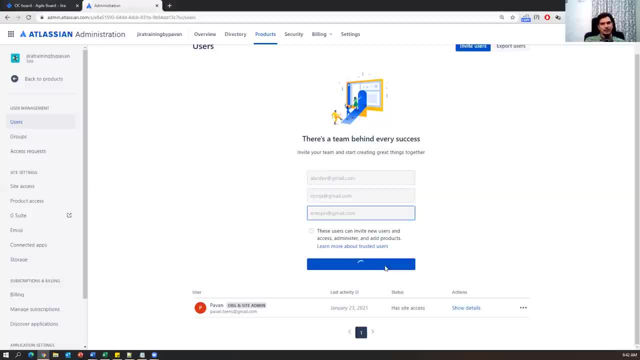 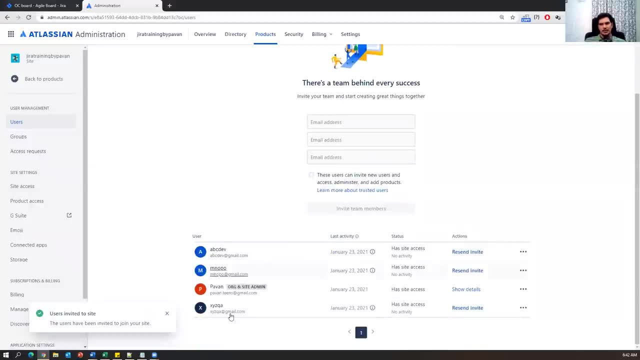 on that, automatically the people will be added to your project. who is working under your team will be added to this project. so now it is added and if i just come down here, you can just look at here. so these are the different people i have added to this particular project. okay, so this. 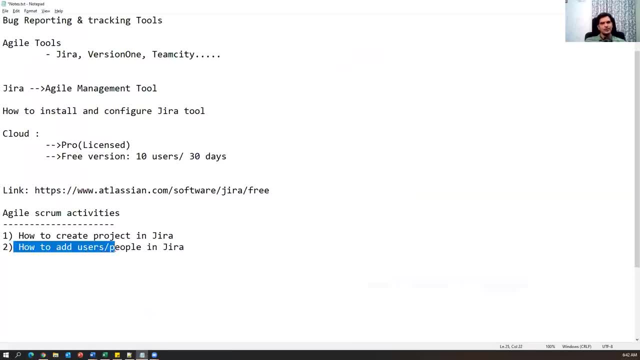 is a basically user management- how to add users or people in jira tool, right? so once we have done this, then actual workflow will start. so in the scrum, where exactly we will start. so first we need to start with the backlog, so we need to have 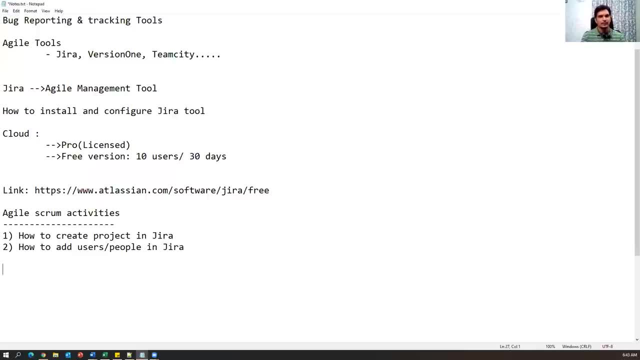 product backlog, then we will have stories in the backlog. we have to create epics and first we need to have a backlog, right? so in the backlog, what you will have, we will have epics, or each epic is having multiple stories. okay, each epic is having stories and once. 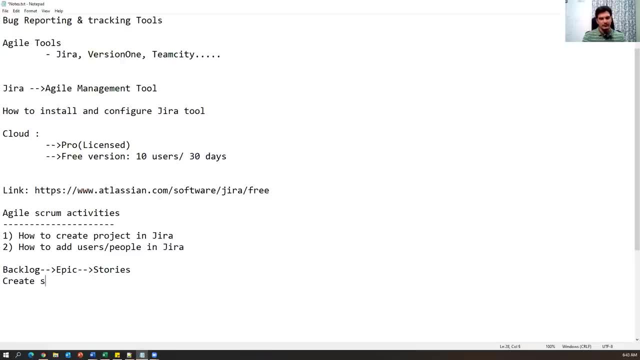 we have done this, then we have to create a sprint. we have to create a sprint, and then we need to add stories to the sprint. we have to add stories to the sprint and then we have to start sprint. we have to start the sprint and, at the same time, once you start a sprint, 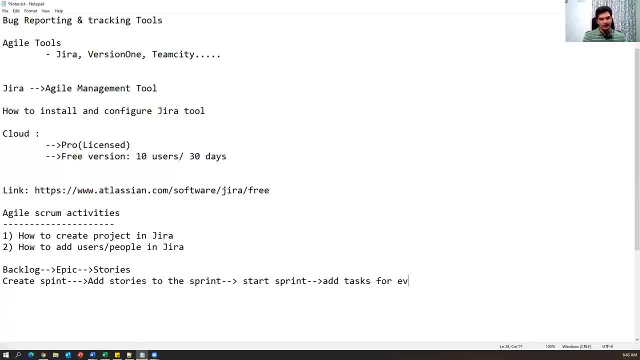 we need to add tasks. tasks for every story, right? so these are the workflow step-by-step activity. so first we will see this. first we need to have a backlog. then backlog contains what? so we will create the backlog. product owner will create the backlog by taking the requirement. 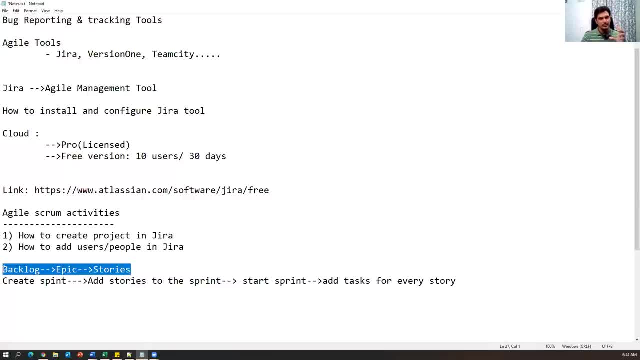 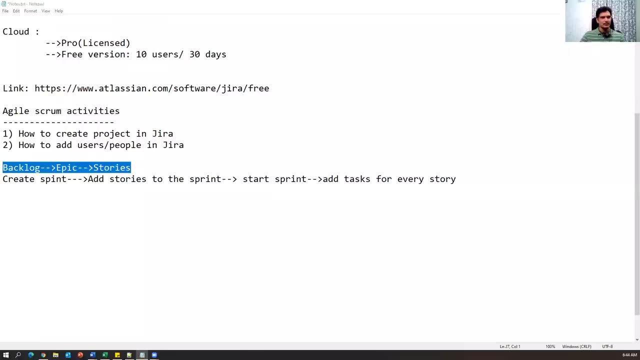 from the customer, right? so first we need to have a backlog for the project. then the backlog contains epic- one or more number of epics, then the epic contains the stories, right? so let us try to create this first. so let's go step by step. so first we will try to create. 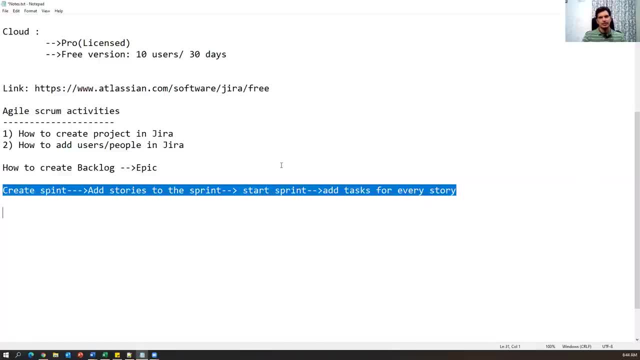 a backlog and epic. then i'll come back to the stories. how to create a backlog inside the. we will have a epic. inside the epic, we will create the stories now here, uh, yesterday, i have shown you one small document, guys so, which contains all the epic stories and everything right. so let me just 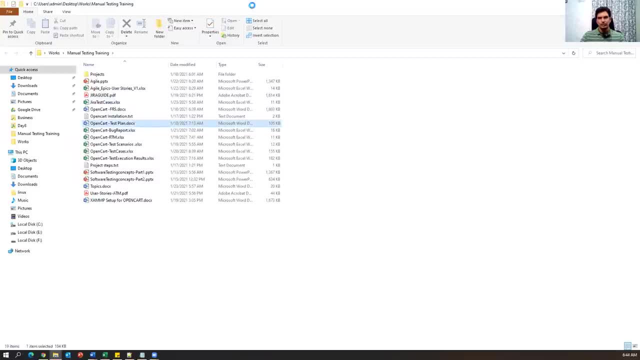 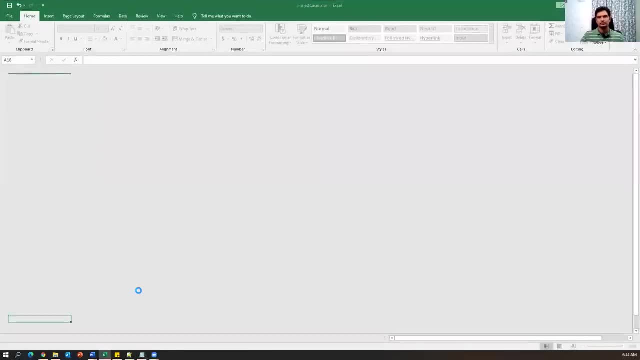 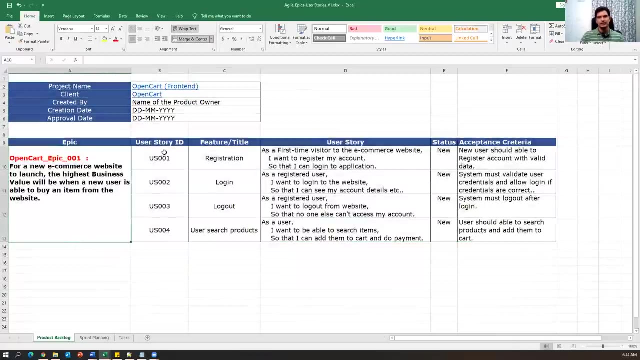 open the document. so let me just open the document. yeah, all right. so here this is my product backlogs. so yesterday class we have seen this, so this is my epic. uh, epic contains a multiple stories, so these are the stories and these are the titles of our feature names and this acceptance criteria. 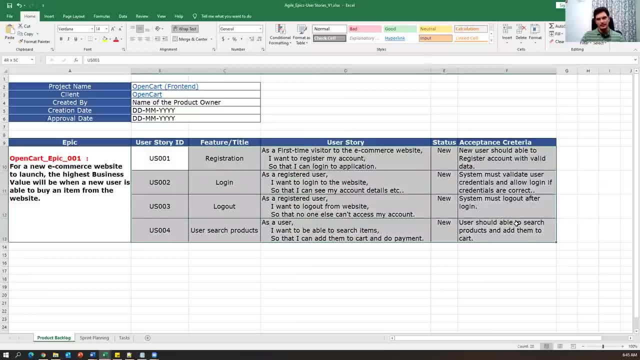 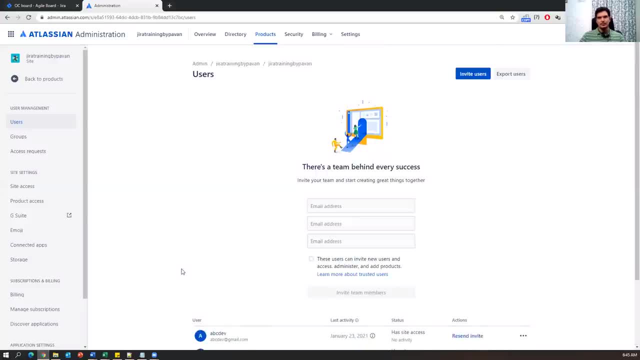 so let us try to create epic and corresponding stories in jira tool. okay, right, so now let's go to jira tool. and here, if i just go to your project now, i can just close this and this is our project home page, right? so if i just go here, 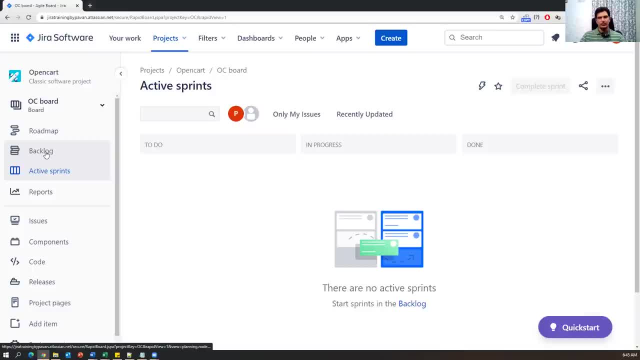 there is small thing called backlog here you can just look at here. this is my backlog. okay, so if i just go to the backlog, click on this backlog, right, so we can just look at. uh, two options here: versions and epics. versions and epics backlog. we no need to create separately. 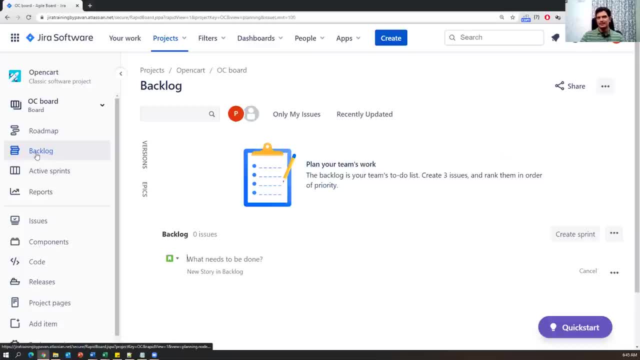 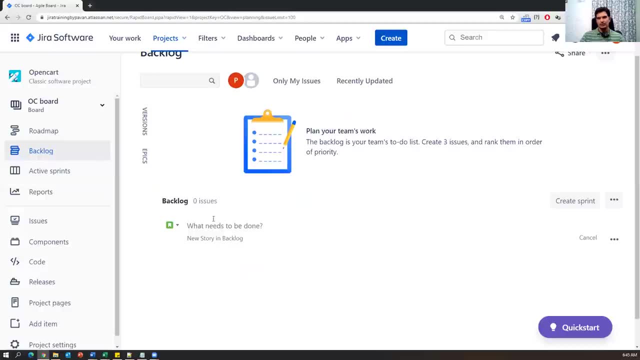 which is already there inside the project. okay, so inside the backlogs. we have two options here: versions and epics. there is no, uh, there are no stories or backlogs so far we created. this is completely empty. now it doesn't have anything. if there is any epics or stories, which 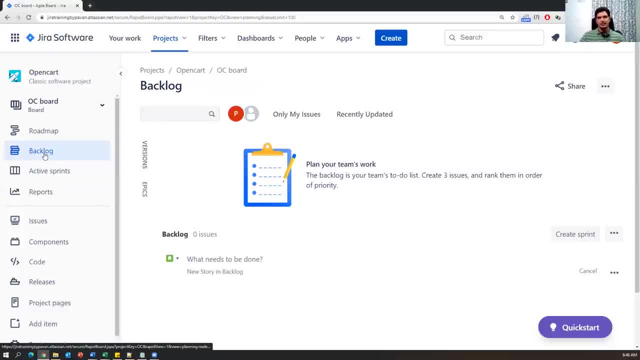 will show you here. okay, so now inside the backlog, when i click on the backlog here, which will show you this window. so here we have to create something called versions, okay, and then epics. so first let's go to versions, okay. once you click on the versions, just a moment. 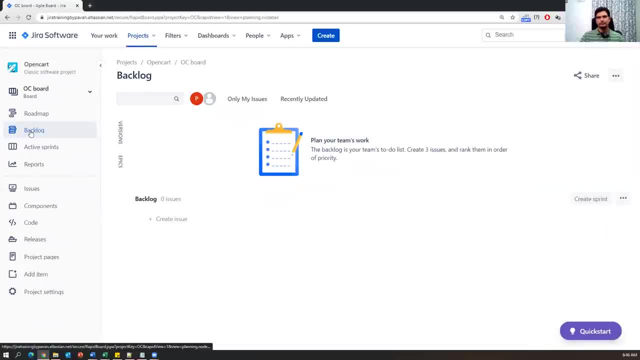 we need to create a new version. okay, so we need to create a new version. so we need to create a new version. okay, so show with a versions panel. use versions to keep track and code release. just a moment, as soon as i when i click on that option. 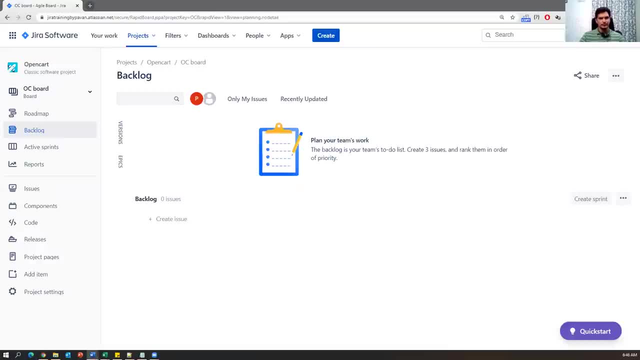 which will show you: uh, we need to add some versions there. let me click on once again. so sometimes it will be very, very slow guys, so we need to just keep wait for few seconds, okay, so let me click on once again seconds, and then it will automatically. uh, the menu will start. okay, so select the backlog here. 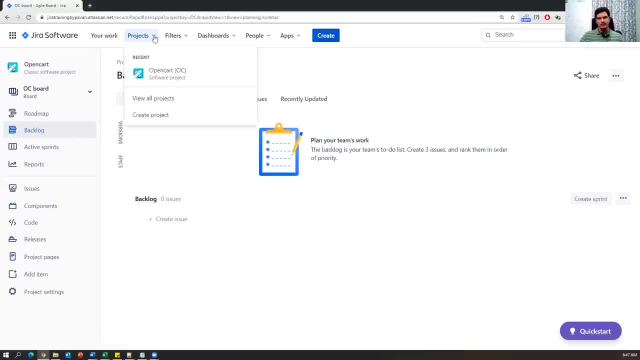 okay, and then, uh, go to projects and then select the project once again here. so select the backlog, go to projects and select the project, what you want to work on, which project you want to work, so click on project once again here. okay, and then, uh, it will show you. 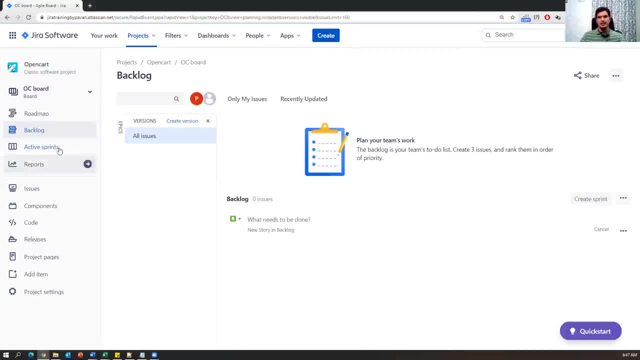 again go to backlog once again. yeah, now you can see. just select the backlog. go to projects and select whichever project you are currently working. then again come back to the backlog. then you will see these options. so under epics you will see versions and issues and one more. 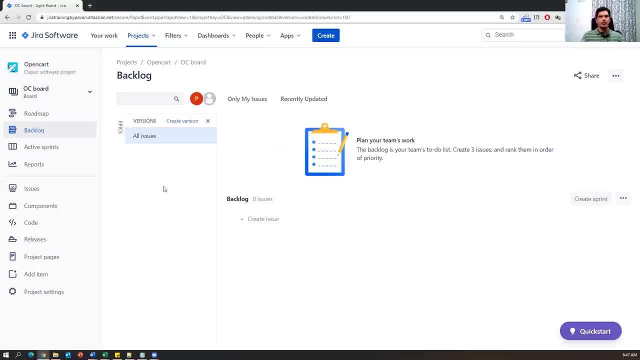 important thing in jira is in every object we call it as a issue. so don't think issue is nothing at a bug. so in jira language, in jira point of view, every object which we call as a uh issue- so for example, story is a one issue type and similarly uh bug is a an issue type. task is also. 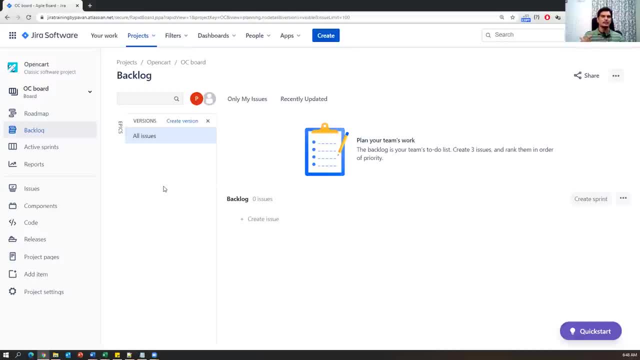 an issue type, right? similarly, a test case is also an issue type. so everything in jira, each and every object, we'll consider as one issue type. so what are the issue types, like story, task, epic? so all these things are comes under issue types in jira. okay, so now, if i just select the backlog and go to project and select your project, then automatically the the theme here will known to types because the theme is covered in the theme Is as valid as that's one thing. grabbing the documentation is tightly used in jira, so we experience things also by couriering and exploring things also to the UI environment. but today, uh, there is another issue type, so i will also try to design a- only a file. 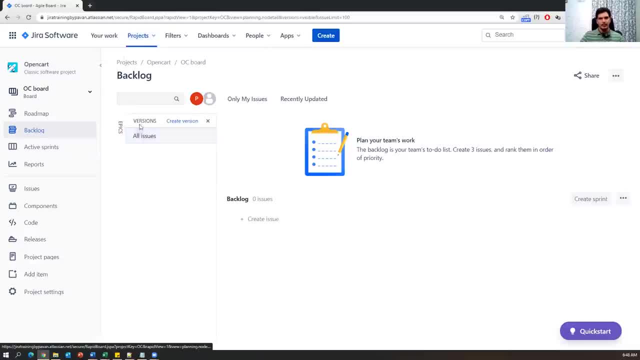 log and go to project and select your project. then automatically the backlog items will come here. so currently i don't have any epics or stories. what you have to do is first we need to create a epic. so how to create an epic? so here, select the epics and here you can see versions and 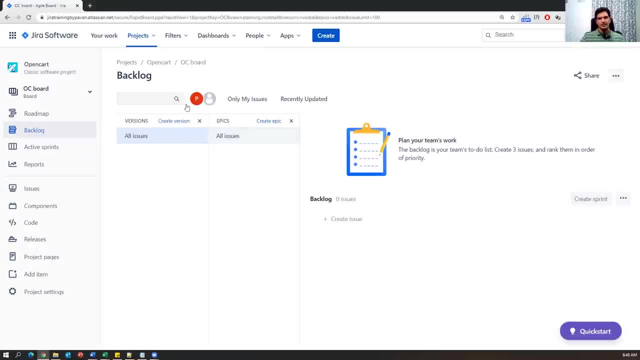 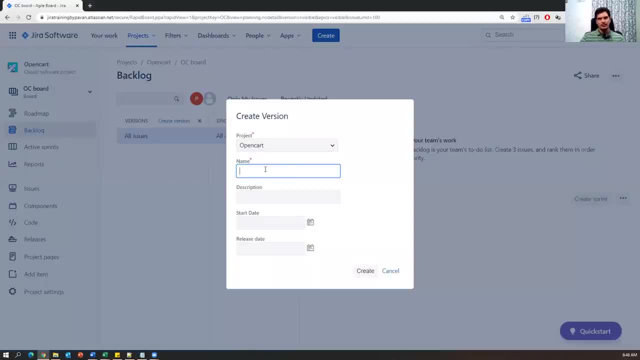 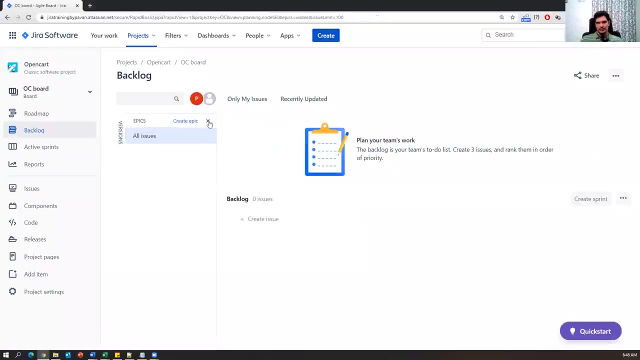 all issues. currently i don't have any versions or any epics, so first we will create a version. so click on this, create version and under this project, i'm just providing some name to the epic. okay, so just a moment, let me just close these things. first of all, so this is the initial screen. 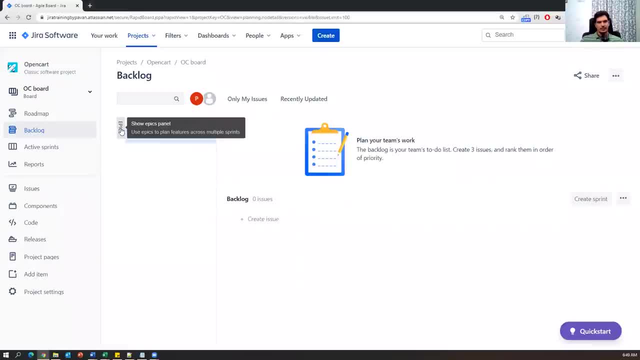 guys. okay, when i click on the versions, versions information will come. when i click on the epics, epics information also will come. so first of all let us try to add version. so i'm just clicking on the versions here and then create a version. so here i'm just giving some version name. okay, i'll. 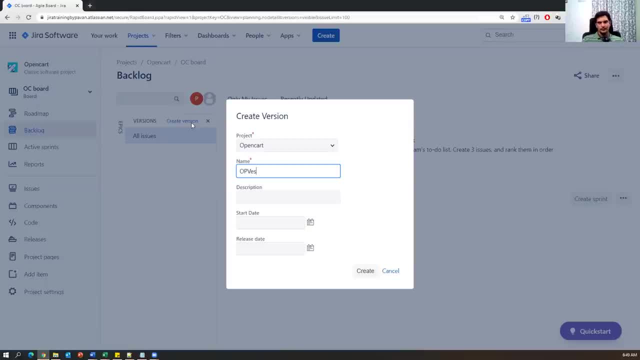 say this is open cart, open cart, open cart version 001. i'm just giving some number. i say v001, open cart, v001. if you want to write some description, you can write it, and when this project start, when the project is end, you can select the date. so today i'm starting and the whole project, uh, will end. let's say sorry. i say: 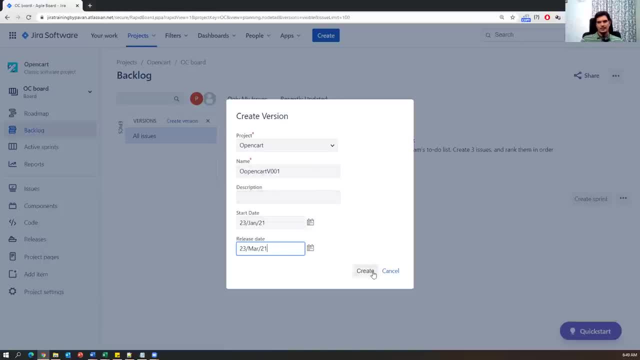 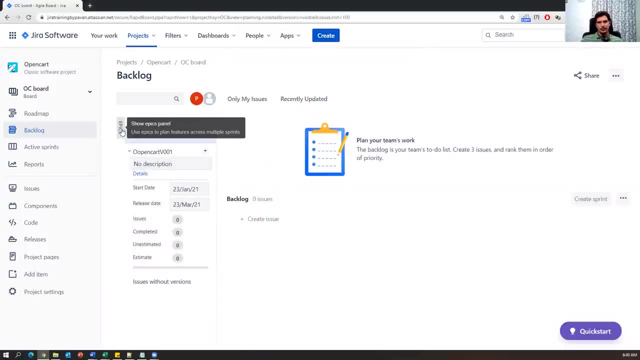 february, march 23, so two months of time. i'm not going to be able to do that. so i'm just going to give you the date of the project. and i'm just going to give you the date of the project and i'm giving and just say create. so now we can see the version is created and then we need to go to. 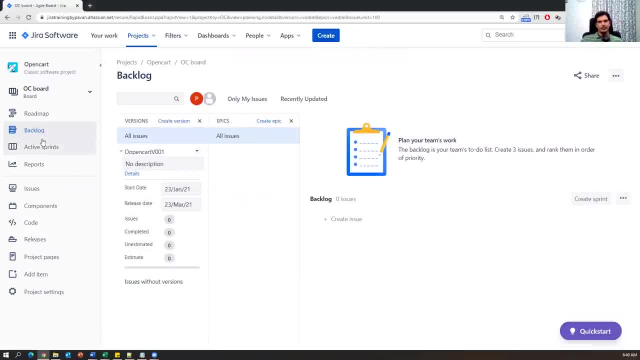 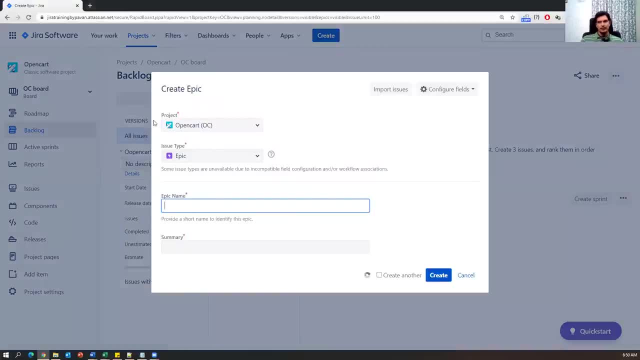 epics and now we need to add epics to this backlog. okay, now we can just see one small link here: create epic. so i'm just clicking on the create epic. now you can see. this is my project name. now here these are the issue types: task, story and bug. so these are the main three issue types. we 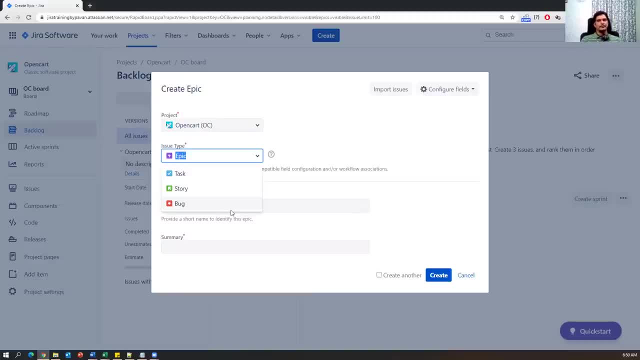 have in jira guys task story and bug. okay, so what kind of issue type we are creating now? epic, so we have to select the epic here and then here we have to provide the name of the epic and summary of the epic. so we can just look at the excel sheet. we have something called name of the epic, summary of the epic and what i 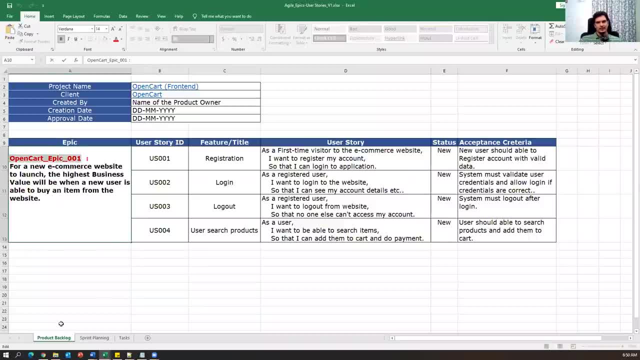 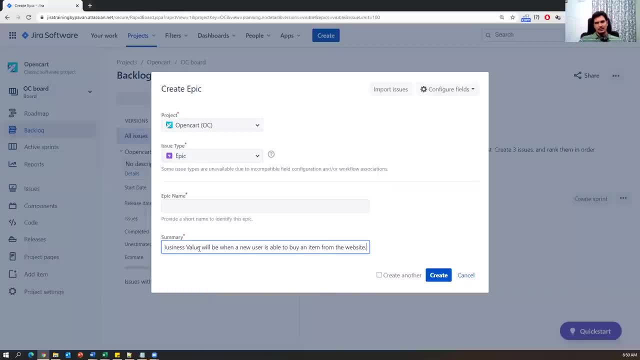 can do is you can just simply specify: uh, this is the name of the epic. oh, this is a summary actually. so let me just type summary here and provide a short name to identify the epic. so i can just give this as a name of the epic. so this: 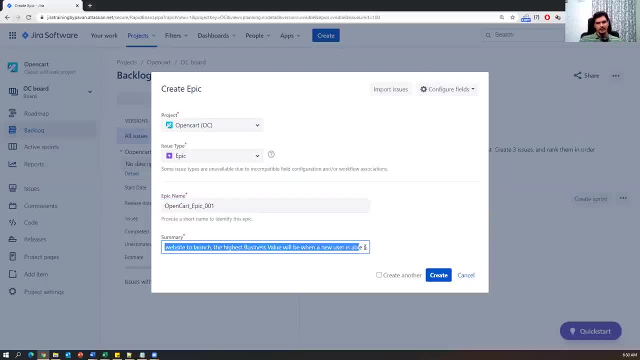 is my name of the epic and this is a small description of my epic or summary of my epic. similarly, if you want to create another epics, you can just select this check mark, automatically create another and just automatically, which will give you another screen- this epic will be created. 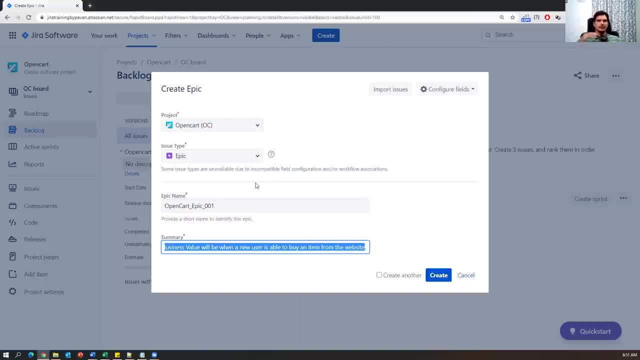 and then another epic will be created, and if you have multiple epics, you can just use this option: create another. then it will automatically give you an episode like this. of course, you can also click the another screen to add another epic. so currently i have only one epic under this epic. i'll try to. 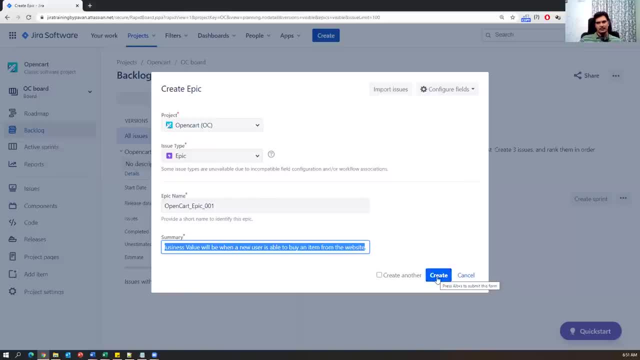 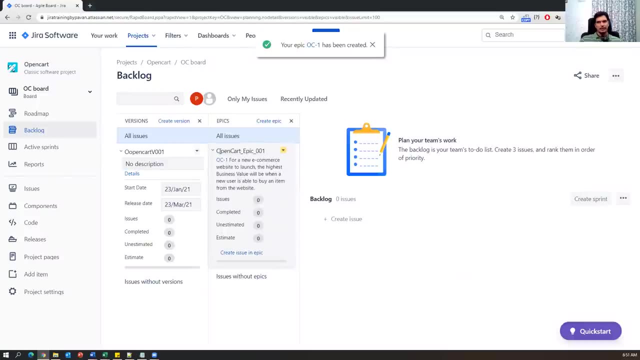 add multiple stories. so for now, i'm just saying create. so once you have done this, now you can see a new epic is created. so so far what i have done under this project, we have created one version and also we have created one epic. so opencart, underscore, epic 001. so this is a our epic and 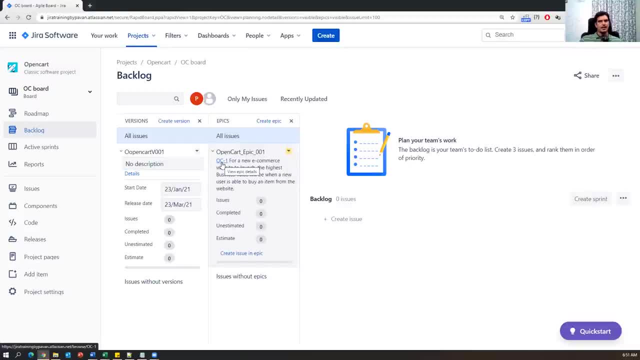 this is the automatic one. id will be created oc and iphone one. this is a epic id which is created by jira tool itself. okay, so if you want to see what are epics are available inside the backlog, just you select your project here and then go to backlog and then you can see what are epics. you 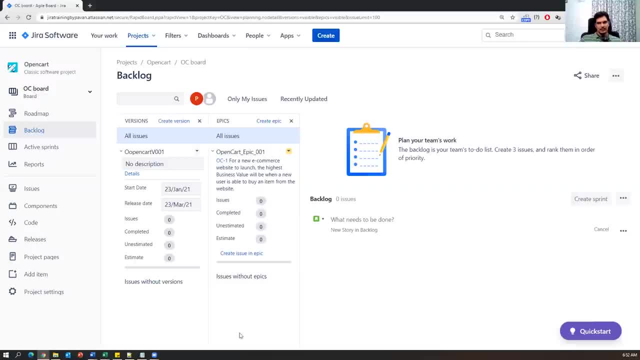 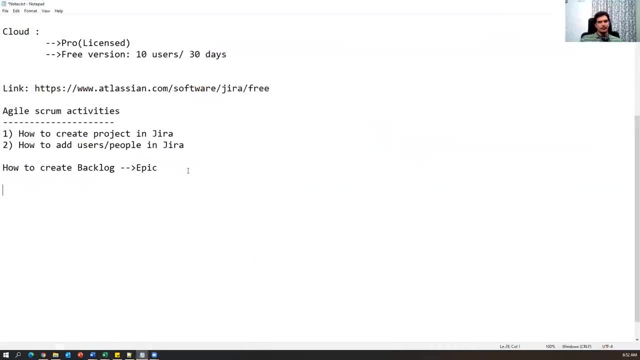 have here and if you add one more epic that will come here. below this epic, one more epic will come here. okay, so this is where we need to create an epic. so inside the backlog- and we created one epics. how to create a backlog epic we have seen. okay, so we have to select the backlog. go to projects. 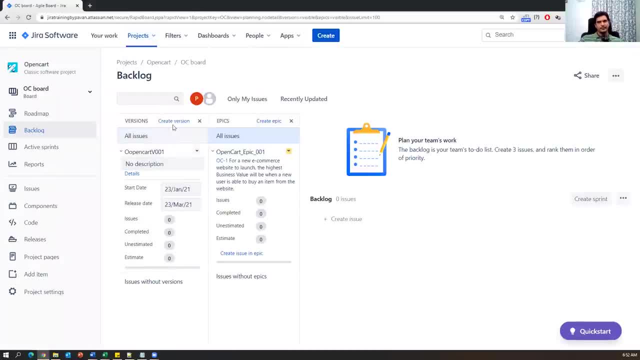 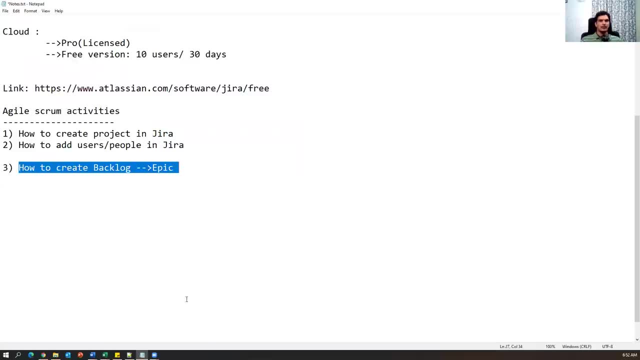 select the project automatically. these things will come. first create a version, then create an epic. so once your epic is ready, what is epic? epic is a collection of stories. so inside the epic we have to create multiple stories. so we have to create a collection of stories. so inside the epic we have 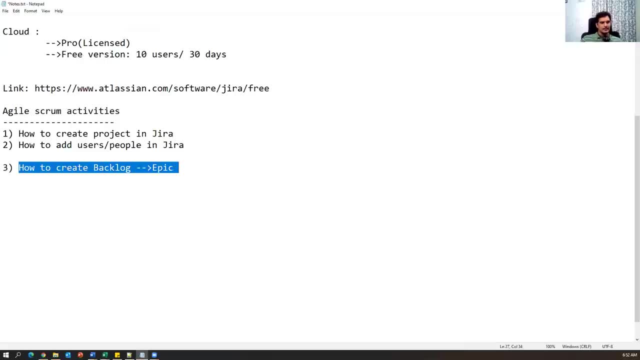 to create multiple stories, right, so that is a next activity. so once you created your backlog epic, right, so that is the next activity. so once you created your backlog epic, then we have to create. then we have to create stories in jira and then we need to add story points to them. that is a fourth. 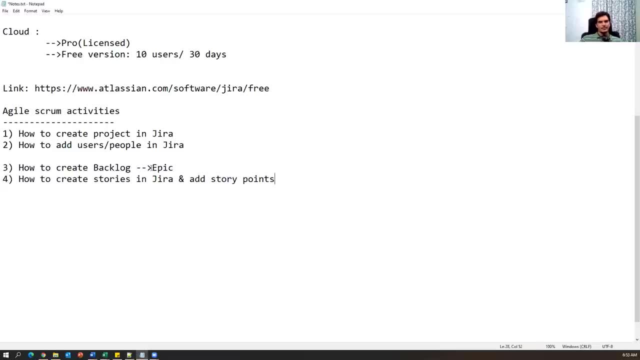 head. so once epic is ready, we have to create a stories under this epic, and for every story we need to add story points. what is story point means estimation, rough estimation, which we need to define for that particular story. so now i'll show you how each articulation look, how to easily have 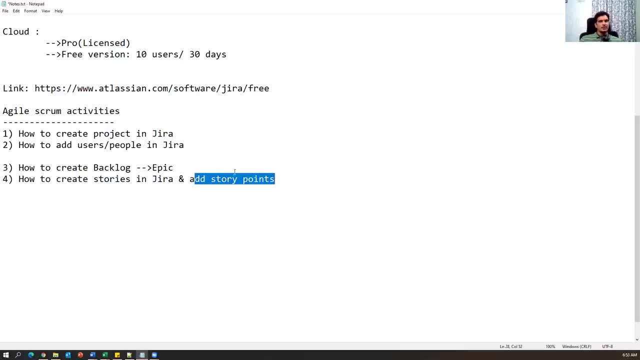 a story, so let's see there we go, so you can see these three products. what is the Hunter? these are doping. that these are the story points. well, i'm a fastest蚤 escort, so let's continue. we need toapanie and you. how to add stories to this particular epic story is a small requirement, so now i'll show you. 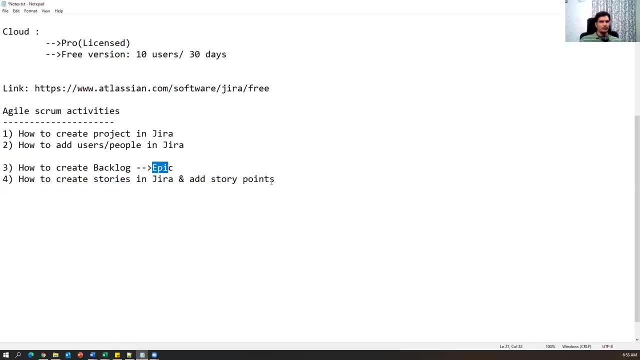 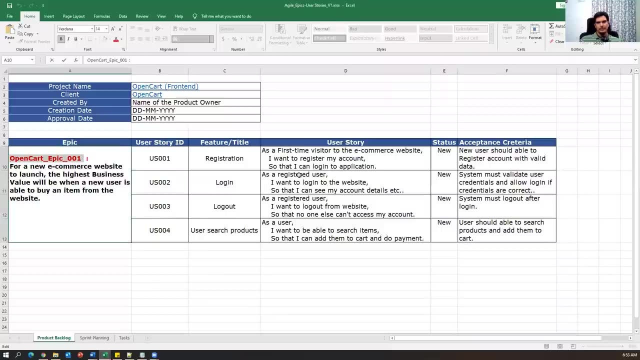 how to add the stories to this particular epic and also we will add story points to that particular story. okay, now, as per our excel file. so these are the user stories, right? so now we have to create these stories under the epic. now let us see how we can create them. so go back and now to create. 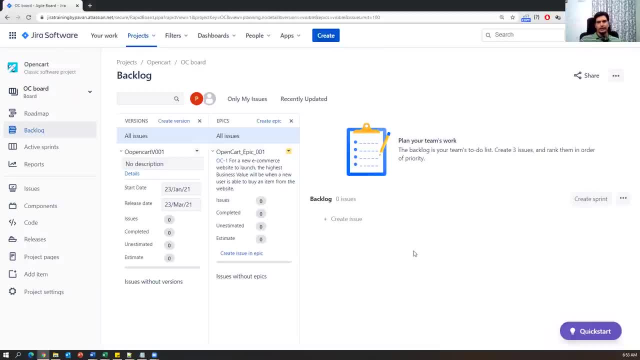 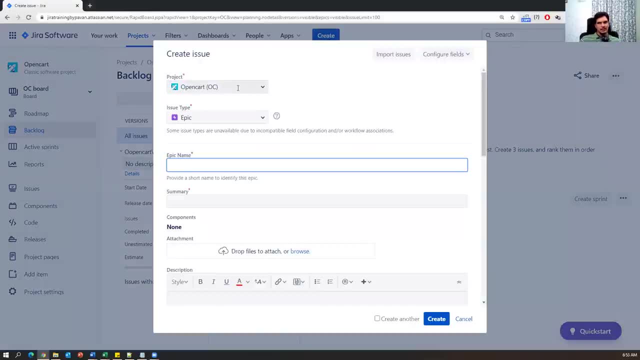 the stories under this epic. what you have to do is we have to directly go to create button here. okay, if you click on the create button, you will see the project name and under this is the epic core, which one you want to create story we have to create. so select the story, okay, and once you 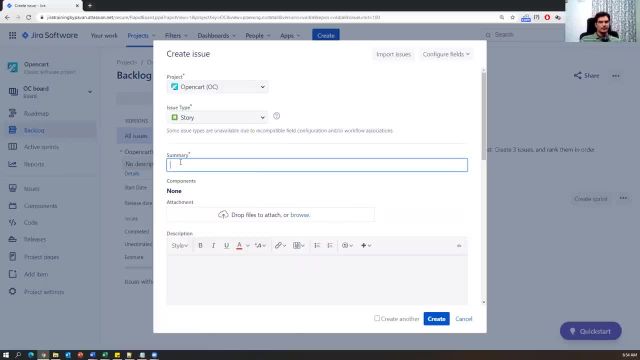 selected this story. here we have to provide the summary of the story. here we have to provide the summary of the story. okay, so how to provide the summary of the story is just: we need to copy from the excel sheet. so let me just copy here. and this is a summary. you can say feature or title, we can. 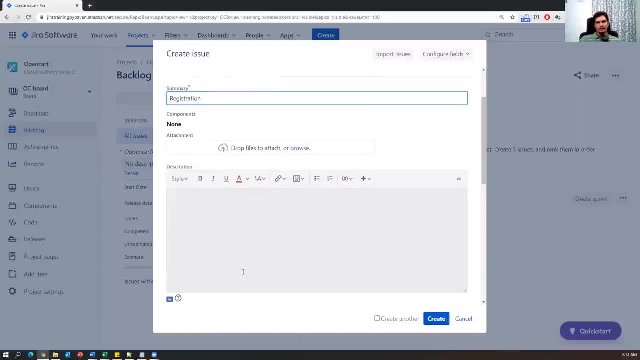 provide as a summary and here, if there is any documentation have for this particular story to understand better, the product owner will attach those documents here, like ui screens or mock screens or dft diagrams. if there is any, any documents are available for this particular story, so product owner will attach those. 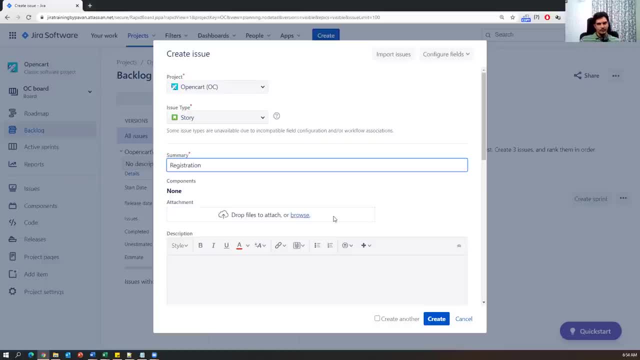 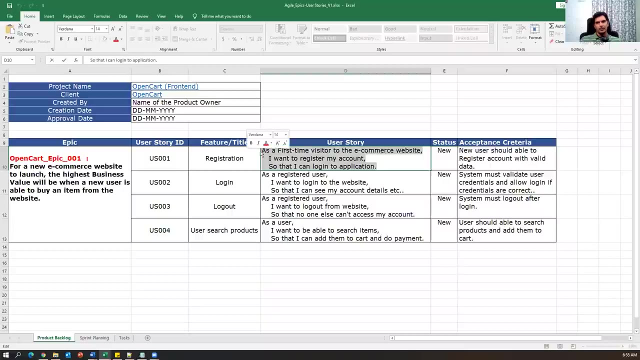 documents to this particular story. okay, that upload documentation is the option is available here and then under description. so in the inside the description we have to add our story. so this is our user story which we need to add. copy this document and then we have to add our story, so this: 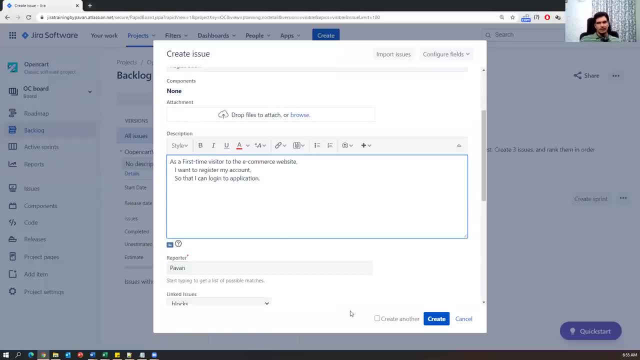 is our user story and specify here: and reporter. so who is creating the user story? normally, here the product owner name automatically will come. if it is a product owner is doing this task and reporter, and then he is a reporter. and if i just look at here, yeah, it will come here automatically. 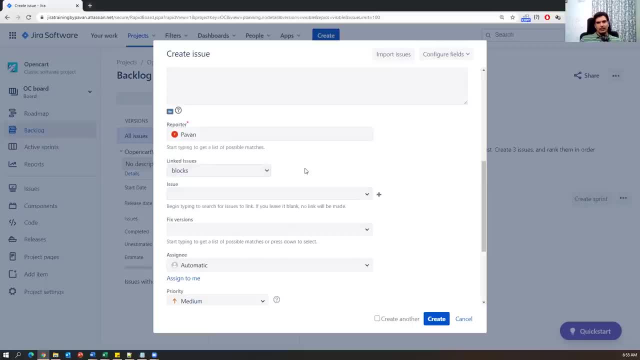 so we have to select that reporter name and if there are any link issues, we can link it or else you can leave it. issues not required: these things are not required and as any, so whom you are assigning the story? so you have to select that person who is responsible for that story. you have to select the proper user or is responsible. 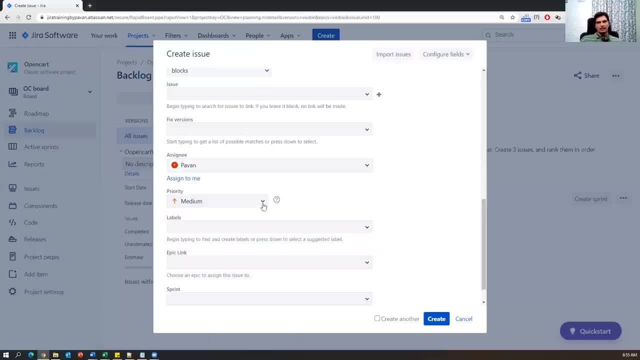 for the story. currently i'm selecting myself- and then what is the priority of the particular story? so how much important it is, how soon we have to release this story to the customer- highest, high, low and lowest we have to select- and the labels you can give for every object, like you can provide. 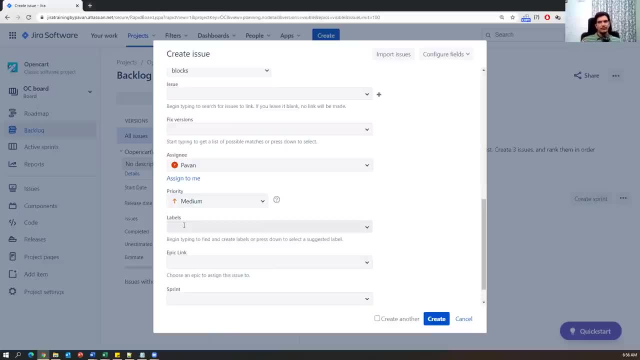 the labels for stories, tasks, epics, everything, because later the searching point of view, it will be very useful if you want to search particular story or particular task or whatever. you can just search with the label and then automatically the story is a task will be displayed, which are: 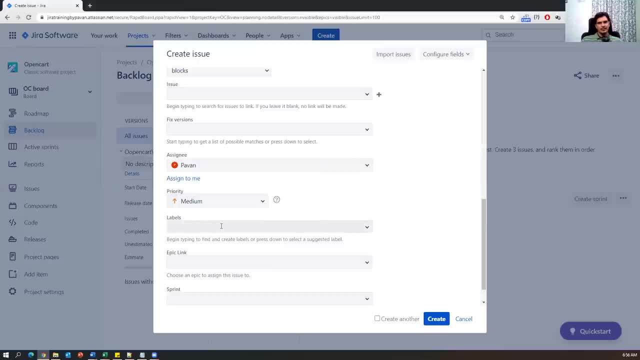 matching with the label names. if you want to provide, you can provide some label names or just leave it empty. and here the epic link. so if i just select this drop down which will show you the epic which you have created, so for which epic, under which epic you are creating this story, so that epic we have? 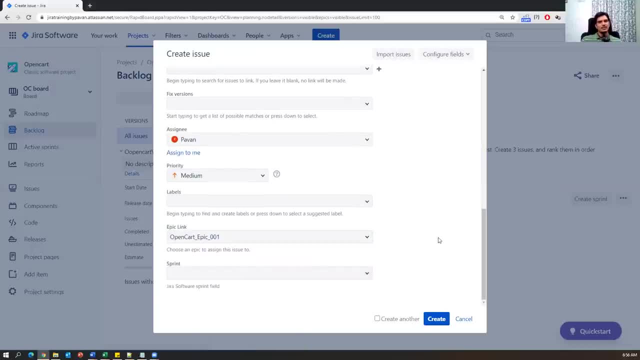 to select here, okay, and on which sprint you are planning this story? so currently we don't created any sprint. we haven't created any spring, so currently you can just leave this as empty. so this is how we need to provide the details in the story and then we just say create. 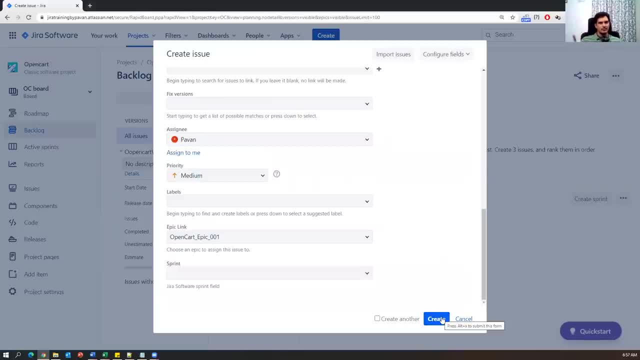 so, again, if i just click on the create button, which will just create only single story, and if you want to add multiple stories, then you can select this option. and then what happens when you create? when you click on this create, then this story will be created and again it will give you. 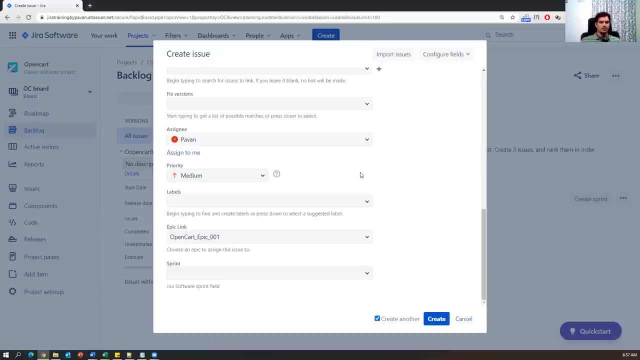 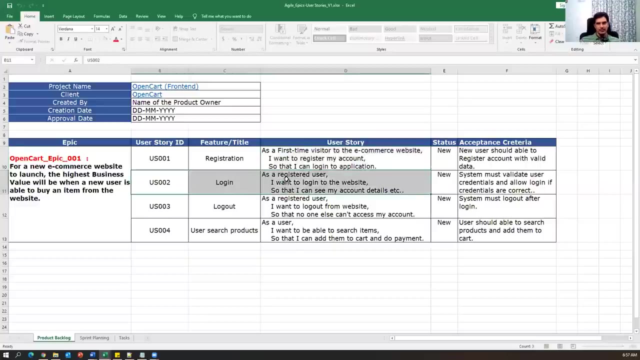 the same screen once again, which will allow you to add one more story. so let me show you that. so select this check mark and then say: create now. observe this: now this story has been successfully created. now i want to add one more story. so again, the empty screen is displayed here. you can just look. 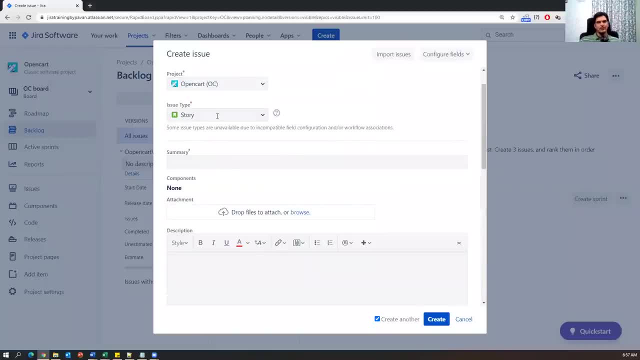 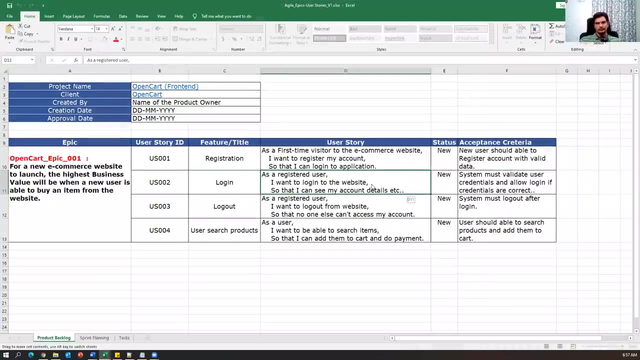 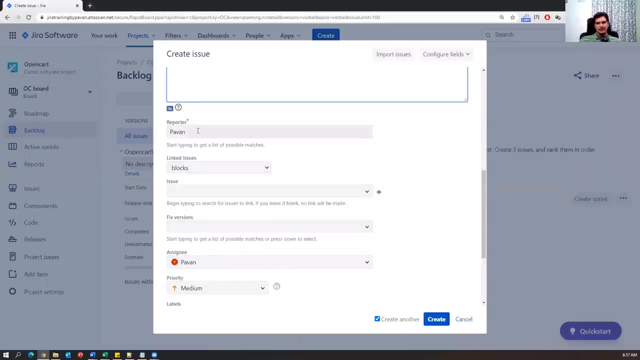 at here right now i am just going to add one more story. so now the other story is a login is another story. i'm just summary and if there is any documentation you can add it. and then i am passing this one user story description, copy this, specify: i say myself is a user. and then i am going to say 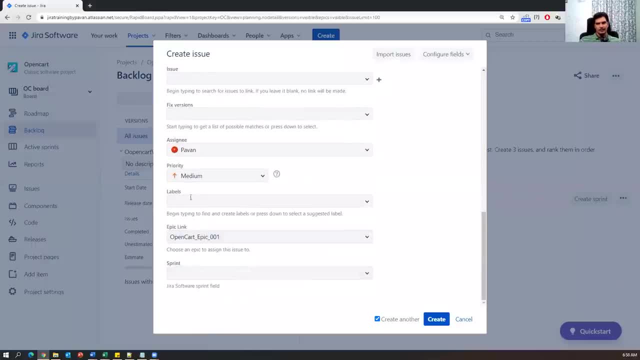 reporter and you don't need to modify anything here if required, and epic link is also automatically linked. i say again: select this check mark because i have one more story to add. so i say create. okay, now it is oc0-3 login has been successfully created. now i'm going to add one more story. so 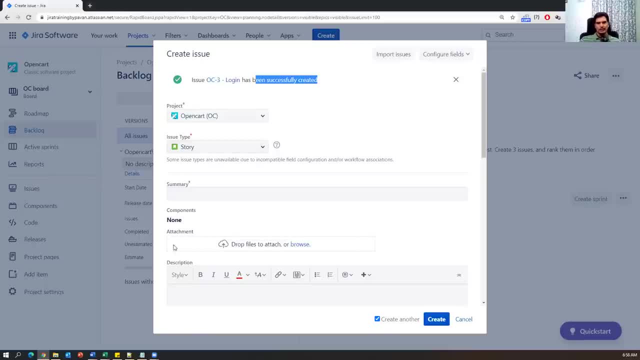 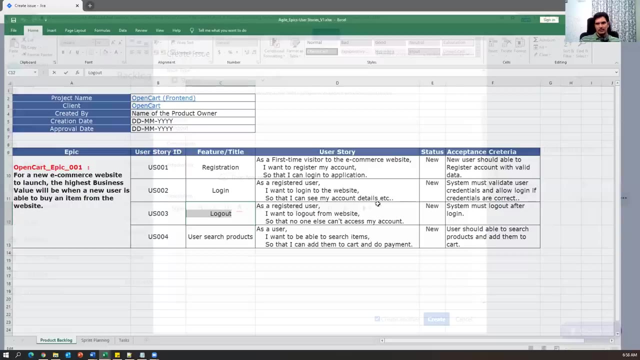 select the project, select the issue type as a story and then i'll provide the summary and then a logout story. i'm just going to add logout and this is a responsibility of the product owner, so tester won't do this activity, okay, so here i'm just copying the story description, put it here: 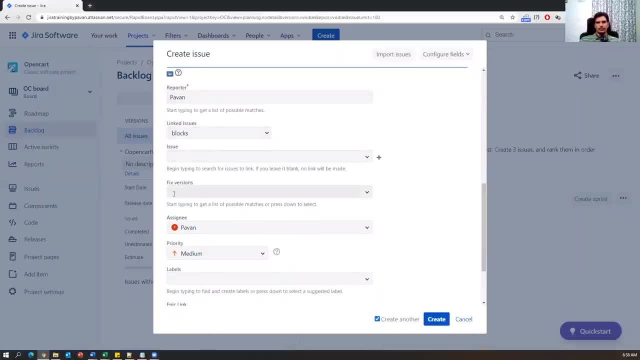 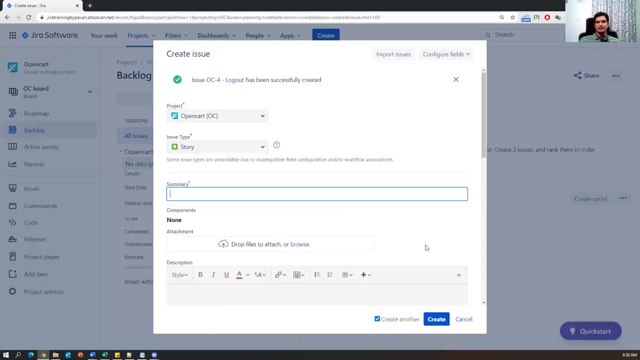 and then reporter linked issues and you can just select assignee and required information we can just put here. otherwise you can just leave it guys. so sprint, we are not selecting here. okay, later we will add the stories to the sprint. so again, create another. just say click, create. now again one more story is being created. 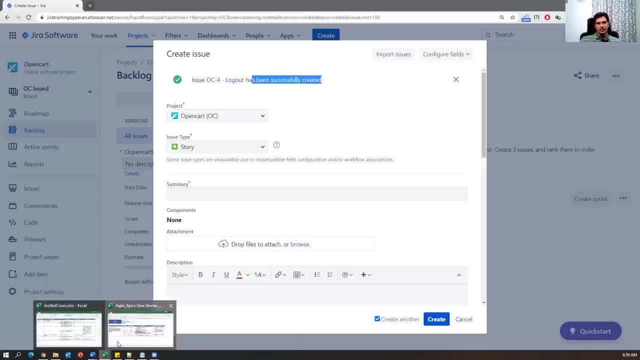 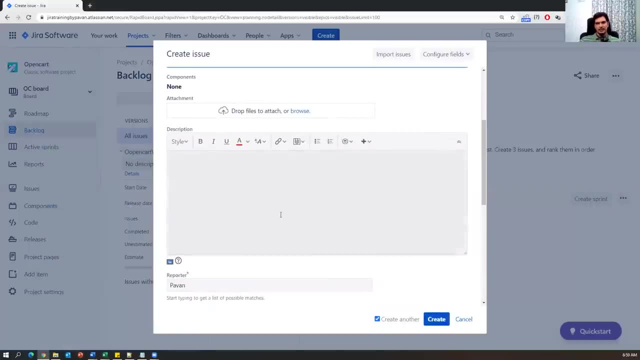 logout has been successfully created. now i have one more last story which i'm going to create. user such products, so provide the summary and the description. this is a user story and the rest of the details as it is, and then this time i don't have any other stories. 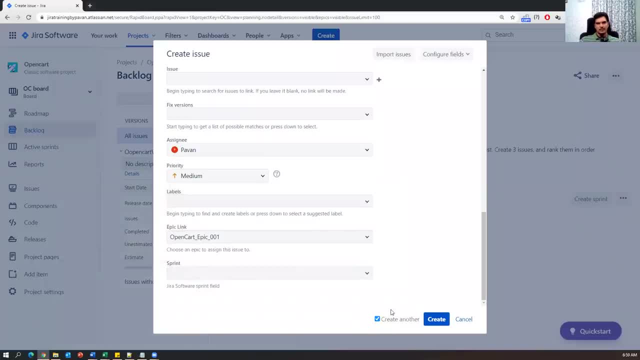 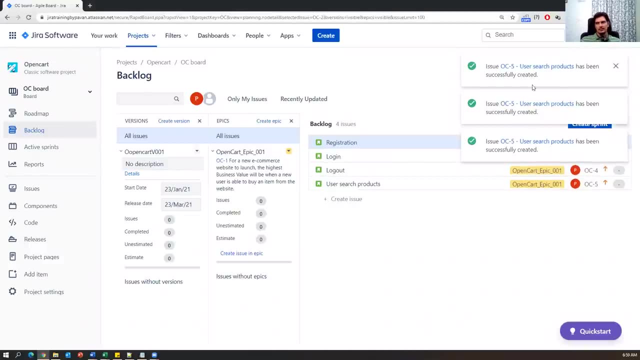 so this is my last story and i'm going to create another story and then i'm going to create another story. so i just remove the check mark and then say create. so now, totally four stories have been created. now you can just check the confirmation messages. now you can see as soon as i go to. 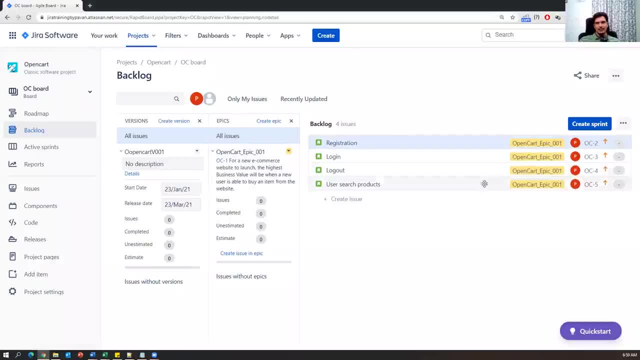 backlog and as soon as you can see epic, and here you can see what are the stories just now we created. so one, two, three, four stories we have created under this particular epic and every story is having some unique id. you can just look at here: oc02, oc0345. 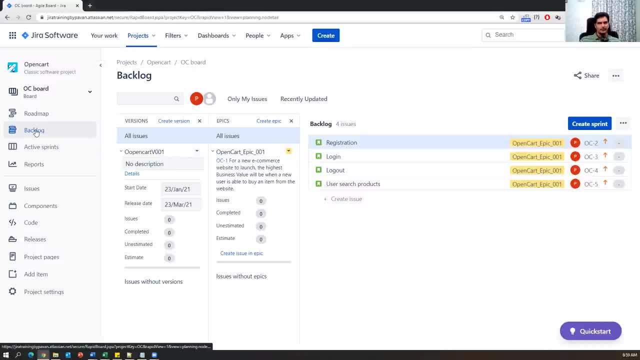 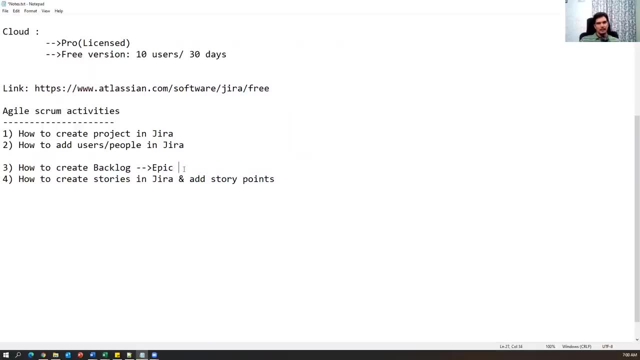 there are multiple stories which we have created under this epic, so this is the next step. so, for what we have done, we have go to backlog and we created epic along with the version under this epic. we created stories- okay, and four stories we have created under this epic. how to create. 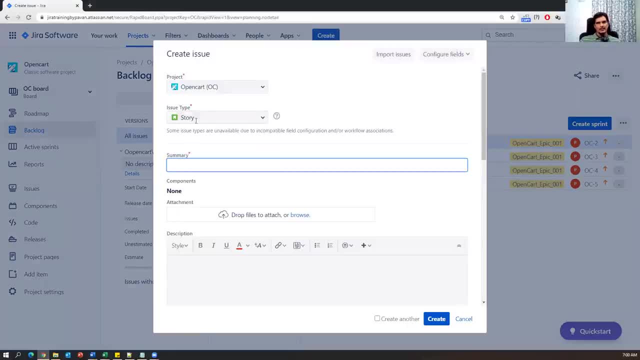 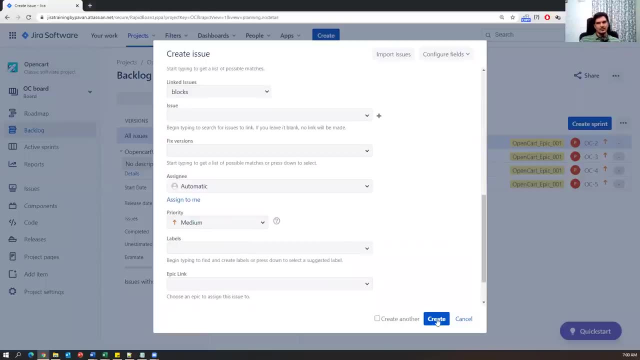 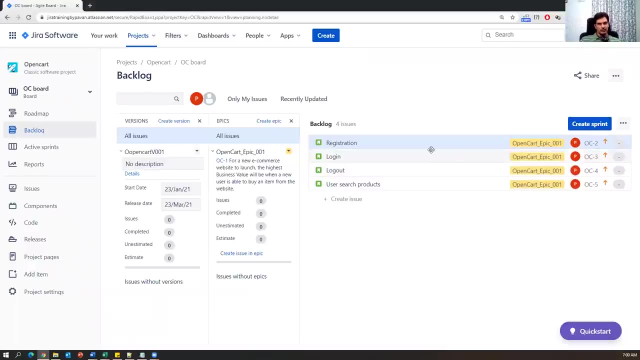 these stories go to create and select that issue type as a story and provide the description summary. you can provide the description and just create as many stories you want. you can just create them, okay. so this is how we need to create all the stories under the particular epic. now, once you. 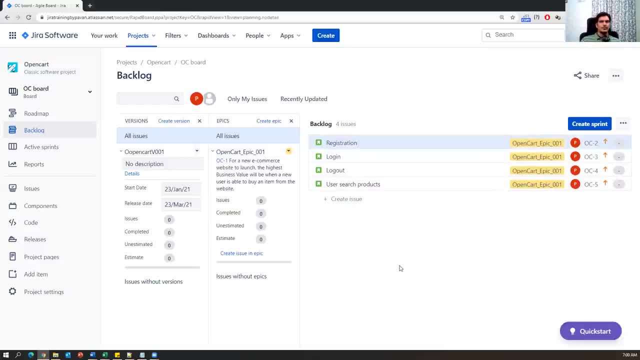 created your story. we have to add story points because we need to estimate that story and, based upon the estimation, based upon the story point, we will select that story for the particular sprint depends upon the duration. okay, so now how we need to add story points to this particular user stories. now let me add some story points. so 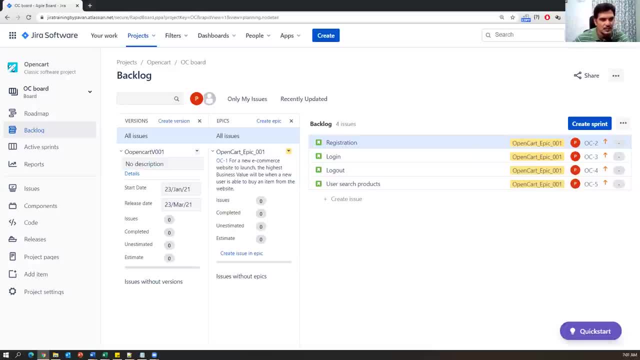 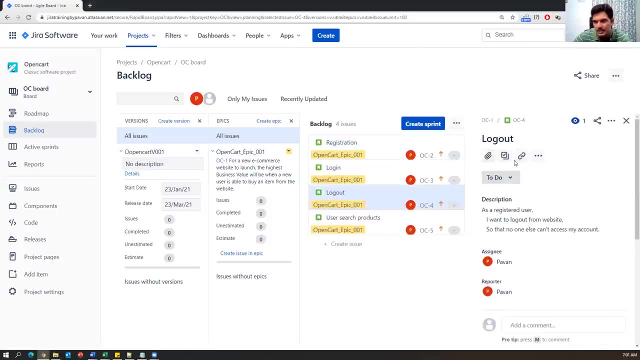 to add story points, this particular story. what you can do is we can just click on the story. so here this is my story registration, so i'm just clicking on the story. so once you click on the story, another side you can just look at. here you can see: 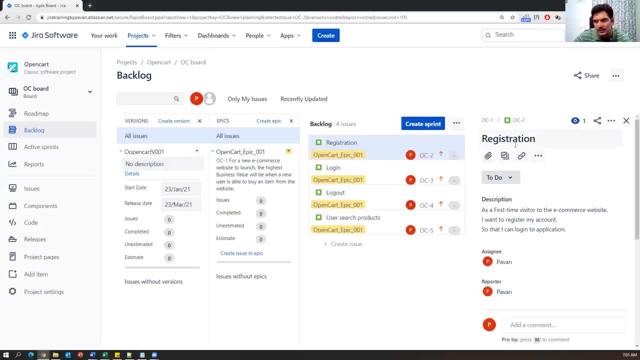 story details. i'm just clicking on the registration. observe this. registration details are appeared here. story details are displayed here. when i select the login, the login details are displayed. when i select the logout: logout details. when i select the user- such products, users- such product- details are displayed. so now i need to add story points to this particular stories. now. first story register. 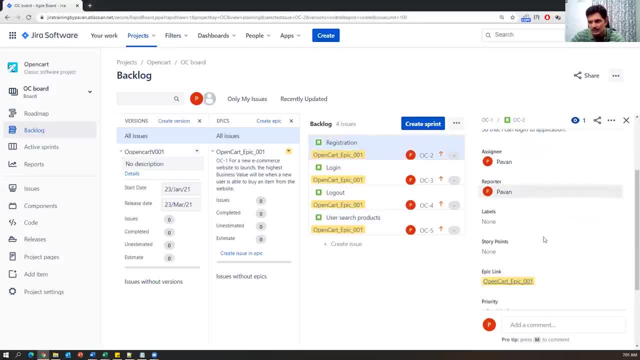 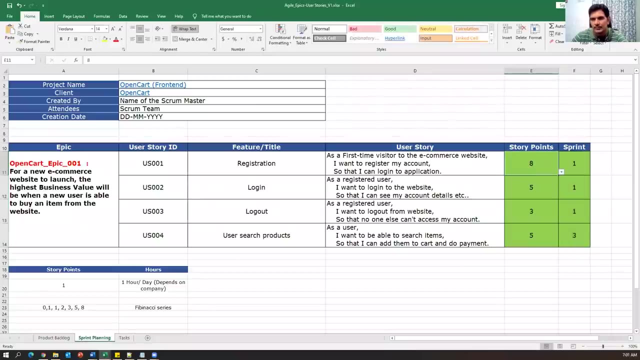 i selected. now, if i just look at here, all the details will be displayed along with the story points. so here we have to provide the story point number. so during the sprint planning meeting we will do all these things. so what is the story point for this eight? so i'm just giving the story point as. 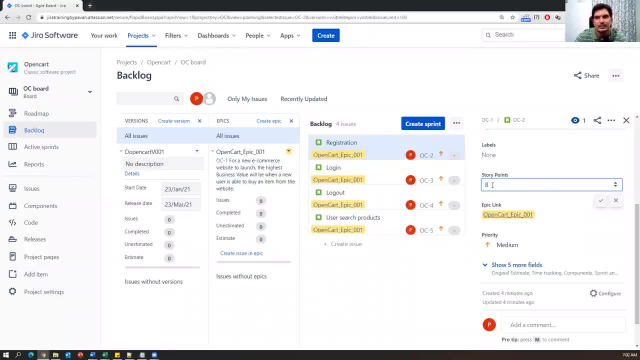 eight, because these are very, very important guys later while calculating the metrics, like when you're generating the burnt down chats. so these story points, time will be calculated. so there's a reason we must specify the story point number for every story. so story point once you provide some number. 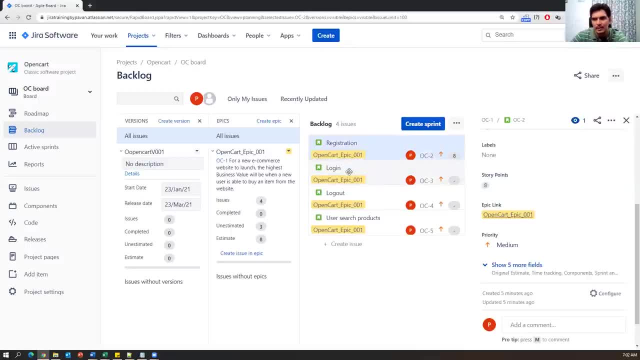 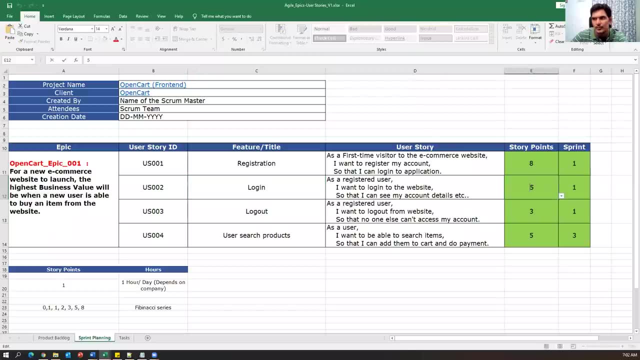 i say tick mark, which is saved. similarly, for login story also i'm trying to add story points. so for login, uh, for login, five story points. you can consider them. some companies will consider each story point, one story point equal to one hour, or some companies will consider like one story point. 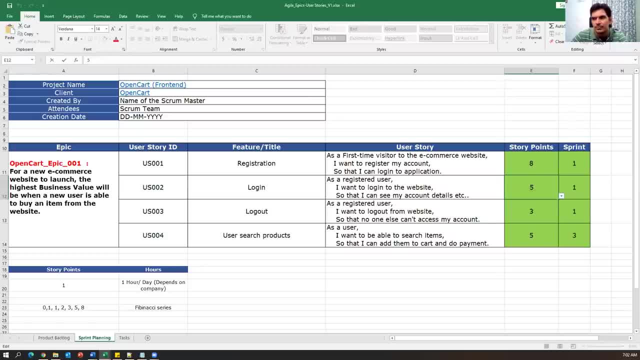 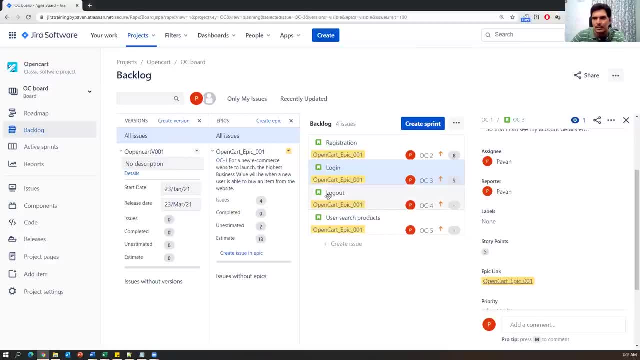 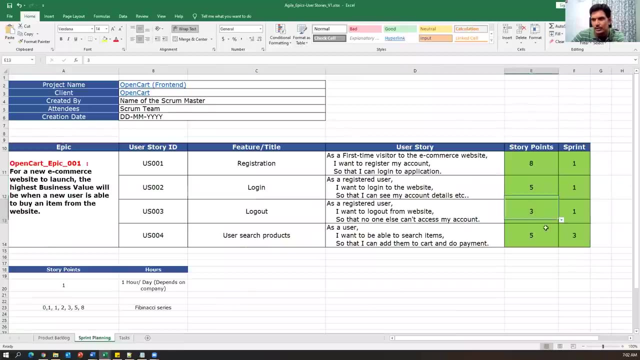 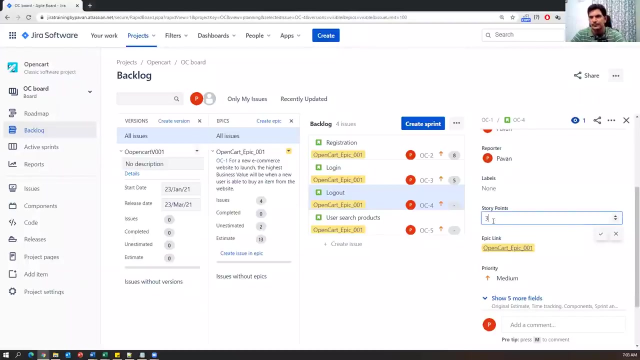 equal to six hours. that means one, uh, one day, so five. so the next two story: login, story point is five and say tick mark so that is saved, then log out. so for logout, okay, so for logout the story point is three. so i'm just going to provide story point as three and then selects and. 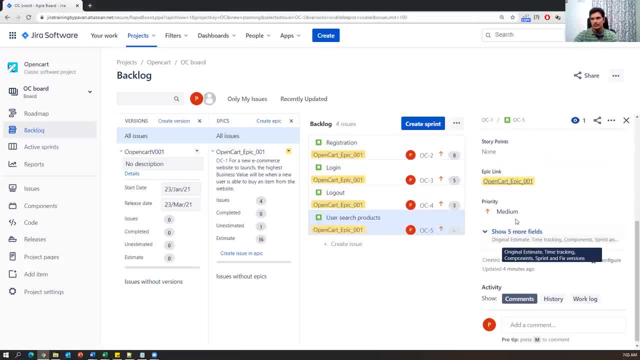 then for user search products, story point is: i say five, i say five and then say tick mark. so now we have have added story points for every story. whatever stories we have added into that particular epic, we have added story points. okay, so that's the next step. so we have created the number of stories. 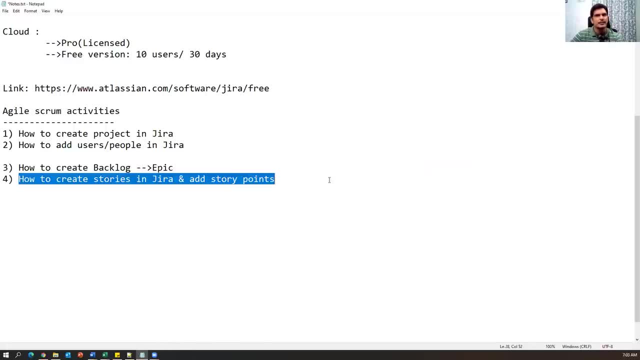 inside the epic, and for each story we have added story points. so with this the backlog is ready, so product backlog is ready. so backlog contains epic- one epic currently- and the epic contains multiple stories along with the story points. so now the next step is we have to create a sprint. 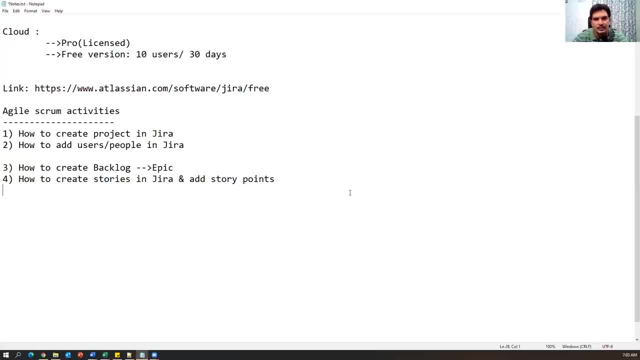 okay, so in the agile process, in the during sprint planning meeting, we will decide so how many stories we have in the backlog, how many stories we have to develop and test for that particular sprint and what is the sprint duration. we will do that right so now, as soon as we have ready with 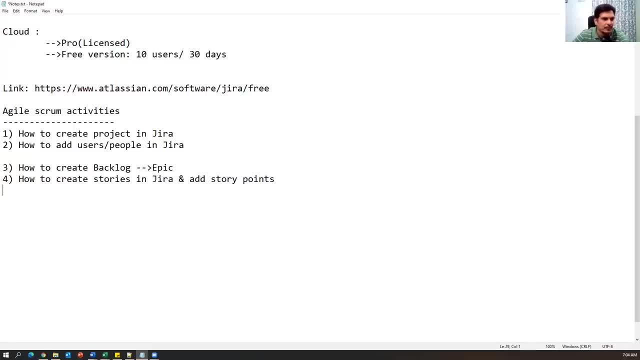 the product backlog and stories are there. now the next step is we have to create a sprint. so we have to create a sprint and then we have to add stories to the print and then we have to start the sprint. that's the next activity. fifth step and 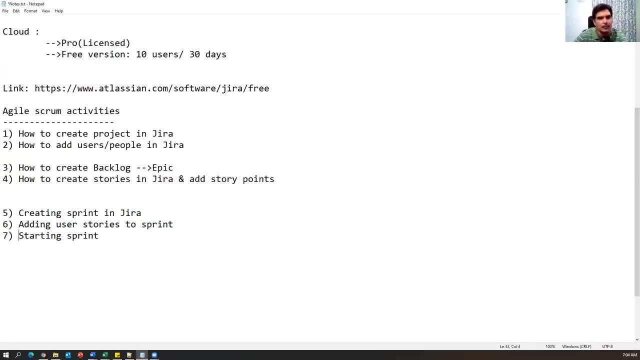 sixth and seventh. so now backlog is ready with that, which contains a number of stories. now the next step is we have to create a sprint. sprint is nothing but three, two to four weeks of time. a small, small period of time. we can call it as a sprint. 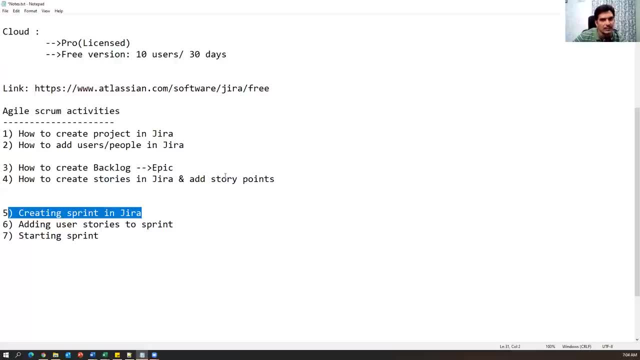 so once you created a sprint, then we have to select some stories from backlog, add those stories to the particular sprint and then sprint will start. so as soon as we added stories to the sprint, developer and testers will add their tasks for each story. okay, and then the sprint will start. 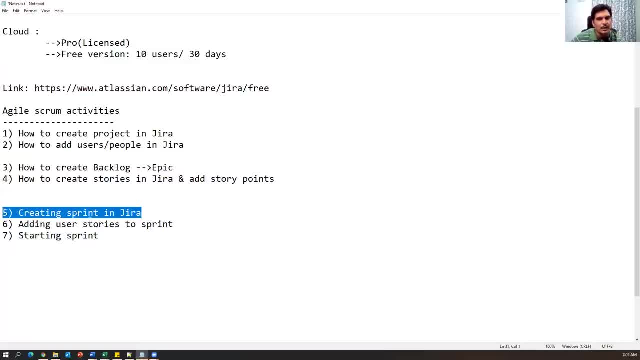 now we'll see how we can create a sprint then how to add the stories to the sprint. so the stories of the product are already ready in the product backlog, which are created by the product owner. now we have to choose the particular stories and add them to the sprint. then we will start the. 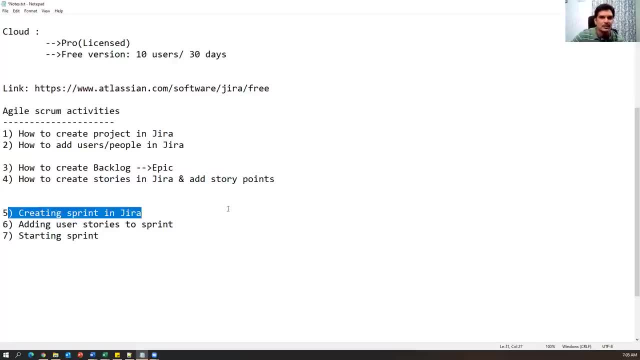 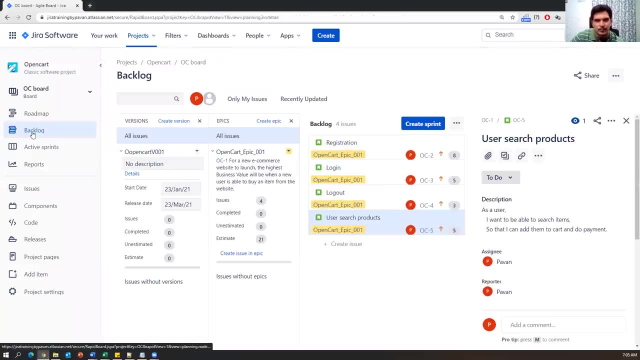 sprint. okay, now let's see how to create a sprint in jira. so to create a sprint in jira, what you have to do is so. if i just look at here, we already went to backlog and current project and backlog. click on the backlog. you can see the a pixel list and stories, everything here you can just 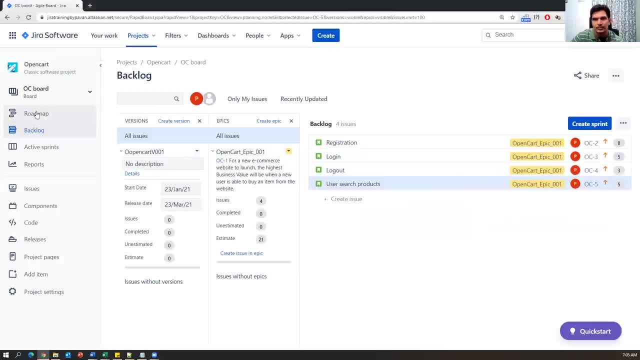 close this window. also right so now we are ready with the backlog. so backlog contains the epic. epic contains the stories. now, to develop and test these stories, we should start with the sprinter. right so now we need to create a sprint. so to create a sprint, the first sprint, and just click. 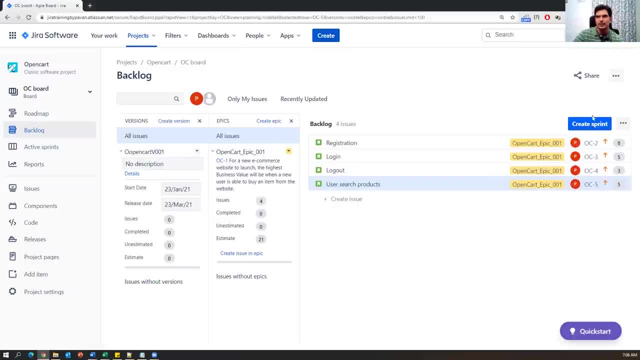 on the create sprint button. you can just look at here. a small button is up here: create a sprint. okay, what is print sprint is a, a cycle which contains a two, two, four weeks of duration. within the duration, we have to implement few number of stories, not all the stories. okay, we will choose specific stories which are uh enough to particular two to. 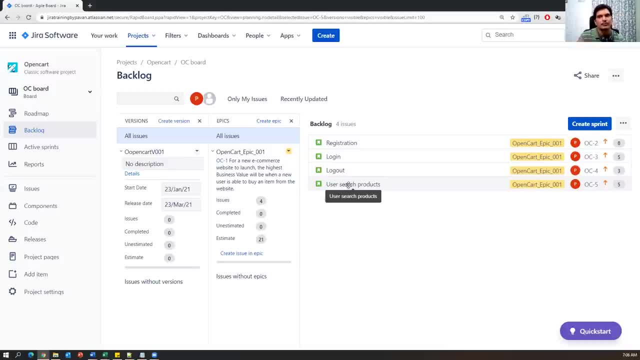 four weeks of time- like within two to four weeks of time, how many stories we are able to develop and test, and only those stories. we will pick up and add them to sprint and then we'll continue the process. so let us create a sprint. so i just clicking on create sprint. okay, so once you click, 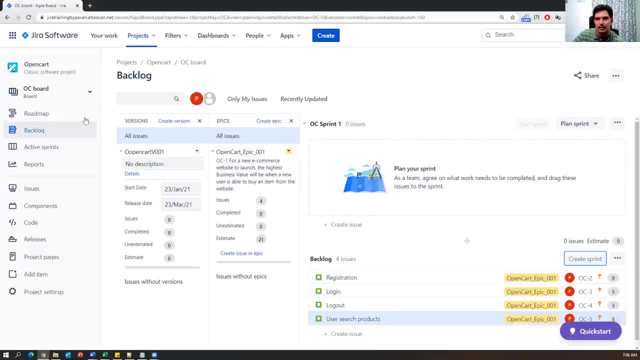 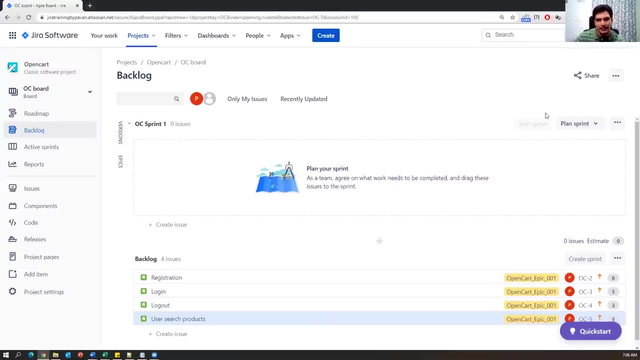 on create sprint now. observe this. okay, i'm also closing this epic window and this versions window. yeah, now, as soon as i click on the uh, create a sprint now, you observe, you will see a new screen something like this: so this is a osis print, one which is created now. it doesn't have any issues. 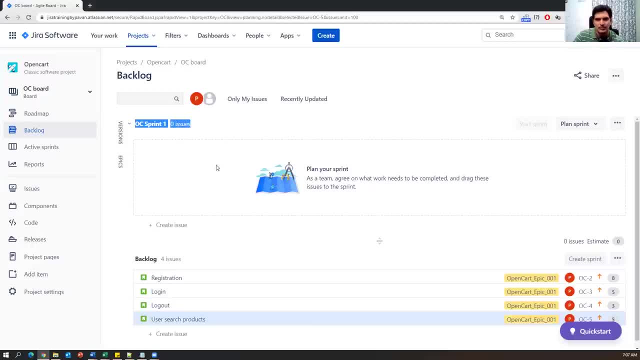 means what if this print is empty now it doesn't have any stories planned for the sprint. as soon as i click on the create a sprint, you will see this osis print one. it doesn't have any stories. now what you have to do from this backlog, from this backlog we have to. 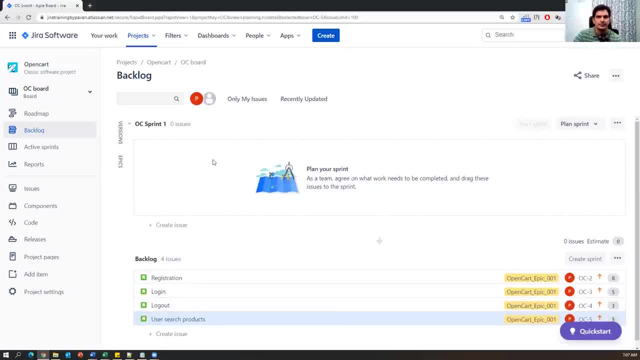 add some stories into this particular sprint. so now, as per the planning, let us say, developers and testers decided to develop and test registration, login and logout functionalities as part of sprint one. then what you have to do is just we need to drag the stories like this into sprint. 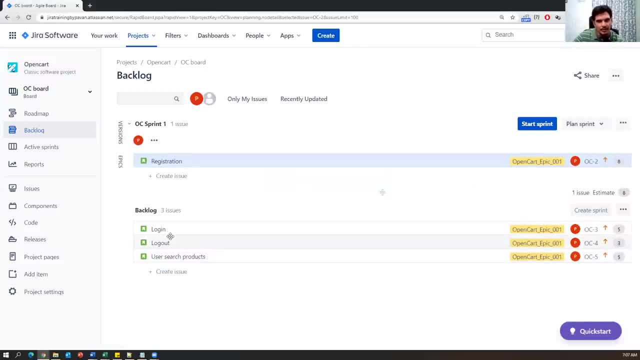 so first two stories added to the sprint one now. similarly, login is also. i'm dragging to the sprint one and logout also have planned for sprint one now. user search words. i will take this story for the another print later. so now i have selected few number of stories from the backlog into sprint one. 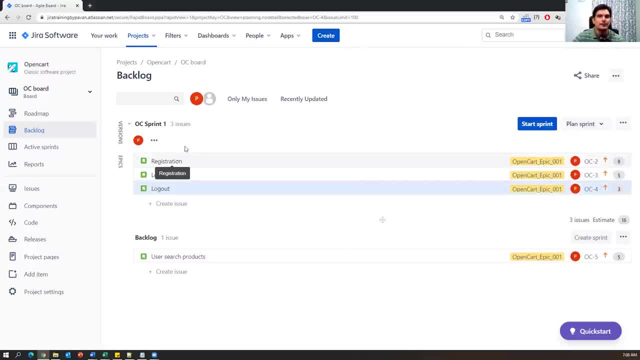 okay, so now these three stories are part of sprint one. so now currently three issues are there in the sprint one. what are those three issues? three stories, registration is one story, login and logout. okay, so now our sprint is ready, so sprint is created and stories also added to the sprint. so 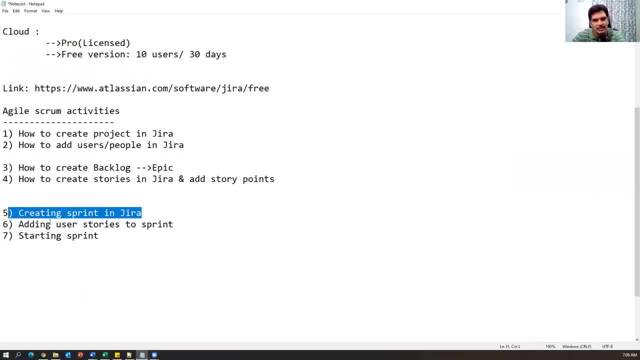 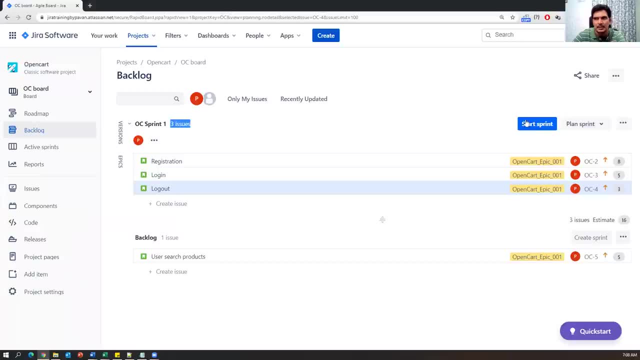 once we have done this, what is the next thing? we have created a sprint in jira, added stories to the sprint down. then we have to start the sprint. so how to start the sprint? there is one option called here start sprint. so once you click on this start sprint, then the sprint will start. 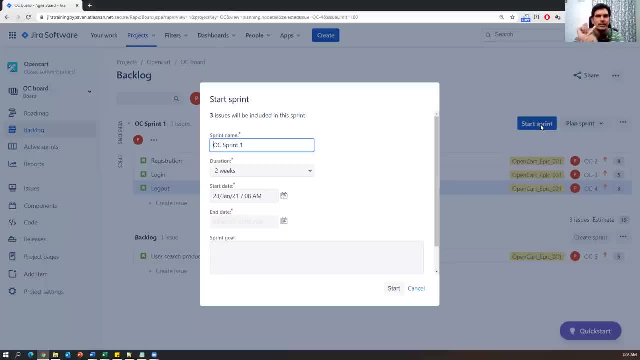 so when i click on the start sprint you can just look at here. so we need to specify the duration, very, very important. so this is a sprint. we have started first to sprint how much? how much duration? one to four weeks, that depends on the company. okay, so some people will take one to two weeks. 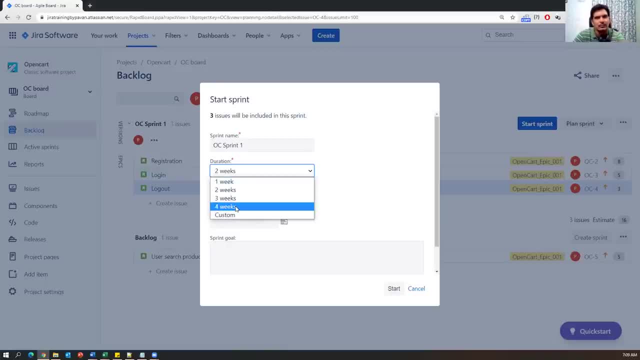 or one to three weeks, one to four weeks, max four weeks, but it can also extend if you want. so i'll say two weeks duration and from which day to which? i have already selected two weeks here, so the end it automatically calculated. okay, what is the sprint goal? so to develop and test registration. 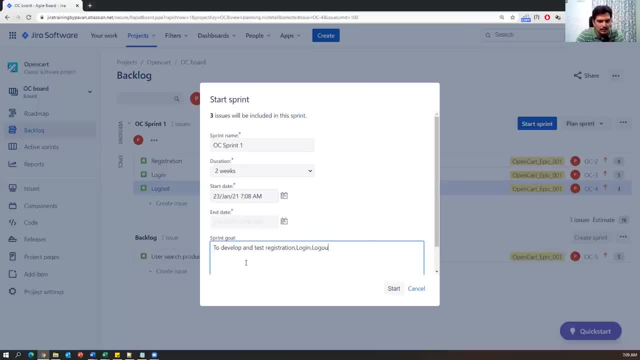 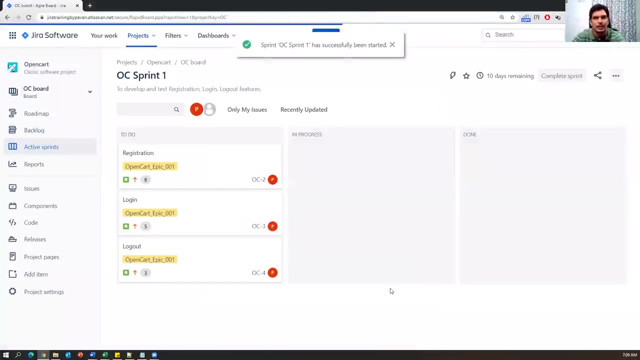 registration, login, logout features. this is the goal of this particular sprint. okay, because we have selected only three stories for this particular sprint. so once you return the goal, you can just come down. nothing is there, so then just say start. so as soon as you start here, the sprint is started. now this is a scrum board, or we can say storyboard, so we can see the statuses. 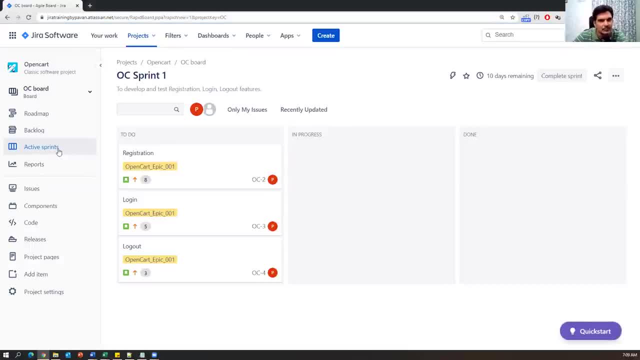 everything in this particular board and this is the active sprint. so currently, which sprint is going? so sprint one is going. if i just click on the active sprints, then what in which sprint you are currently working on, which will show you here. so currently all three stories have added to the sprint. so to do and in progress, and done so still we have not. 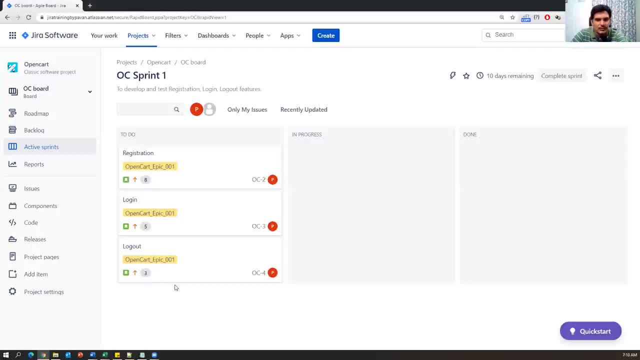 started these stories as of now. so it is there in to do section now. once it is in progress, we can just slowly move on like this. we can drag like: once it is story is completed, then we have to move it to the done state. so normally these things will be done by the scrum master guys. 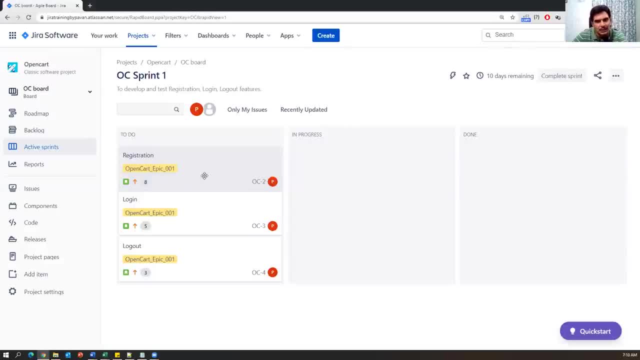 okay, during the scrum meetings they will ask the dev and qa team: okay, what is the status of the story? and developer says, okay, i have done all the tasks for this story. and tester says i have done all tasks for this particular story and then, if it is in progress, he will put in in progress section. 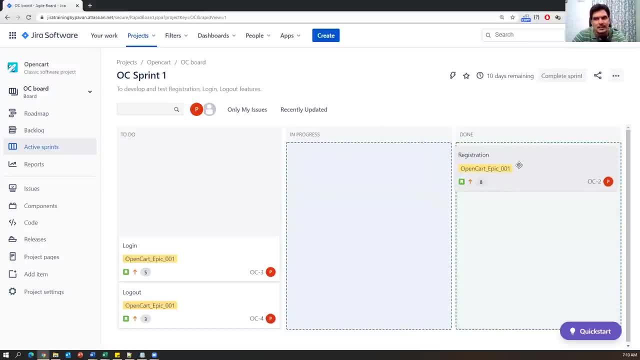 or, if it is completed, then he'll put the done state. once it is moved to, the done state means what: that story is ready for demo. the story is ready for demo and once the product owner is accept or approve that demo, then we will release that as part of the feature. so this is how we need. 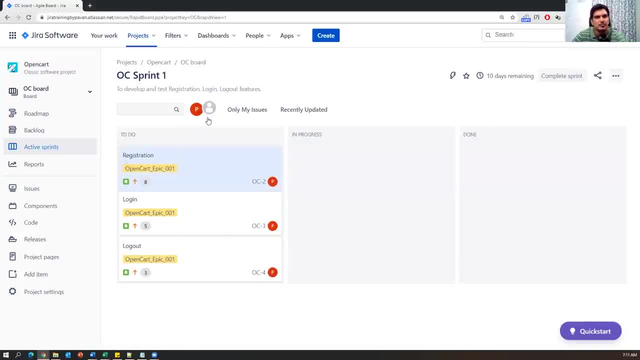 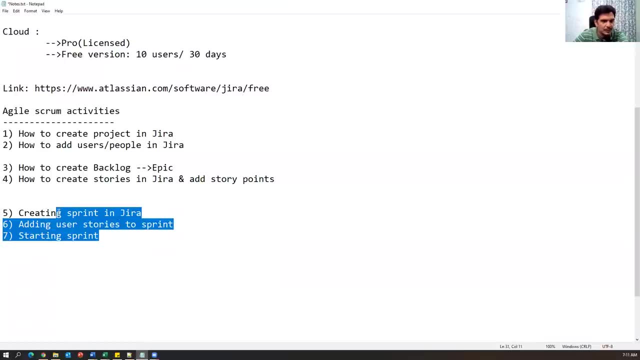 to track the statuses. so now we have just done the demo and we are ready to move on to the next step. we have just created one sprint, added the stories to the sprint. now we have started the sprint, so started the sprint now. once you started a sprint, each story is having different tasks. 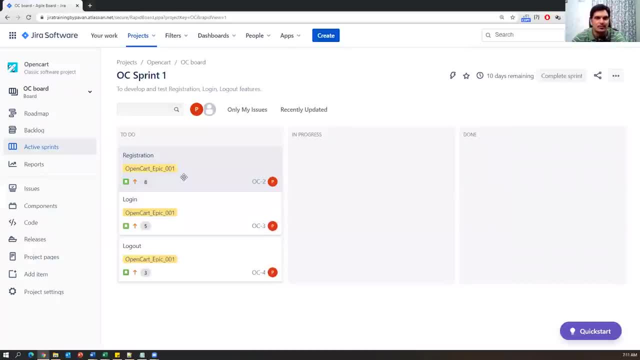 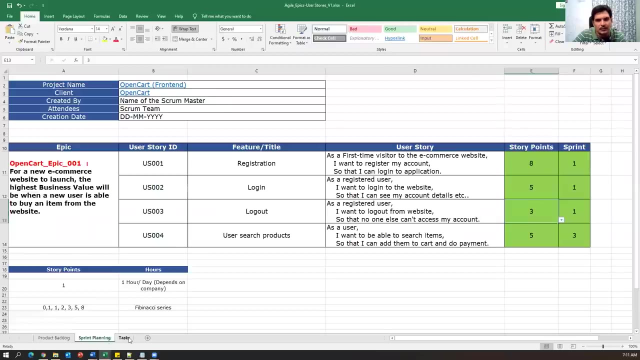 suppose when i say registration is my story or feature, for that registration story developer will do their own activities. tester also will do their own activities, right? so for registration, what are the developer tasks? normally what developer will do is: developer will perform these tasks: understanding the story or requirement, design the story, coding. 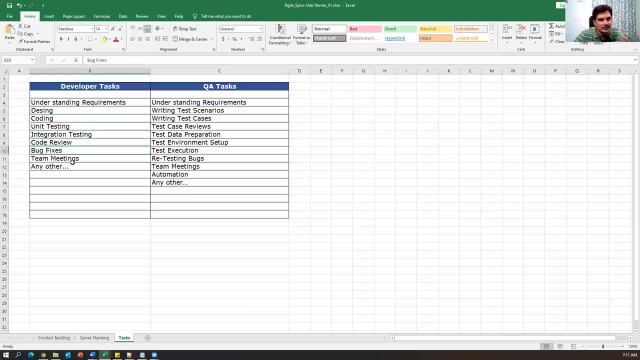 the story: unit testing, integration, coding, bug fixes, team meetings. these are all different tasks done by the developer for that particular story. similarly, as part of the qa, you will understand the story or requirement: writing the scenarios, writing the test cases, reviews, data preparation, environment, setup, execution, bugs, retesting team meetings, automation. these are all different tasks. 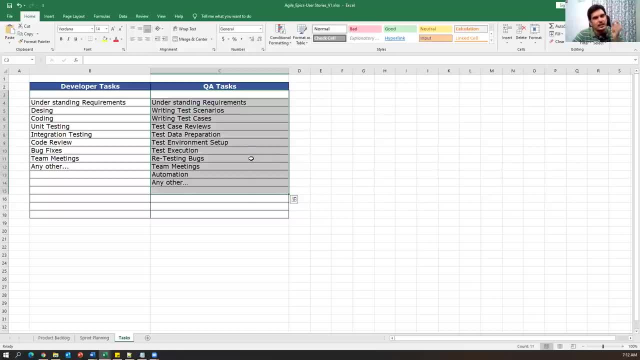 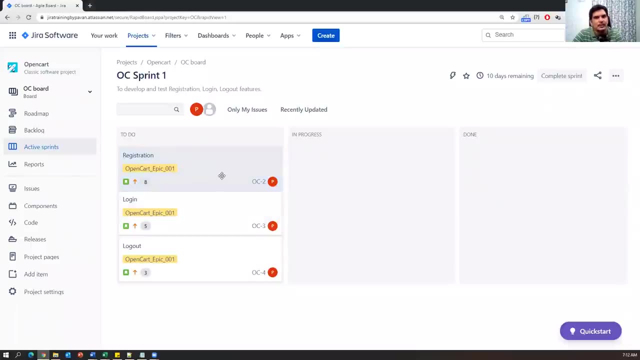 done by the tester for the particular story. so for each and every story there are set of developer tasks. there are some qa tasks. okay, now we need to write these tasks inside the story. so now, if i just go back, for each story we have to define: developer will define their own task, tester will define. 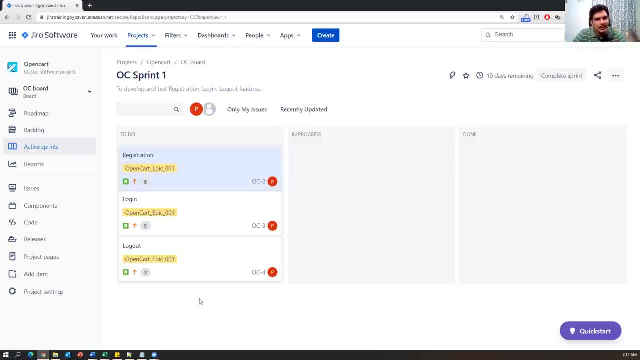 their own task. now, from here, this is a responsibility of testers and developers guys. so once a sprint is created and started from there on this, downwards developers and tester responsibility will be the more. but during product backlog, reading the stories, planning the stories- these things will be part of product owner responsibility. 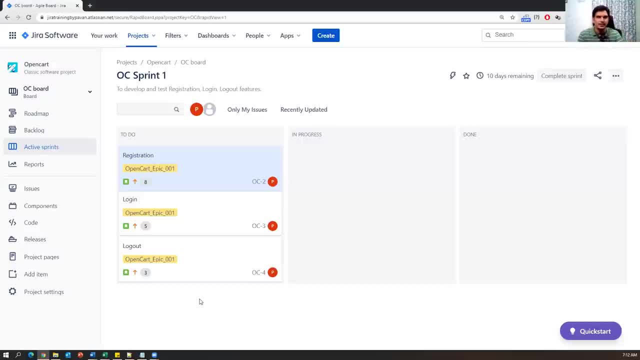 of the product owner has come master. once the sprint is created- committed stories- then the responsibility is developers and testers. now, before, once you started the sprint one, then what you have to do is: for every story developer will add their tasks. similarly, for every story tester also will add their own task. and one more thing: these stories will 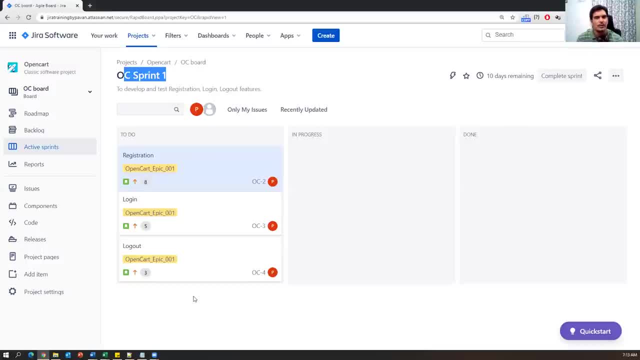 be developed and tested by multiple people. so only one developer is not responsible for all the stories. similarly, one tester is not responsible for all the stories. okay, suppose let us say first story, one registration. some group of developers work, one or two developers and one or two testers. 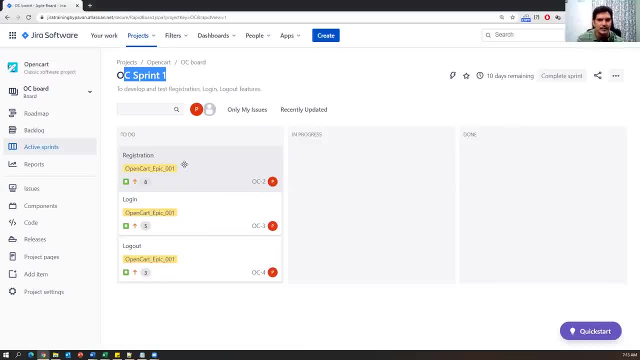 similarly for every story, there are multiple developers and multiple testers working together for that particular story. now, so, before progressing this story, the first thing is we have to clearly define the tasks for each story. we have to clearly define the tasks and we will define those tasks. developers and testers will define the task. now let us see how we can add tasks. 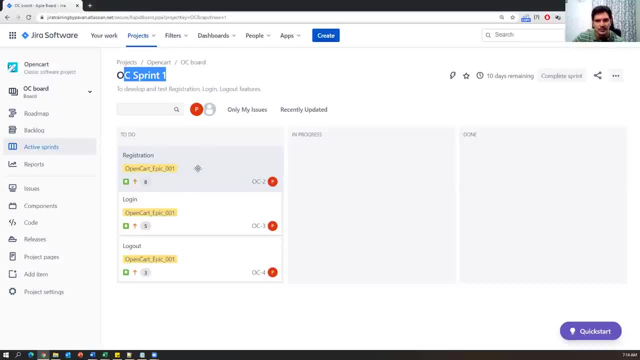 for this particular story. now just click on the registration. once you click on this, you can see there are two questions only: vs and b �途 Mil takai nì班 ar Spiel, Gracias, Okay, so all this, what you can do is just a moment, because you need to just click on the. 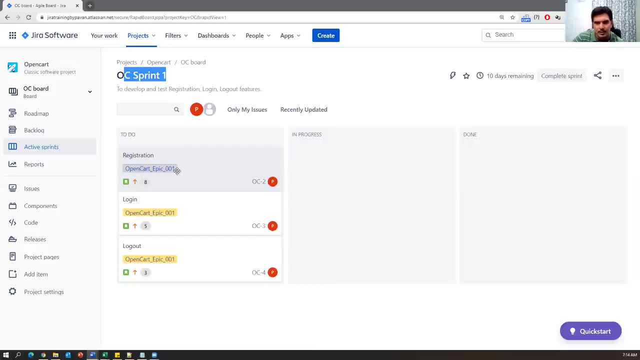 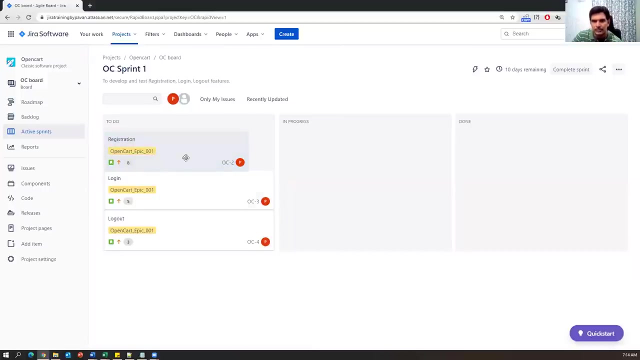 here. you can just look at OpenCart. a pink 00 one is the right. so I just click on this, which will open up one smart green that's hijacked. it is a corresponding very slow guys just a second worms with. so once you click on this, it will open up one small screen. there you can specify the. 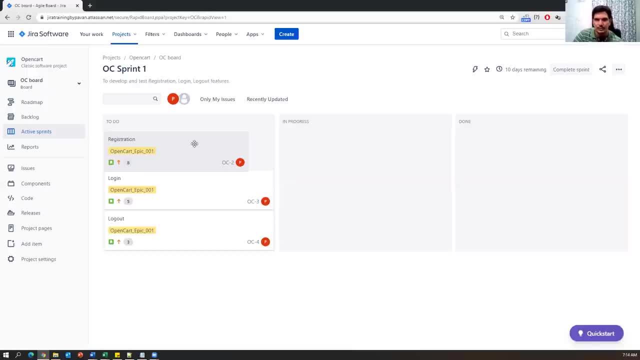 tasks. you can add the tasks for this particular story. okay, let me just go to projects again. i'm just coming from the beginning, so go to project. select your project. yeah, now you can see. you got the screen now. so it has come very late, guys, slowly we have to do so. let me show. 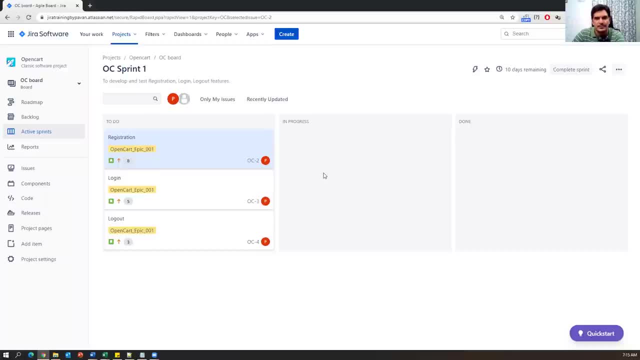 you once again. so this is our scrum board. okay, we have started sprint. now we need to add tasks for each story. so let us take one one story. okay, now i'll show you how we can add tasks and everything. so let us see first story registration. so click on this registration. okay, once you click. 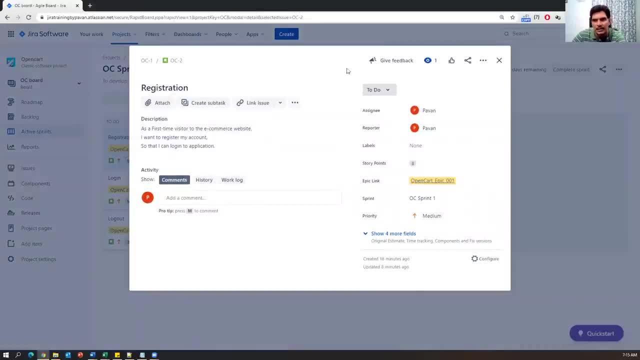 on the registration story. now you will see this screen and in this butler screen you will see all the details about the story. okay, now you can see the description of the story and everything. so now we need to add tasks for each story, so let me show you once again. so this is our scrum board. 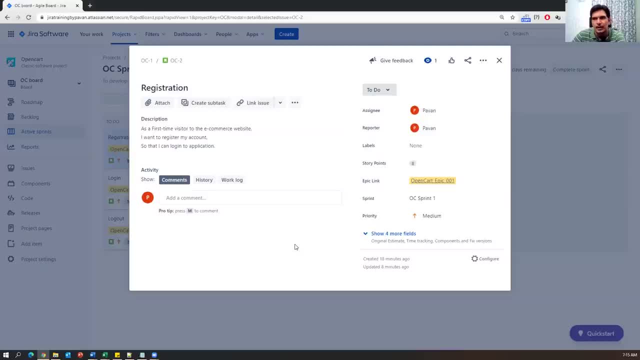 add tasks for this particular story. so how we can add tasks, you can just look at here, create a subtask, and when i say create subtask means which will create a new task for this particular story, okay, or in other way, what you can do is we can just directly go to create here. 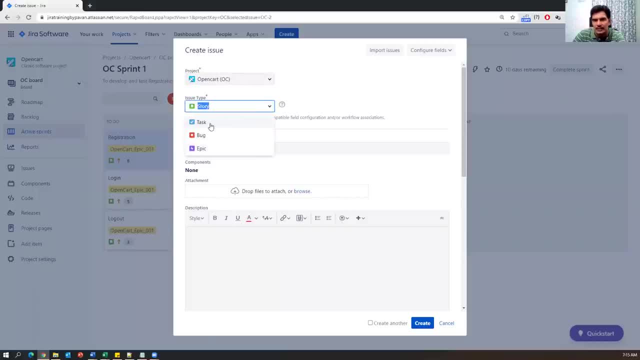 and inside the project you can select the task directly here. okay, so select the task, and now you can just specify the summary and here you can just select the something called on which epic and which sprint you are going to add the task. and this is task, is very high level. task means: 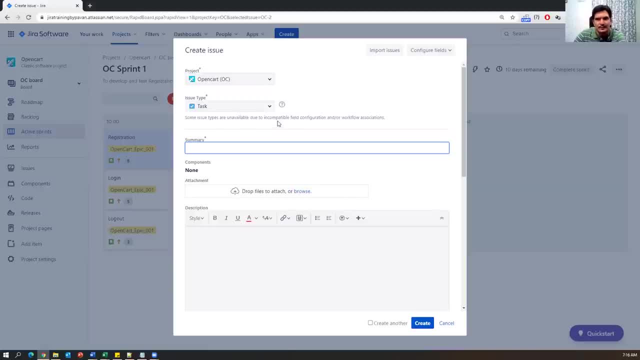 it can be anything not specific to story. the task can be anything not specific to story. it can be any meeting or it can be a review. okay, any task which is not specific to that particular story, right, but i want to create a task which is specific to story. 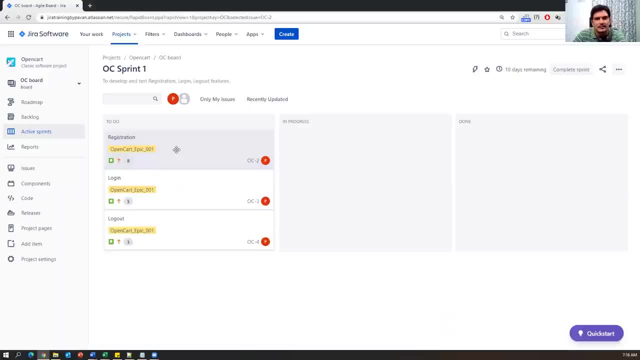 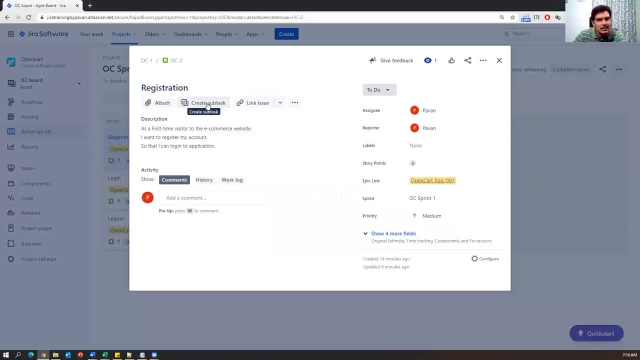 okay, now what i have to do is we need to call it as a subtask. so just click on the story, then you will see this window and here you can see one option called create subtask. so once you click on the create subtask, then subtask- what are the tasks you want to do? so the first task: as a tester, we. 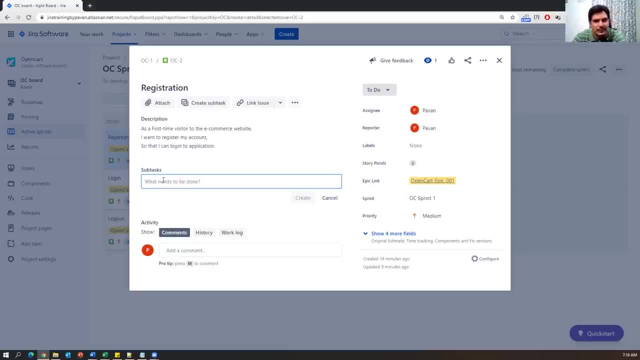 need to add some tasks. as a developer also, we need to add some tasks. okay, now let me add first development task. so, as a developer, what you will do first. so these are the tasks that we are going to do. uh, different activities we do. so understand the requirement: design, coding, unit testing and 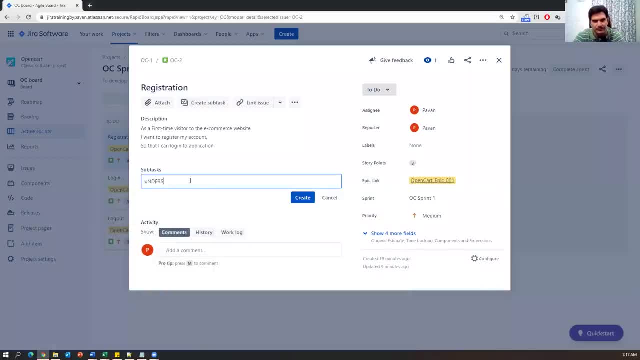 everything. so let me add some tasks. so first understand. let's say, or we can simply directly i'll say: understand, understand requirements is understand, requirement create. and this is qa and dev, both the job combine. we will do okay. i'll say: dev and the qa together will understand the. 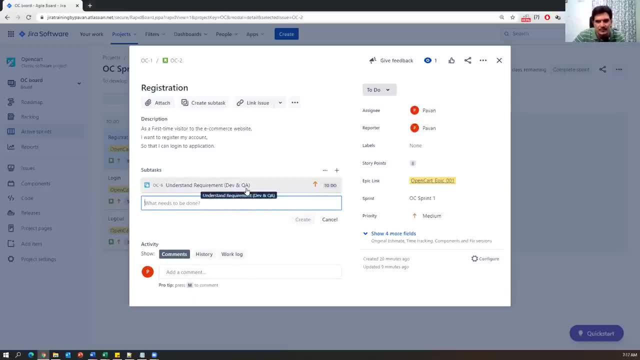 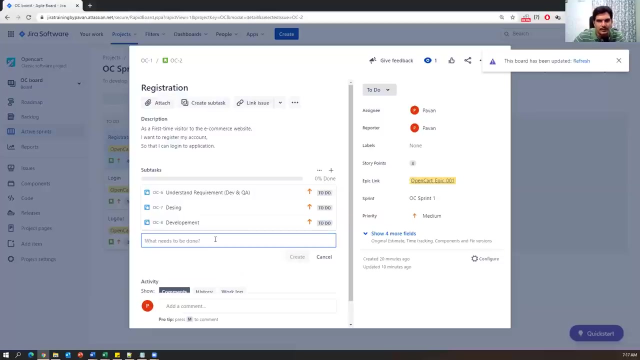 requirements create. so now one task is created. you can see, and somebody in the team, we can just complete the status task later. so now another task. i say development, or we can simply say design. design is one task, and then development, development done by the developer, and then 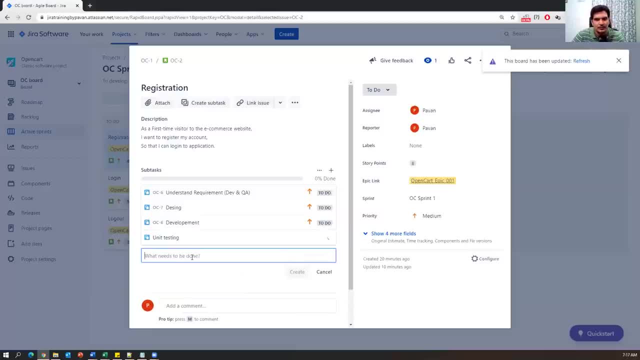 unit testing. unit testing is done by the developer. and then what else they can do? unit testing and integration testing, integration testing, and developer will do that. and also developer fix the bugs. so bug fixing, bug fixing, so these are all the different tasks will add by the developers. and similarly, for the same story, we also add our qa tasks. so just you can just close. 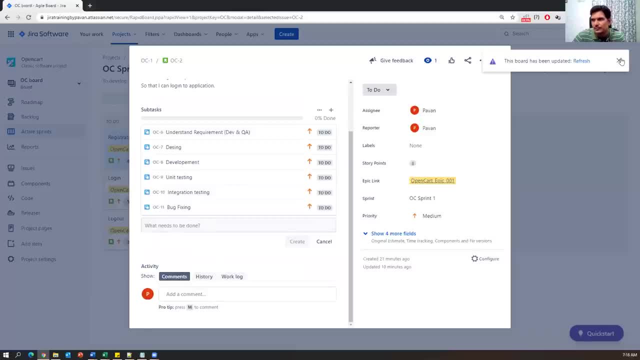 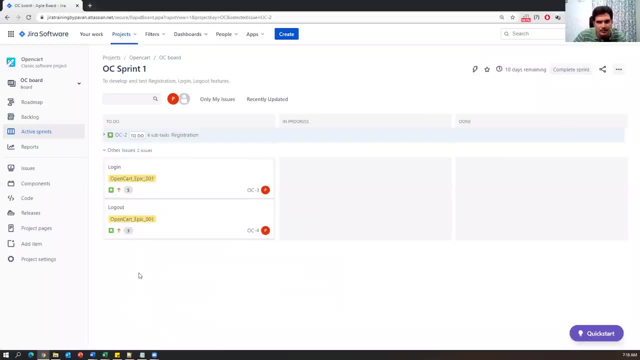 this for now and, uh, once it is closed, so you can just close it then. so developer is define their own tasks for this particular story. now you can just look at the scrum board, see this. this is the registration story. login story, logout story. right, so for registration story, developer is added their 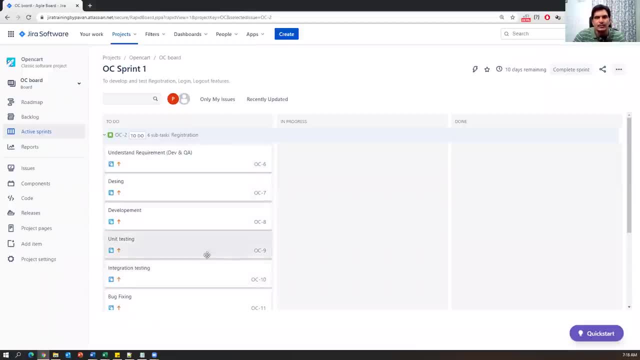 own tasks: understanding requirement, design, development, unit testing, integration, testing, bug fix, right. so now we need to add our own task, testing task. we need to add. so how we can add again. click on the same story- registration, which will open up the window. now these are the stories. 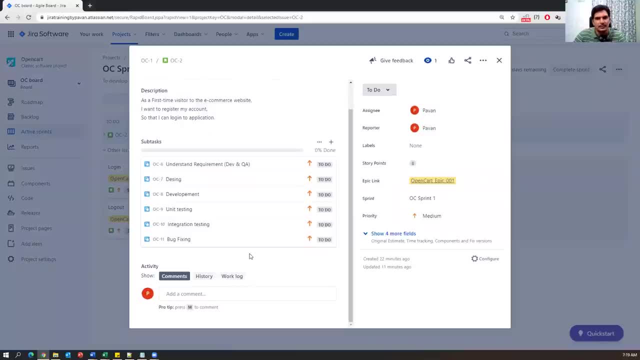 created by the sorry. these are the stories created by the sorry. these are the stories created by the. these are the tasks created by the developer, so he is responsible for completing these tasks. and once the developer is completed these all tasks and also testing tester tasks, then only 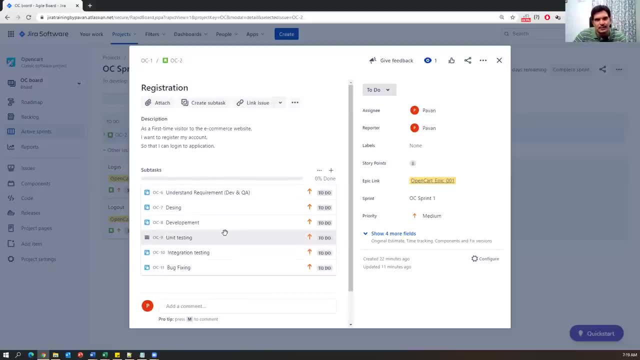 we can say: story is completed. okay, now let us add few more tasks from the q8 side. so click on this plus button, you can add, or you can click on this: create sub task. okay now q aside. so understand the requirement. devon q is already there, so now test cases. test cases creation. 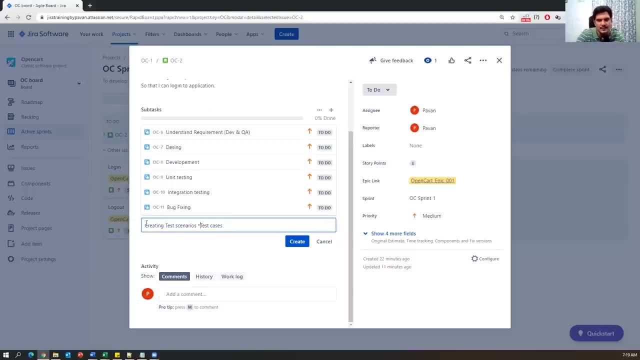 creating test scenarios and test cases. so this is a one activity done by the qa. so create: now one task is created and then, after test cases, what you will do is we will set up environment and install. build- this is another task because it takes some few number of hours right. so each and every. 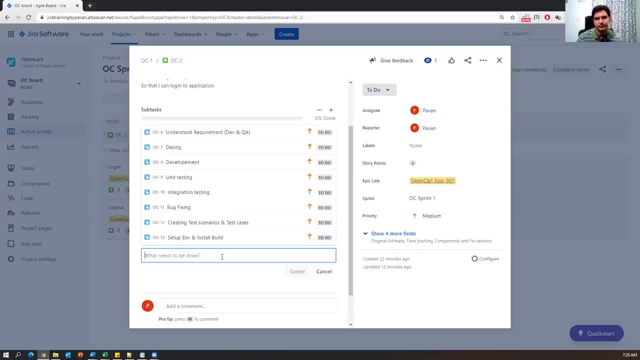 task we have to calculate, guys, okay. so because we will track each and every activity in the hours, so you need to, even if you do some one hour tasks, we have to track that so, which will again automatically impact at your burn down charts and reports. so, setting up environment and installation of build, and then finally, uh, execute test cases, test. 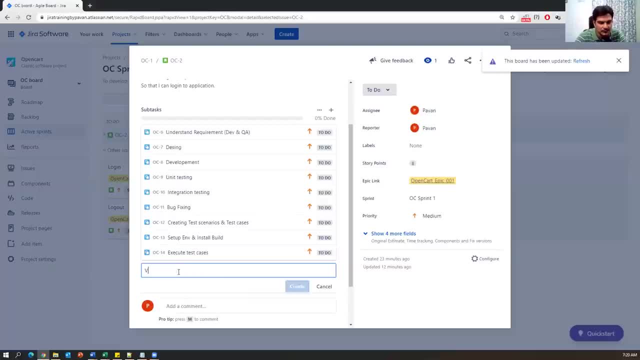 cases and then verifying bugs. verify bugs- right. so these are the qa tasks. so once we added all the development and qa tasks to this particular story, we can just close this. so developers and testers will do these tasks. product owner will not do this. product owner just will. 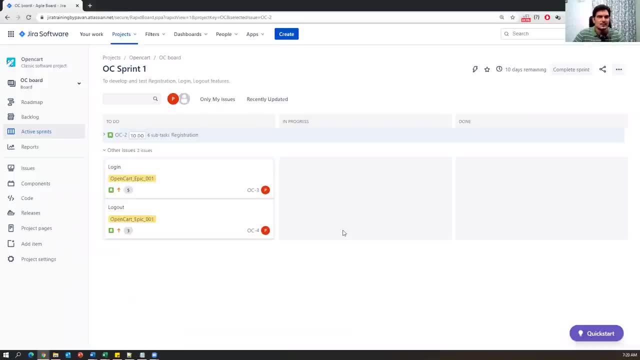 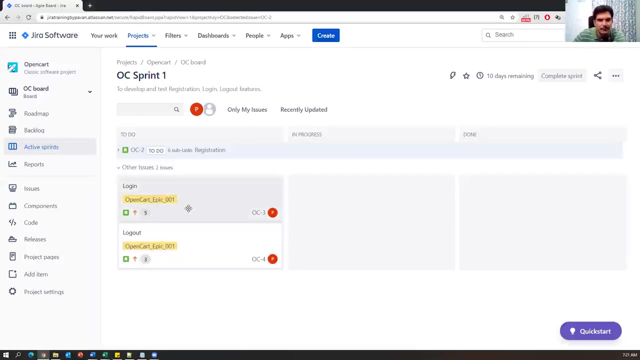 add the stories to the sprint once the sprint is started. that is again testers and developers responsibility. now we can just look at the scrum board. if i just look at this board and then we can add this expedition here, we will have also added the conversion to. 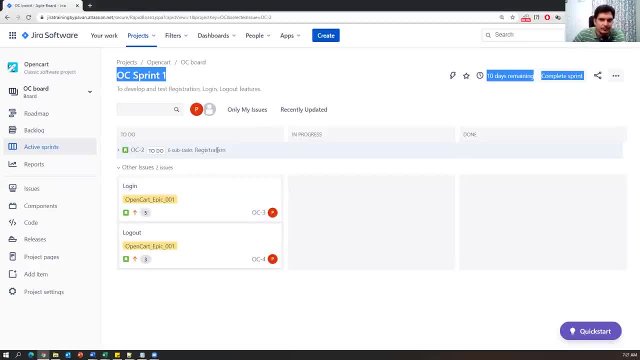 sprint story, we have added tasks, developer tasks and qa tasks. okay, so, once we added this, now we need to progress. so how we need to progress? so as soon as we have done this registration, suppose as a qa or dev, we have done this task, for example, or this task is in progress. 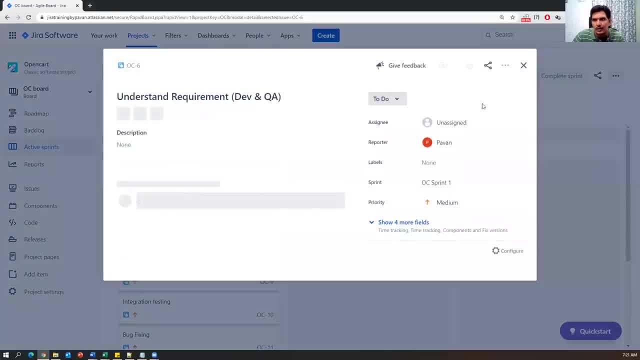 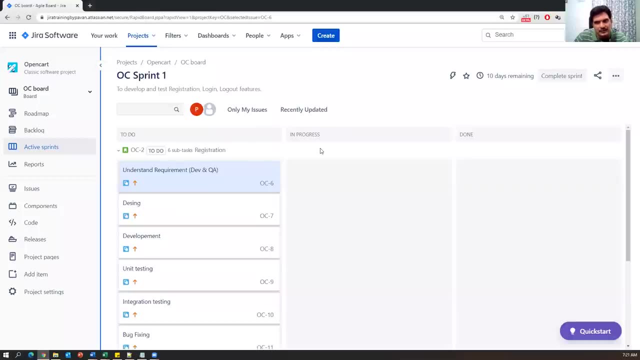 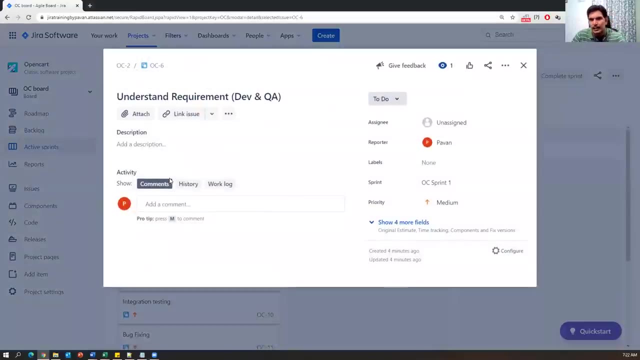 then we have to move it into the progress slowly. we have to, we have to drag it just a moment, so we cannot directly drag this. we can only drag the stories, not the tasks. so what you have to do, as soon as we completed this story, we have to just click on this, okay, and uh, there will be something. 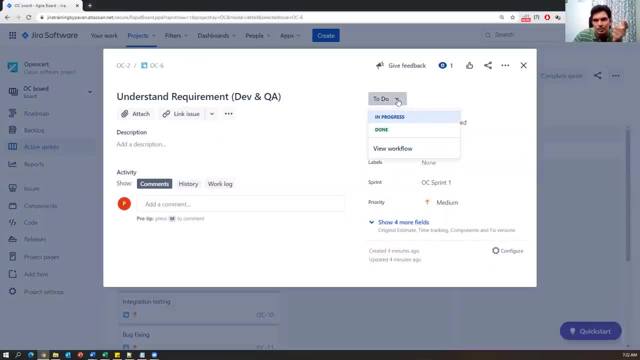 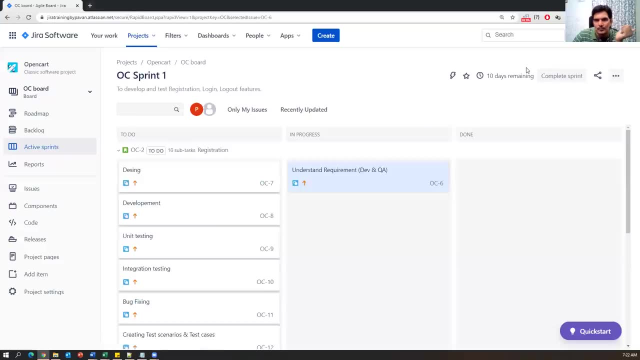 called to do. you can see the status is to do, right. so if you want to put as in progress, you can just put in progress, okay, and then say close. now it is automatically more to in progress section. the task is more to in progress, right understanding. i want to put in progress. 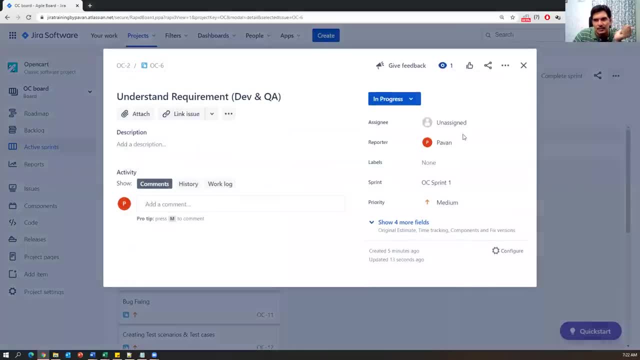 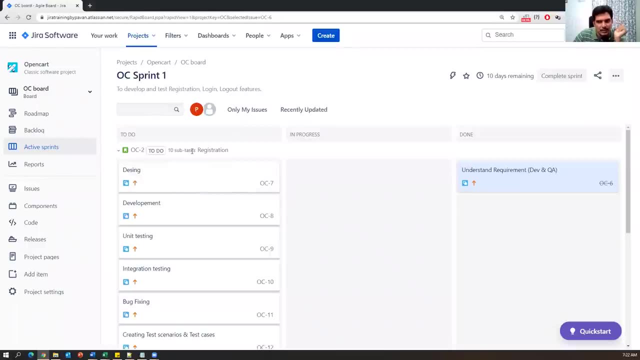 once it is done, once it is completed, again click on the same thing and you can change the status. so done so, let's say close. so now it is more to downstairs. so for this particular story, understanding requirement by dev and qa is done, so we have moved it to the done so one. 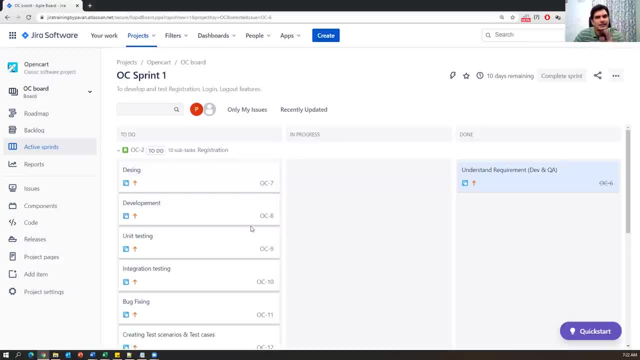 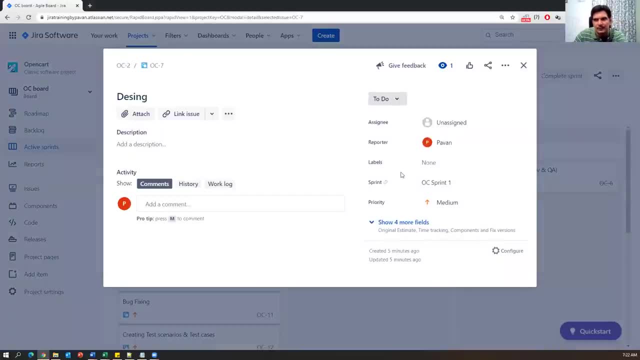 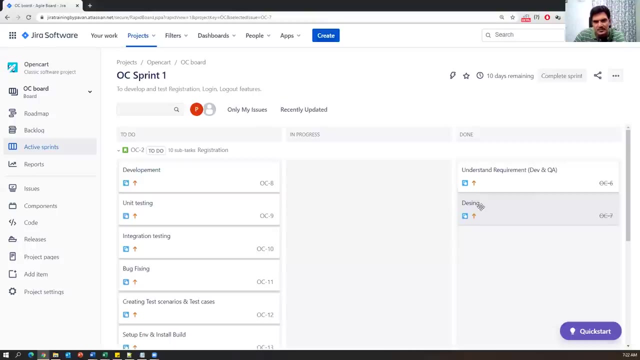 task is completed. further story now. development testing task will go parallelly, right, so what we can do? development, uh, design part. so developer will complete the design done. okay, now the design is completed by the developer. now, once the design is also done, development testing activities goal will go parallelly. so both the tasks should be in the in progress. so 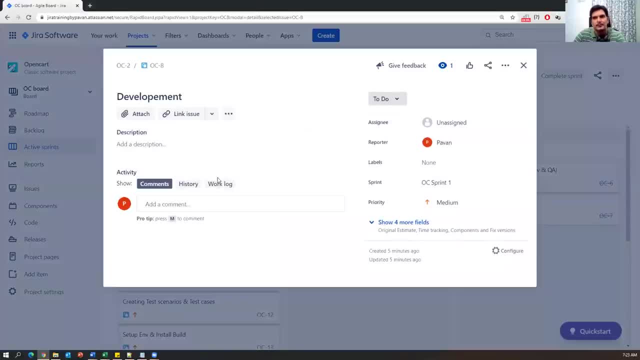 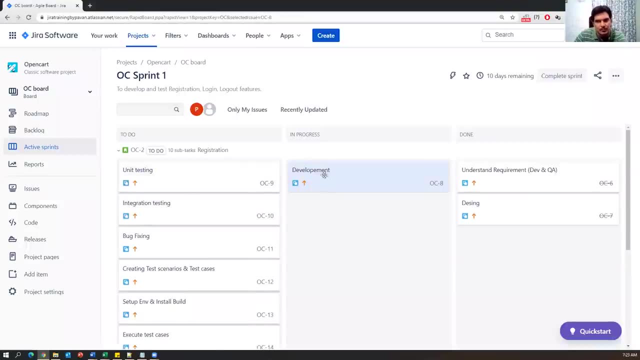 how we can change it. so development is in progress now. currently developers are developing the software so we can put in the in progress and developer will update the status on day-to-day basis. now development is in progress. parallelly, our testing should also in progress, as per testing. 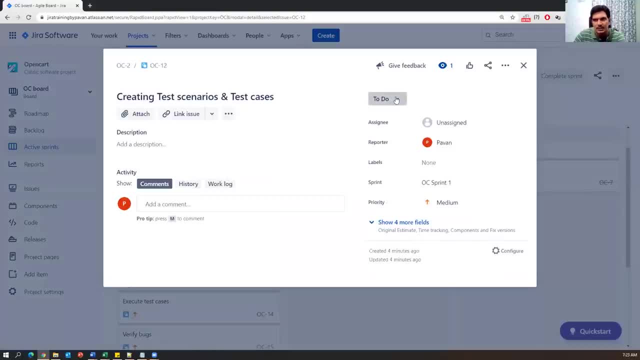 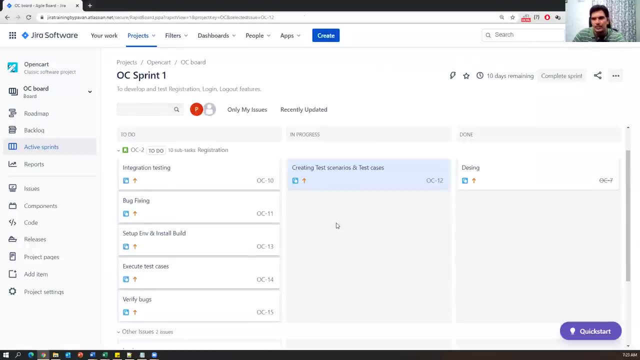 what you will do: creating the test scenario as a test scenario. so tester will update this tester what he will update in progress. so once you click on the in progress and then close it, so now you can just look at here development and test scenarios and test cases from qa said these: 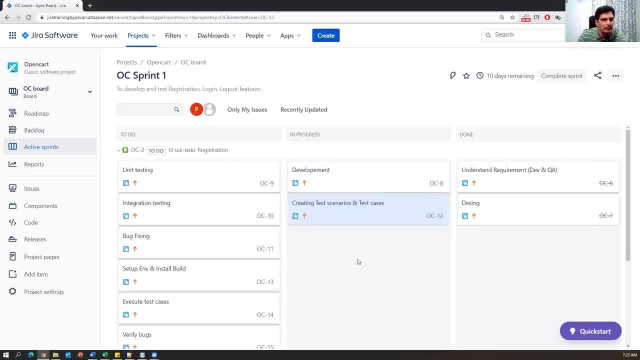 two tasks are in progress. so scrum master will manage all these things, guys. so come master, every day, look at this particular scrum board and check how people are working and how people are progressing. what are the tasks that are in progress? what how tasks are completed or done so? 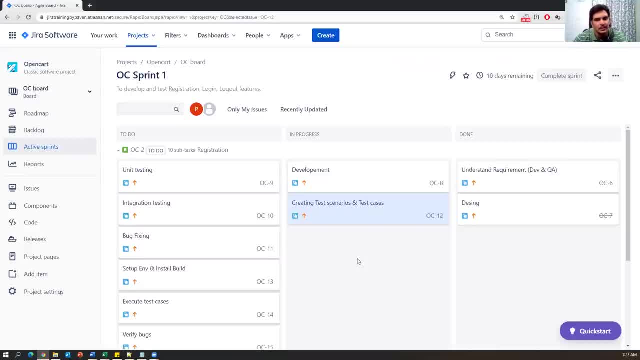 okay, if there is any delaying in scrum meeting or scrum call, they will discuss. so once you added all the tasks, this is a developer and tester responsibility to complete these tasks which are created for the story. so once all the tasks are completed for this particular story, then we 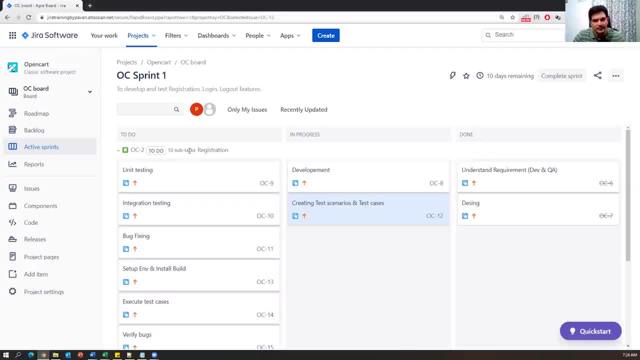 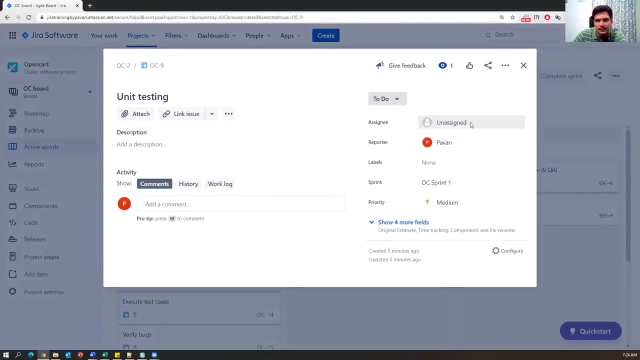 can say the story is completed, the story is done. now let us assume, let me complete all the tasks, so you can just say unit testing, right, so unit testing, click on the unit testing. let's say developer is done. you can, just, you can also assign here developer, suppose. 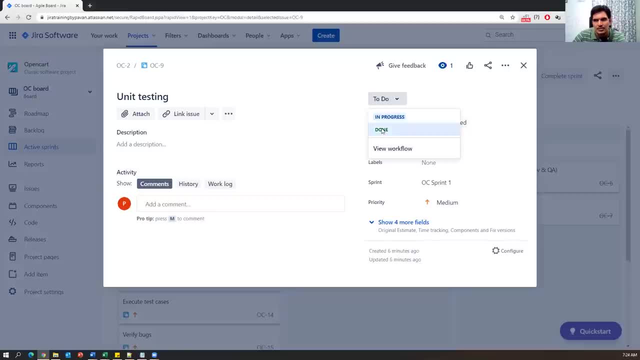 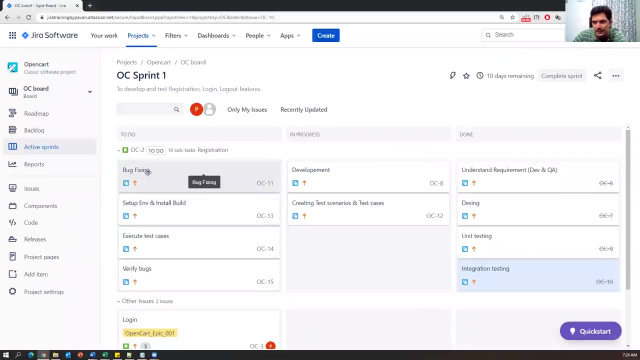 at the time of adding the stories itself. we have to select the assign here. so i said done. so unit testing is also done, so integration testing. so integration testing is also as updating as a done. and then these are all queue activities. so let us see development activities. 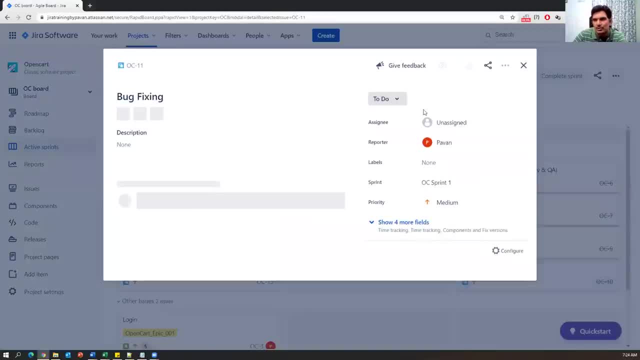 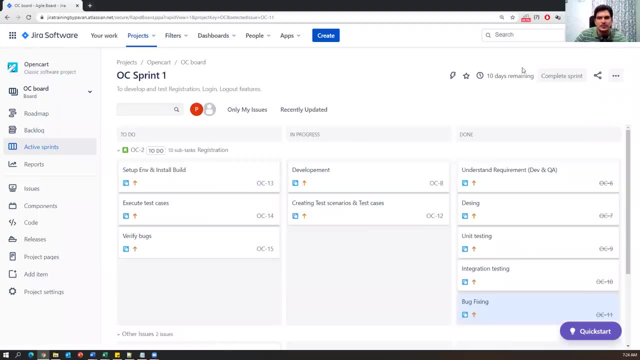 are done or not. so bug fixing is also developer activity, so this is also done. so to complete the story. first of all, we need to complete all the tasks which are associated to that particular story, and so development tasks are done, so now only qa tasks are pending. so now i am also. 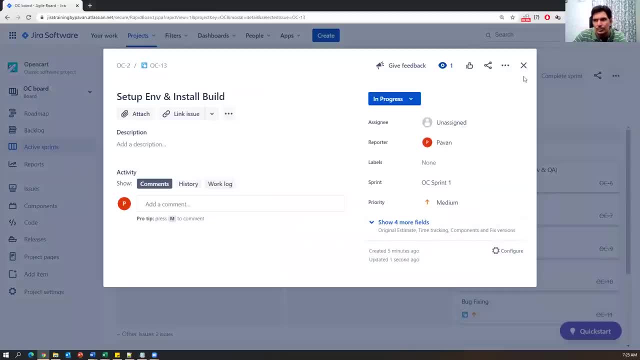 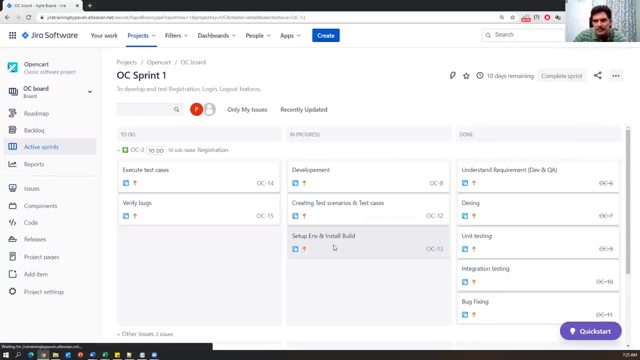 progressing so you can update in progress. if i say, which will go to the second section, so set up an environment installation build is in progress, and then again, if i just click on this, i can just finish this, you can say done and close it. so now it will go to done state and. 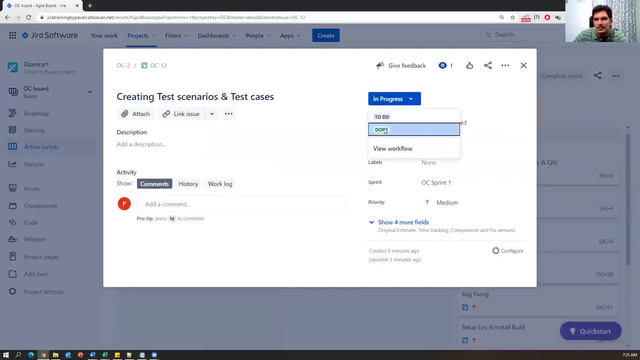 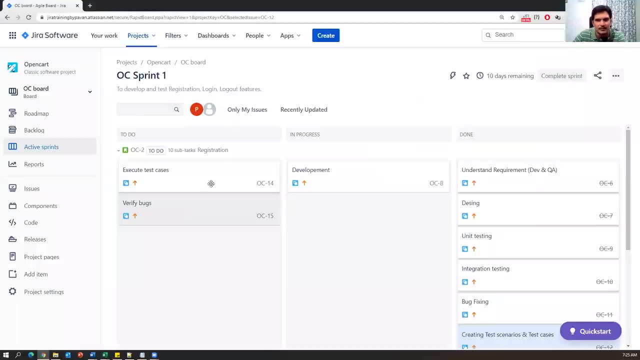 creating the test scenarios of test case are also completed, so you can just say done and say close and automatically go to done state and two tasks are pending: only executing verifying box and test case. execution is also completed. then you can say done or if it is in progress, you can say it's. 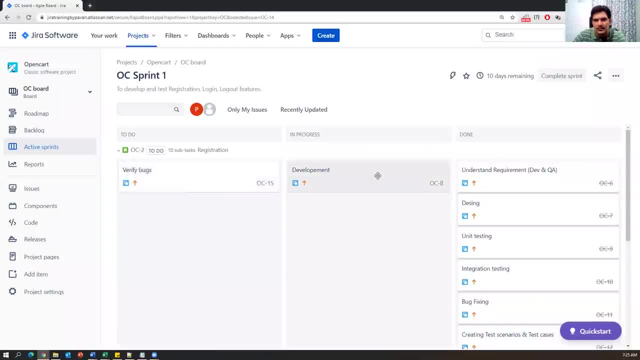 progress. then what is the final task is pending? is development is also completed? right, so you can say is done, move to done, state so all the tasks have completed except the verify box. so to close this particular story, or we can say to done for particular story, all the tasks should be completed. 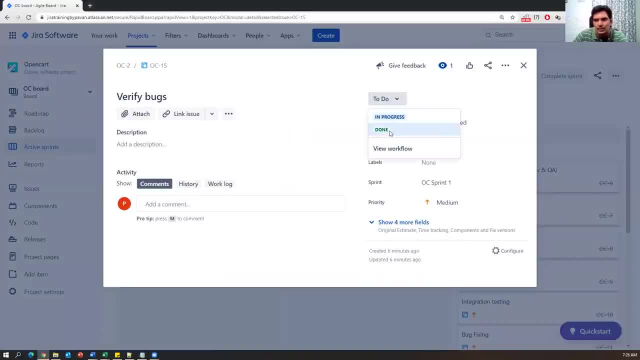 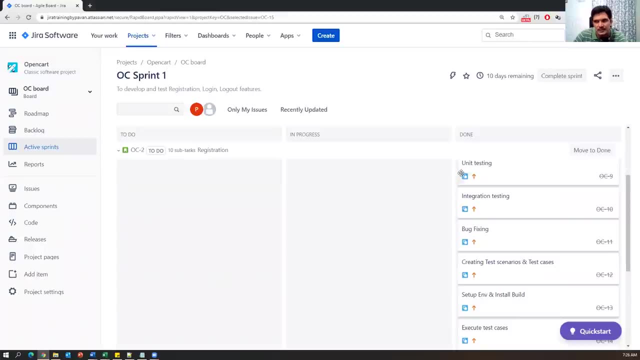 so, if i just look at here again, this is also should be closed- done, so now we can just look at. for this particular story, there are no tasks are pending, so these tasks will be updated on day-to-day basis based upon your progress. so now, now it is done, everything is moved to the done. okay, now finally, what we can do. we can move this. 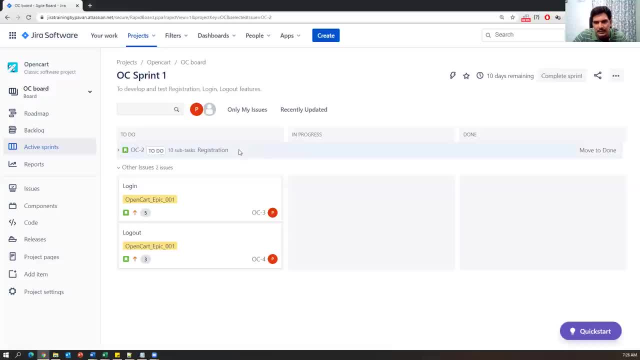 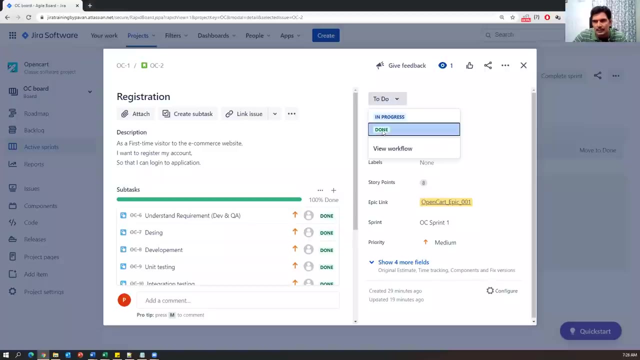 story to the done state. that means we can directly drag this story to the done state or we can click on the move to done. you can see here: click on this move to done, then automatically the story update. parent issue not required. so here we can say: done story. i'm saying so you can also look. 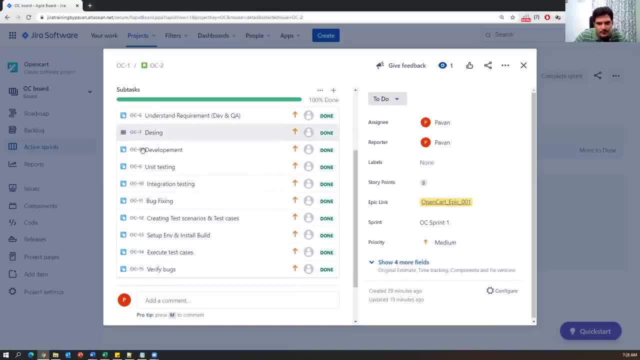 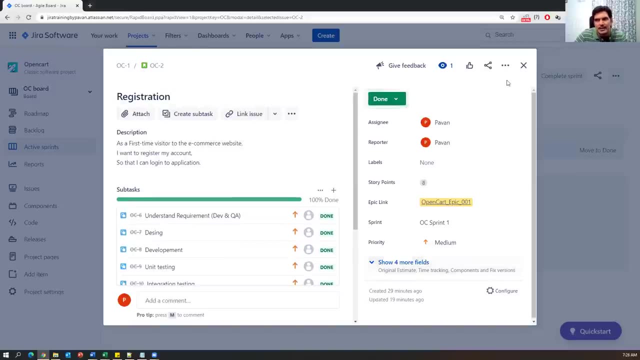 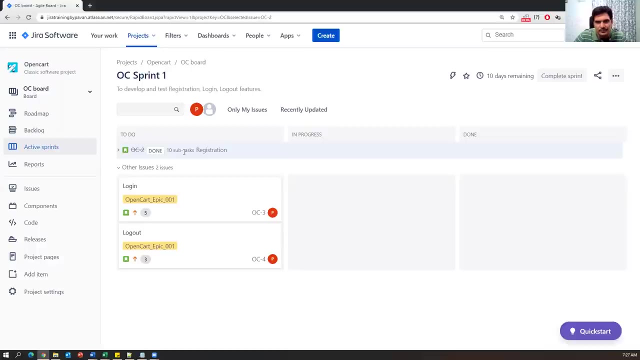 at here. all the tasks are crossed here. that means what? all the tasks are completed, okay. and then we say: done so. once the tasks are completed, then we can say: the story is done. now we can see the story is crossed here. okay, so registration flow story is completed once you done all the tasks. similarly, 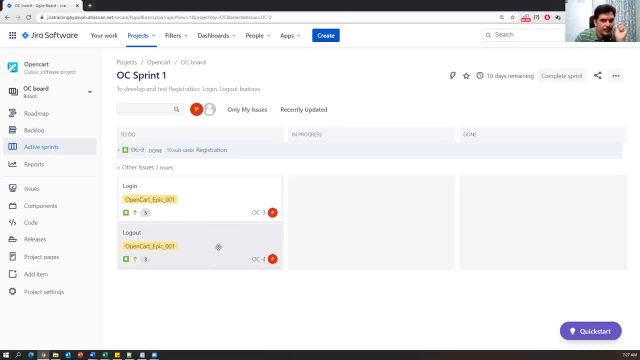 the same thing will be done for every story. same thing will be done for every story simultaneously. Similarly, once all the stories are completed, all the stories are in done state. then we can say: within the sprint duration we have to complete this Suppose if there is any story which is not completed in that particular sprint. again, 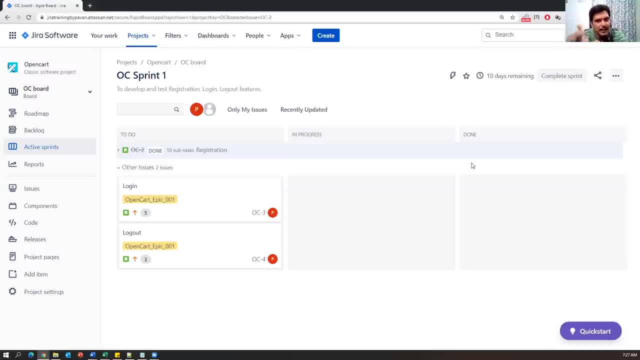 that we will replan for the next sprint. Okay, we can add the same story for the next sprint if it is not completed Or if there are any bugs which are not fixed in the sprint one, those bugs also we can create as a task. we can add them into next sprint. 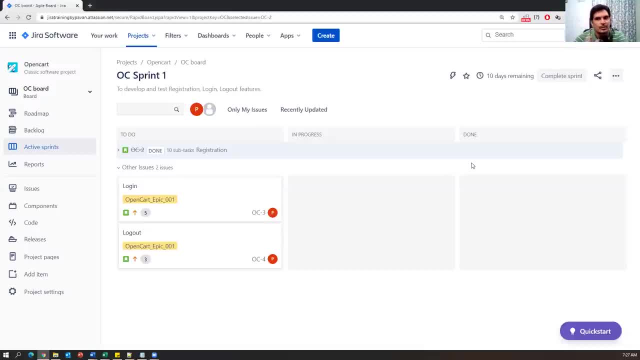 Okay, this is again continuous process. So once all the stories have been completed, first it will come to in progress, then it will come to done. So once it is done, your cycle will be completed, your sprint cycle will be completed. 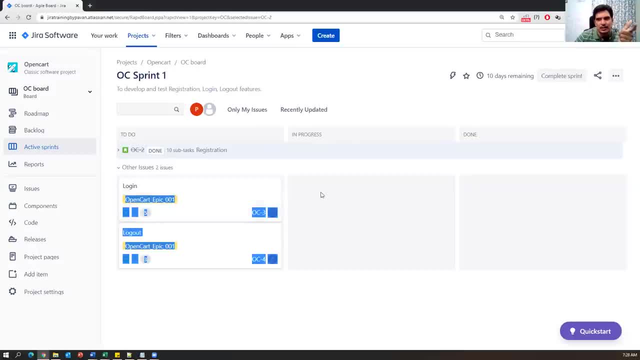 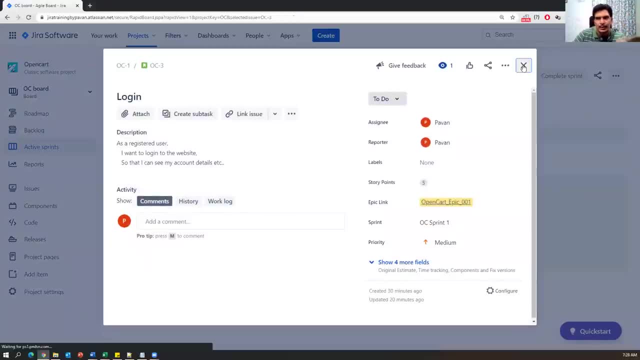 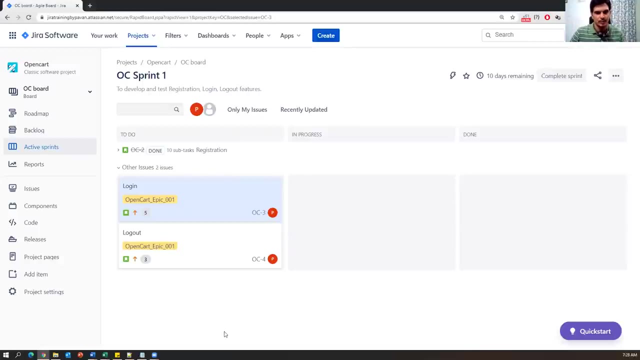 So now we can just look at here: registration is completed. I say login, So login, we need to add task first of all. okay, without adding task, without complete that, we don't do any activity on the story. This is called as a scrum board, which will automatically provided by the Jira tool itself. 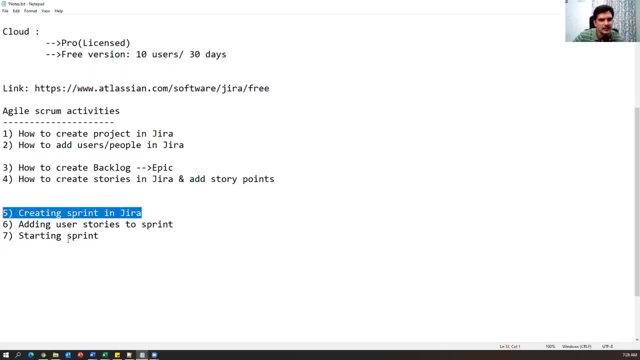 So what we have seen so far is: we have seen how to create a sprint, how to add user stories to the sprint. we have started the sprint And also we have added the subtasks. Also, we have added the subtasks and added the subtasks to the story. 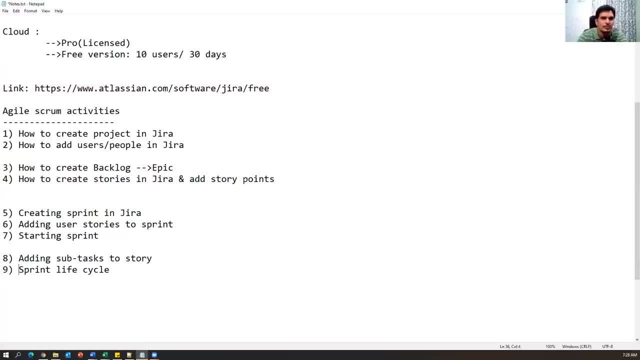 And also we have added the subtasks to the story And also we have added the subtasks to the story And also we have seen sprint cycle like to do in progress. done So, each story will move on to the different cycle. 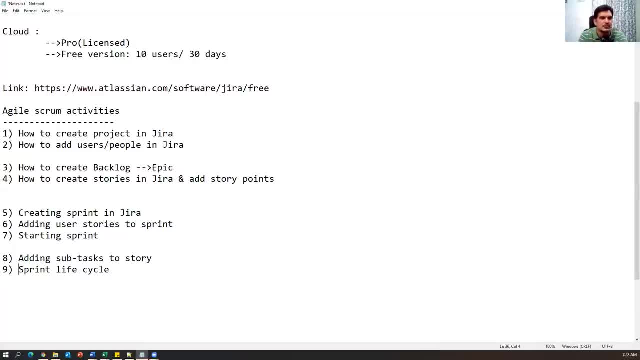 So different stages, sorry stories, stories within the sprint will move to the first to do state, then in progress, then done So, to move the story one stage, another story. first we need to finish all the tasks which 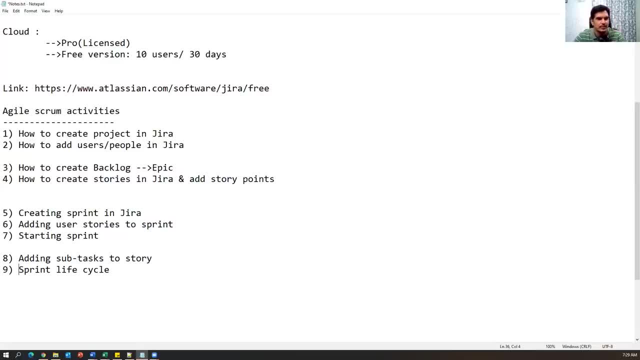 are defined for that particular story. Okay, so these are the activities we do finally suppose if you found any bug in the particular story. So if you found any bug in the particular story, then how we can report the bug? then simply just go to the create. 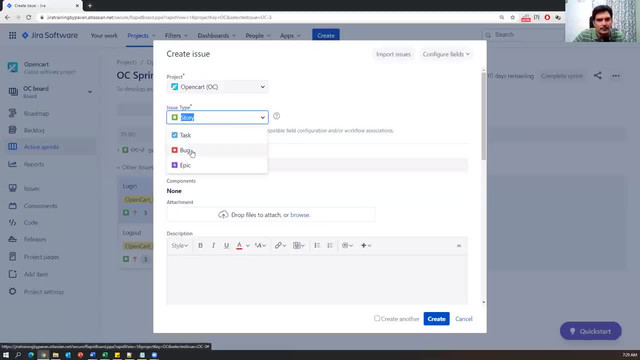 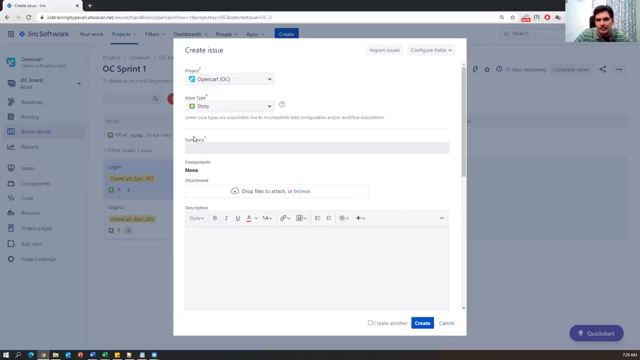 And here, instead of story and tasks, select the bug. So, once you selected the bug, this is a bug actually. So, once you selected the bug, just a moment Right. so create- And this is the project I'm going to create- a bug. 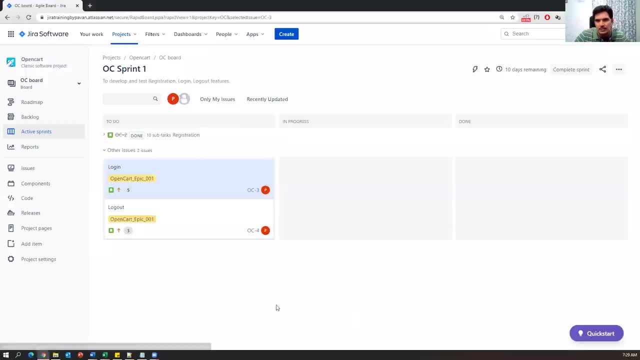 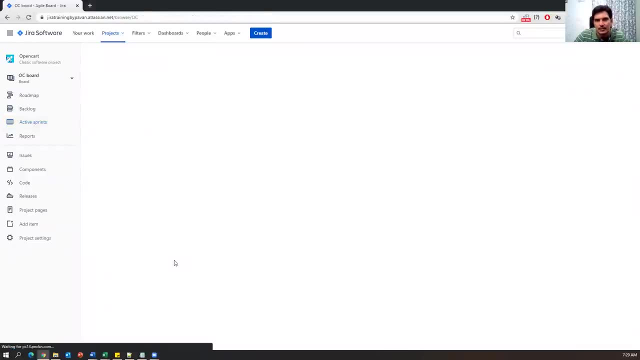 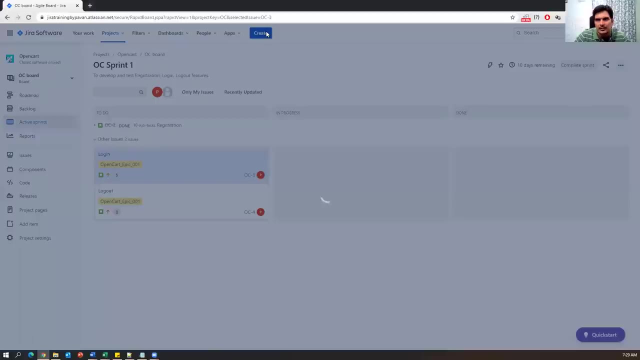 It should select actually. Okay, Just a moment. So let's open the project once again, refresh the page. If something is not working, sometimes it is not responding properly. All right, So now we can just go to create, and here issue type is story, and just selecting the bug here. 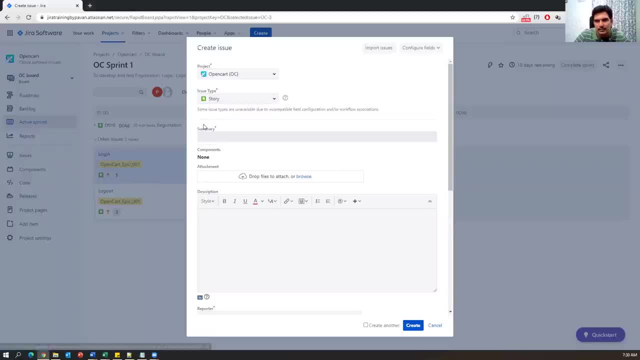 Sorry, it is not selecting. Actually, it should select the bug. This is a problem with the browser. See this. It is not. It is not selecting the bug Task. also, nothing is selecting. It's just selecting only story. Okay, 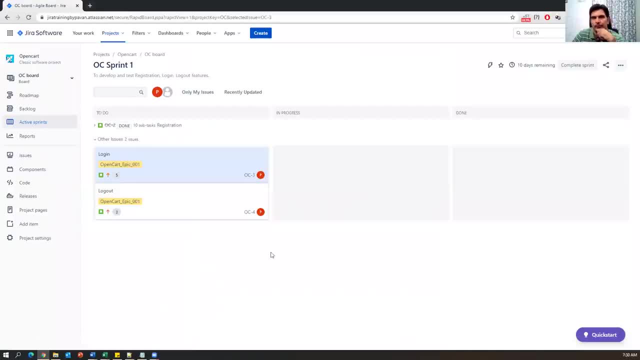 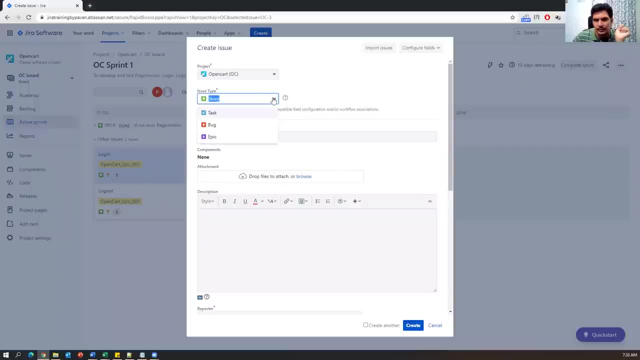 So what we can do is One sec. Okay, So here. we are not able to select any bug here, because this is a small problem with the application or UI It is. I think it is a problem with the UI browser, So I'll show you this after a few minutes, in a different way. 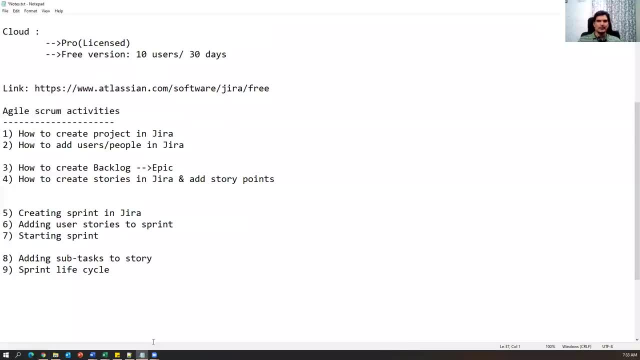 So this is how we can just Do the scrum activities. Okay, Because reporting the bug is again comes under the test cycle so that we will see a separately. So creating the sprint in Jira we have seen and add a user stories to the sprint starting sprint. 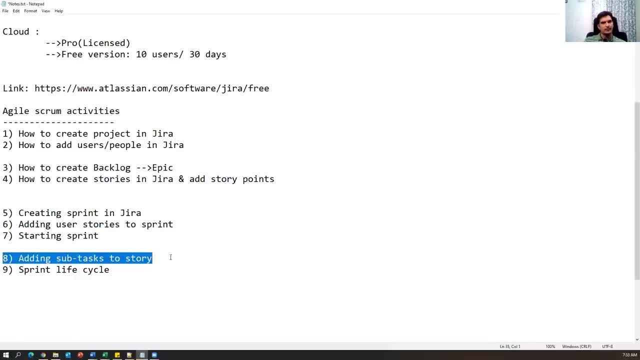 Then we also added subtask to the story and we have updated the status of the stories And, finally, we completed the task for that particular story and then we close the story. This is all about sprint lifecycle. Okay, so this is how we need to do the scrum activities within the Jira tool. 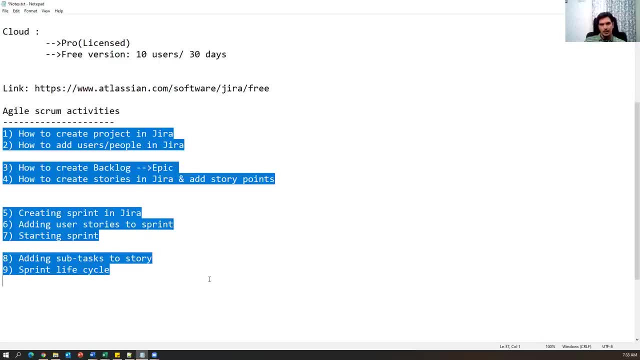 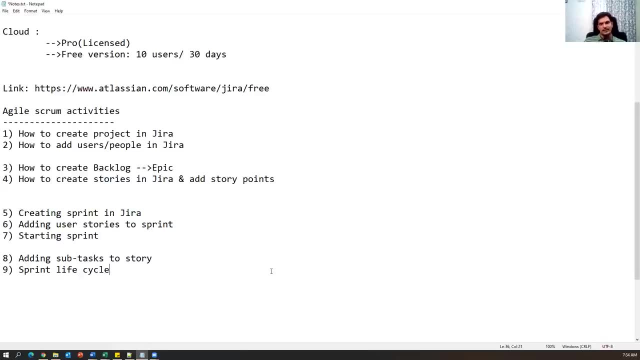 Okay, so apart from this, we also can do test management activities, like we can write a test cases and we can create a test cycles. we can add the test cases to the particular cycles, we can update the execution status, we can report the bugs. 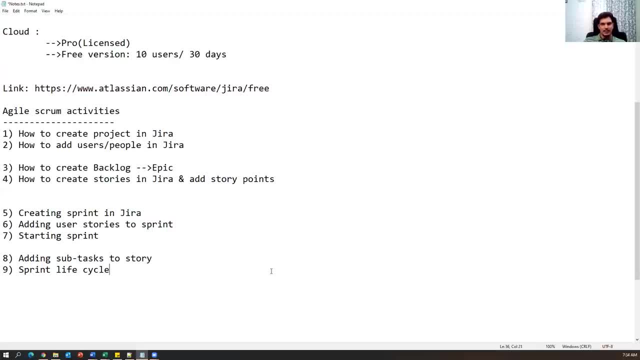 So these things are comes under the test management activities. That is the next activity. Okay, So this is how we need to do the test management Activities, But by default, Jira will not provide you these options. test management activities: to perform test management activities. 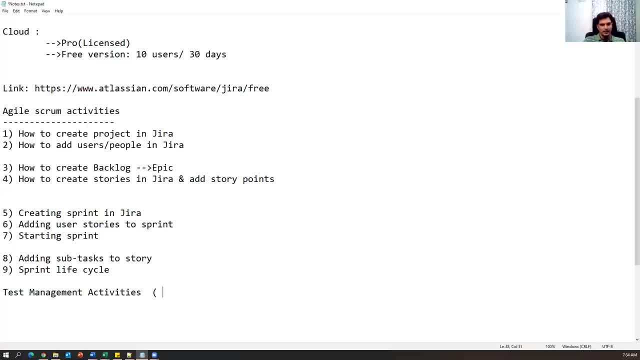 So we have to install a special plugin called Jeff fire plugin. Okay, so this is a new plugin which we have to install to perform test management activities. Okay, so that we will see now. So now let us start test management, Okay. 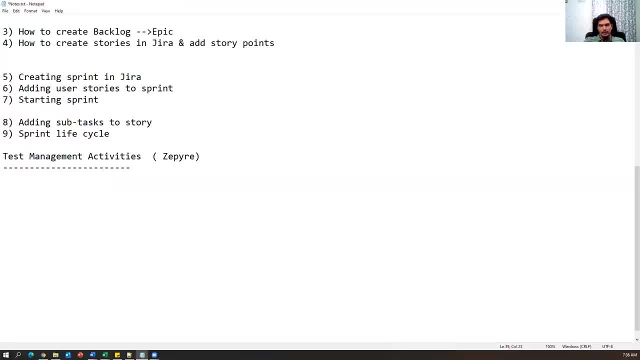 So what are the test management activities? we do normally in the test management activities we will write the test cases. Okay, or suppose you already written the test cases in Excel sheet or Excel file? we can directly import all the test cases into Jira, so we can write our own test cases directly in Jira, or we can import the test cases from Jira, so test cases we can write. 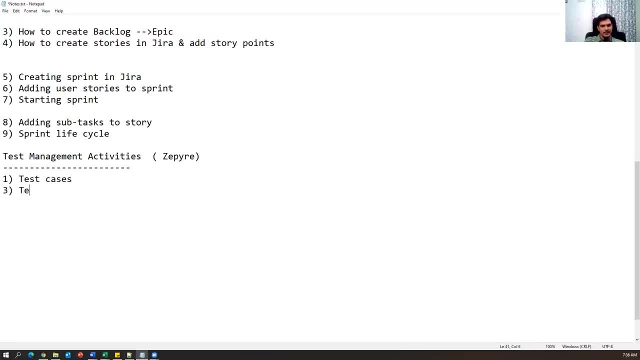 And what else. we create the test cycles. So what is the test cycle means? The test cycle means We can say regression test cycle or functional test cycle or sanity test cycle. So each cycle we will add some number of test cases and we'll execute the test cases in that particular cycle. 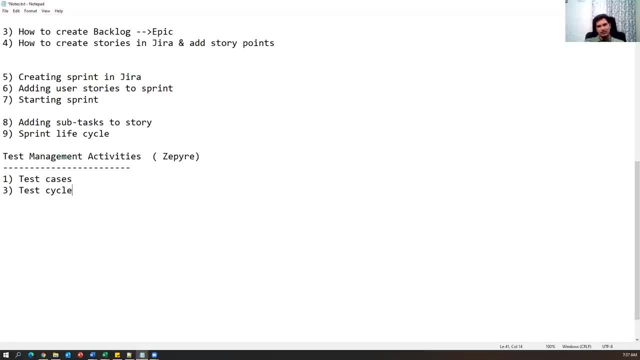 And then we report the bugs, if there is any mismatches between expected and actual, So that we should happen in the test cycle. So, creating the test cases, creating the test cycle And once the cycle started we will execute the test cases manually. 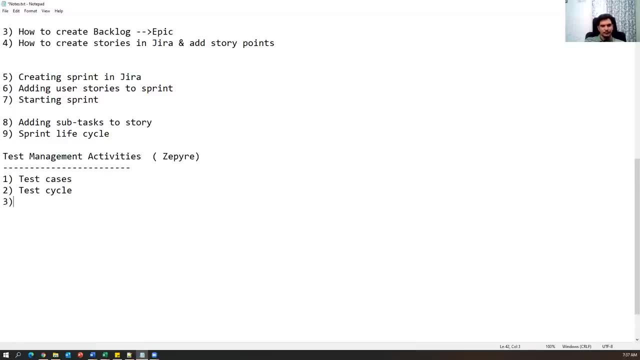 And then we will update the test cases. Update test cases passed or failed or blocked, Okay, and after that we can see the. we can also report the bugs. report the bugs and then we can generate the reports. So these are the main activities we'll do as part of test management. 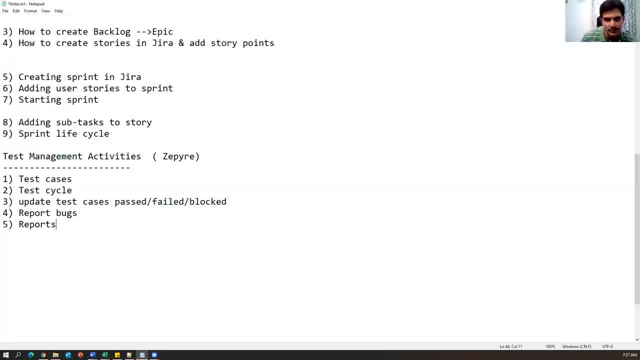 Right. So now I will show you how we can do these activities in Jira. Okay, So we can do these activities in Jira tool by using Jetfire plugin. So normally Jira don't provide any options to do this, So we have to install additional plugin called Jetfire inside the Jira. then it is possible. 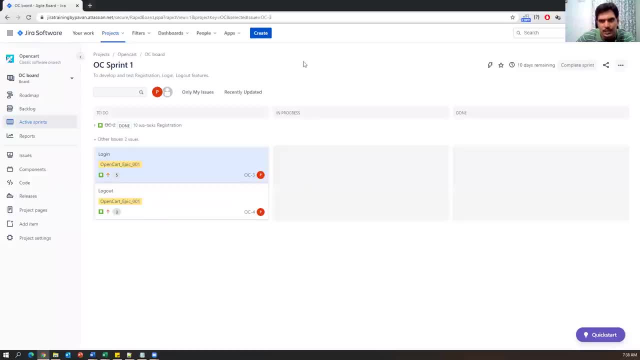 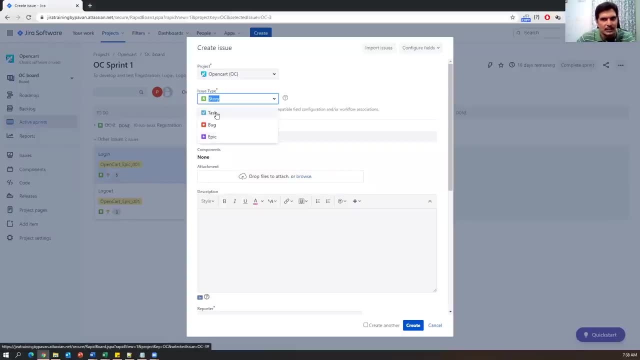 Okay, Now we can just look at here. go to the project And when you click on the create here you will see only three types here: Story, task, bugs task and epic. Nothing- Story, task, bug and epic. 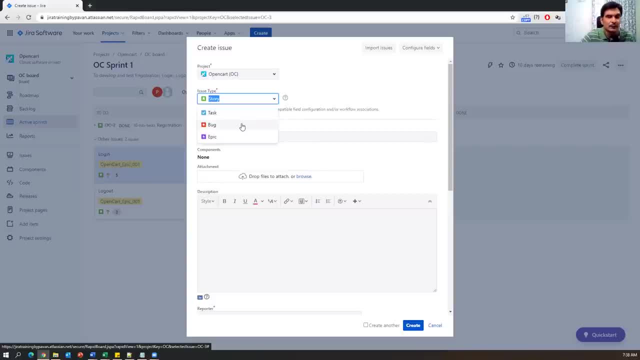 Only four issue types you can see. But if you want to write the test cases And test cycles, if you want to create, you have to see one more type here that is called as a test. So test the issue type you have to see here, along with the task bug and epic. 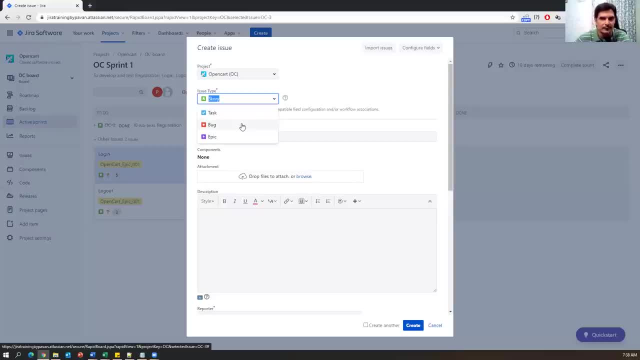 But by default it is not appeared here, because so far we haven't installed Jetfire plugin. So now I'm going to install Jetfire plugin and then we will see one more task you will get here, So cancel it. So how we can install Jetfire plugin. 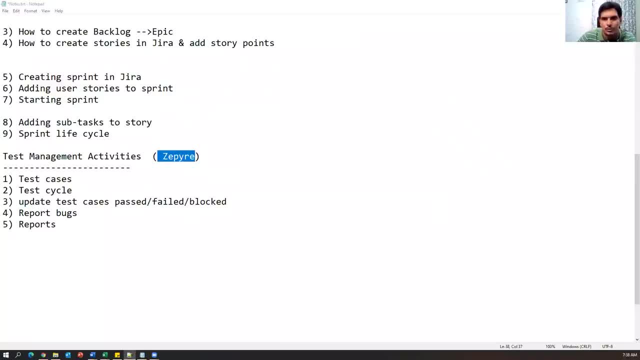 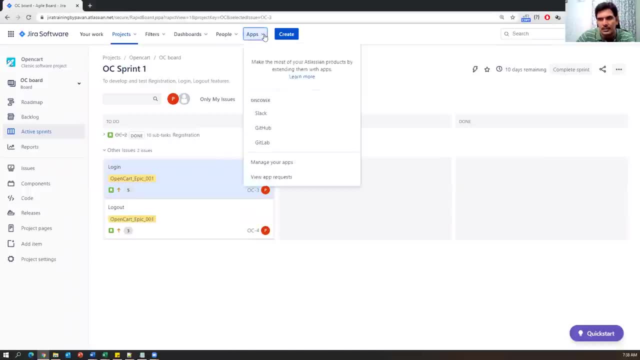 So to install Jetfire plugin first we need to go to apps section in the Jira tool. There is something called apps menu Here you can just look at, go to apps And you can just say: find new apps, Click on this. 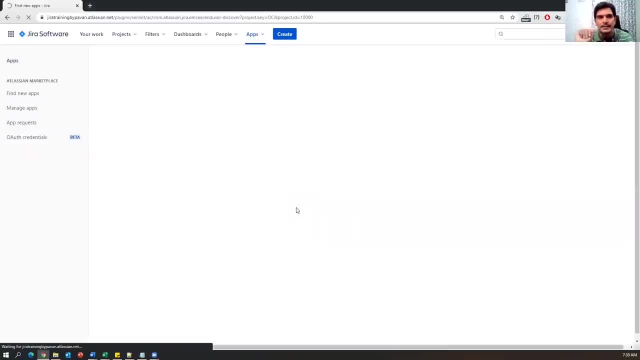 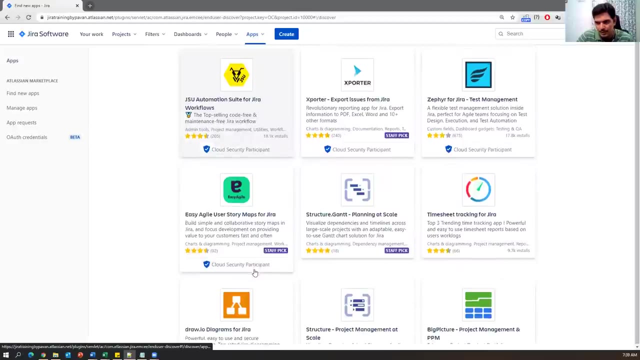 Find new apps. So inside this find new apps, you have to search for Jetfire. So once it displayed everything, you can search for Jetfire. So these are the different plugins which are supported in Jira tool. Now we are searching for Jetfire. 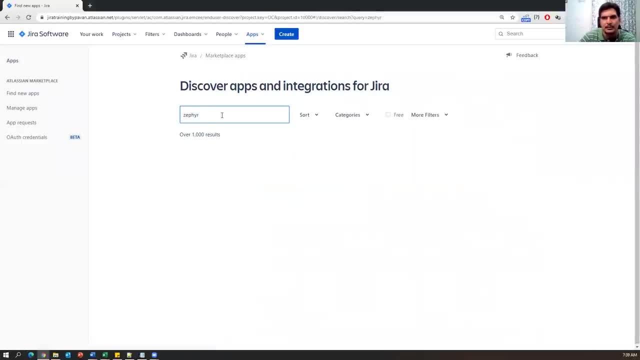 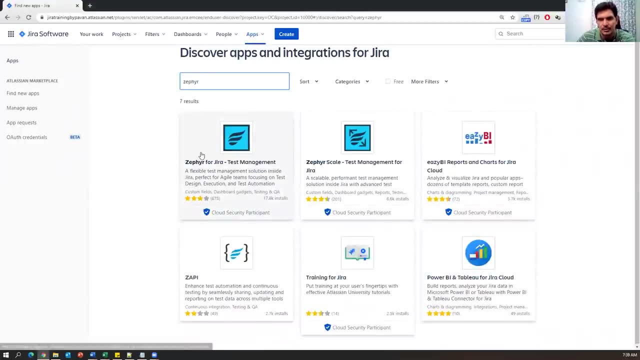 And once you type Jetfire, just press enter. Now we can see multiple plugins, So this is the first plugin which we have to install. So Jetfire for Jira test management, So a flexible test management solution inside Jira, Perfect for agile teams focusing on the test design, execution and execution. 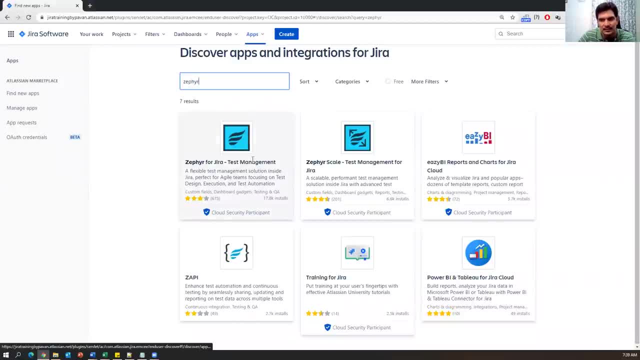 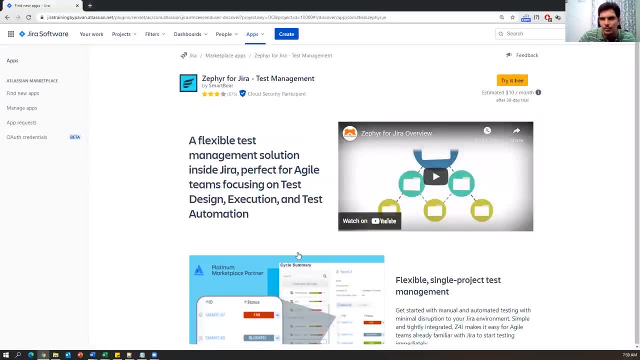 And test automation and so on. So we have to just select this, click on this. So once you click on that app or a plugin, which will go to another screen And this is again free for one month. 30 days trial is there. 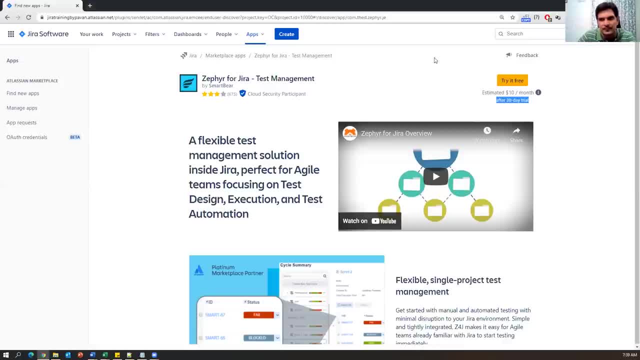 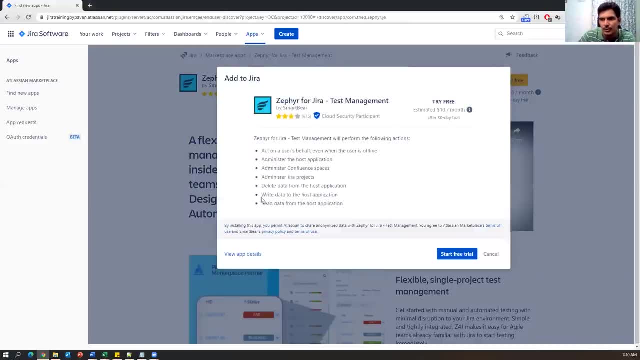 After 30 days, which will expire This particular plugin. So now we can just click on try it free And once you add this plugin so, which will show you all the information about this, Then say start free trial. Click on start free trial. 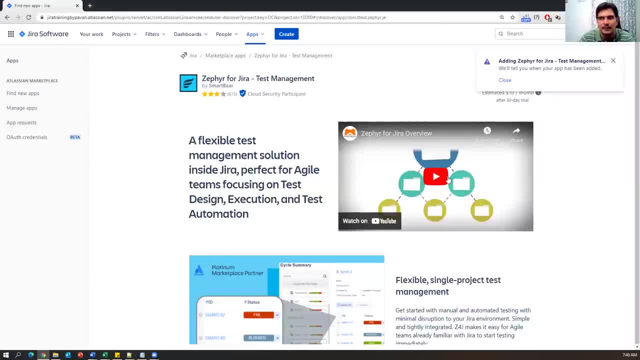 And then which is adding Jetfire plugin into Jira tool. So once it is added successfully, then we can do test management activities. So once it is done you can just close this So you can say: we will tell you when your app has been added. 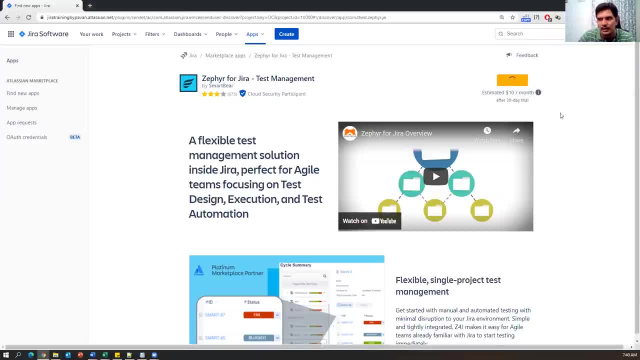 You can just close this Now it is see it is trying to add the plugin into Jira tool, So still it is in progress. So once it is done Now we can get the success message. Jetfire for Jira test management was added. 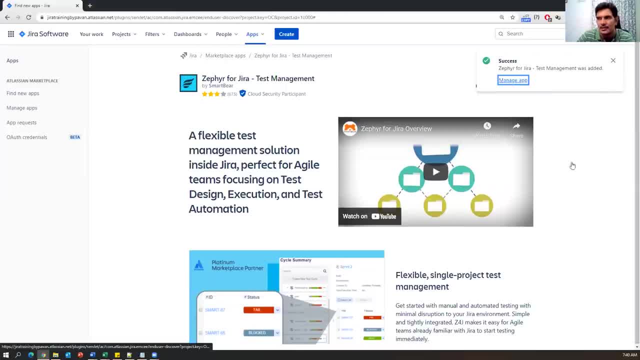 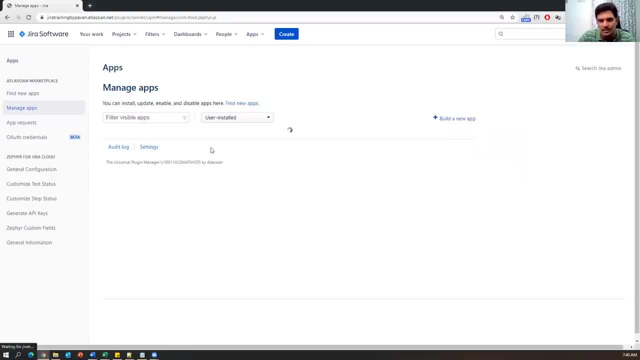 So once you have done this, you can just go to manage app, Click on manage app and which will show you again all the different apps which are installed in Jira. tool Not required Now. just go to Jira software logo and it will go to homepage. 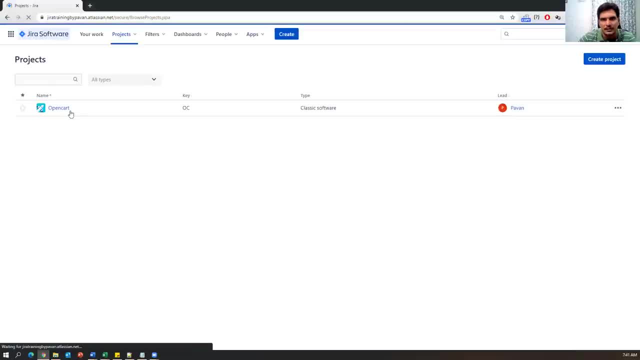 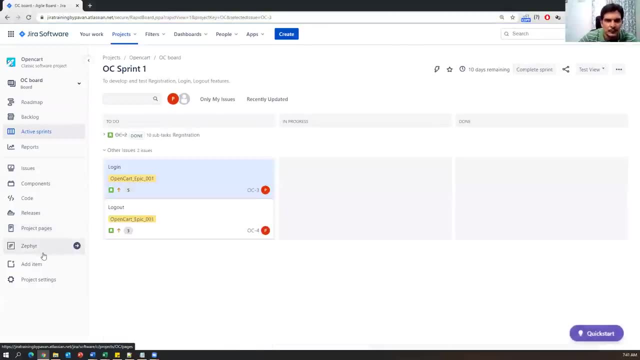 Now observe this: When you click on the Jira software here, your project is showing. Click on the project, You will see the homepage again. Now observe this: Previously we don't have this option- Jetfire option. we don't have previously. 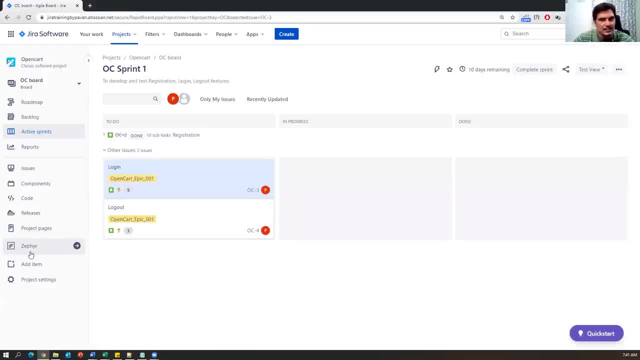 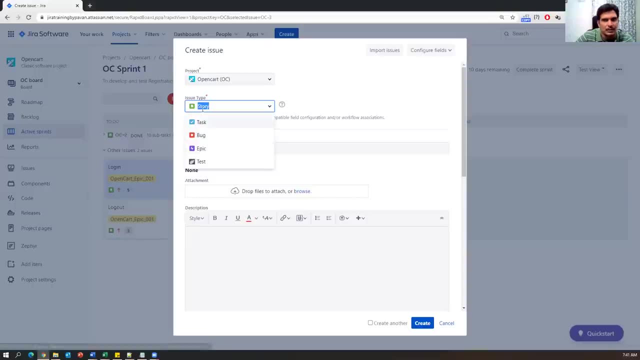 Now it is added here. That is the one change. The next thing is: previously, when I click on the create, we can see only task bug and epic story Test was not there. Now we got additionally test option. Okay, Additionally, we got the test option. 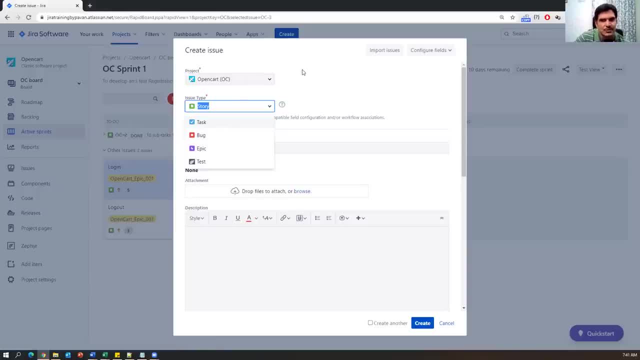 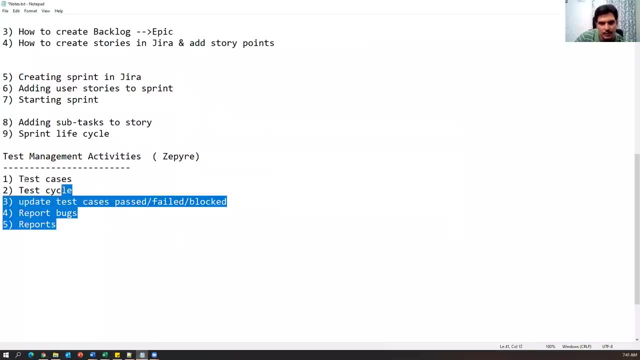 So these two changes you will notice after installing- After installing Jetfire plugin within the Jira tool. Okay, So once you have done this, then we can do test management activities in Jira tool. Okay, Now let me show you how we can do this quickly. 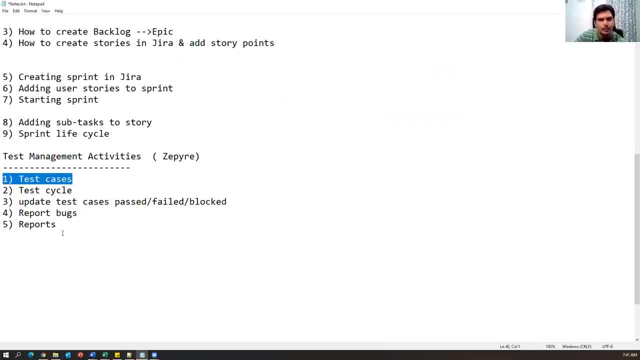 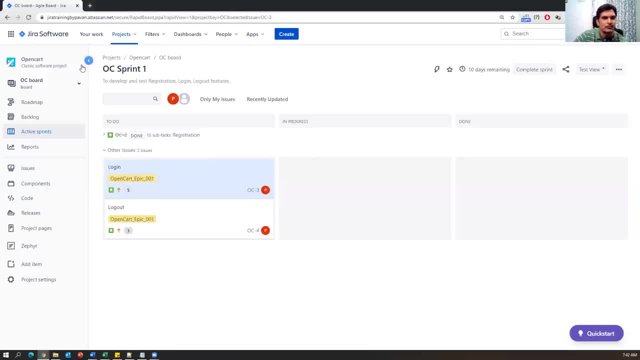 Very simple and very easy also. So first let me show you how to write the test cases. So to write the test cases first we need to go to Jira here. So these are all options which are available for agile or scrum process. 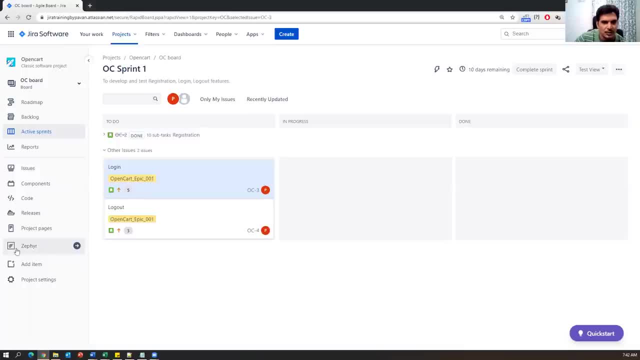 But if you want to do the test management activities, we need to click on Jetfire. We need to click on Jetfire option here. Click on Jetfire Then it will give you few more options And there are multiple sections are there? 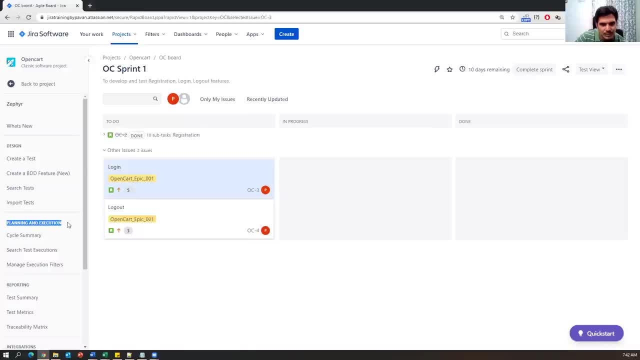 So you can just look at design section, planning and execution and reporting And then integrations. There are multiple sections are there- And design section: mainly we create a test case and BDD type of test case And we can search the test which we have already written. 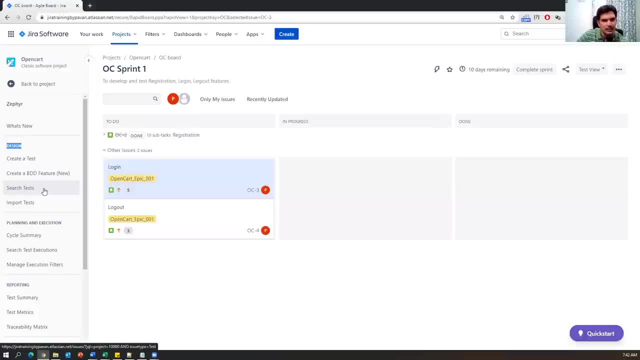 And if you have test case in some Excel file or some other sources, we can import those test cases. So these things we can do as part of design part, And planning and execution we can create as test cycles. We can execute our test cases. 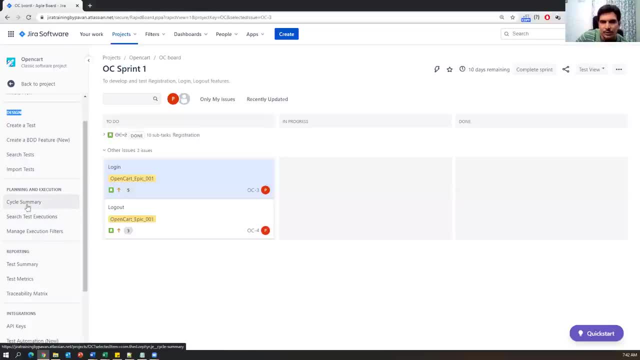 And we can also update the status or pass or fail. So these things we can do as part of planning and execution And after execution is completed, we can see the reports: Test summary report, test metrics, traceability metrics. So these things we can see as part of reporting. 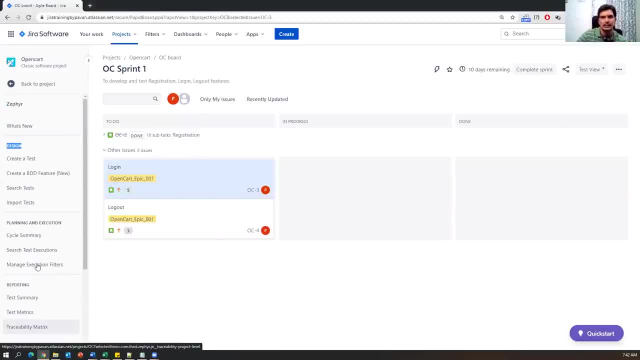 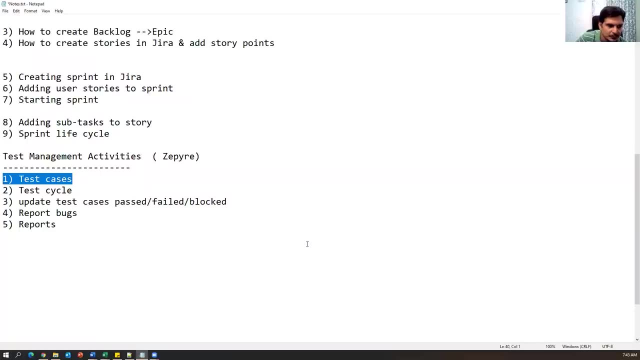 These are the things as possible through Jetfire plugin. So now I will quickly show you how to write the test cases And two ways we can do this, guys. One thing is: we can directly write the test case in Jira. That is one thing. 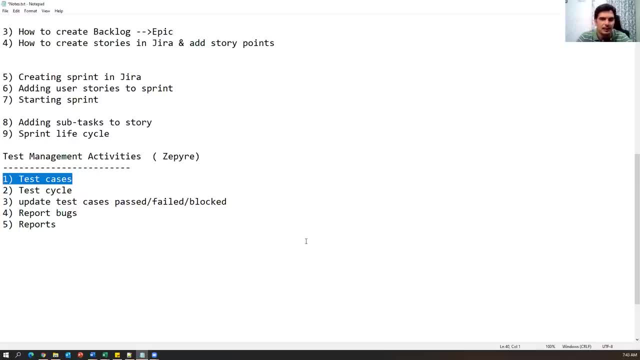 Or if you have written multiple test cases which are already there in Excel file, You can import those test cases in Jira. You can import those test cases in Jira. So I will show you both the ways. So what we can do is go to Jira tool. 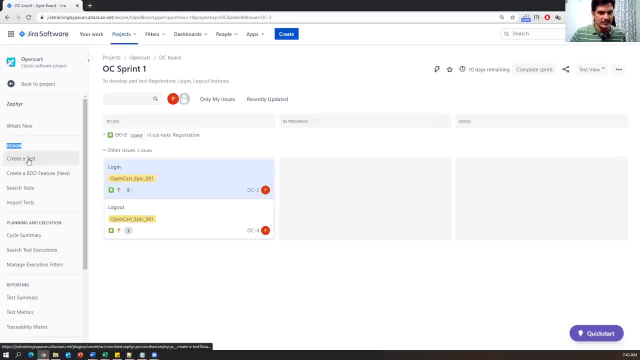 So how to create a test cases. So click on the create test. So how we have to navigate here From the main home page. Click on Jetfire plugin, Then you can see create test. So click on the create test And then you will get one more screen like this: 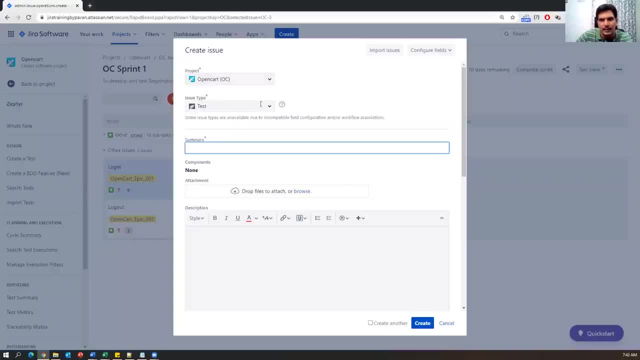 Inside this: this is a project name And issue type is a test. Issue type is a test by default selected. Now here we have to provide the test summary. Okay, Let me add one small test case. So here I have few test cases. 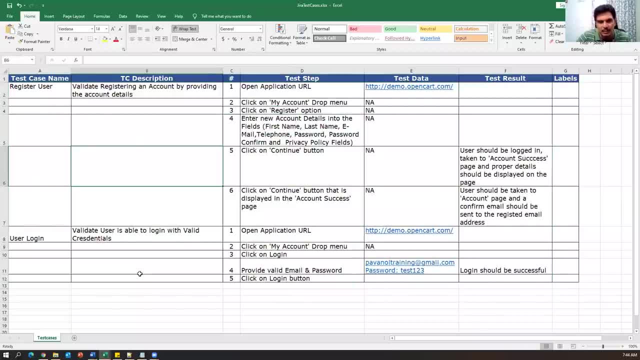 Okay, Now let me add one test case, Or we can also add one more test case, Or we can also add open card test cases, which we have already created earlier. So let me add one small test case here. So let me add one small test case here. 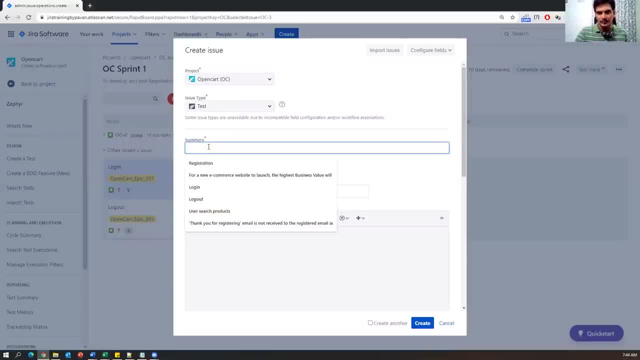 Some sample test case for registration. Or we can say: register user. This is a summary, Or you can just copy this summary as it is, Or else I will upload those test cases later And then scale them high. i'll try to show you a small test case, how to write the test case, okay. so here the summary is. 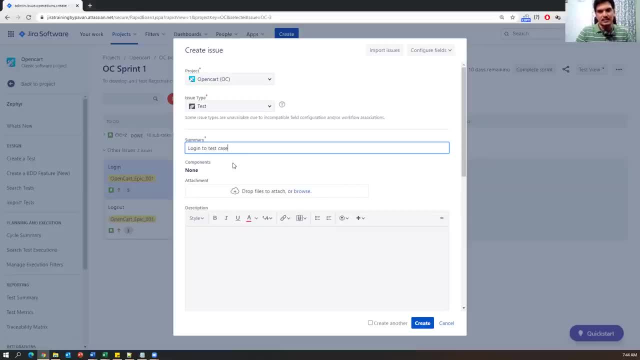 i say: log into test case. later, if you want, you can delete this, no problem. so log into test case. so log into application. so this is my summary of the test case and if you have any document which is required to understand the test case, you can upload and you can write the description. 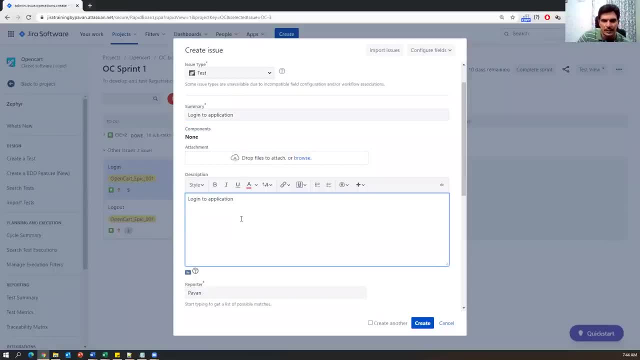 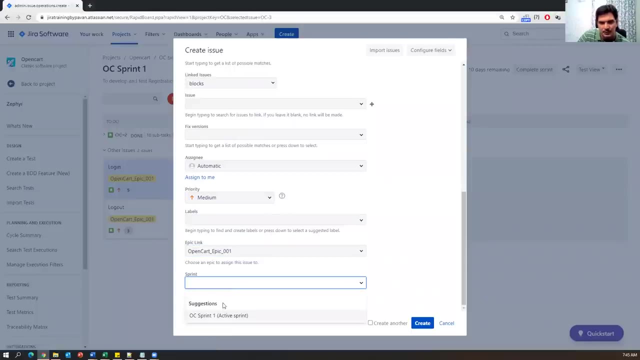 so log into application this small description you can provide and then whatever the information you want to add, you can add, like as any, who is responsible for executing test case and on for which epic you are creating and on which sprint you are planning. you can just specify that active. 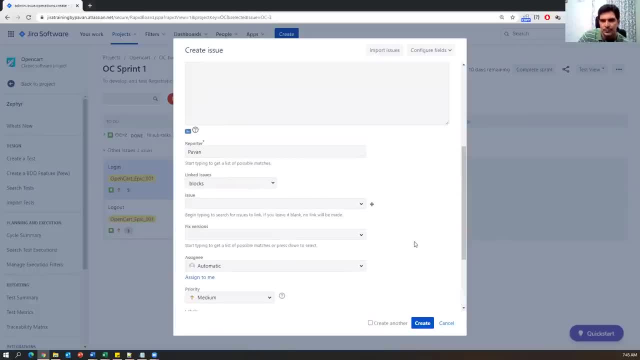 sprint or future print so you can also update these details later. so for now, just create a new test case like this. so, but test case means what we need to provide, the actions and expect result and everything right. but this one doesn't have anything, so where we have to update them, so we 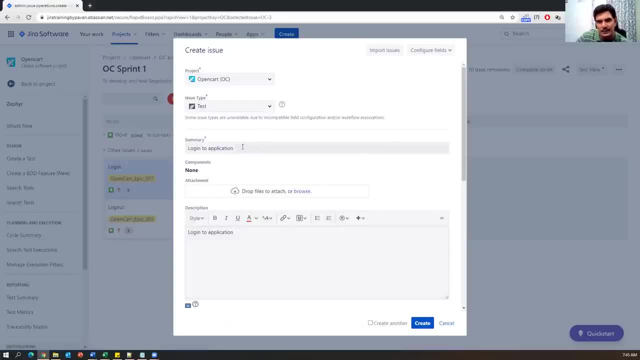 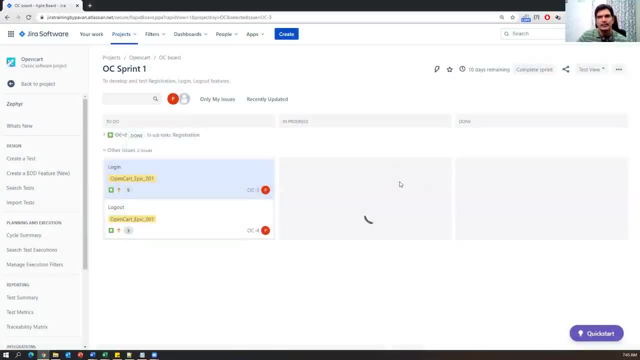 will update in the next video. next screen. so after filling the details- basic details, summary and description and everything- then we have to click on create. so once you click on the create, then the test case is created. just we need to click on this issue link. so your issue has been created but is not currently visible. 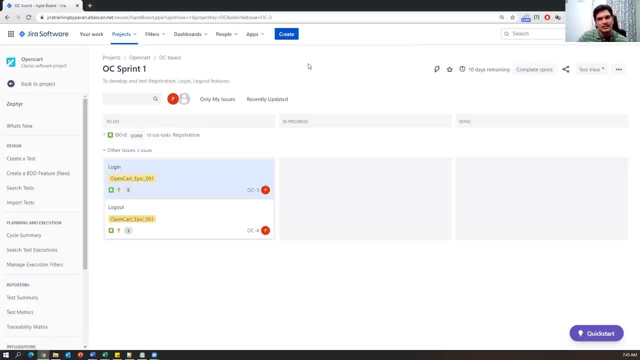 you can just click here or after a few seconds it will disappear. but where you can see the test case which is created, you have to go to search test. okay, click on the search test, then here you can see whatever test case you created. so this is a test case just now we created. 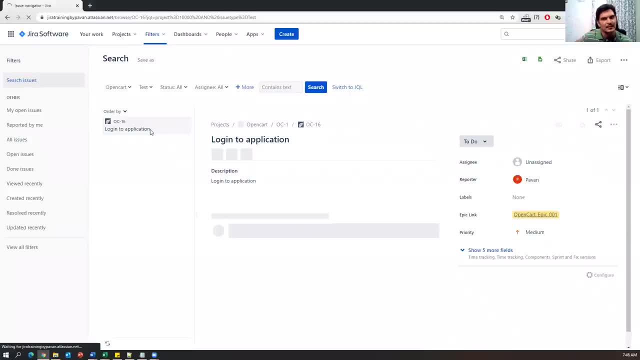 but we haven't provided any actions, expected results, priorities and everything right, so now we need to add them. so where we can add, just click on this test case link now it will show you this particular screen and here you can find multiple options. here: attachment, create a subtask link and jfair: actions and test details and test executions. 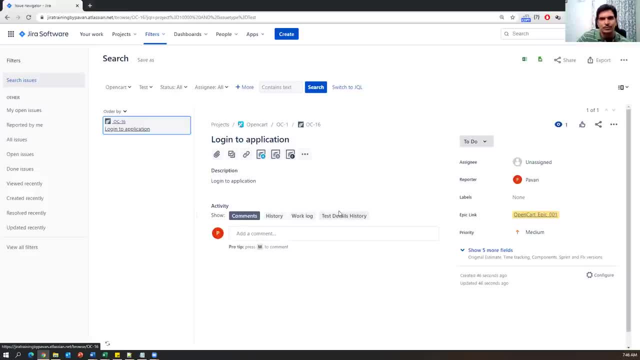 and so on. multiple options are displayed. so now we need to add steps and expected results to this particular test case. now, how we can add it. if you want to add it, what we can do is we just go to details- test details icon. we have to click. so once you click on test details, i icon. 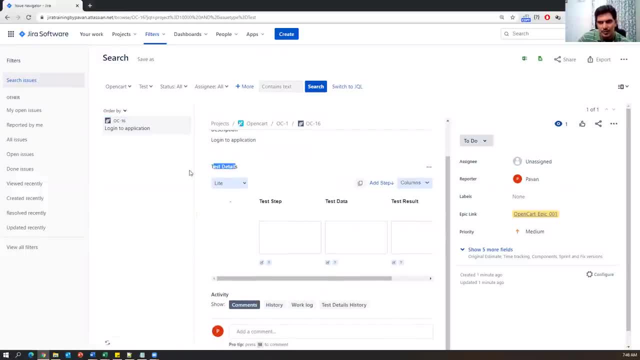 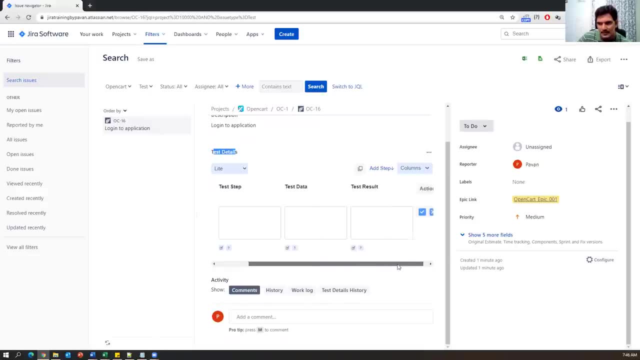 then you can see the small form: test details, form: right, so here you have to provide the test step: data, test result. okay, what step we have to perform, what data i have to use? what is the result we are expecting? so these three things we have to add. so first let me write one step. so here, open application url. 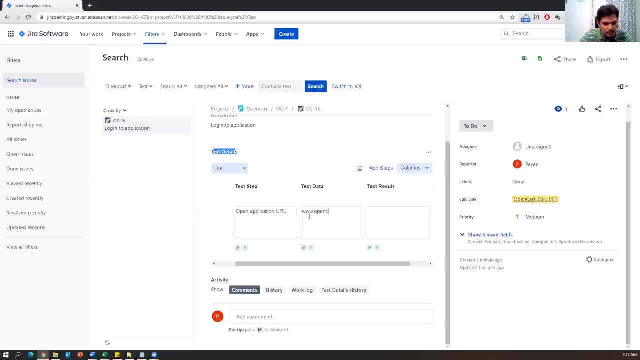 okay, what is the test data? we use wwwsayopencardcom and test results. what you are expecting? app url open and able to see able to see home page. this is what expected: able to see home page, the first step. then, after completion of the first step, click on the tick mark. then we can add one more step. say this one: 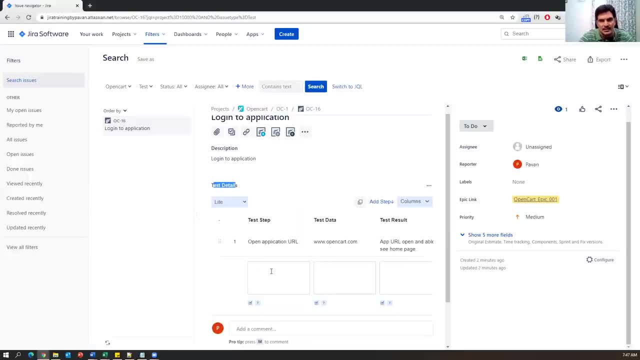 step is added and the second step. so what is the second step? to login. so here, provide valid username, username and password, and what is the data here, where the user and password and what is the expected? what is the expected? uh, provide valid username and password. values, any password. what is expected here? 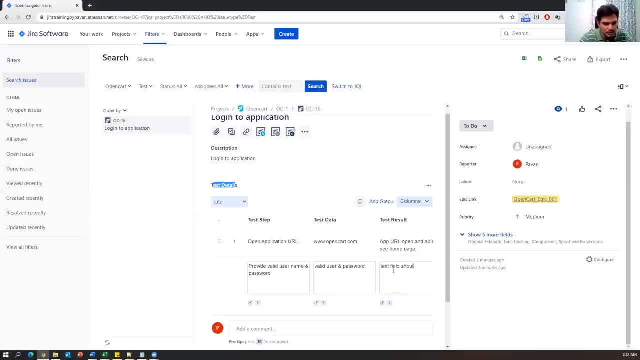 text fields. text fields should allow values. okay, done, so next step is done. after completion of this step, again we have to click on the tick mark, then one step is added. so two steps added so far. now third step: so after providing username, password, then what you have to, we have to. 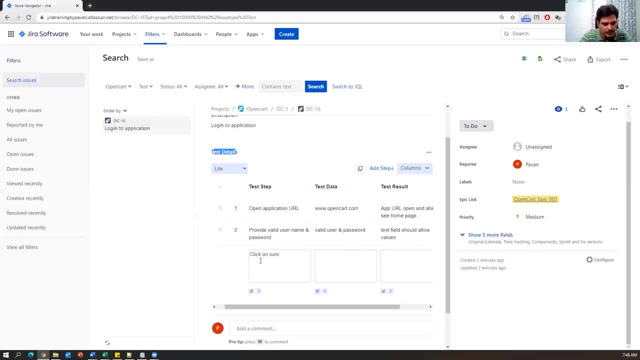 click on submit. you can click on submit button and then no data not required, not applicable, and user should go to my account page. so this is our expected result and this is my last step, so we can just click on this. done so, another step you don't need, you can just click on the. 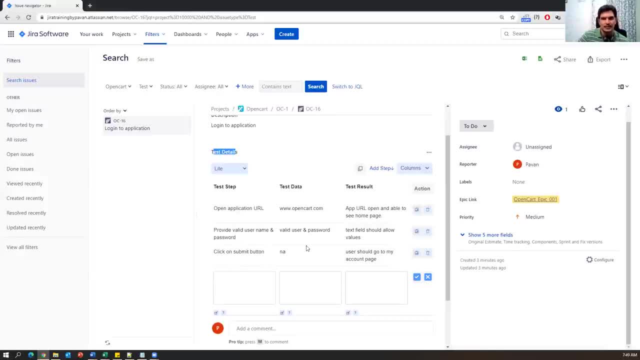 or let it be there. so three steps. we have added test data, test results and everything apart from this. we can also add some other information and any comments if you have history working log. so all these things we can update if required, or else we can leave it empty. 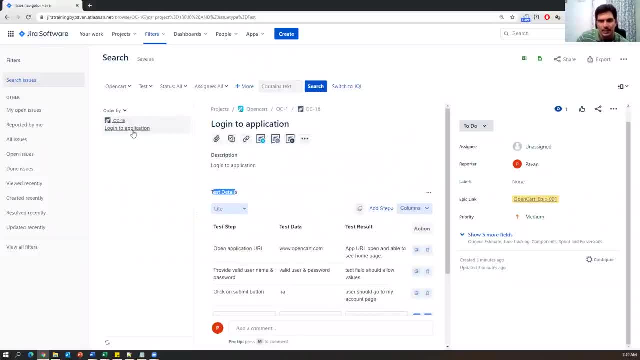 so this is how we need to create a test case. now i have created one test case manually in jira tool, but again, this is little difficult. but again, this is little difficult, guys, because if you have 100 test cases, if you want to do this like this 100 times, it is very. 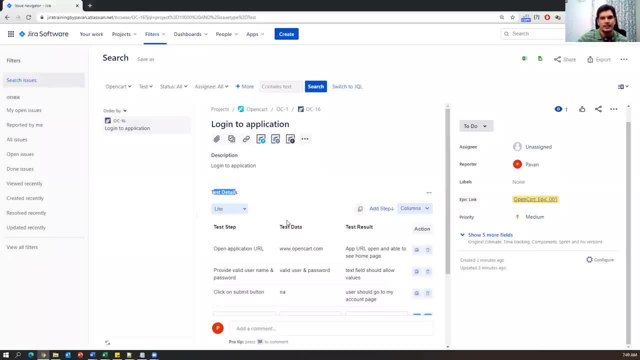 very difficult task, right? so normally what you will do in the beginning levels, we will write all the test cases in the excel sheet or excel file, so we will conduct multiple reviews once you upload your test cases. then we will upload all the test cases and one shot instead of writing. 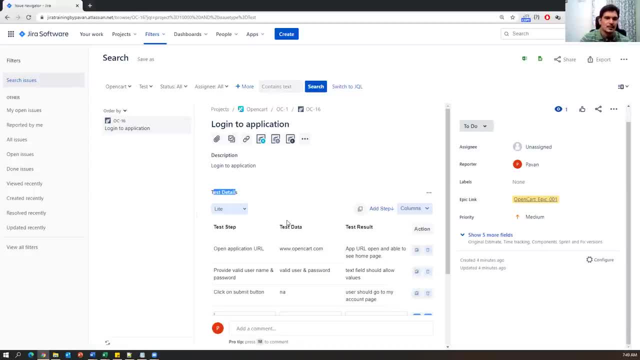 multiple test cases like this. we will import all the test cases into jira at one shot. okay, now i'll show you how we can do that import also. so once you created your test case where you can see the test cases in where exactly, in which place we can see the test cases, first go to the project. 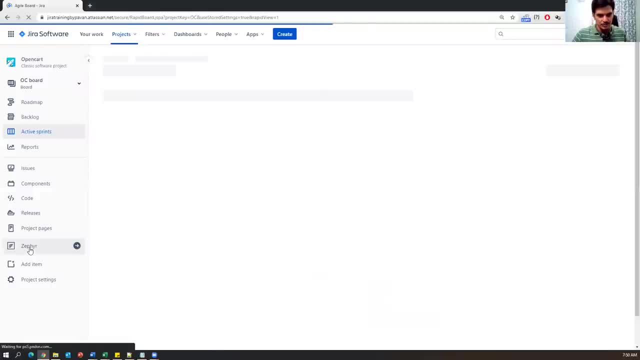 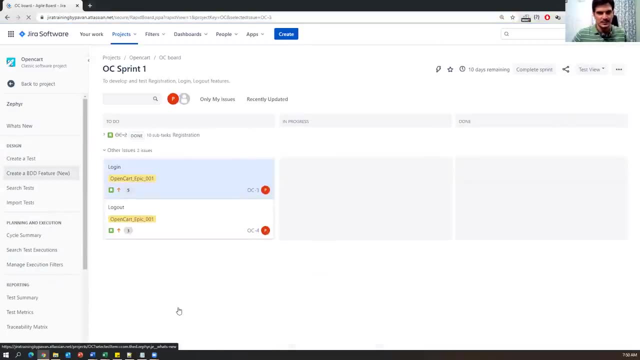 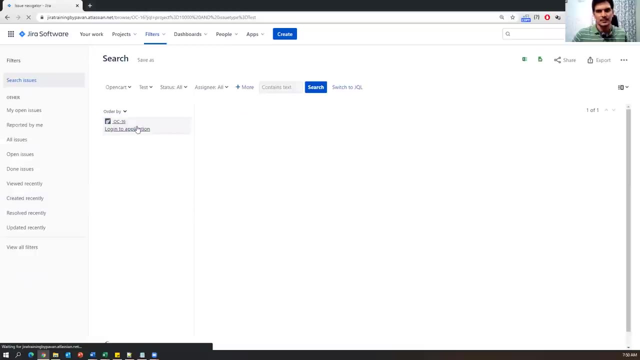 and you will see the project home page. we need to first go to jfire plugin and here, inside the jfire, okay, you can see the search test and inside the search test you can see the test case. and once you click on the test case, once you click on the test case, 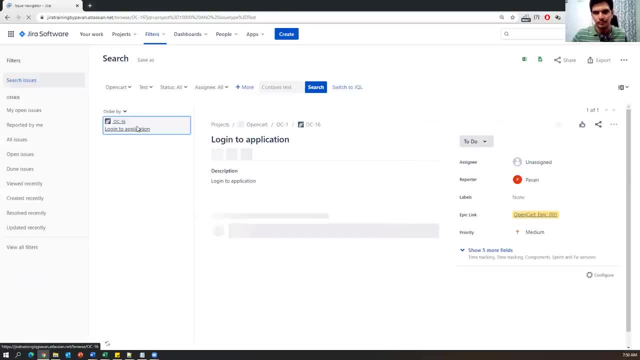 and then you can see the details. so these are the details. yeah, now you can see the all the steps and everything. so if you want to execute the test case, then we can go to execute. so, test execution. so this option we will use later, once we added this test cases to the test cycle, then we will do that. okay, so this is a way we 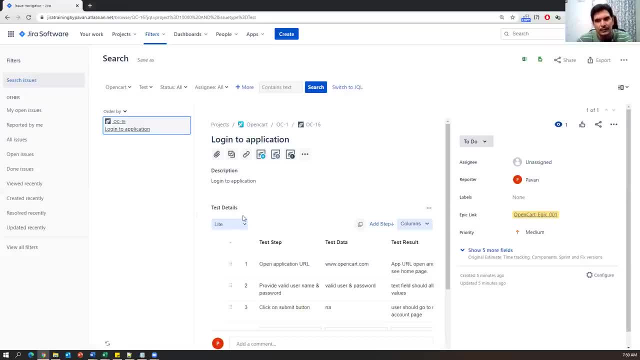 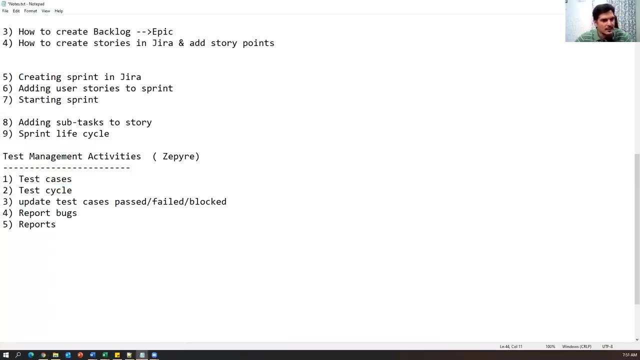 can create test case manually in jira suppose. i don't want to do like this. i want to even import bulk number of test cases into jira at one shot. okay, then, how we can do that. so now i'm going to show you. the next thing is how to import the test cases. so far, we have seen two things. 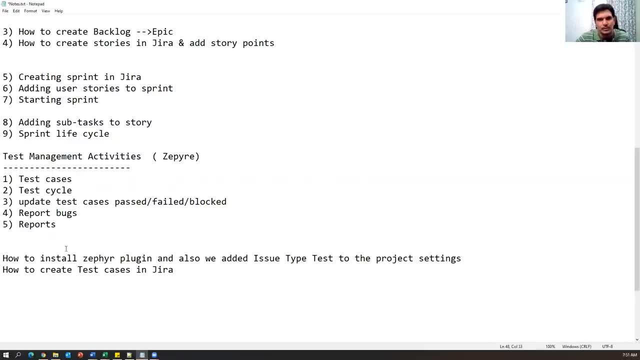 so how to install jfr plugin, and also we added issue type test to the project issue we have. we have seen like this is not required, and then we have seen how to create a test case in jira manually right. so now i'm going to show you how to import. 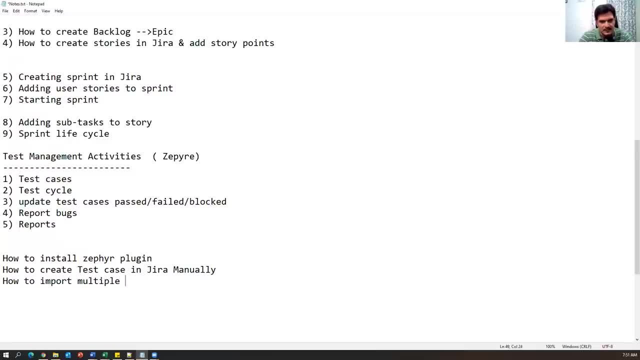 multiple test cases into jira tool. so now i have already test cases written in my excel file, so i want to import them into jira tool. so So how we can do that? So to do this we need to follow certain prerequisites. So we have to write the test cases in Excel by using proper template. 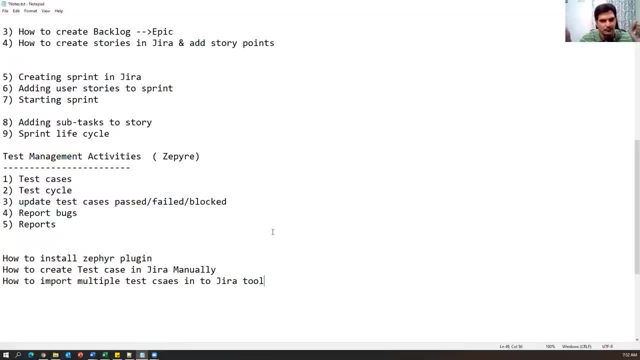 Because in our Excel file, in our test cases, the headings will be different And, as per the Jira perspective, the headings will be different. So we need to be thinking both like Excel sheet. whatever headings we are using, in which format we are using Excel file that should exactly match with the Jira format. 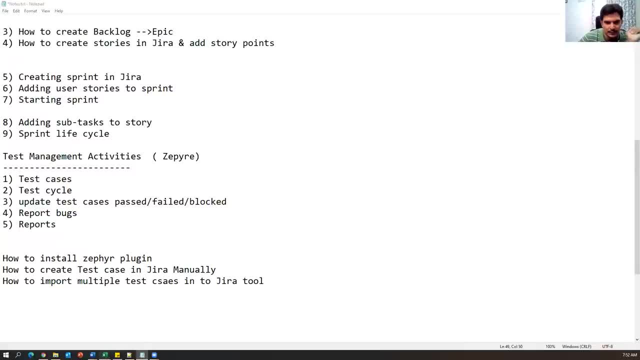 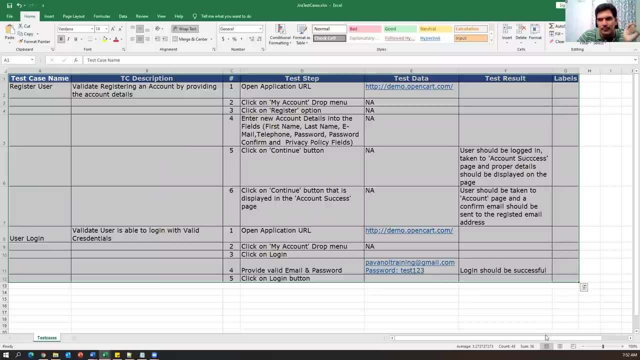 And then only we can import. So here I have created a few number of test cases according to Jira template or Jira format. So here the main. you can add any number of fields, but you need to map later. So here I have written a few number of fields, let's say test case names, test case description. 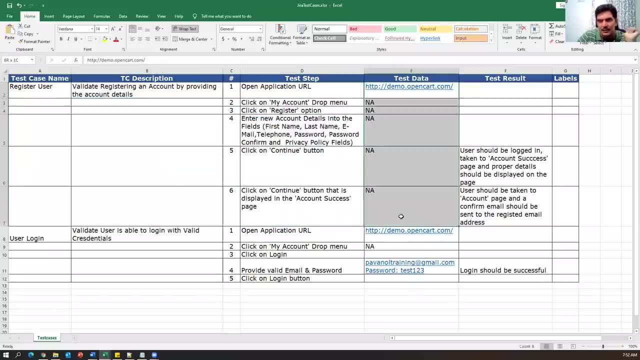 And these are the steps for one test case. These are the test data for each step: test results and labels. if you're required, you can update the labels also. So this is it. This is one test case still here And this is another test case. 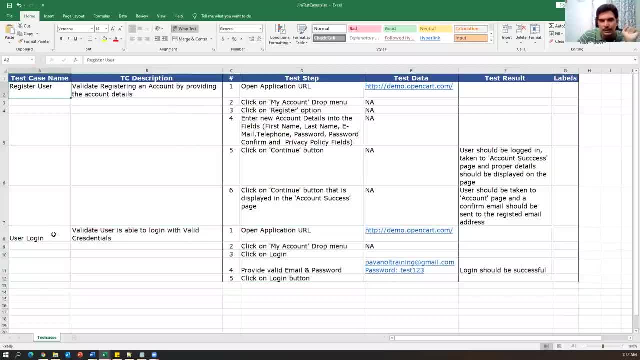 So totally, two test cases. I have register user, user login. So let us say I have n number of test cases like this. I want to import all the test cases in my Jira, So how we can import them. Instead of writing each and every step, I can import all the test cases in one shot. 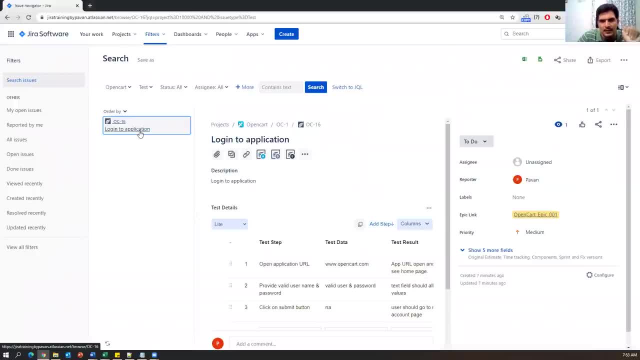 So let's see how we can do that. So we have login to application already there. So let me try to delete this test case, Because I'm just going to import now, So I'm just deleting the test case. So now I don't have any test cases. 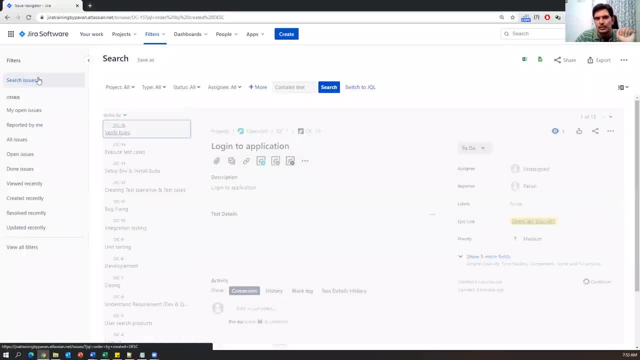 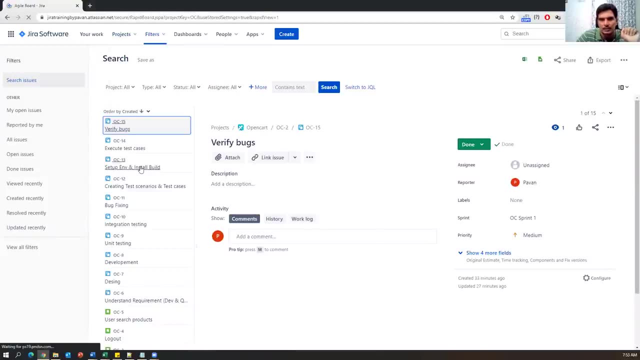 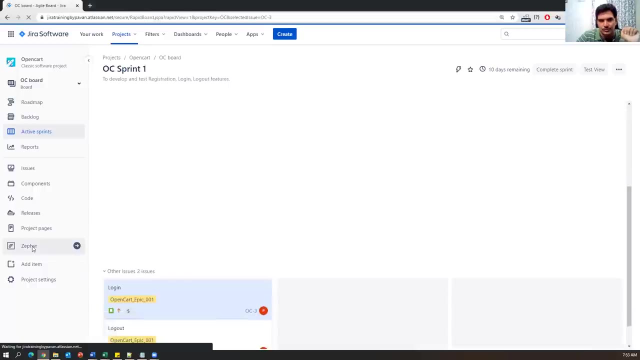 Now we just go to search issues, Right, so not here. we need to go back to the project And here go to Jifier. inside the Jifier we have to search for issues. go to the Jifier, click on the Jifier. 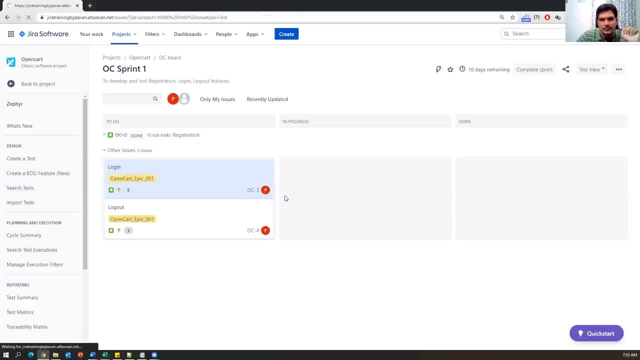 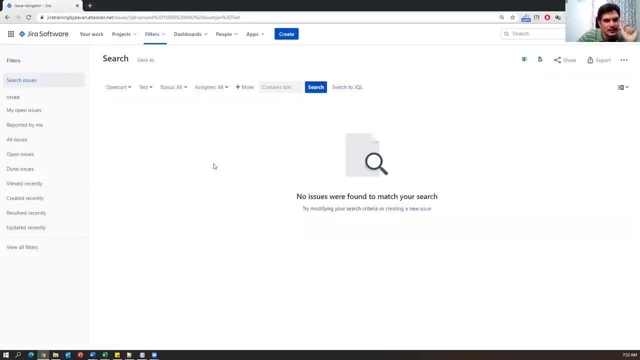 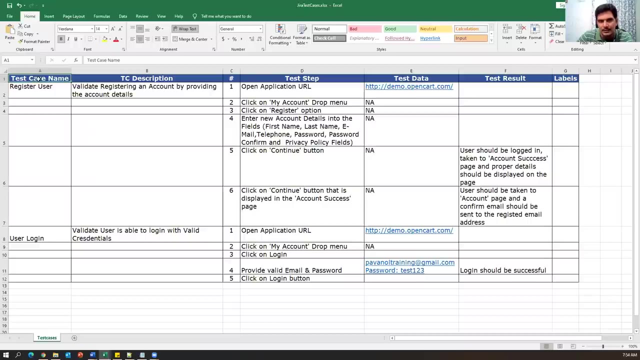 And then you can see: Okay, So here we have the search test. So in the search test I don't have any test cases, Everything is empty. Okay, Now I want to import the test cases. So to import the test cases, make sure your Excel file or your test case template should. 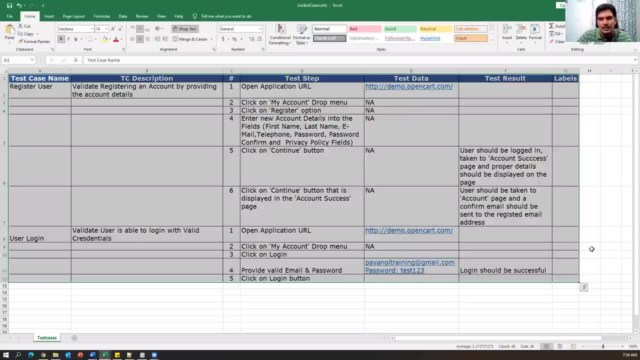 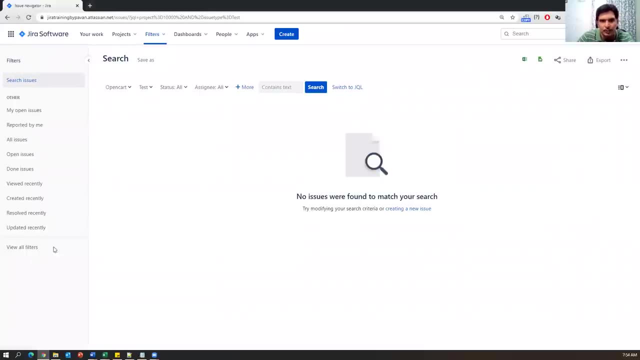 exactly match with Jira template. Okay, So this is the format exactly Jira will follow. So now let us try to import these test cases in Jira tool. So how we can do that? So here you can see some functionality called import again, go back. go back to Jira, go. 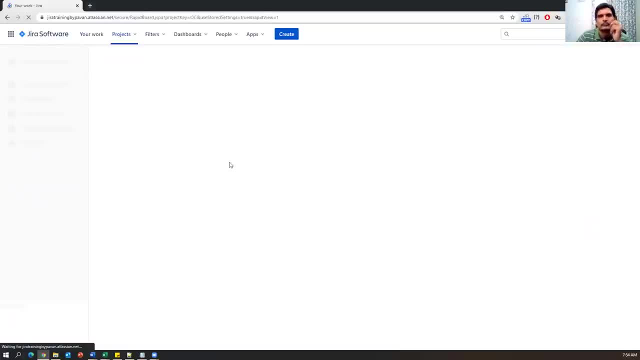 back to our project And everything we can do only within the Jifier plugin. just select the Jifier here. So here we have to select something called import test. You can see here: this is import test. click on this import test. 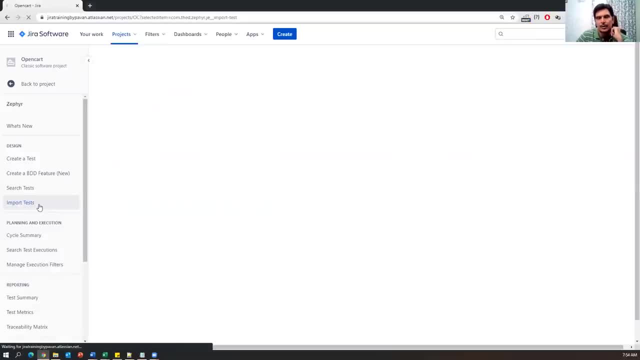 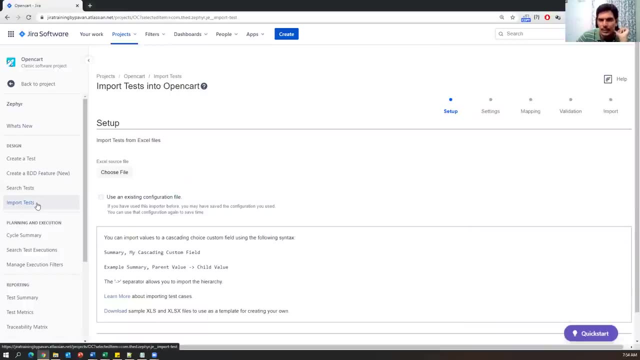 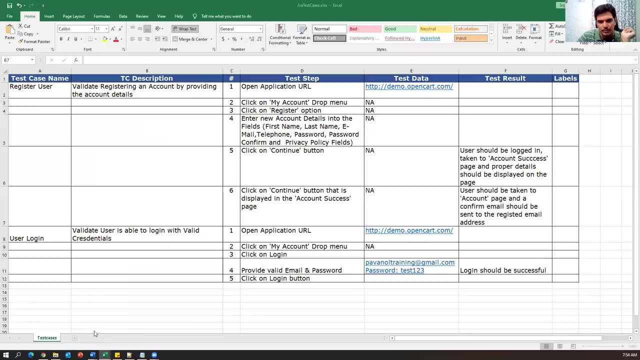 Okay, Okay, Okay. So once you click on the import test, so here you have to choose the Excel file. So this is the Excel file which I'm going to import, the Excel file which I'm going to import two test cases register user. user login. 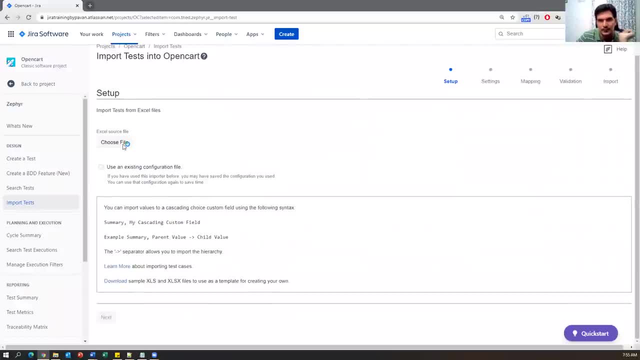 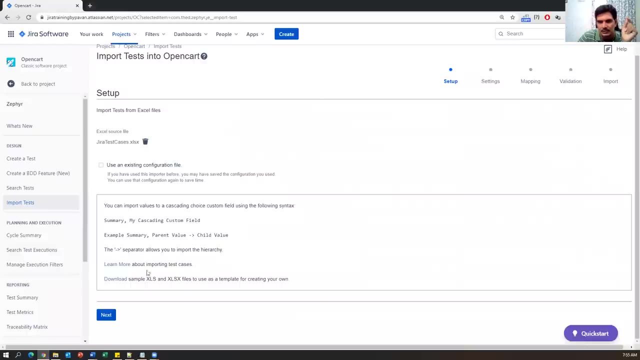 So close this Excel file before. So here I'm browsing the file, click on the choose file and selecting the Excel file open. Okay, So now it is trying to get that file. Okay, Once it is done and I can just click on the next, it is success. 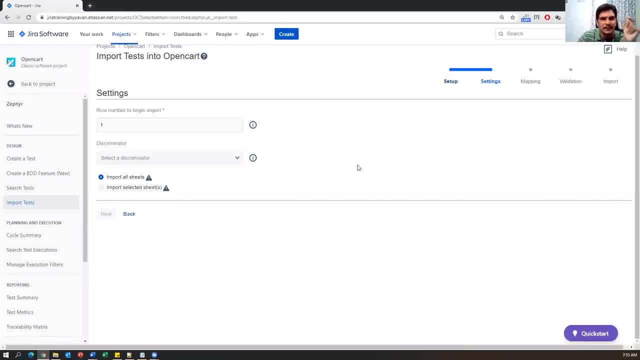 Then click on the next and here in the Excel file or Excel sheet, the first row is a heading part, right, So we have to start from the second. So instead of one we have to say two here, Okay, And then delimiter discriminator. you can just look at here in the Excel sheet how. 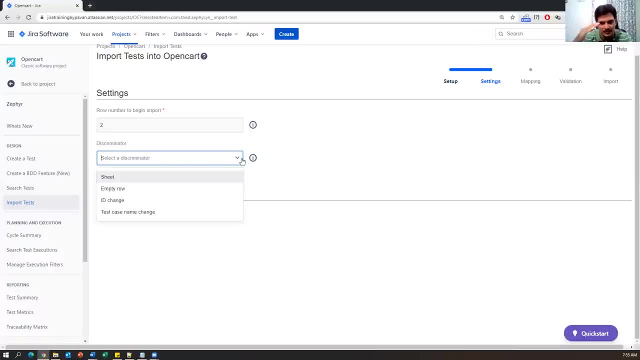 the test cases recognize. Okay, How we can recognize the test cases are different. So one test case to another test case. is there any discriminator there? So, based on the test case, name change suppose if there is an empty row between one test. 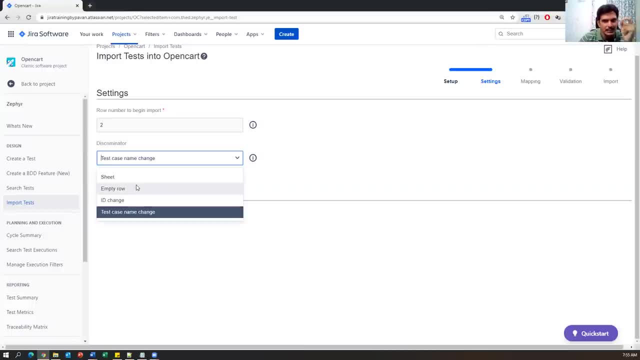 case- another test case- you have to select empty row or if you are using ID, so you can use ID change. So multiple options are available. So currently the test case name is a different, so I can say test case name. 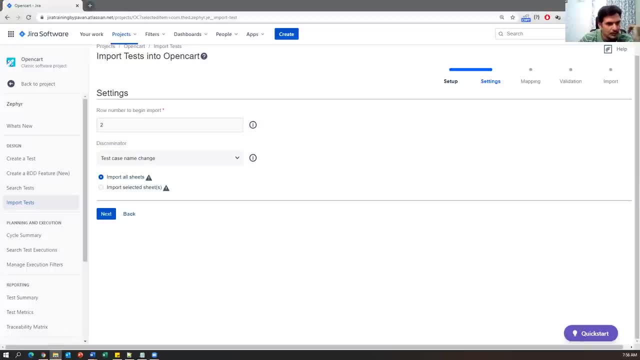 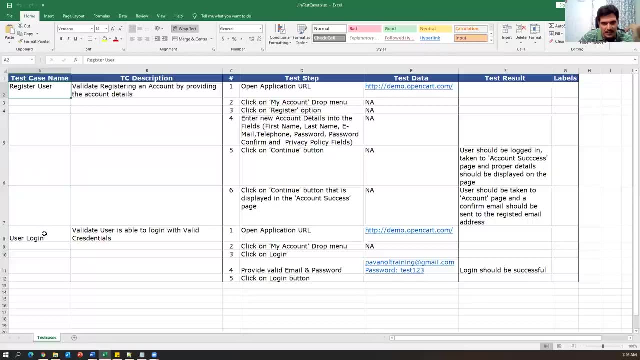 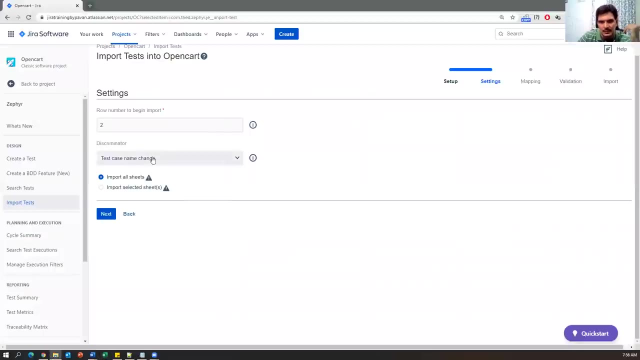 So if I just look at again Jira test cases, See this. So here the test case name is here, And what's the next test case where it start again with the test case name? So test case name is a discriminator. Similarly, I selected this and import all the sheets or import selectors. 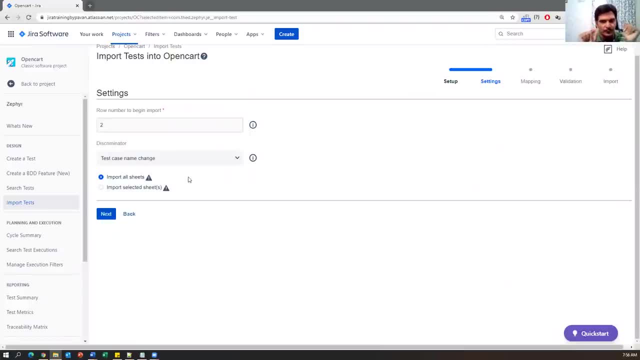 If you have multiple sheets in your Excel, you can select the first one If you want to select. if you want to import only test case from specific sheet, then select the second one. import selected sheets, And here we have to provide the name of the sheet. 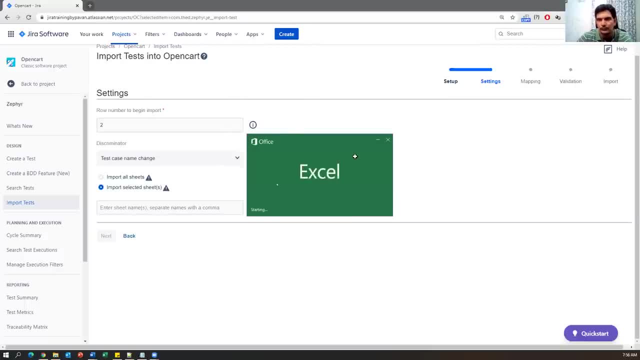 So let me check the name of the sheet, Okay. So test cases. this is the name of the sheet, So I'm just writing them: test cases, Okay, And then click on next. So once you click on the next, it will try to import the Excel sheet which contains: 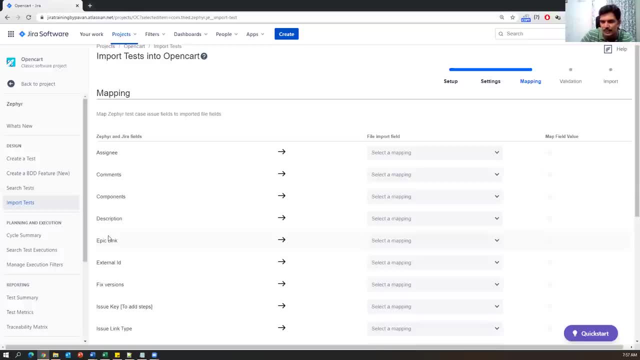 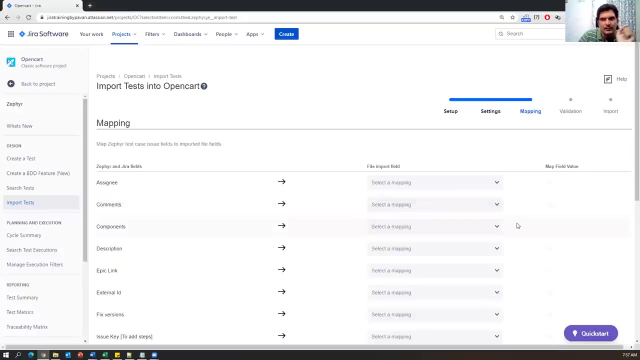 all the test cases. Yeah, So now this is the very, very most important step here. So these are the actual Jira fields for every test case. there will be assignee comments, component description. There are a lot of things that are there for every test case but in our Excel template. 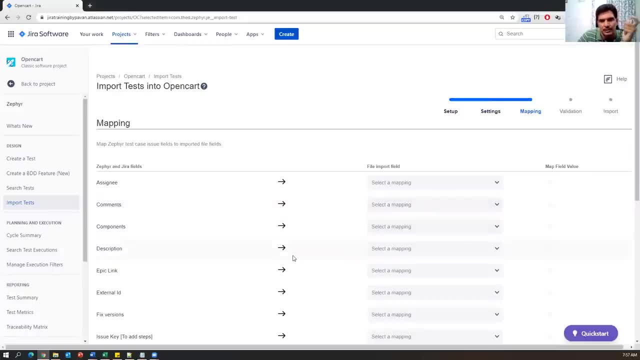 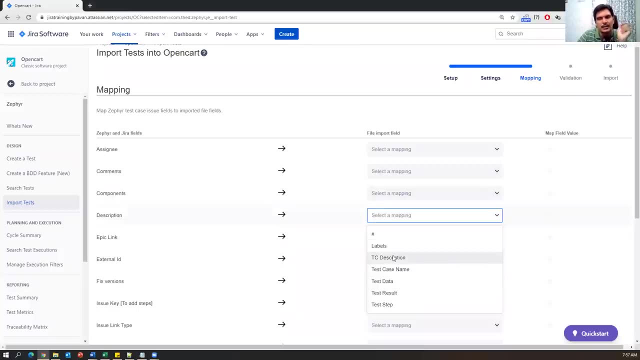 we have to map these fields with our Excel template. For example, in Excel, what are the headings we have? So we have description, So just select the dropdown and these are the fields which we have written in our Excel sheet. So we need to exactly map with that. 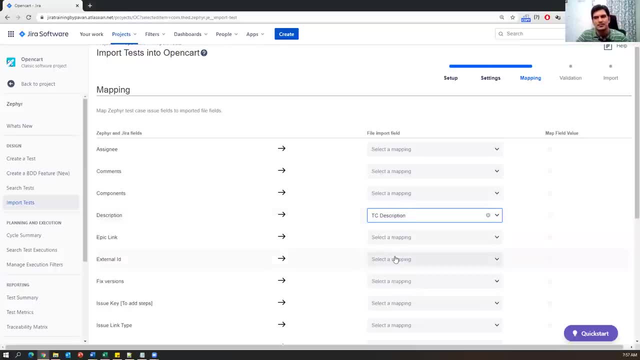 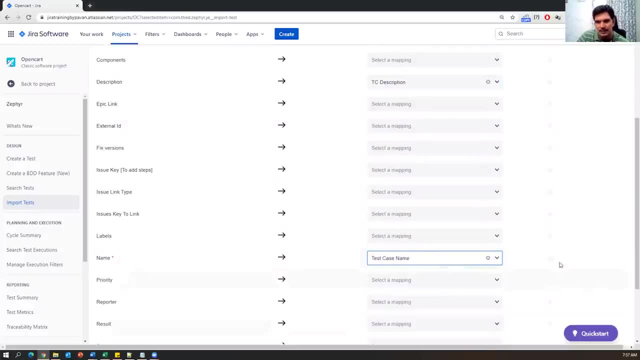 So description is available in our Excel. So we need to select the test case description and what else we have in Excel file. So we have a name also. So you see name, test case name We can map And then what else we have. 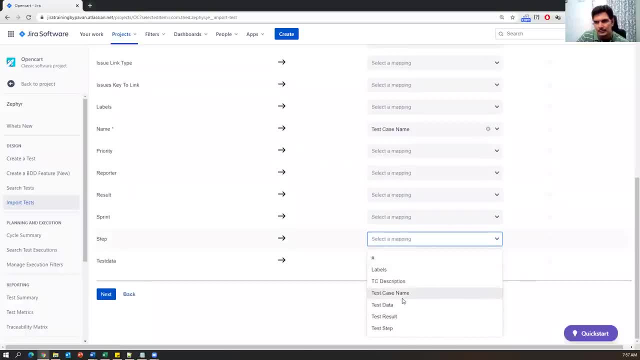 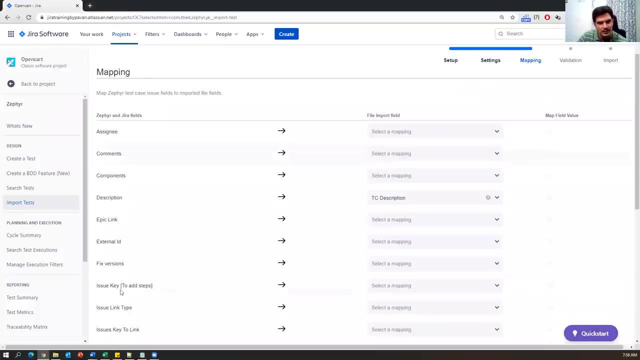 We have a steps, So steps we can map with the test step and test data is also there, So test data we can map. So like this: whatever fields or columns we have in Excel field, Excel file, So we need to map all the columns with the Jira fields. 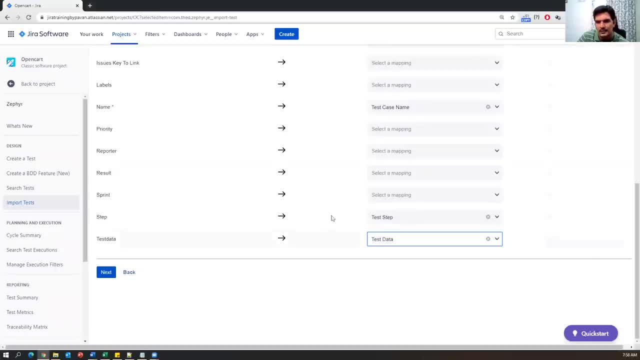 Okay, So once the mapping is done, right, So then you can say next: And do we have anything? Result is also: we have it. Yeah, Right, So expect a result. So test results also we can map, That's it. 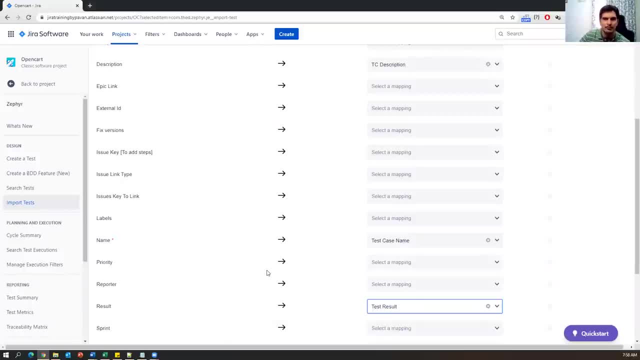 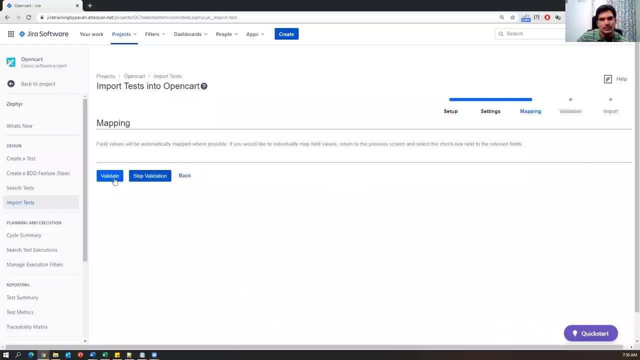 So whatever the columns we have written in the Excel, the same fields, we need to map it here and then next done. So once we click on the next, so just validate here, because every mapping, whatever we have done, is correct or not. if you want to validate you can just click on validate. 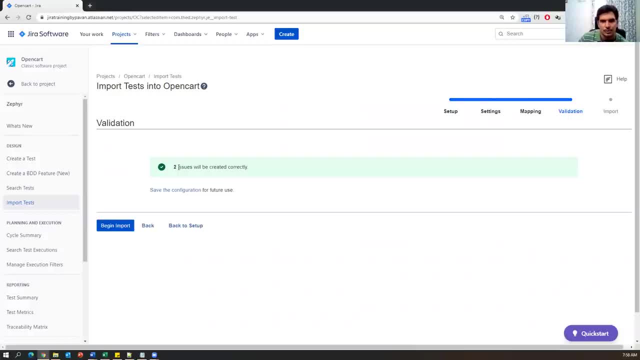 And if mapping is perfectly done, so, which is success- or two issues will be created successfully, And then Again, you can just begin import. Click on begin import. So once you click on begin import, now your test cases are importing. So previously we don't have any test cases. 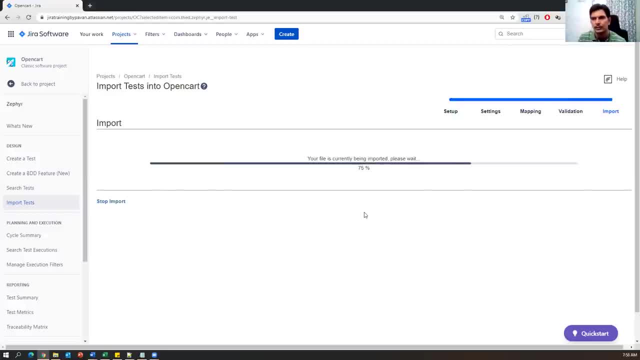 Now I'm trying to import two test cases, So now let it complete. Yeah, Now two issues have been imported successfully, And again, if you want to import a few more test cases again, go begin another input. Again. process will start. 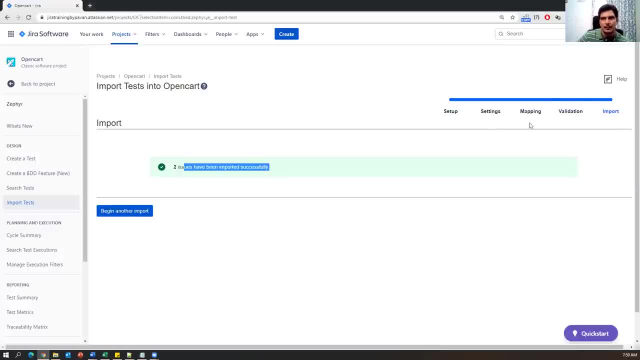 Okay, This is the workflow of importing Excel setup settings, mapping, validation and then import. So now, where I can see the test cases which are imported, just again go to search tests. Then here you will able to see the two test cases. 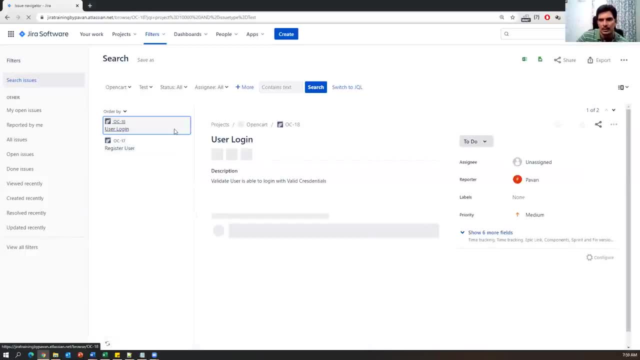 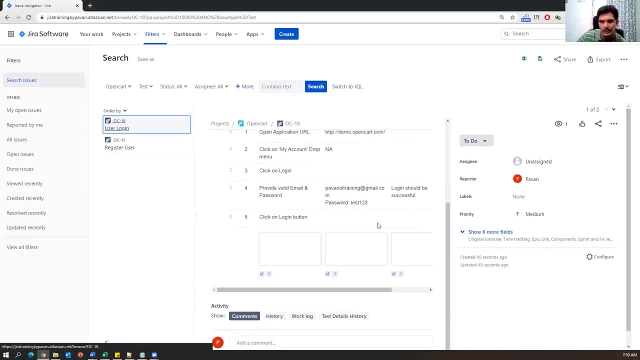 So now let me open the login. click on the login. Now you see the description and also you will see the steps. Go to the details here. click on the details Now we can see all the steps have been successfully created: Five steps. 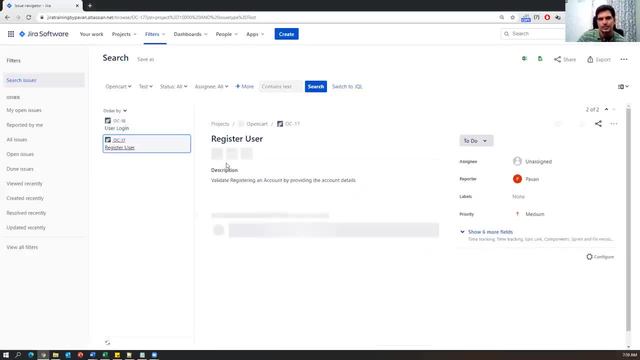 We have in the test case, similarly register user. So go to the details and here all the steps have been created. Okay, So this is how we can import multiple test cases from Excel to Jira. So this is very, very useful option. 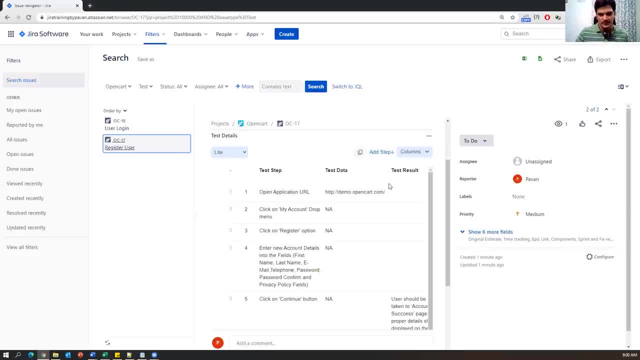 And this is the way we can do most of the times. we don't write individual test cases manually. It takes a lot of time. So instead, because initially we will start with the Excel file, So once all the reviews are completed, Finally, we will import all the test cases from Excel to Jira tool. 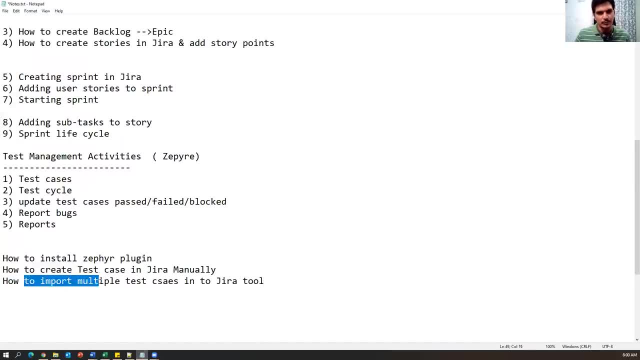 Okay, Done. So this is how we need to import multiple test cases in Jira tool. So this is the first initial task we do. So we have created test cases manually, or we can import the test cases into Jira tool. Okay. 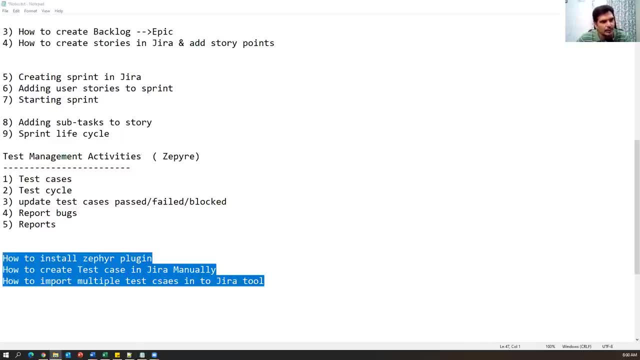 And the next and final action is we have to create the test cycles, We have to add test cases to the cycles, Then we have to execute reports, Okay, And traceability matrix. There are a few options which we have to do, Okay. 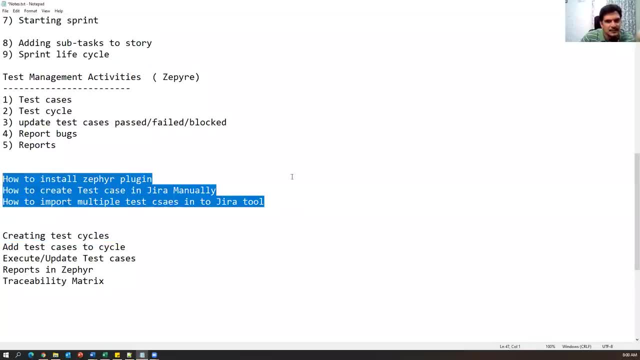 So creating the test cycle? So we have just created the test cases, right, but where exactly? we have to execute them? So we have to execute those test cases while creating a cycle. test cycle within the sprint. Okay, Within the sprint itself, we will get multiple builds from the developer, right? 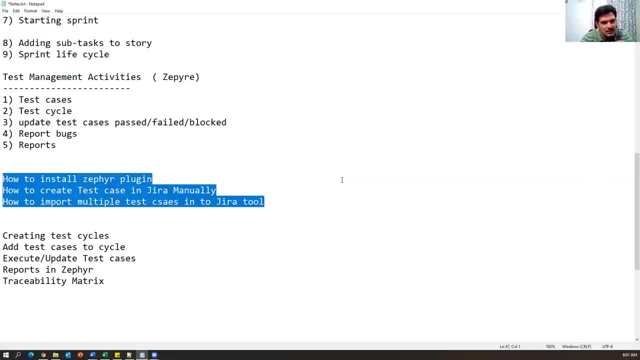 So, for each build, we will create a new cycle and the set of test cases we will add to that particular cycle. We will execute it. Okay, So now I'll show you how to create a cycle, how to add the test cases to the cycle. then 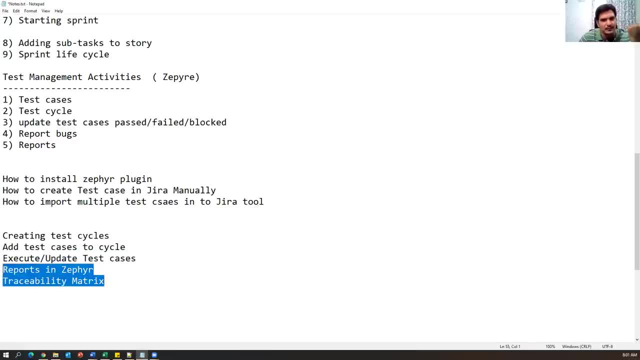 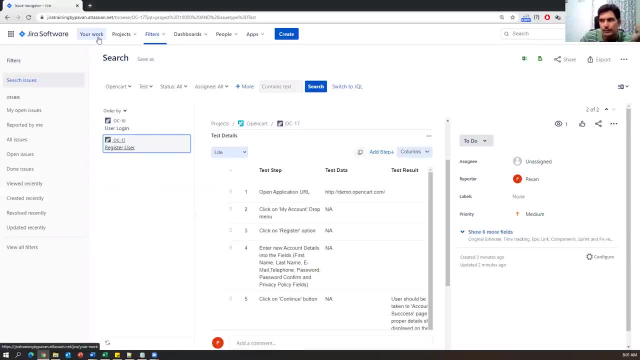 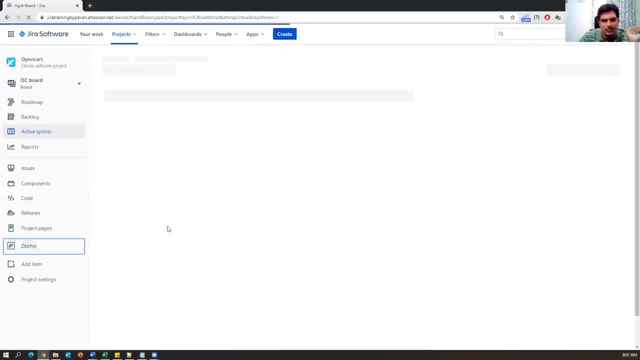 how to execute or update the status of the test cases, And then, finally, we will see the reports. So let's go back Now. we are done with the test cases. Now, again, go back to the Jfire plugin, Go to our projects and click on the Jfire. 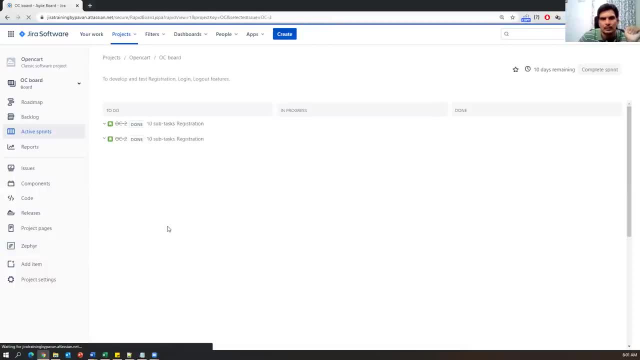 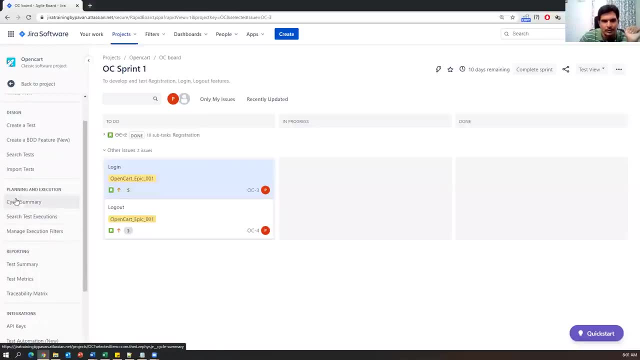 Okay, So we are done. Okay, Once you click on the Jfire, it will show you all the options. Yeah, So now come to the next section: planning and execution. So cycle summary, search, test execution, manage execution filters. 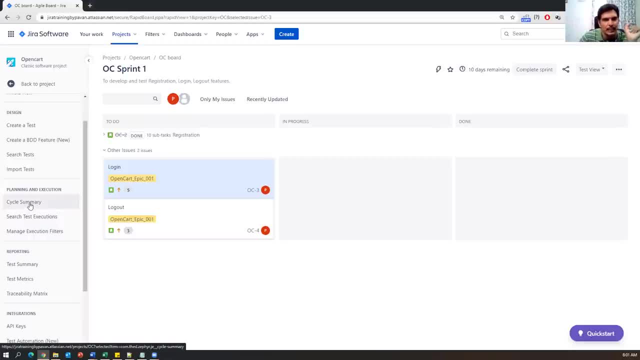 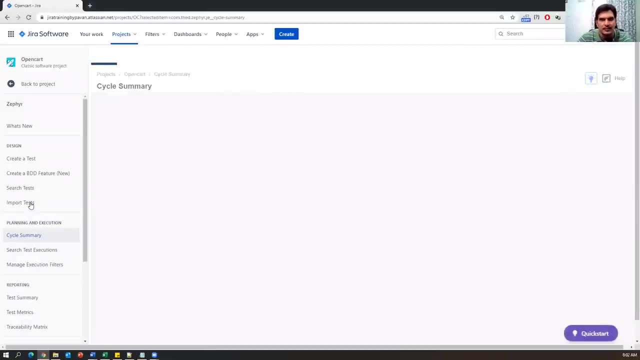 The multiple options are there. So here we have to go to cycle summary to create a new cycle. So cycle summary. So in the cycle summary we have to create a new cycle. Okay, Now we can just look at here. by default there are cycles, are created. 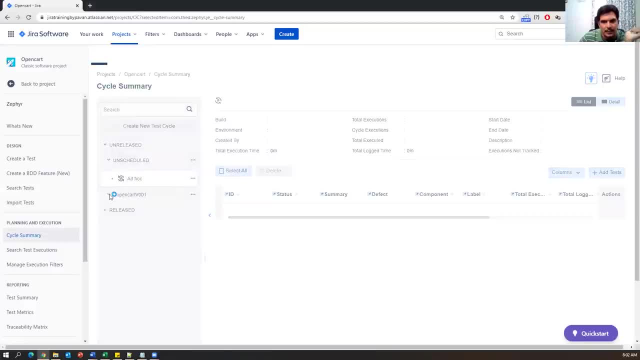 So unscheduled cycle ad hoc by default will be there And apart from this, this with the project version which is also already created, one cycle here, Okay. So if you want to create a new cycle, just click on the create a new test cycle. 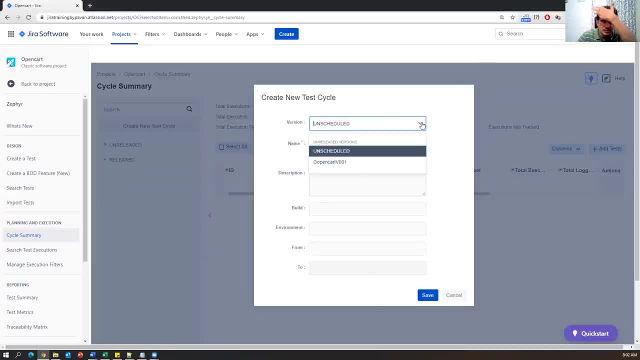 Okay, So here version number is unscheduled, So we have to select the version number. Open card, version 001.. Then cycle. So we can just give a cycle name. So here I name it as my, or you can say regression cycle. 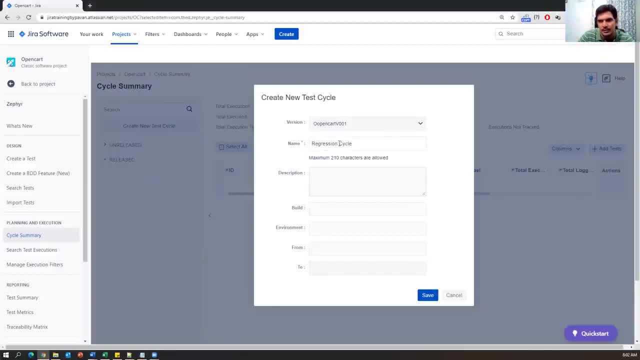 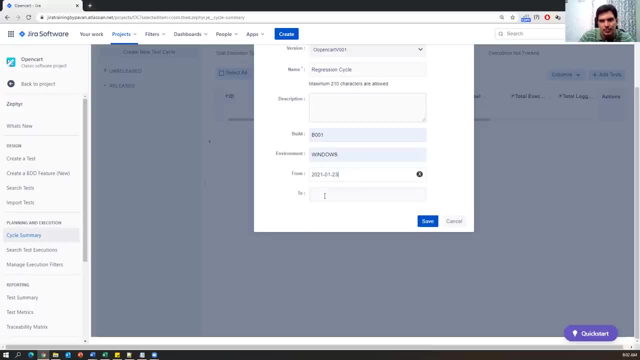 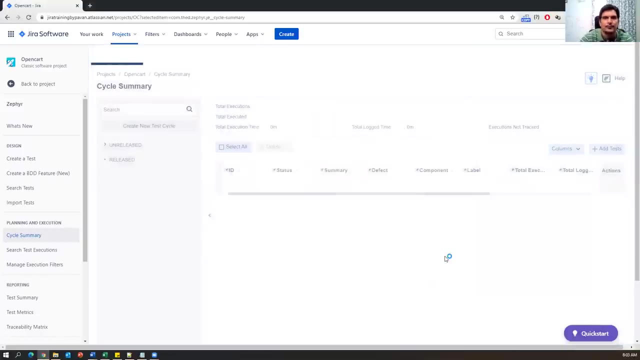 Okay, Regression cycle. And then you can specify the bill number or environment, on which environment you are executing and from date, which date, to which date you are going to execute this cycle. You can spell, select all the details of the cycle and then say save. 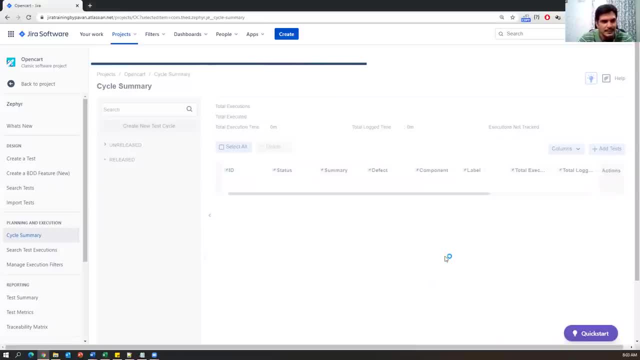 So now cycle is created. Okay, New test cycle is created. So now we need to add test cases to this particular cycle. So what are the test cases we are going to execute as part of the test, as part of this cycle? Okay, 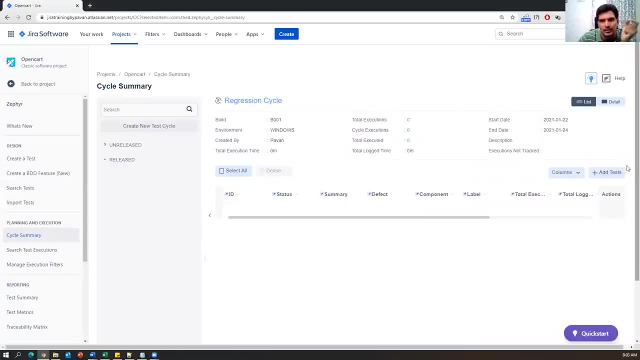 So far that what you can do is you can do two ways. Either you can just open the cycle, like this regression cycle, and you can just add test directly from here, Or else we can go to the test cases- individual test cases- and we will update the cycle also. 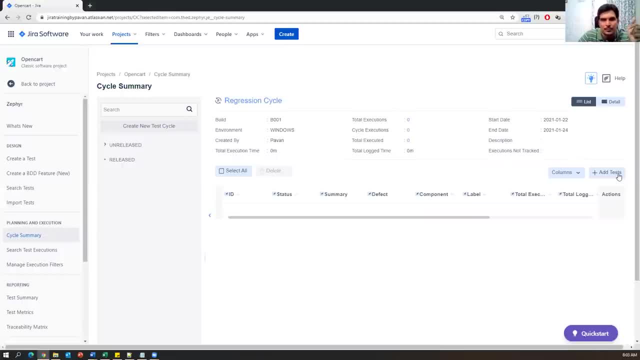 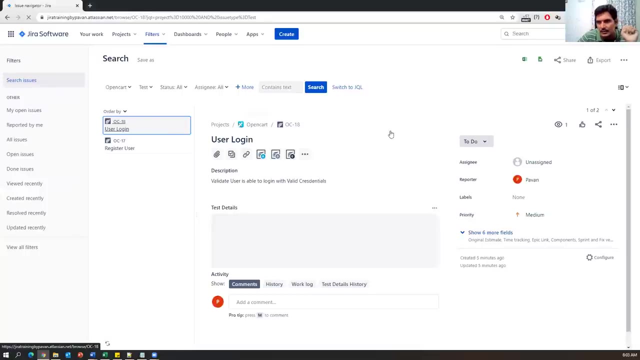 Okay, So that's it, Thank you. okay, suppose, if you go to the test case, let me go back again search test cases. there are two ways we can do. suppose i want to add this login test case to the regression cycle. so select the test case here and you will see the cycle also somewhere. 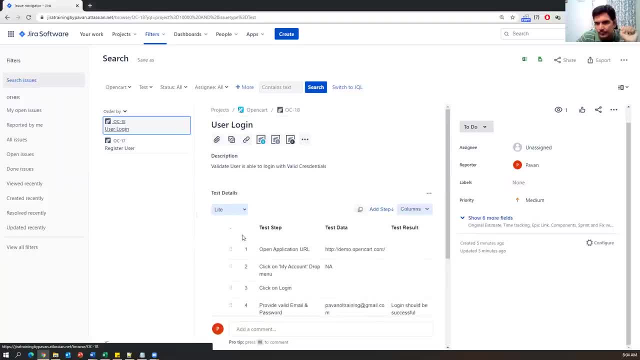 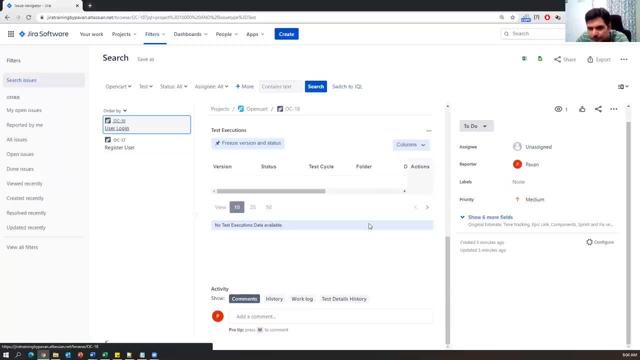 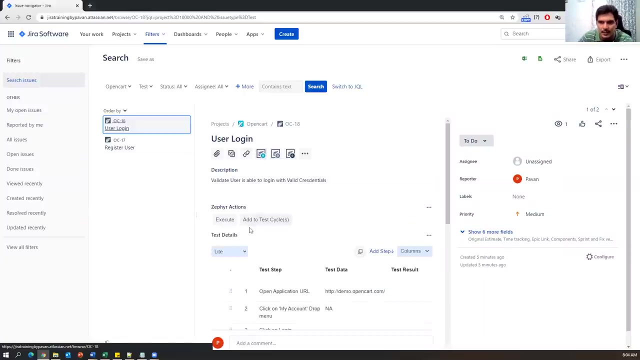 priority label will okay. so here you can just say execution, so test execution or actions, test execution. just go to this: test executions, okay. and here you can see something: okay, not execution actions, yeah. so we can just go to actions for striker and then you can see: add to test cycles. so in which cycle you want to add the test case you? 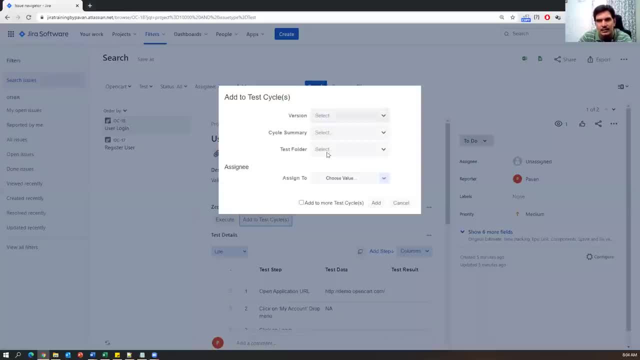 can just click on this button, add to test cycle, and then you can select the which cycle you want to add this test case. so individual test cases we can select which will we can add to the cycle. so this is the one option we have. so the other option is we can directly go to the cycle. let me go back. 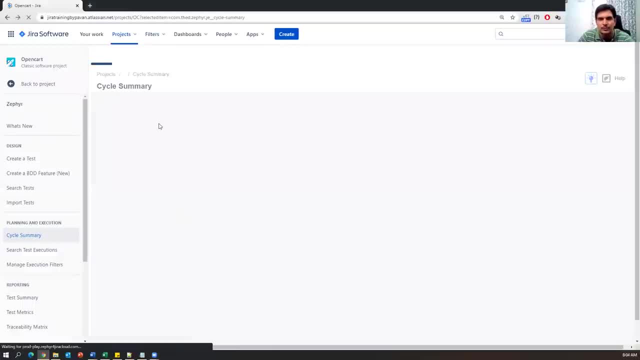 so go to the cycle summary, which will show you the which cycle we have just created. make sure all the trials you are indicating you have been created. so if i just locate here, so regression cycle which is created. so now if i want to add the test cases to the cycle, 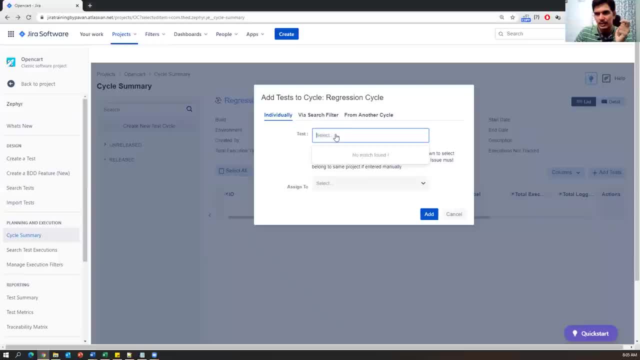 click on add tests here and here we need to add. so we have to write the test case names here. user login, register login. so user login, i'm adding and then it's just also i'm adding. who is responsible to execute this test case? you have to specify it. 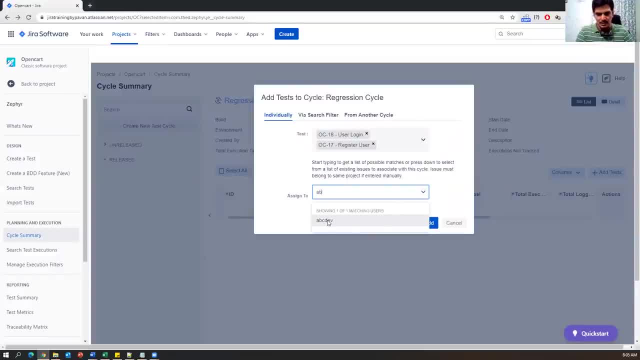 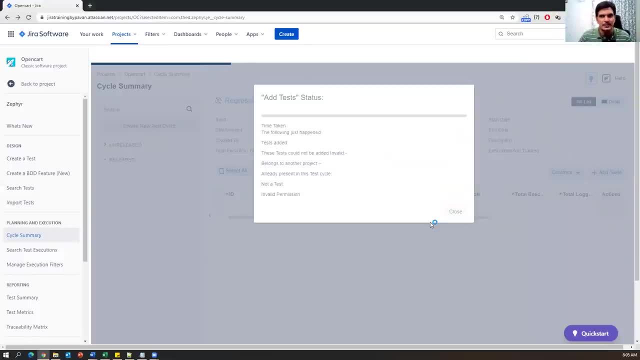 i'm just giving as a some name. worries are saying we have to give it that name. so it just specify and then say add. so once we added this, those test cases will be added to particular cycle. okay, once i added the test cases to the cycle, then we have to execute our test cases as part. 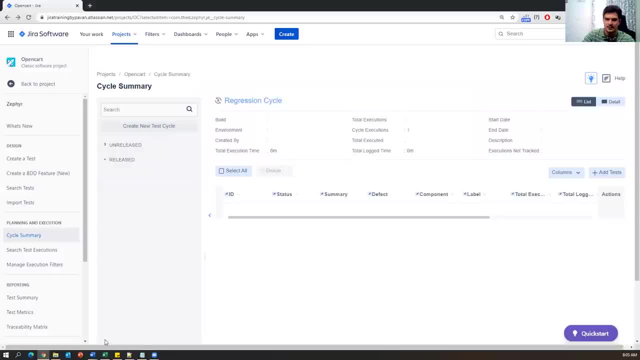 of the cycle. so now i'll show you how to execute and update the status. that's the next thing. so added test cases to the cycle. now we are going to execute and update the statuses. so to execute the test cases, what you have to do is we have to first go to the cycle summary. 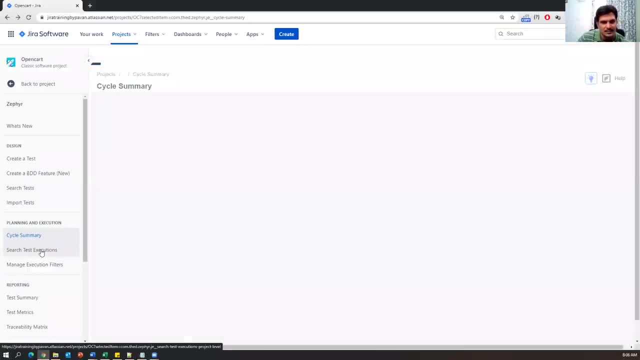 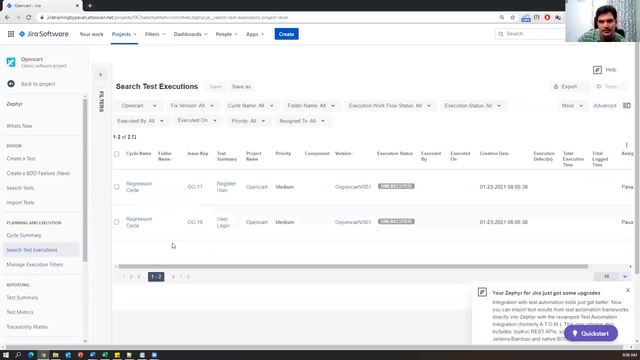 okay, and also you can just go to test search test executions. the second option is available, so go to search test executions. under search test executions you can see the what are our test cases are ready for execution here for this particular cycle. okay, so from here we can update the status. 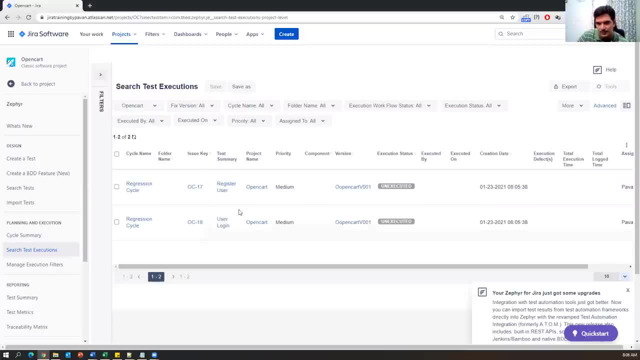 so, for example, this particular cycle, regression cycle- these are the test cases are planned, so still unexecuted. we have not executed this, okay, so need you need to execute these test cases manually? there may be pass or fail. whatever it is, we need to update the status. so how to? 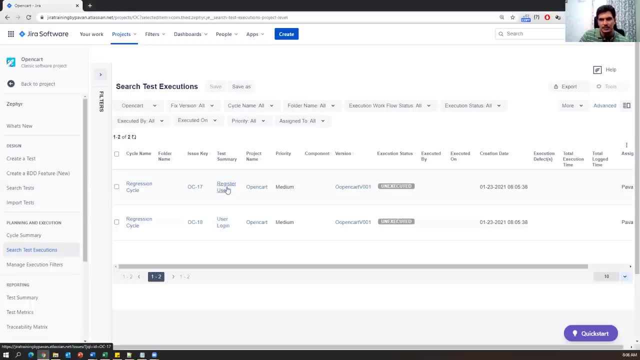 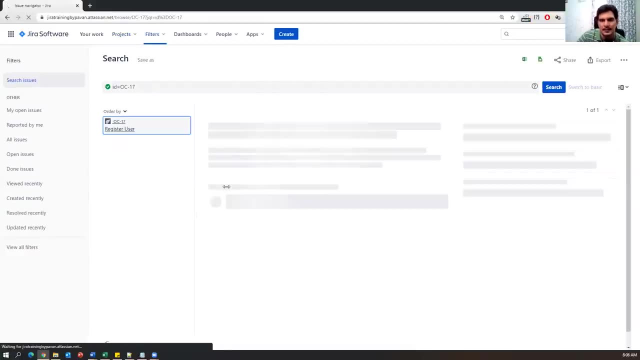 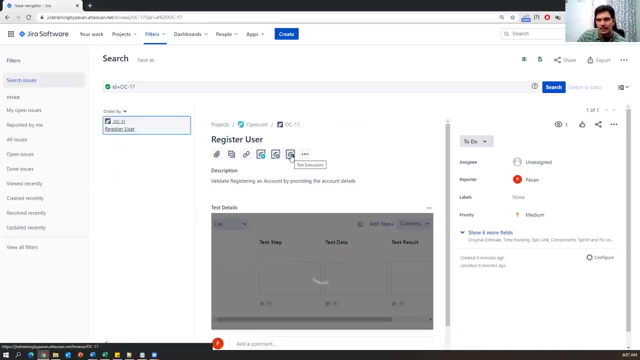 update the status. click on this test case. okay, let us say, register user. click on the test case and once you open the test case and there is an option called e- small test execution- okay, so we need to just click on this e. once you click on the e icon, then here you will able to update. 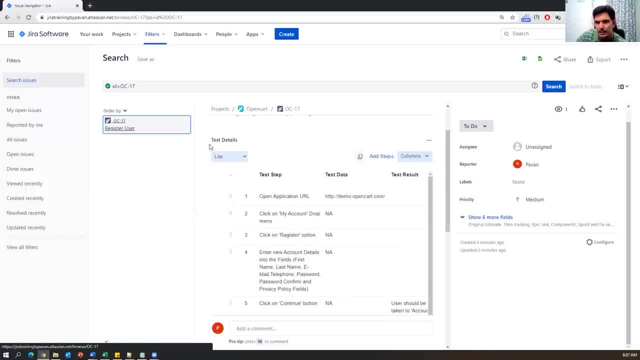 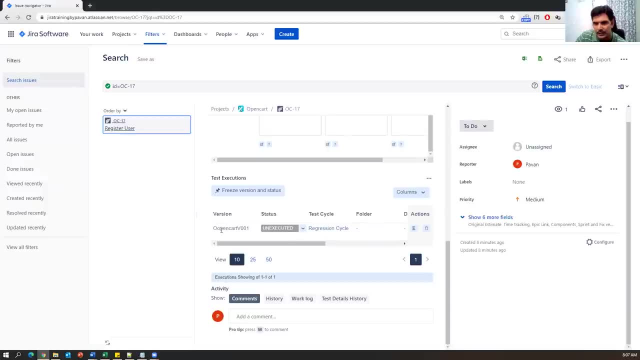 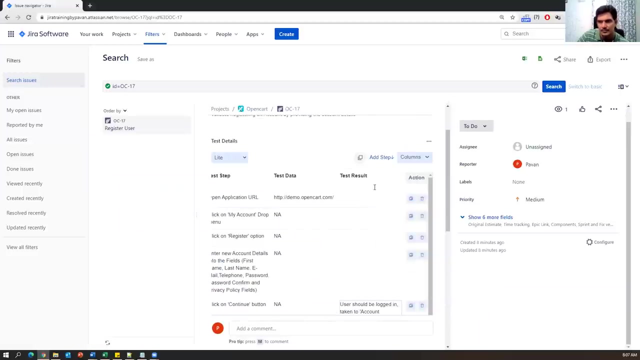 one second. okay, just a moment. somewhere you can see the option. yeah, here you can see. so, if you, this is the test case: unexecuted. unexecuted so far, so now we need to execute. so let me just make it as a pass, or you can also make execution of step by step. okay, just a moment, so to execute. 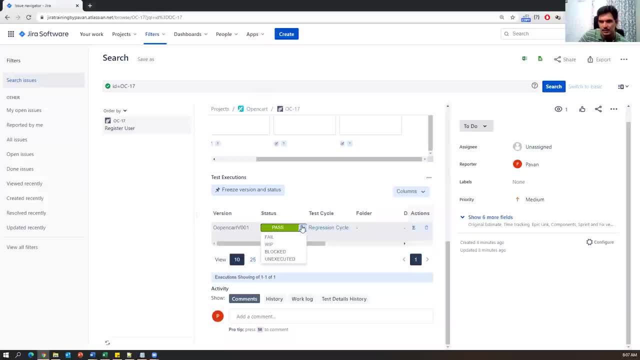 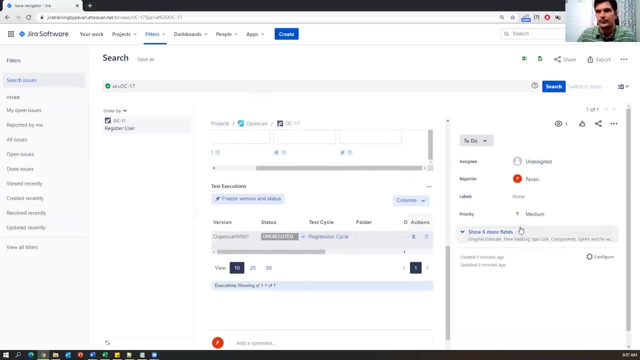 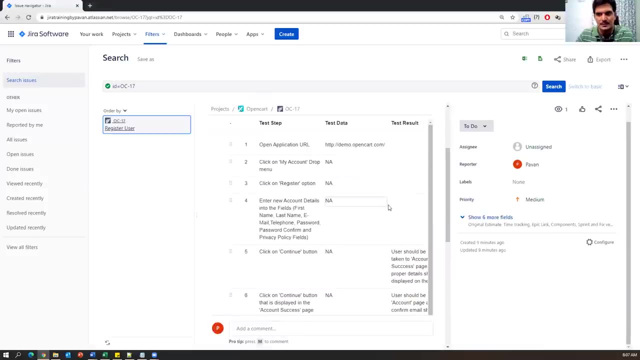 the test case. we can do here directly, or we can also do in some other way. i'll show you just a moment. so first of all, open the test case, go to the details. don't directly go to execution. go to the details, okay. so once you go to the details, one sec. 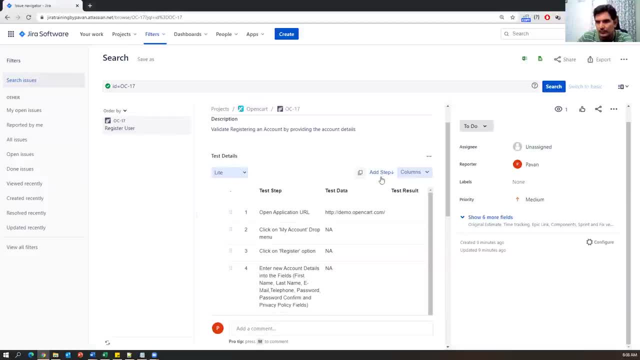 so these are the steps. right, you can see these steps just a moment. okay, so here i think there is another way to do this, but it's not showing anywhere. we can make the test case passed or fail, even step level also we can do that. so somewhere, 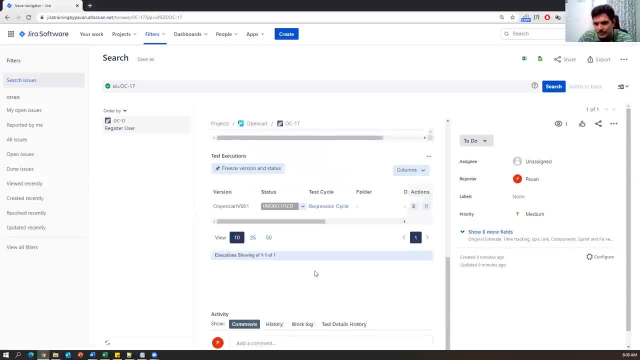 i could not see that option, okay, so we'll see that later, so for now, i'm just using this option. so just come down. so this is a test case, and which one? so this is the test case and we can see where it took us. so now let me. 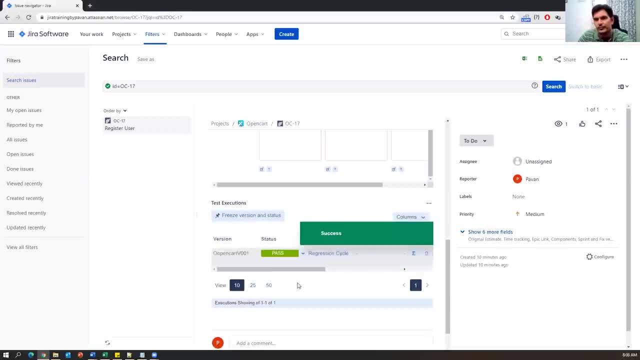 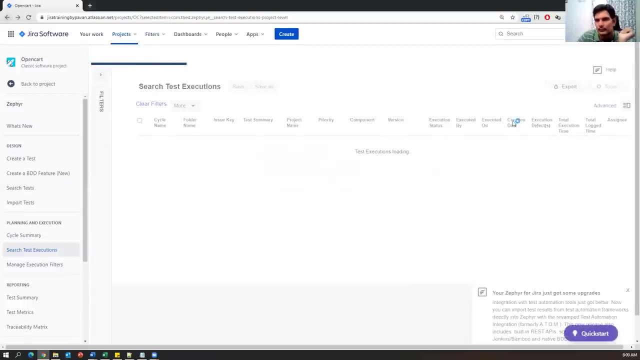 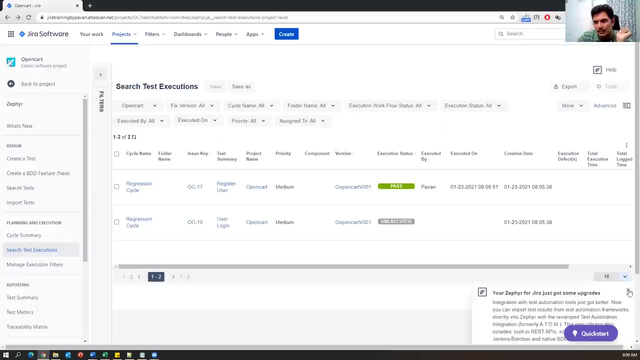 is not executed, so i'm just passing it for now. okay, pass success and similarly, just go back again test cycle. once it is passed, then go back to your test cycle. okay, so now we can just look at here two test cases. one test case got passed, we have executed, so similarly, i'll make one test. 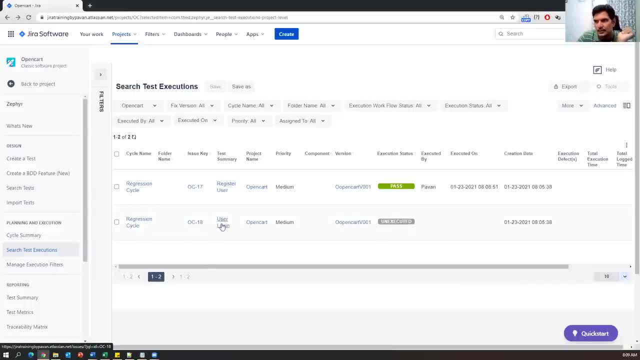 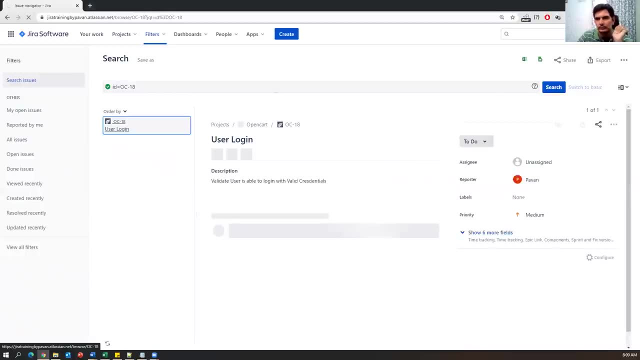 case got failed, so click on the test case once again here. user login. okay, and here again i want to make this: test cases passed, fail, so you can just go here and i make it as a fail. so my test case got failed, so manually you have to execute. okay, execute accordingly, you have. 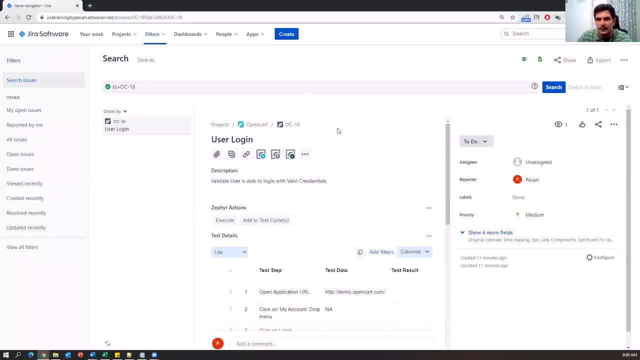 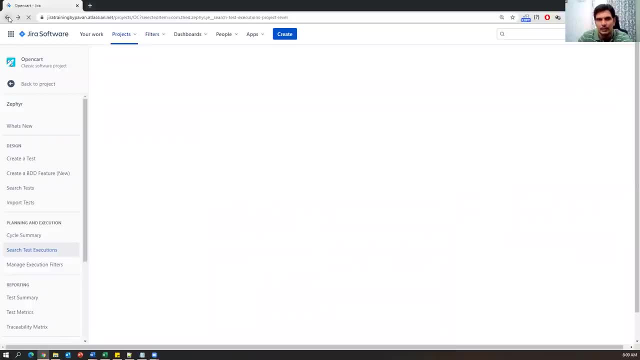 to update the status here. so once it is failed, everything is done. so once you have done all of that, once you click on the test case, you can click on the test case. again is done, go to again, go back right. so once you go back now you can see the execution status. 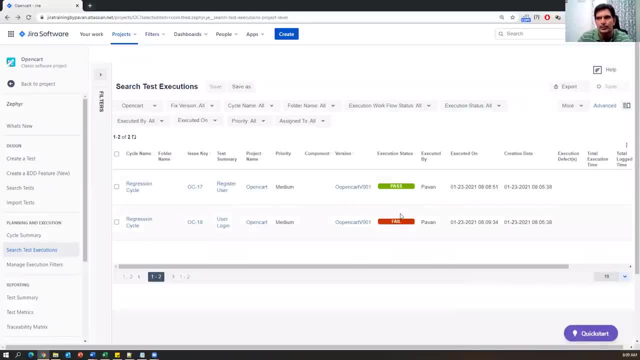 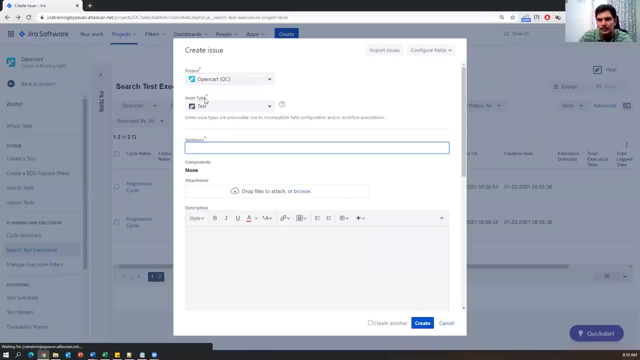 so one is got failed, one is got passed. so now you need to report the failure test case as a bug. right, so then you can just go to create and here, instead of test, you have to select the bug. okay, now bug is selected. now you have to write the summary. so login failed. 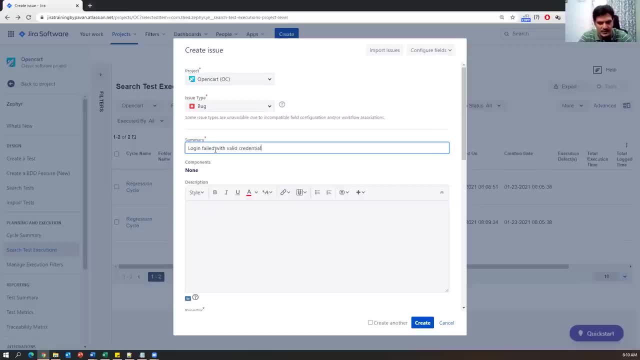 with varied credentials, right? so you need to write all the steps for login, right, you need to write all the steps here and then developer name- so he is a reporter- and fixed versions. so in which version you want to fix so these details automatically populate, guys, okay, your project. 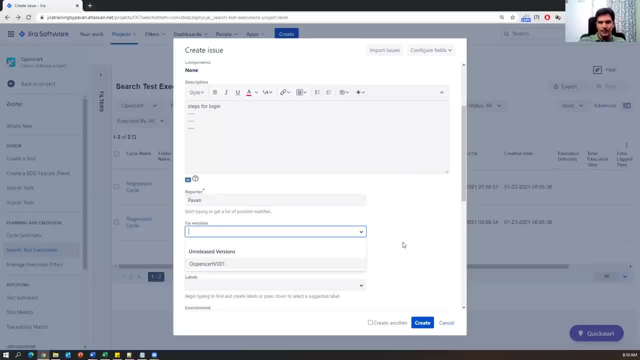 will be set up in the jira before itself. so all the versions, everything will be populated and priority and, as per the jira, by default it will show you only priority. but if you want to get the cvt we need to add some customized options. so the customized options will be added by the 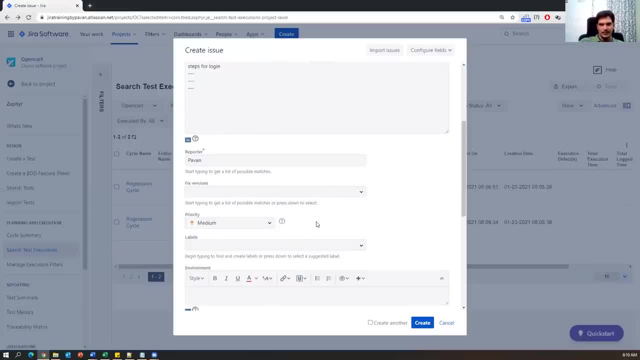 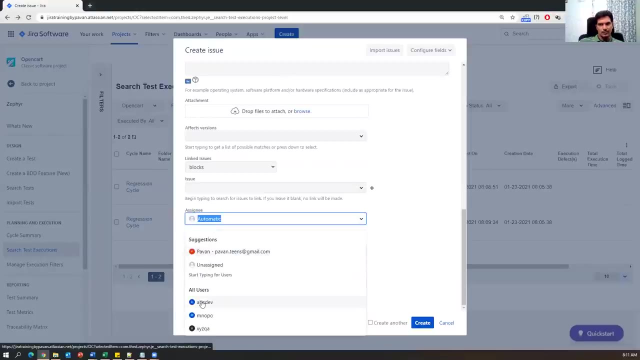 admin, so you guys can also select the priority as well as crt, and then which environment to have executed the test cases and screenshots you can attach here and in which version these bugs are affected. so all these things you have to space any. so we is a responsible for fixing this issue. we have to select the developer name, like this and on we: 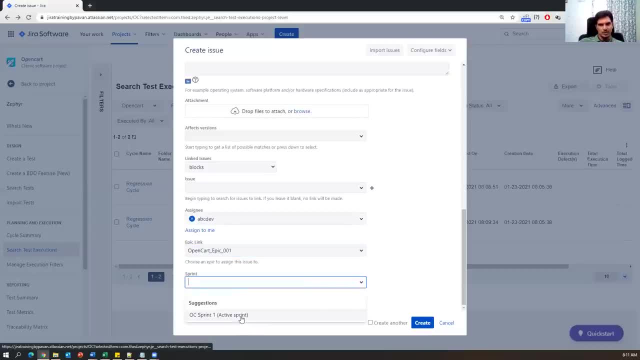 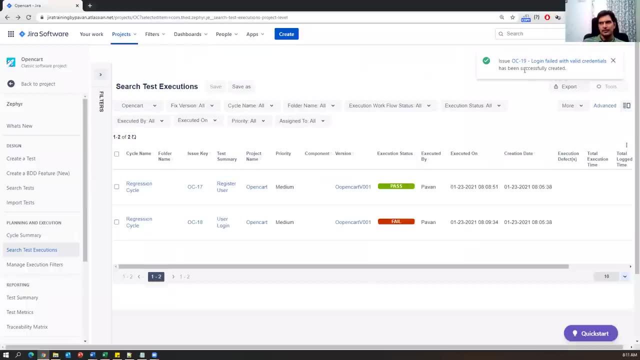 epic. you got this issue. you have to select on which sprint you got this issue. you can spell like the sprint. so all these things you have to select and then create. so this is how we need to raise a bug. so now you can see bug is rise. if i just go and click on this link you can see the. 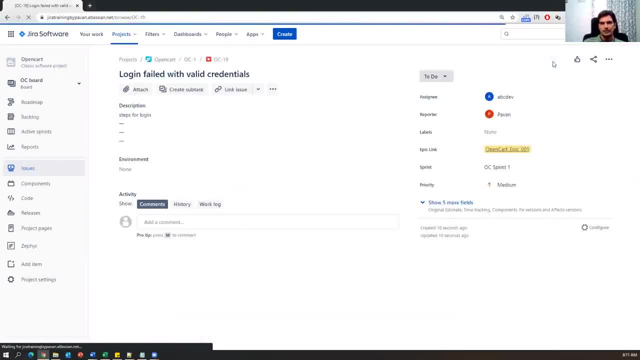 bug information. so this is all about bug details. so once the developer starts working on the debug, they will update the status and they will also write the comments here whether it's fixed or it is in progress and how the what is the status of the bug and accordingly we have to re-verify. 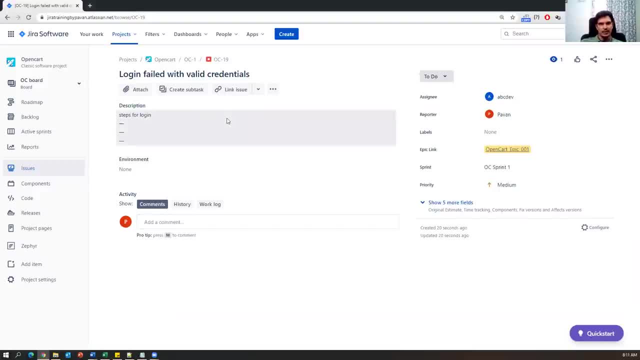 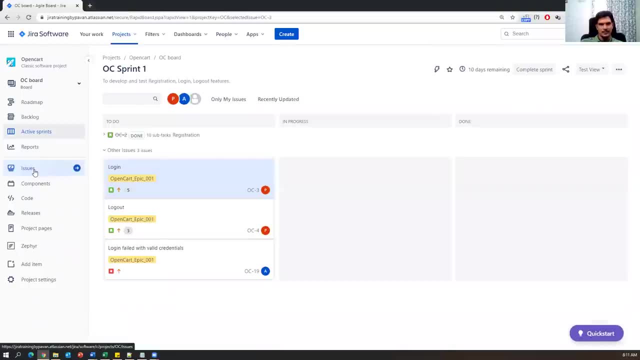 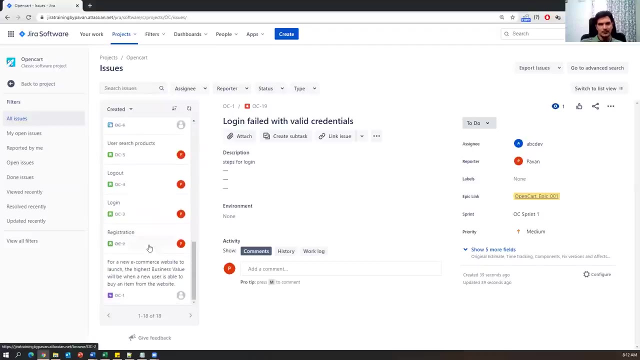 and close it. and if you want to see all the bugs list where you can see, yes, we can just go back to the project again and here you can just look at the issues. right, if i just click on the issues, you will see all kinds of issues, so including stories, tasks, bugs, everything you can see here. 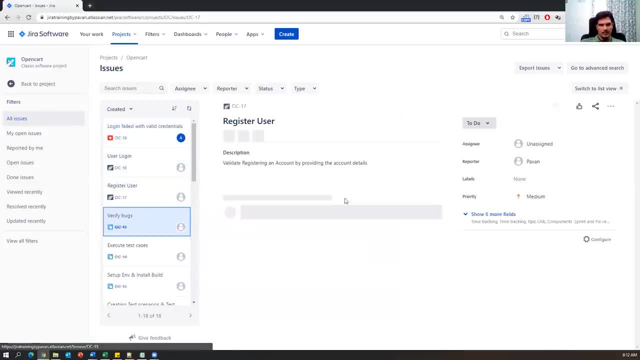 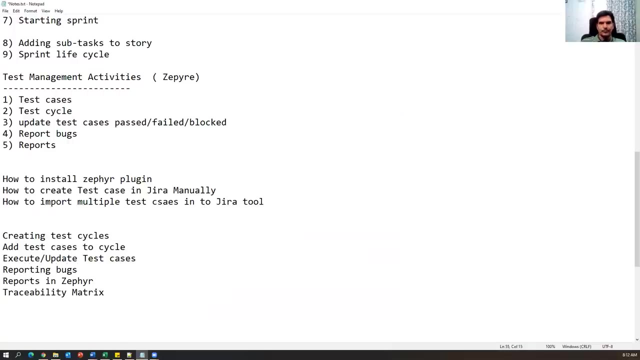 okay, whichever you want to click here, that details will be displayed at the right side. so this is all about bug reporting. so whenever you find a test case got failed, you can report the bug. so we also seen a reporting box and, finally, we can also see the reports. 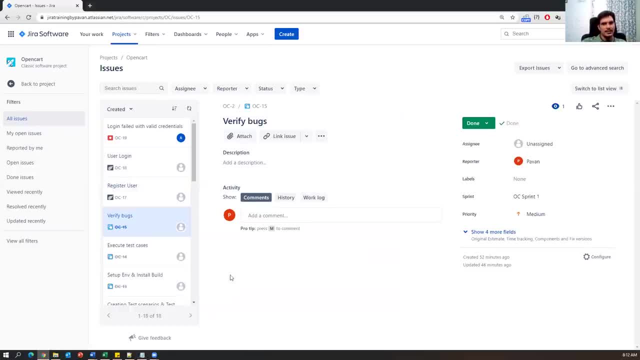 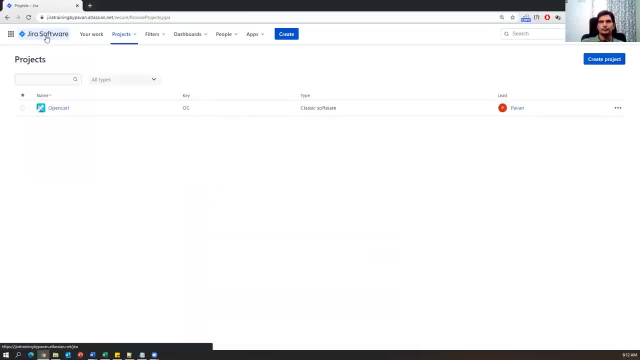 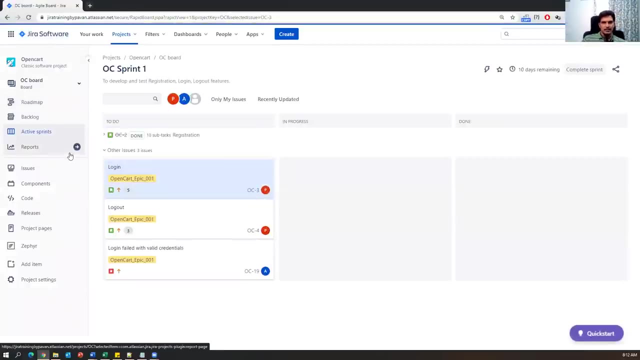 so agile reports will be different. guys, in agile we will see burnt down charts and everything. i will show you that first, and then we'll come back to the test summary reports again, go to the project okay, and then select the project right. so here you can see the something called reports. 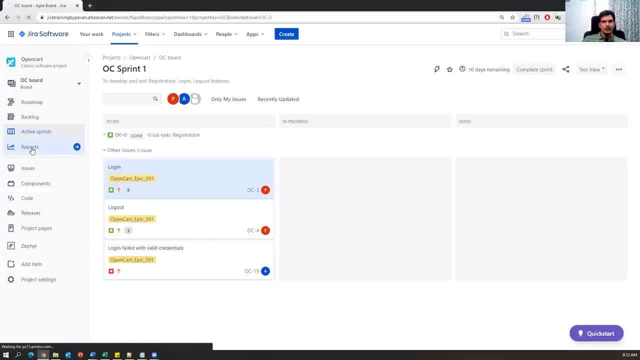 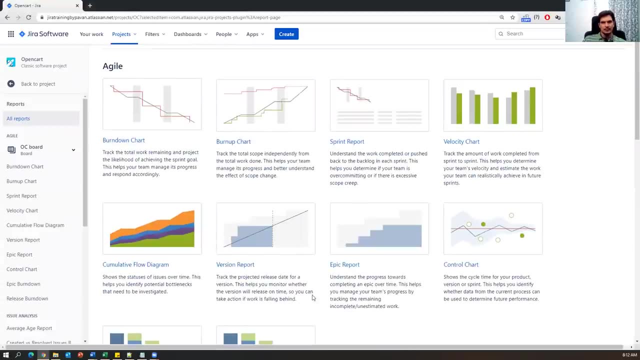 okay, in the project dashboard you can see the reports. so click on the reports. and these are all agile reports, guys, so not a test case reports. now you can see there are so many charts are available, so burn down chart, burn up chart. sprint report, velocity chart, cumulative flow diagram. so 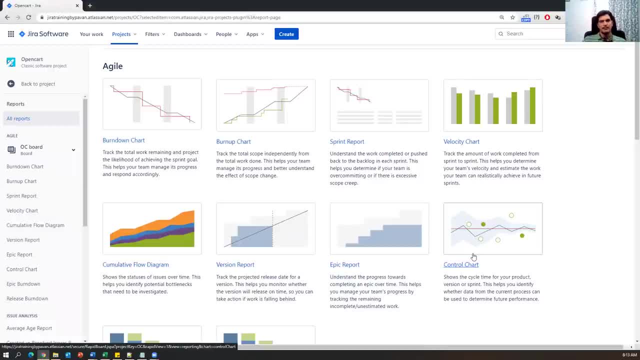 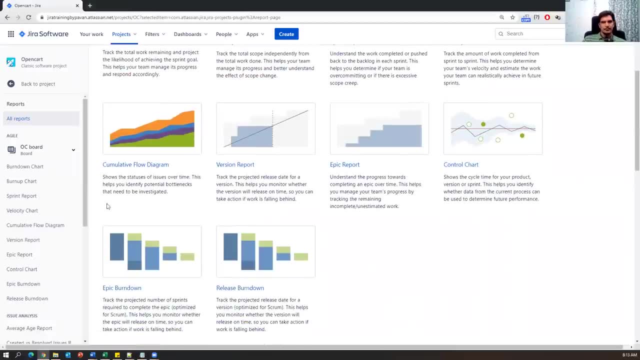 these are all the metrics which will be taken care by the scrum master. so scrum master has to know how, how we can calculate these metrics and how we can check the efforts of the team. and you can just click on each and every chart here: burn down, burn down chart. so this is the chart which is basically. 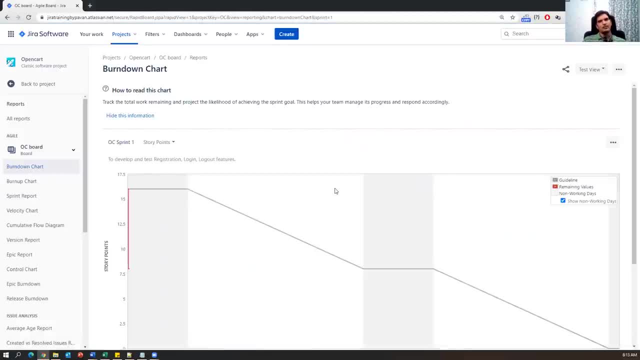 burned down. basically, the main information which will display is how much we have planned, how much we have completed still, how much is pending. okay, so how much? how much story points we have given, how much we uh, how much story points we have expended on the or spend on the particular story. 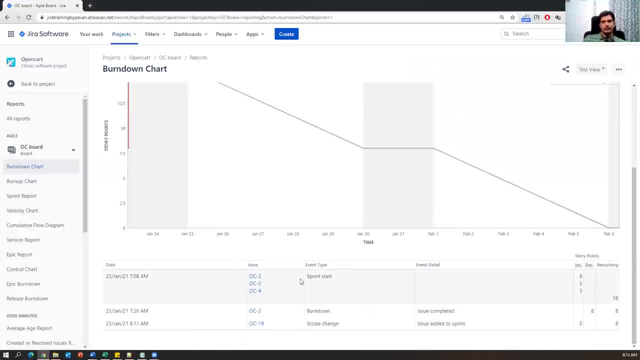 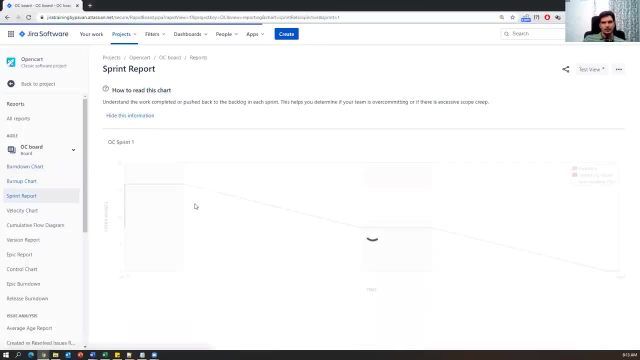 so those details will be displayed in the burn down charts and each and every story level, task level, everything will be displayed. so burn down chart, sprint report- so this is again sprint report. and velocity chart. so these are all automatically displayed in the jira tool. somehow it is not. 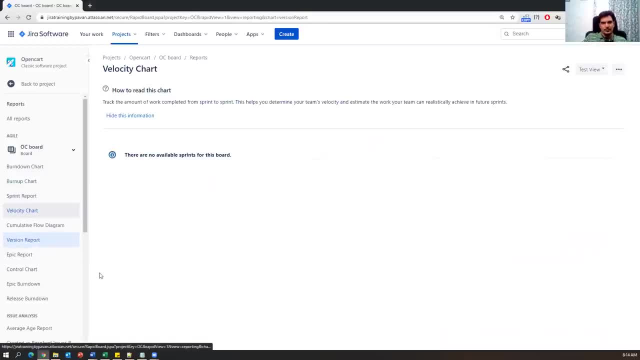 displayed because if it doesn't have proper data which will not display, so version report, epic report, control chat. so there are a lot of things, are there guys? which will taken care by the jira tool scrum master? so he is the main role. okay, he is main, basically driving the process and facilitating. 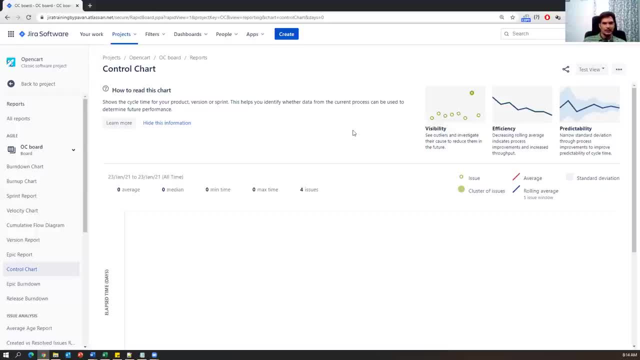 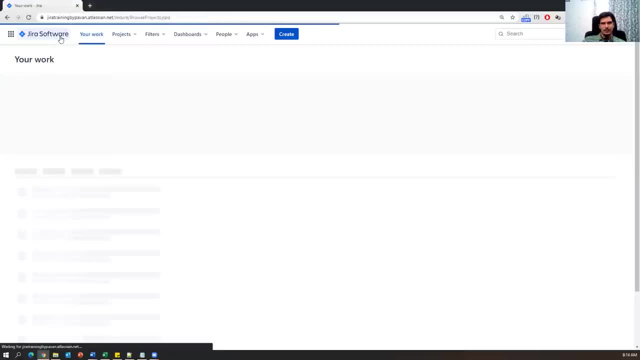 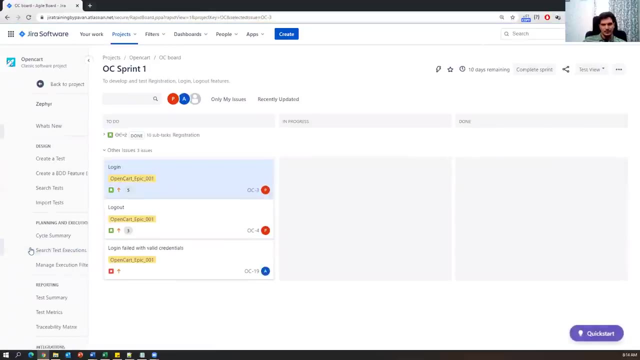 the agile. he will monitor everything. so these are all the agile related reports. but whatever, what about the test summary reports? we need to go to jfile plugin again, go to project, and here there is a project called jfile. right, so jfile all the test related activities. we can. 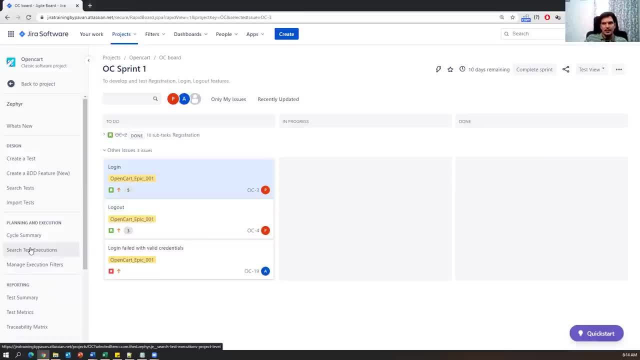 see only in the jfile. okay, because that is the additional plugin through which we are going to, which we have done that. so in the jfile plugin you can see our reporting. test summary, test matrix, traceability matrix. if i just go to test summary, test summary which will give you test: 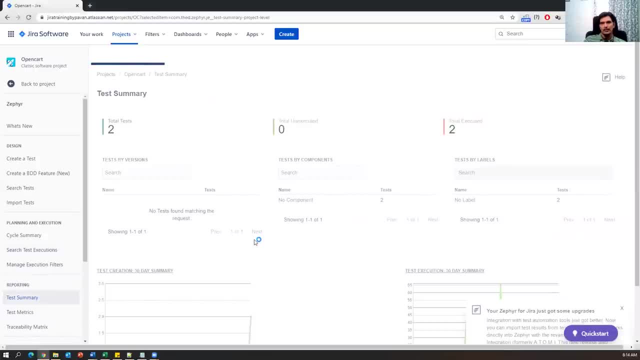 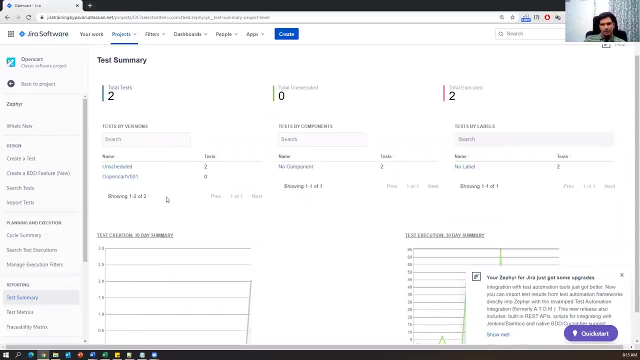 summary report. okay, so you can see here total test. we have created two. two are executed, okay, and everything labels. if there are any labels, so labels will be displayed. if there are any components, components will be displayed. so schedule cycle- unscheduled cycle- will be displayed here. so this is a test summary report. 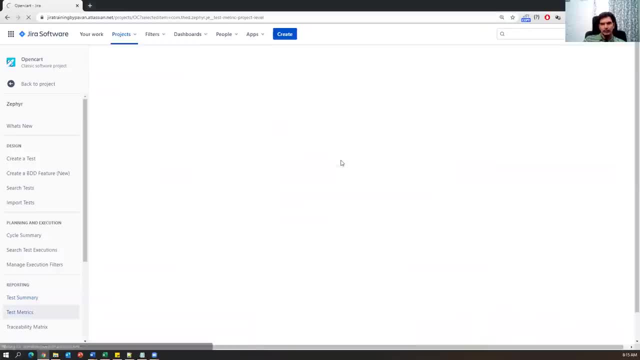 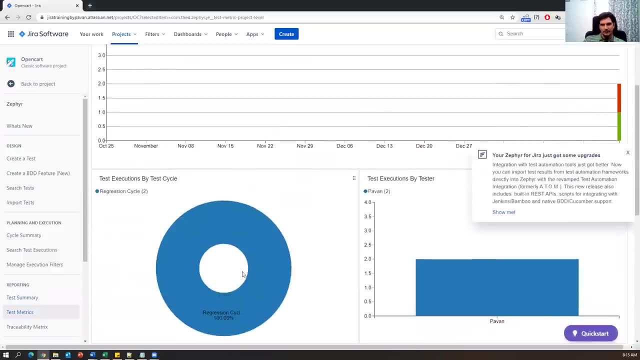 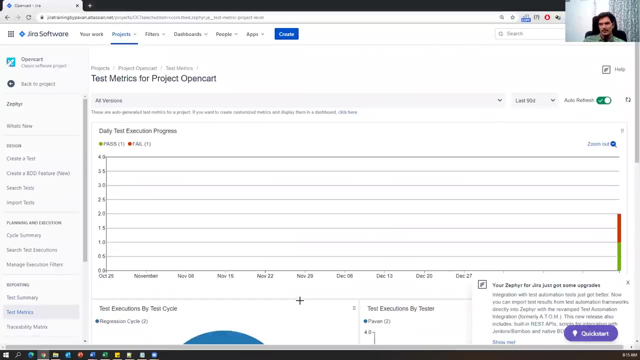 and test matrix. so if we go to test matrix, it will display the test matrix also: how many are failed, how many are passed in the graphical format, okay, which will show you that this is the one type of test summary report. then traceability matrix. these are the three information. 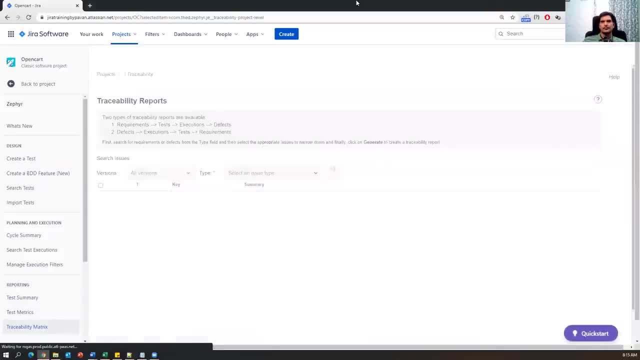 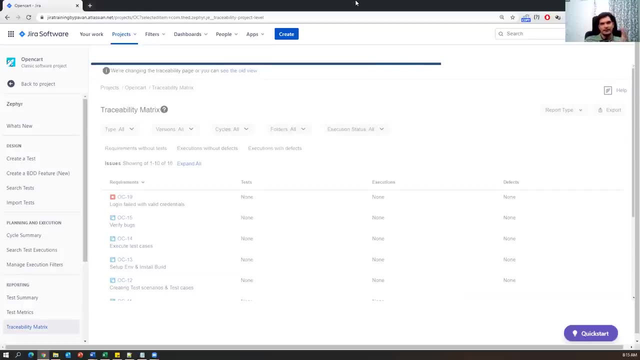 that we need to know in order to know what are the important reports we will have for testing and agile. reports and graphs will be taken care by the scrum master. we don't need to bother about, but at least we need to know what are. the different drafts will be created in agile process in 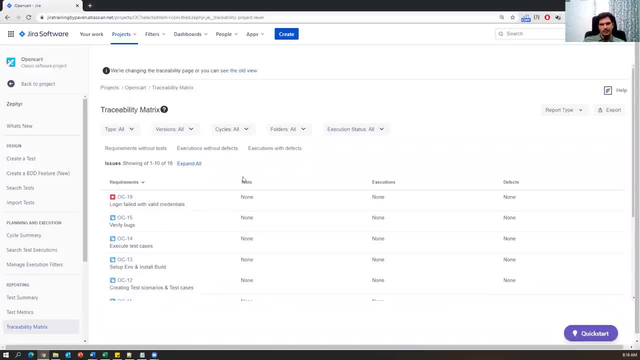 interview people may ask you. so these are the different traceability matrix guys. so what are the requirements we have and what the test we have created executions level defects, so everything will be displayed here. so we have to select the proper. we need to have proper data and we have to map them correctly. 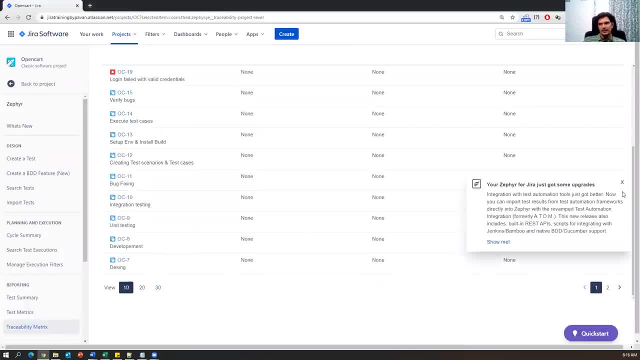 and then only the report will be accurate. right, if there is any mismatching or not, mapping is done like sprint is different test case or different cycle, so then report will not be accurate. so if you provide all the data, test cases, cycles, everything properly, then your reports will be. 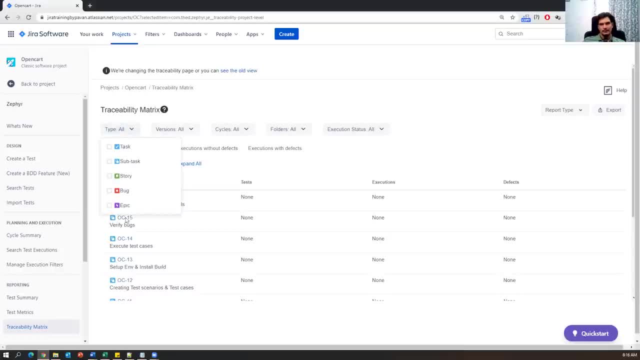 accurate, okay, and you can also filter this: how many, all types, all version, what is the different versions, cycles and if there are any folders within the cycles, we can select the folder level and execution status. how many are passed or many fail. so this kind of information, we can see that, okay. so these are the tasks also we have completed. 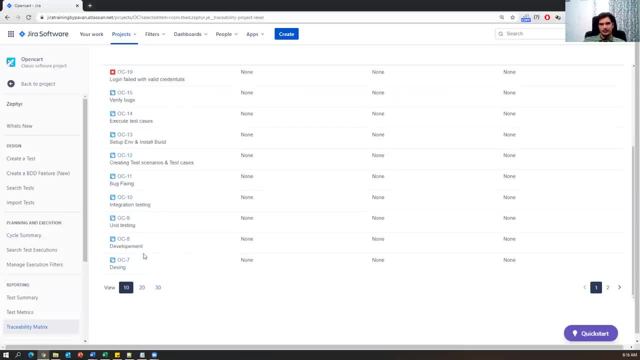 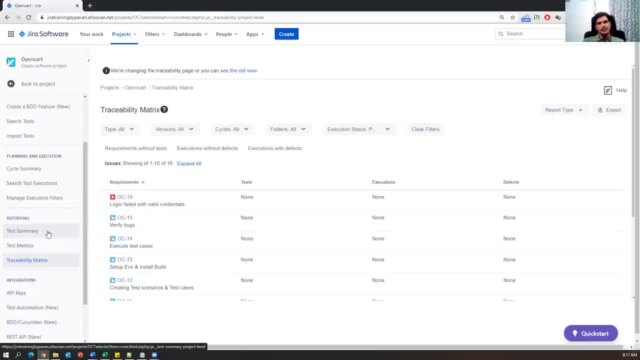 earlier as part of agile right, so that also will be displayed here. so these are the three important uh reportings are there in jira, especially for test management side, and uh charts which are again belongs to agile burn down- burn down charts, velocity charts. so they will take. 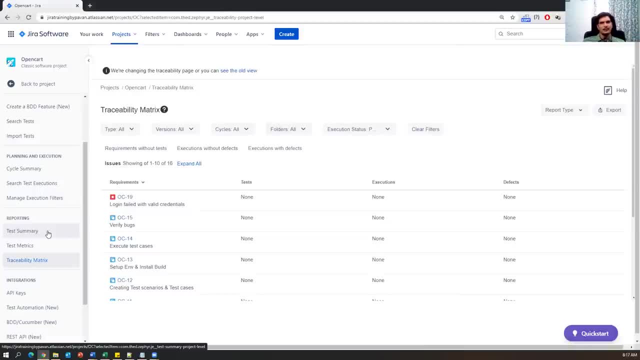 care of our scrum masters. so they will analyze the report and they will check the health of the agile, like how the process is going on, what are the blockers, how much extra time is needed. so those things will be analyzed by the scrum master by seeing those reports and here the test reports we will taken. 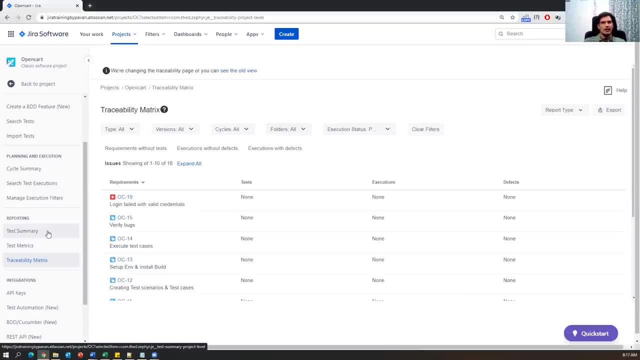 care by us. even our management leads will look at these reports. however, testing is progressed okay, so these things are available and additionally there are some options are provided, integrations. suppose your test cases are automated through selenium or some post main tool or some other api test cases. you can also integrate those tools with the jira, so you 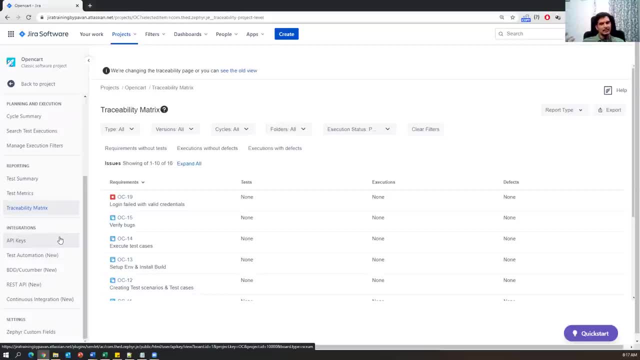 can also execute test cases, automation test cases in selenium and the status we can see in jira also. so for that, uh, some aps are provided here. some options, integration options- are provided within the jira, so by using these options we can also integrate jira with some third-party tools. 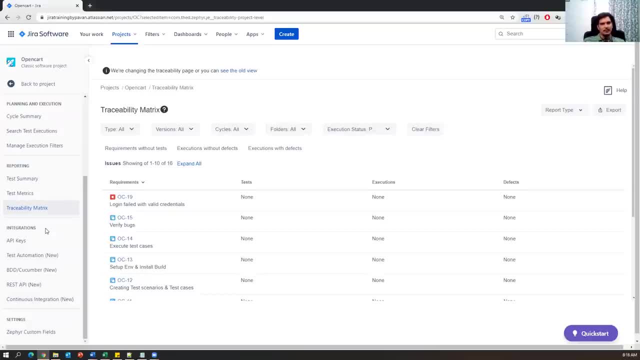 so that kind of facility which is already there in jira by using jeffers plugin, which is impossible, okay, otherwise we cannot do this. so these are all different options are available, very high level and day-to-day basis. we almost work with these options as a test engineer, because different people will involved in the project and different 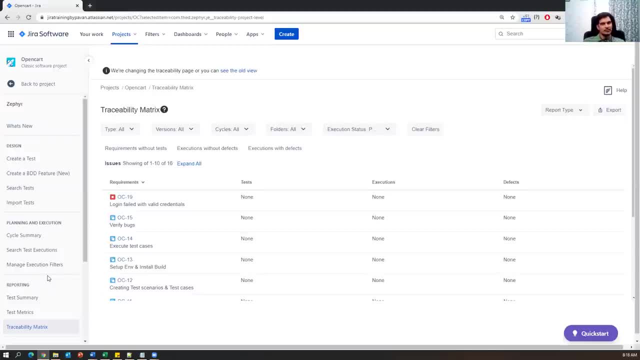 people are having different roles, so according to those roles, permissions will be given and according to those roles they will create the stories. or some people will create the story, some people will add the task, some people will track the status, some people will move the stories to another phase, some people will work on the reports. so depends upon the privileges or 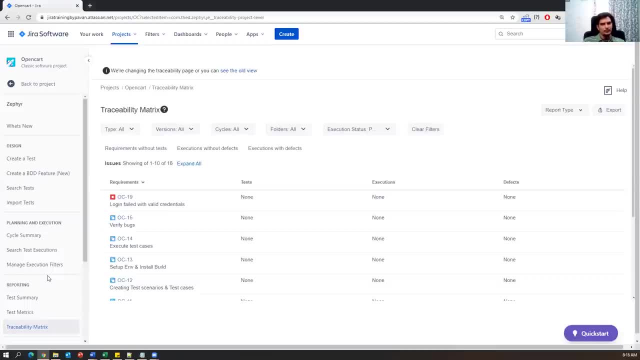 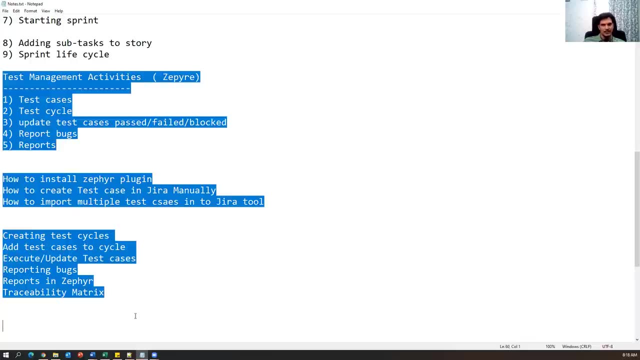 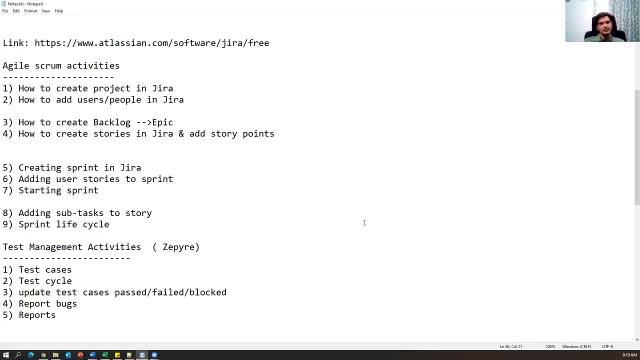 permissions, you will work on the jira tool. okay, so this is all about 0 test management tool. so these are all test management activities and these are all scrum related activities we can do using single tool. so that is the beauty of jira. so in single place we can do everything. 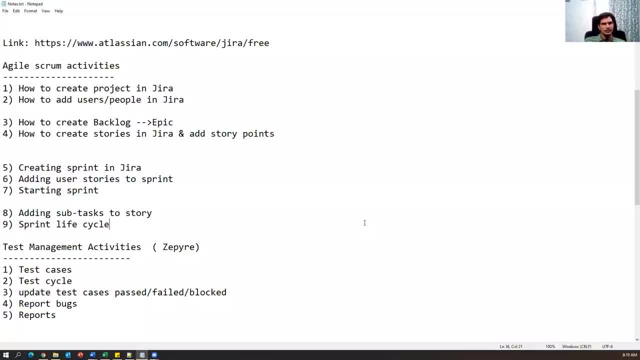 but if i don't use hero, we have to use multiple tools, like for agile. we use some toolir for test management, we use some tool for backtracking, we use another tools. instead of using multiple tools, we can do everything in one place. so that's the reason jira becomes.